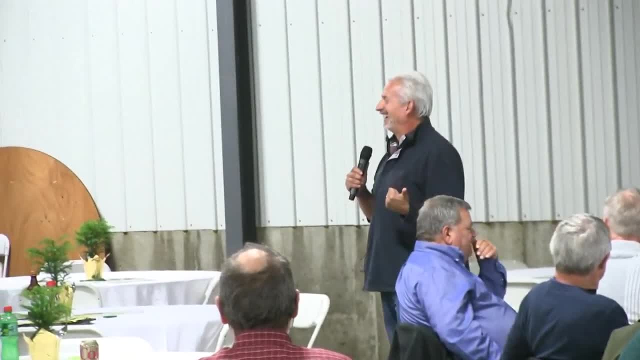 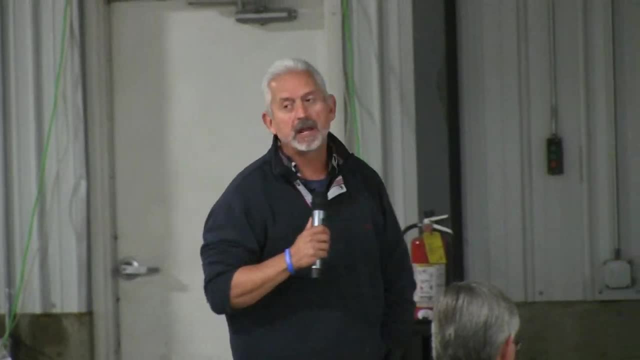 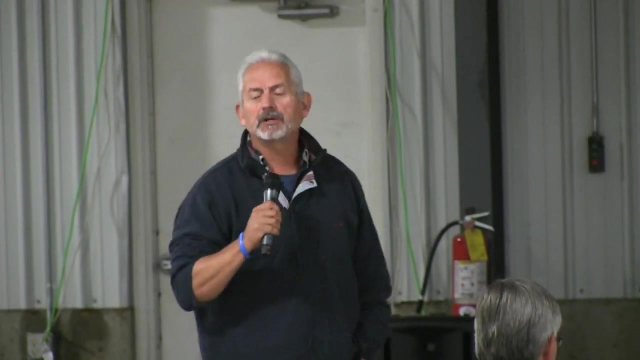 How many here are just lost and ended up grabbing a sandwich? Some of us huh Folks. let me start because I've got a lot to share and this is really about a three-day course. Just recently, we opened up a company: Dave Brown, David Brandt and Dr Ellen Williams. 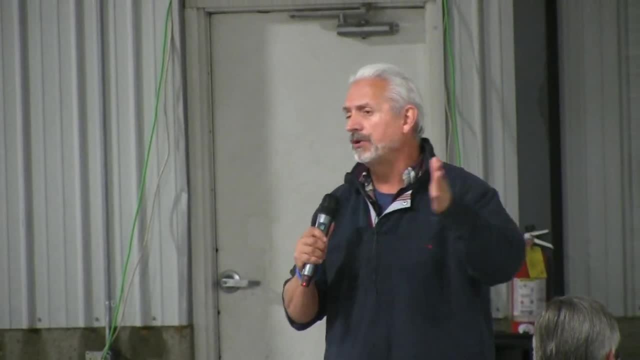 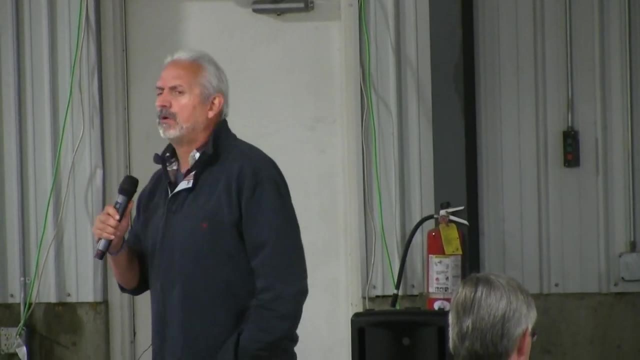 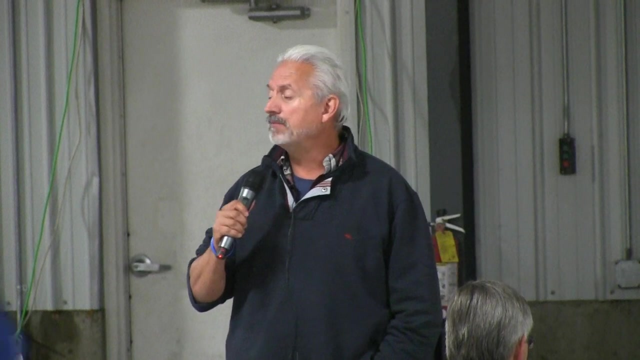 We opened a company, a consulting company, called Soul Health Consulting and Soul Health Academy. The purpose of this whole- starting this- is because we wanted to change the paradigm that's existing throughout the country and maybe throughout the globe. How did it start for us? 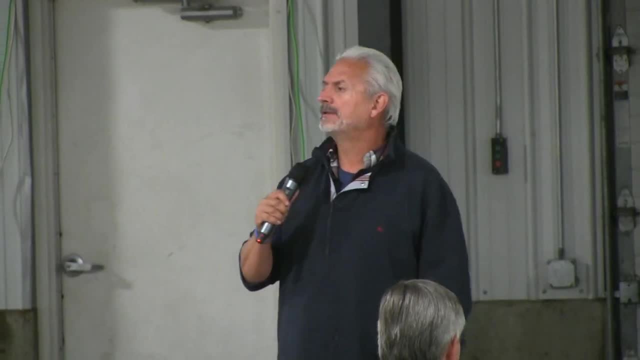 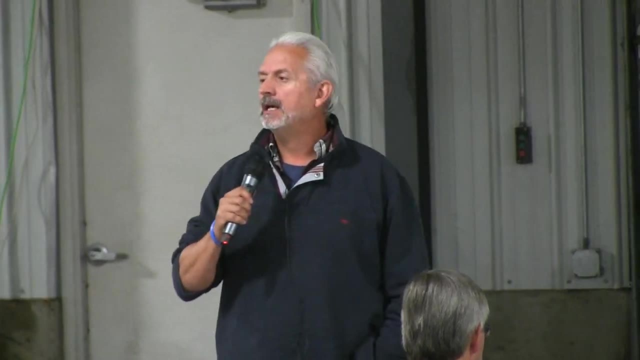 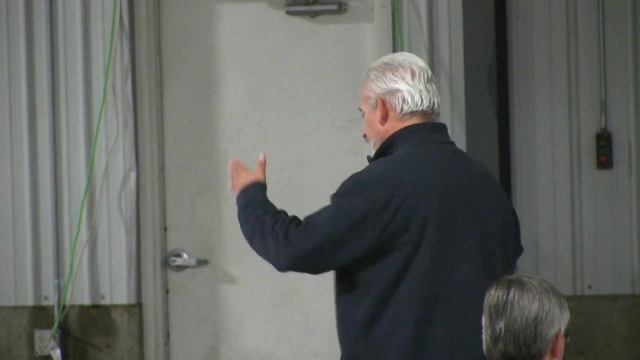 For me it started about 12 years ago. One word: Failure. I was failing miserably as a conservationist, as an agronomist. Farmers were going, broke around me Because I worked in four states, Started off my career in New Mexico. 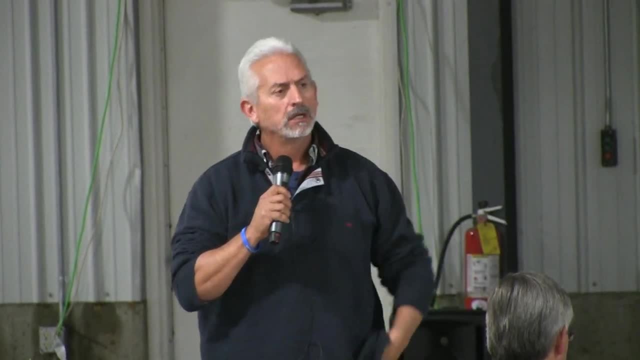 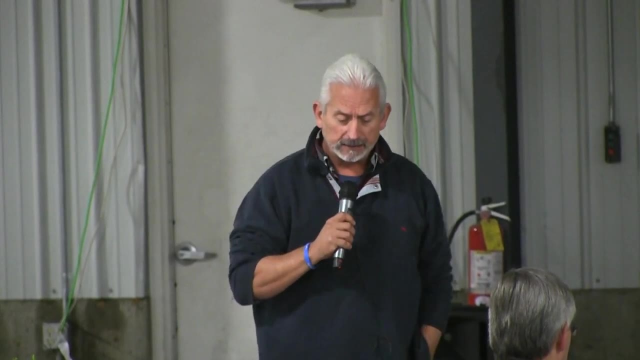 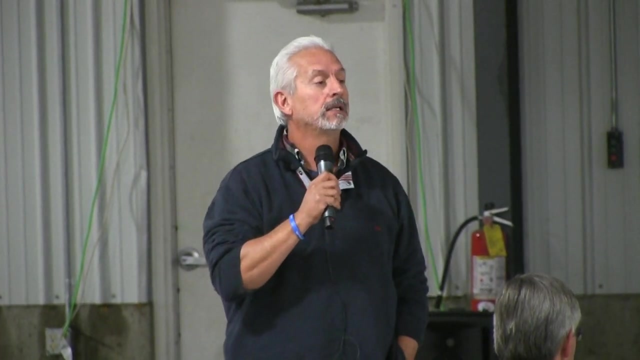 Worked seven years designing irrigation systems, A year and a half as a nutrient irrigation specialist in Missouri- southern Missouri, My wife's from Missouri- Water quality specialist Agronomist And at the last 10 years, 12 years as a soil health specialist. 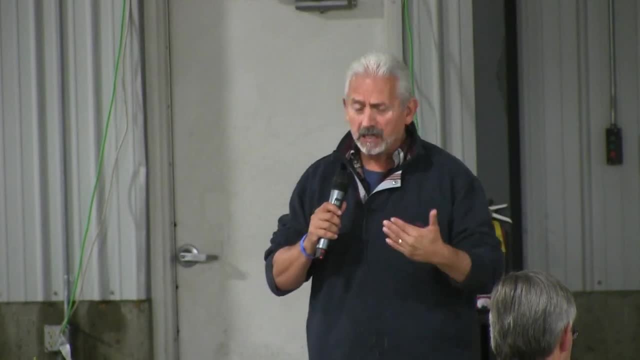 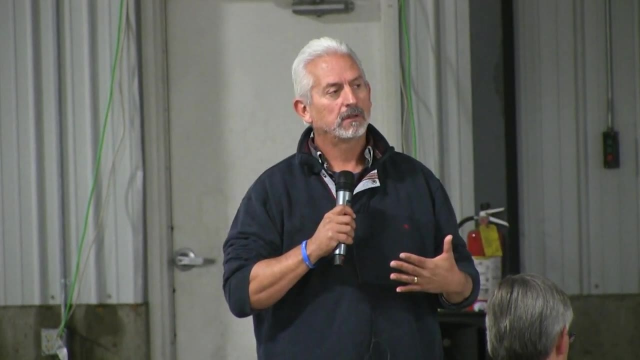 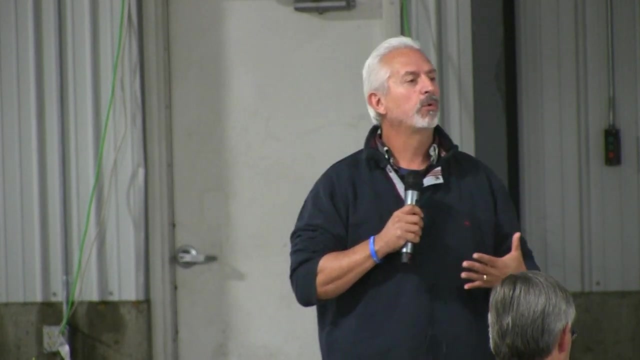 And no matter where I went, I was in the same place, throughout the country. in fact, I was promoting. I was promoting the system that was actually causing farmers to go broke and not becoming regenerative. Notice, I didn't use the word sustainable. 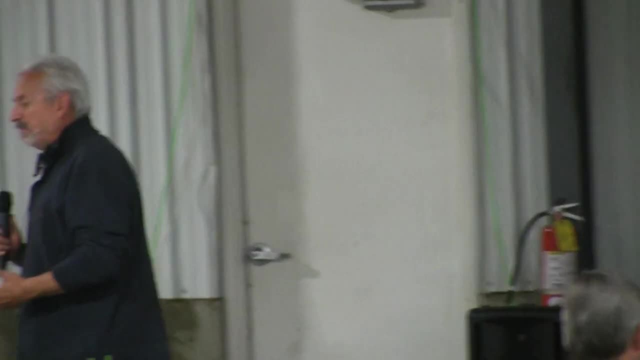 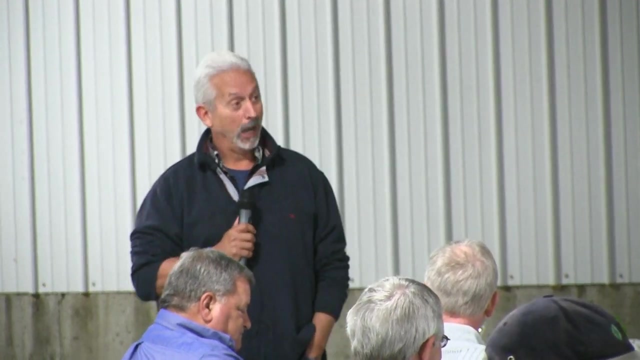 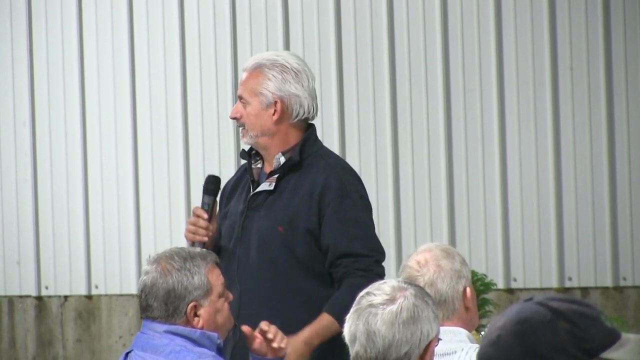 I don't use the word sustainable, because when people tell me, Ray, how's your marriage? It's sustainable. I kind of sucked. What I'm going to talk about is how we can regenerate. When somebody tells me my marriage is regenerative, people are like whoa, I want one of those. 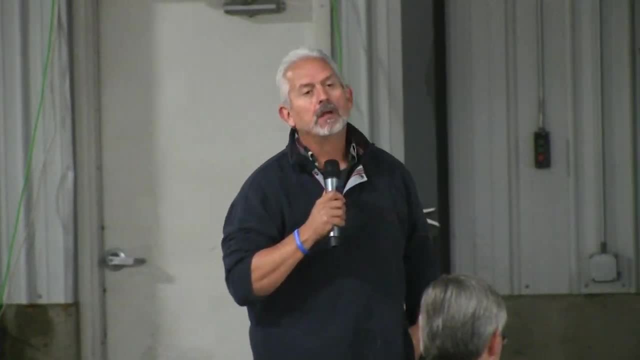 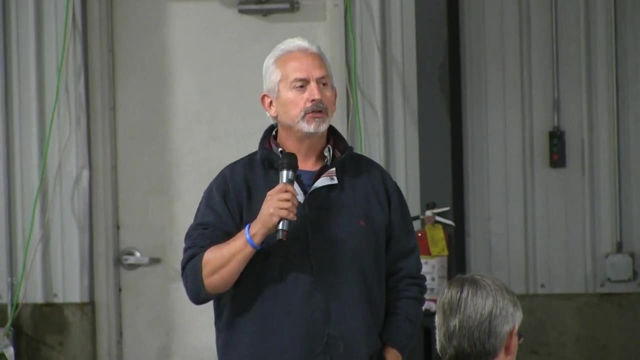 We're here to talk about regeneration, About freedom, About freedom. ladies and gentlemen, We're going to talk about something that all of us do, And I feel like all of us wear a t-shirt as we go into the airport And it says: I am a biologist. 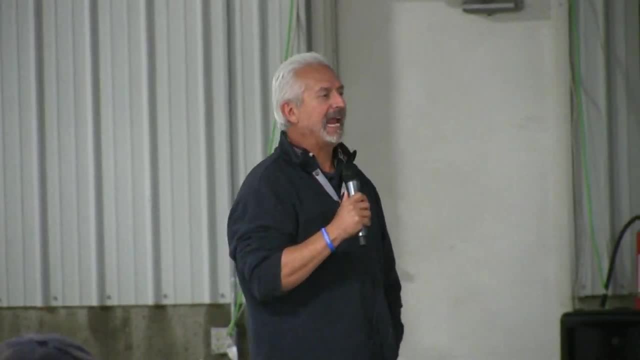 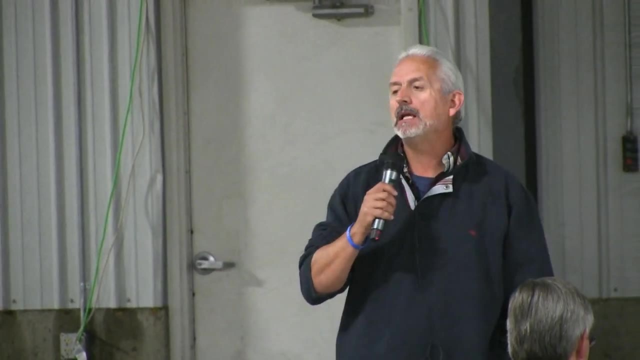 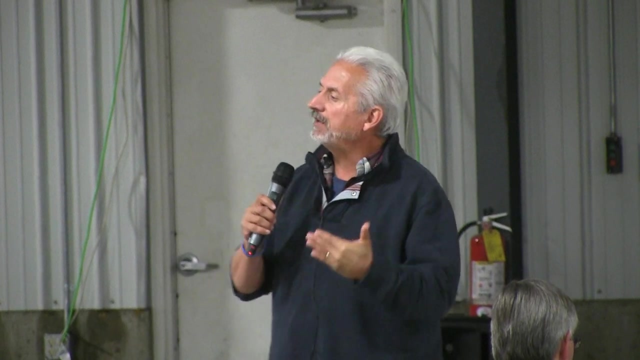 I am a bio-mimicry People go, whoa, what the heck is that Mimic life? We are teaching farmers how to emulate nature, how to mimic life. We're teaching producers to do that And they are saving huge amounts of money. 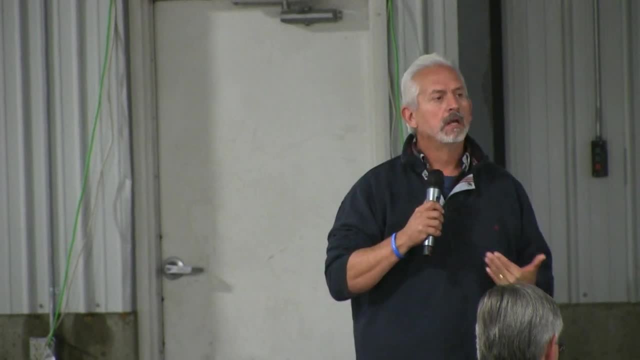 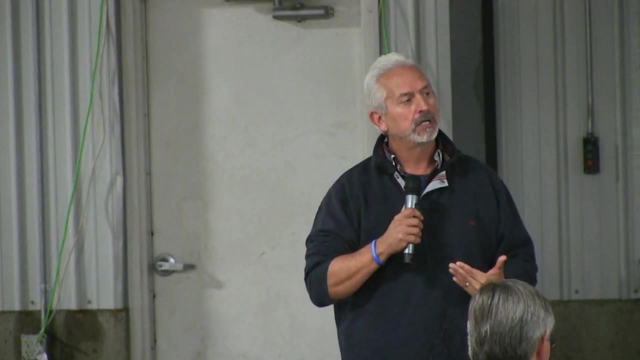 And they're able to bring their sons and daughters back into the operation. There is a silent revolution happening globally, And we were part of it, And it started in the ashes, The ashes of failure. Let's start going down this journey, And before I do that, let me make one more comment. 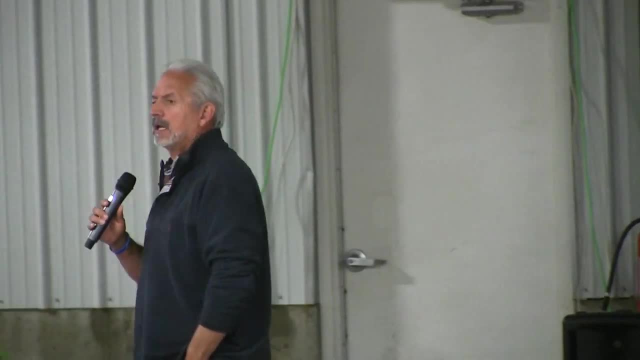 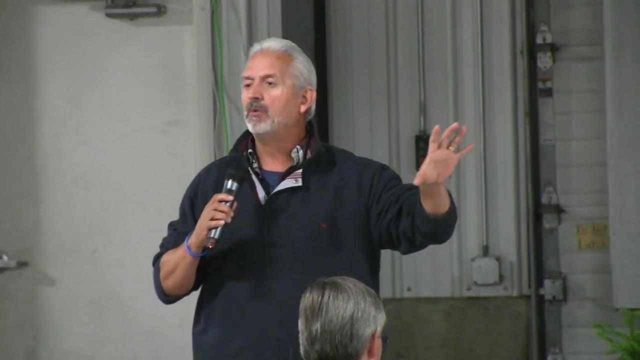 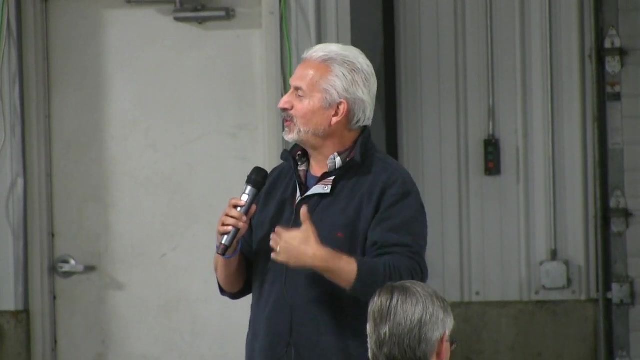 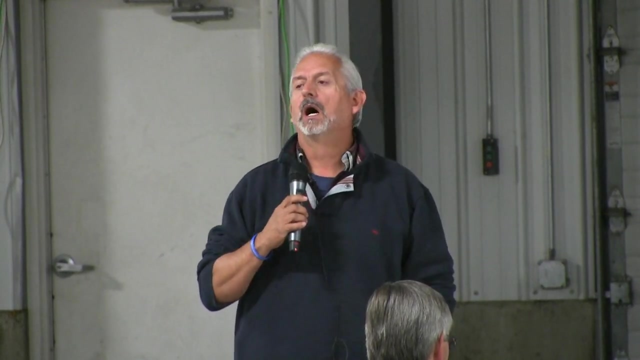 In 2016,. just recently, the Center of Disease came out with a study That, of the top 30 positions globally- I mean in the United States- jobs, the ones that have the highest suicide rate are farmers and ranchers. And I said, whoa, why is that? 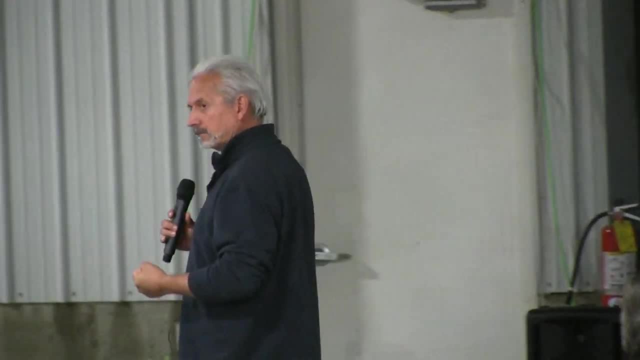 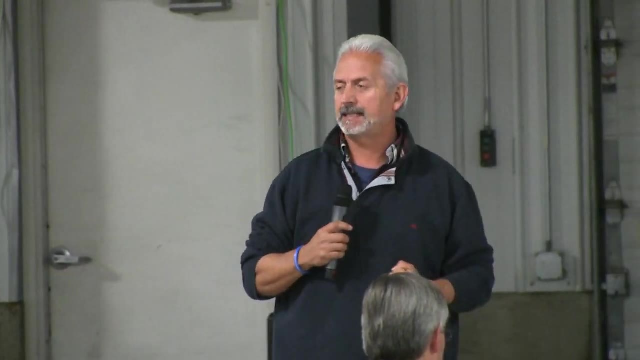 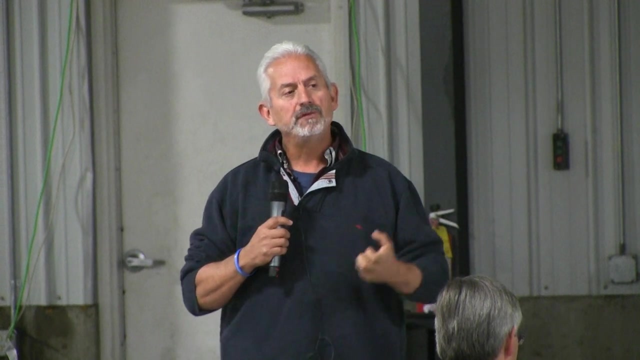 You think about the stress that they're having to maintain The water quality issues that they have, the environmental issues, the economic burden- the stresses that they are dealing with on a regular basis is mind-boggling. I have never seen a group of people like farmers and ranchers which have 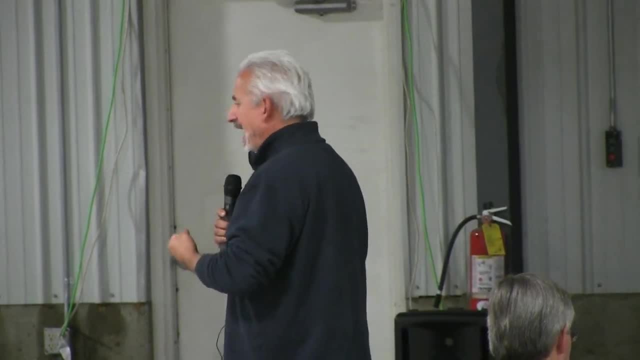 to have the greatest success. I have never seen a group of people like farmers and ranchers which have to have the greatest success. I have seen a single whistle blast right now, But if they talk about this short list, 15 seconds or every minute- 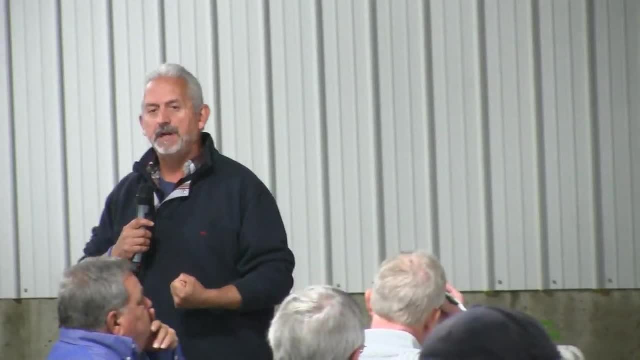 that means that the result of this time is that 40,000 have defected. Let me check my time. We're doing a secret workout 200 hours a day Now. now these morning timelines don't work that well And there's a bad Exposure to Life thing about the human training. 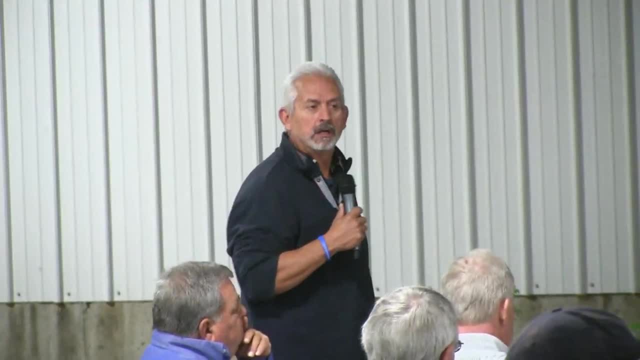 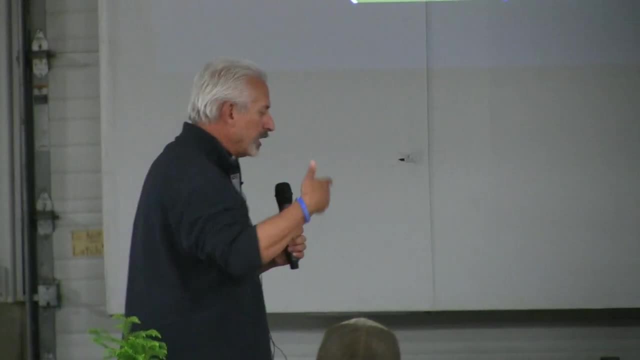 I can't even explain it to you, Because you have to wait 10 years now and you're here. you're assigned. You will be cheated before you know it, but if you do get kicked out of your job because you're out, 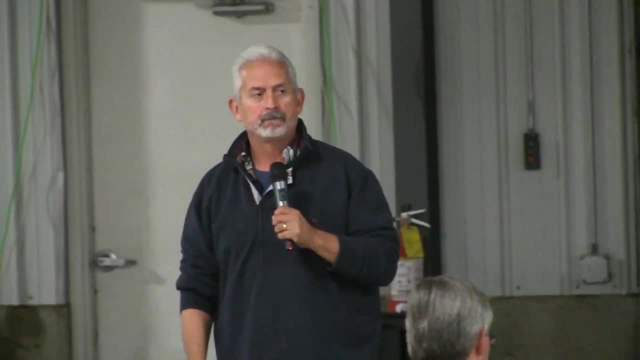 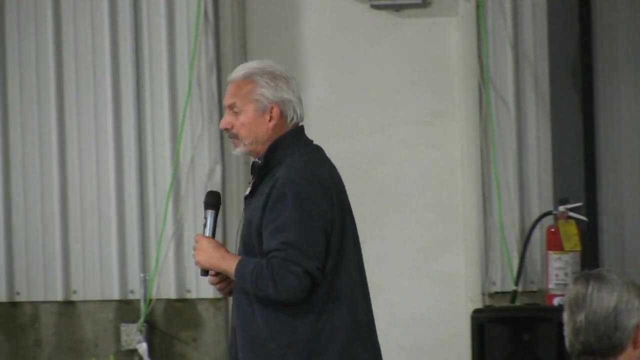 you will beestroffed as a customer because you make all these decisions. That is not something that people try to chase you down to where you want to be, so bad. So how are we going to bring this about? What I teach is these principles, and NRCS teaches four principles of soul health. 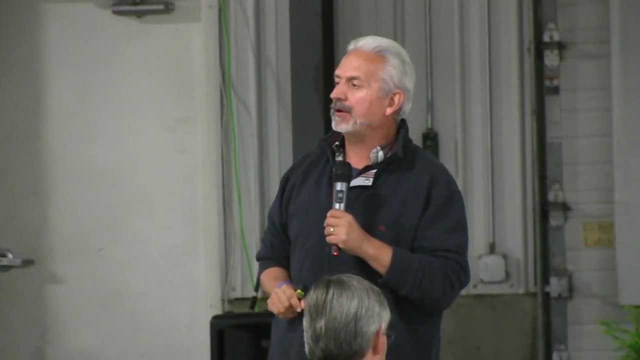 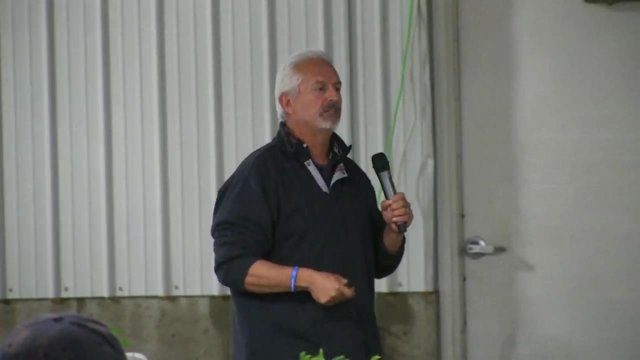 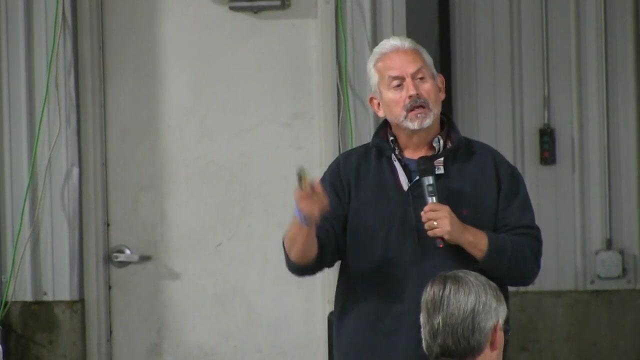 I teach eight. Would I ever get NRCS to embrace? they'll do the grading. maybe they'll accept five, but they will. I don't think they'll ever ever embrace the other three, And the other three are more critical than the other five. 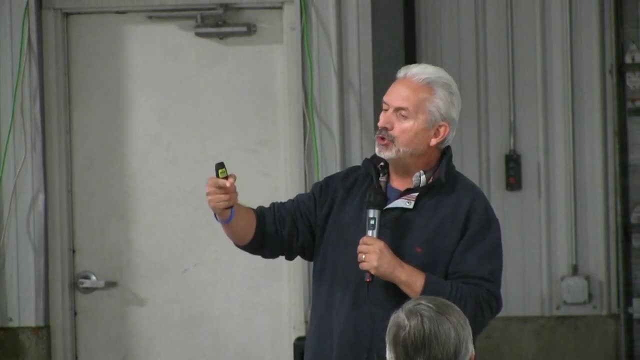 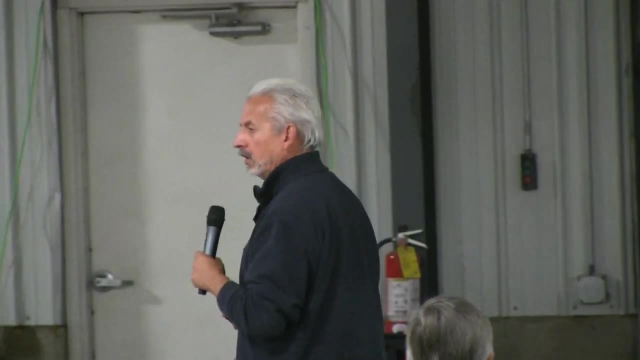 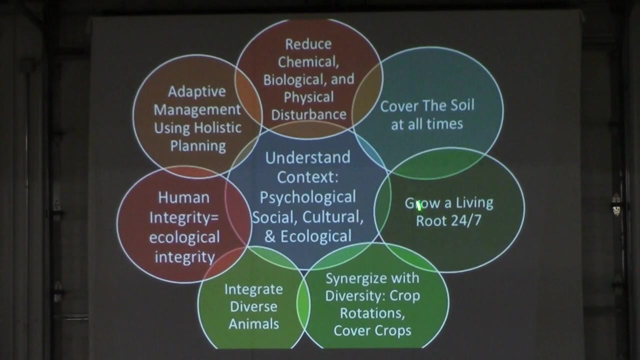 The principles I'm going to teach you, ladies and gentlemen, today. if you apply them judiciously, you will change your life. you will change your soil. When you change your soil, you will change your life. These are the ones I focus on and I'm going to go through them all. 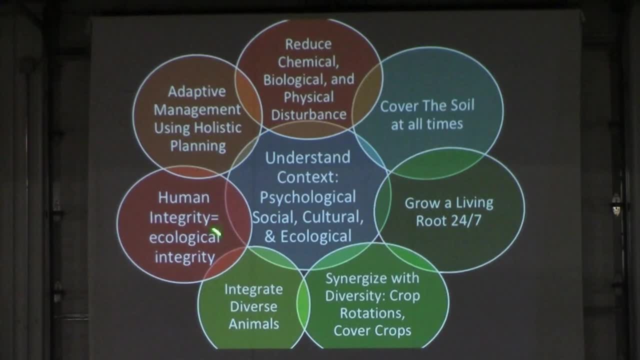 These are the five towards the ecology. These three are towards the sociology. See, if you do not focus on these three, you can't do the other five. You won't do them, You will fail. Let's start down this journey. 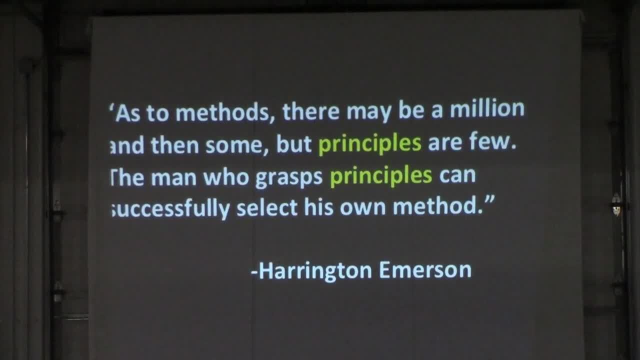 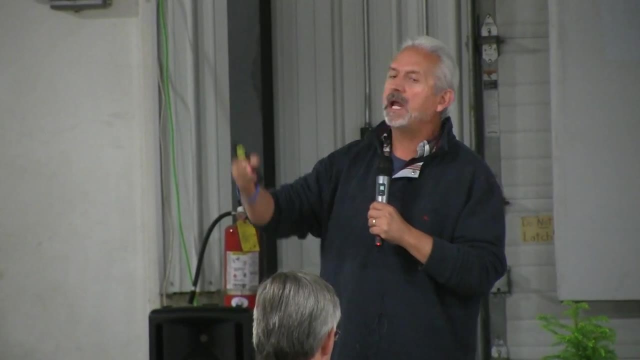 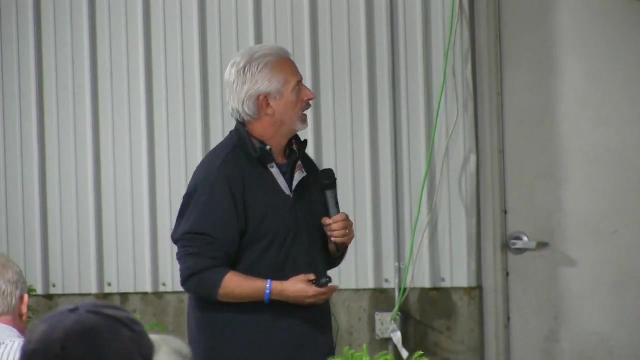 I'll explain. First thing I tell people focus on principles, Principles, the principles of soul, health. These are internal principles in the physical plane, with ecology. This is the way the natural system works. I did not make them up. I am not smart enough to make these up. 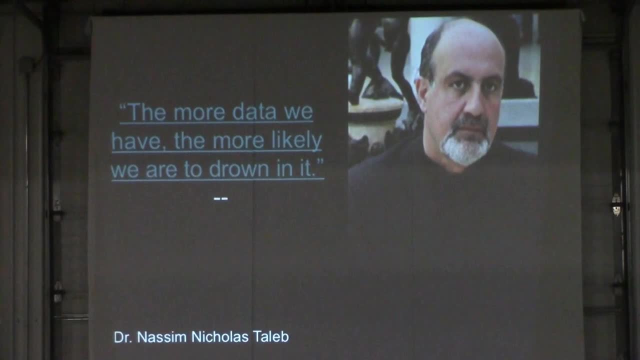 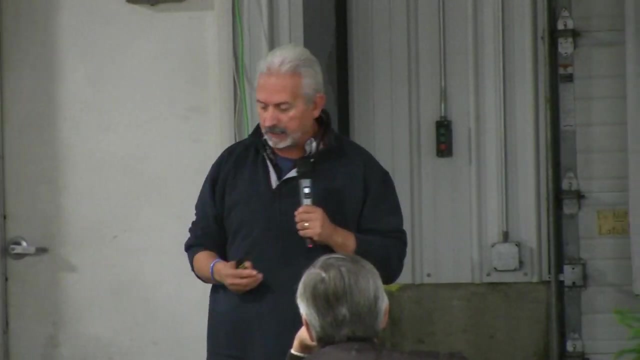 It is principles, Folks. if you ever read any of his books, Dr Nassim Nicholas Taleb- he's a statistician- wrote some wonderful books: The Black Swan, other great books, New York, Best Time, brilliant mind. 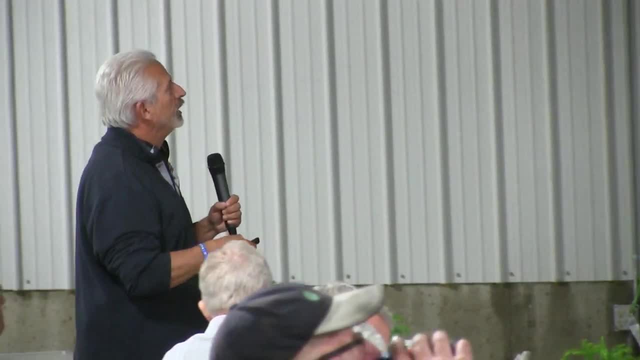 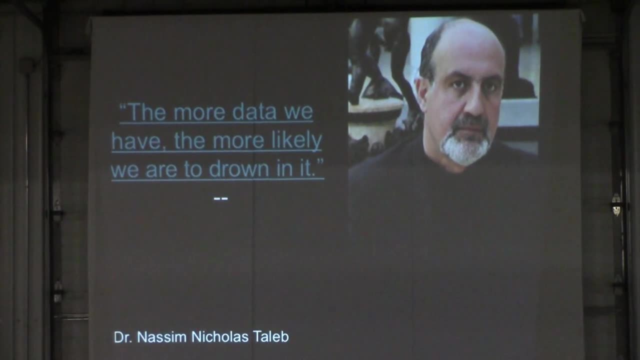 He's a statistician. I love his quote: The more data we have, the more likely we're to drown in it. I want you to focus on principles. See, anybody can make their data say whatever they want, but are you flowing with the principles? 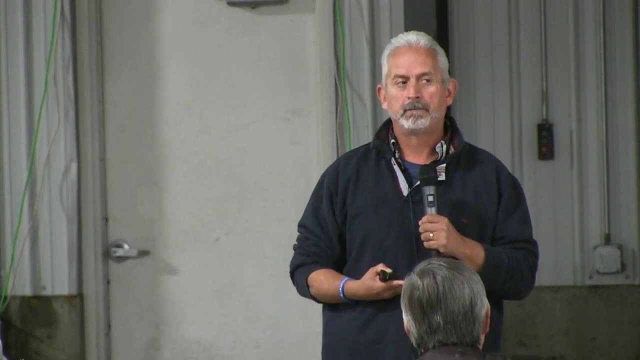 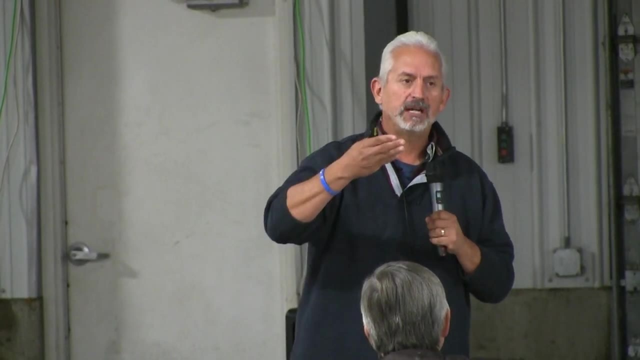 of soul health. They say: are you working with the natural system? Please don't misunderstand me. Data is important, but it's not the nexus, It's understanding principles. because if you understand the principles, when the time gets rough, You will follow through. 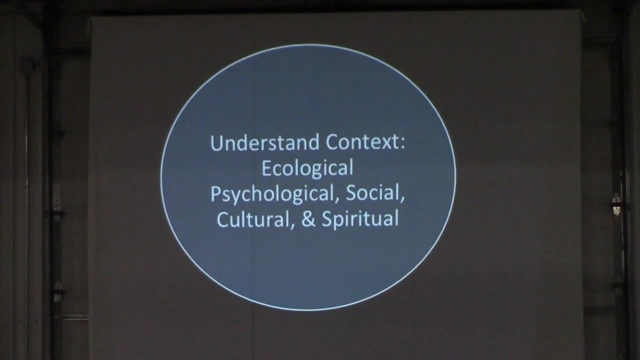 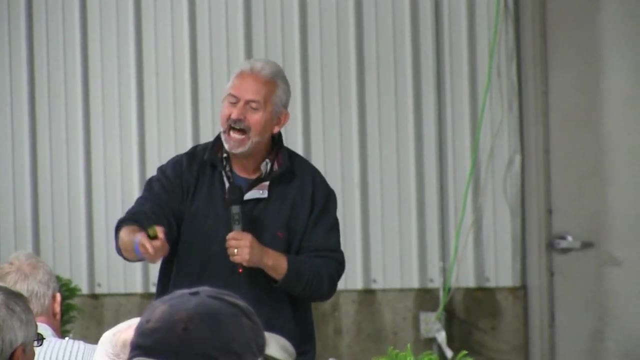 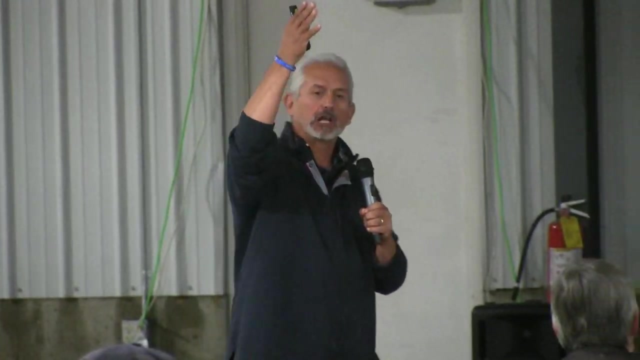 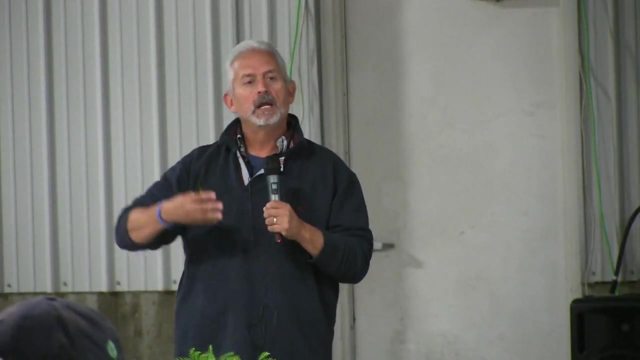 Okay, let's start off with the context. My favorite English word: context, context, context. it is powerful. You always have to understand context. You have to understand your ecological context. Where are you in the region? Social and cultural context. the most difficult thing to work and bring soul health into a. 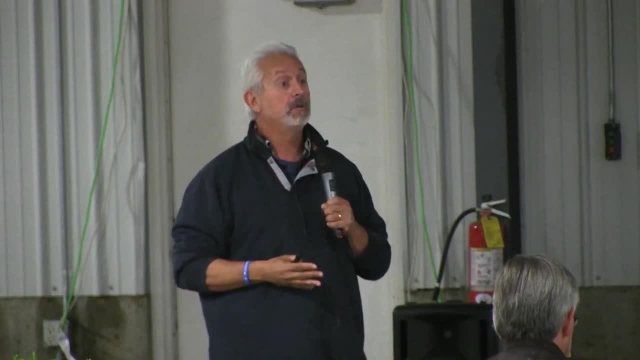 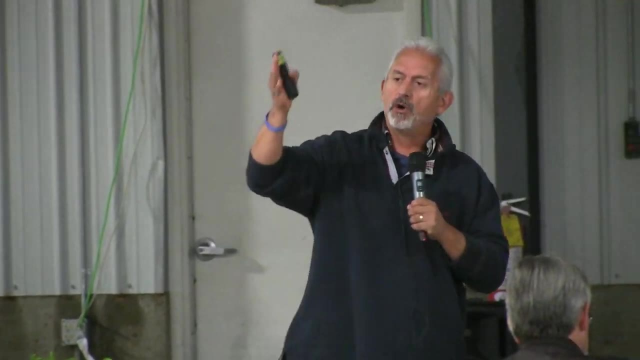 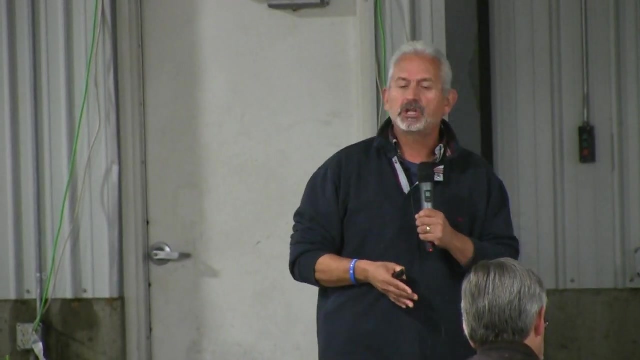 community is the cultural and social context of the community. If you go to Southern Indiana, very Germanic area- a lot of German farmers. Those farms are black, The soil is black, There's not one weed. That's the homestead is. you can eat off the pavement everything that's in place. 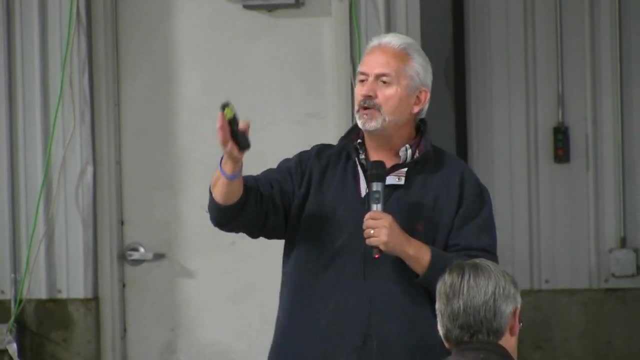 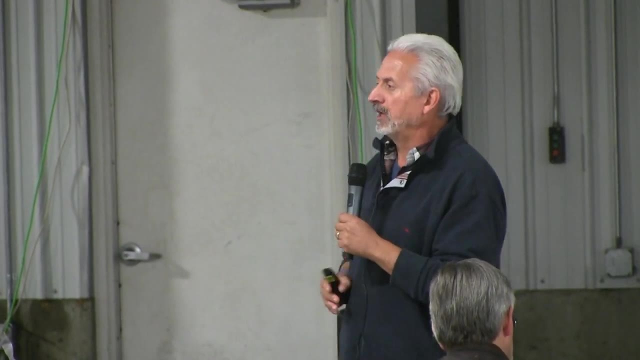 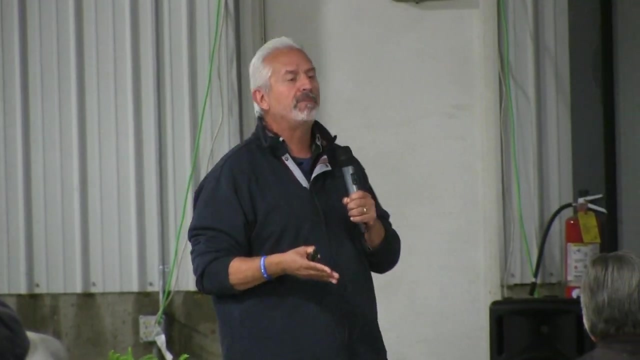 And those who use cover crops and have that during the time when the other farmers are not doing Okay, looked at as bizarre and strange. In fact, I had one rancher in Idaho. He went to no-till. He said, Ray, when I would go to the coffee shop, they would verbally. 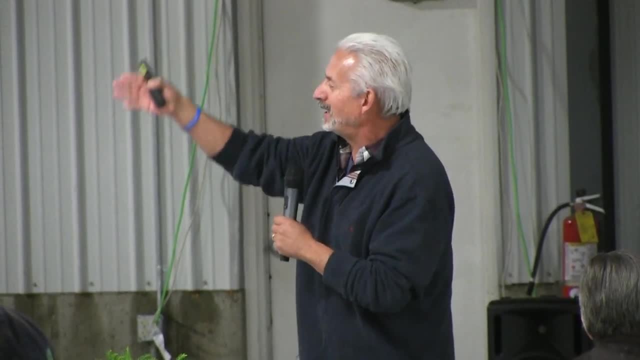 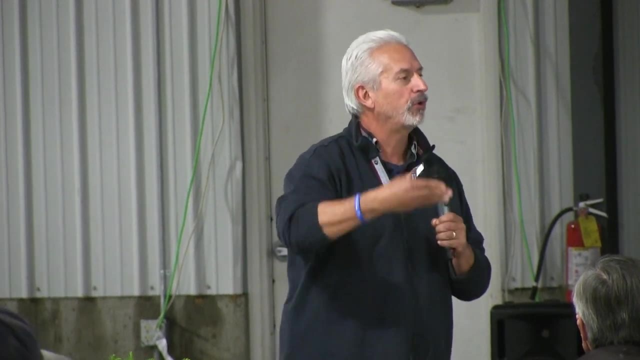 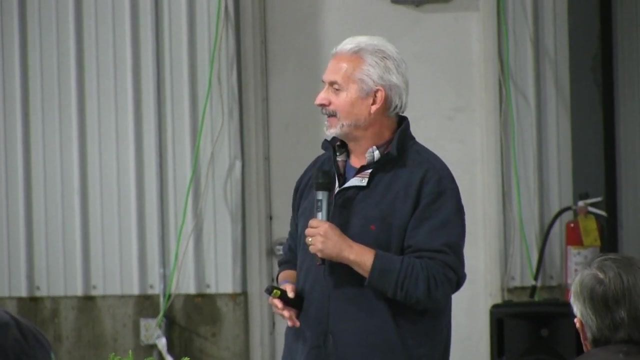 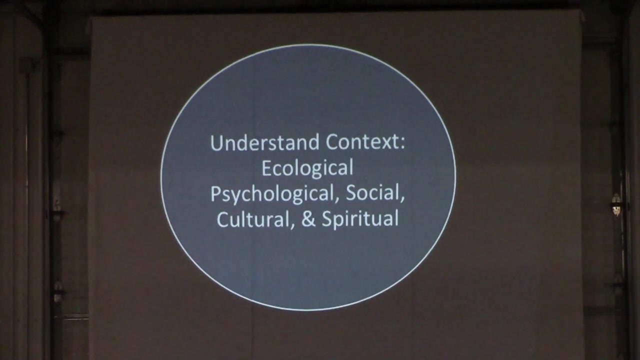 abuse me and say you are degrading the resource. We need to understand the biggest pressure we have is community, social, cultural pressures on the local area. You start doing something new, the pressure is intense. The other aspect of it is the spiritual context. If you go to Hawaii, the Hawaiians to them, the ecology. 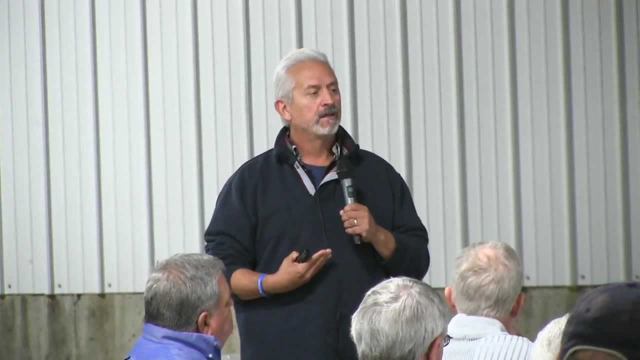 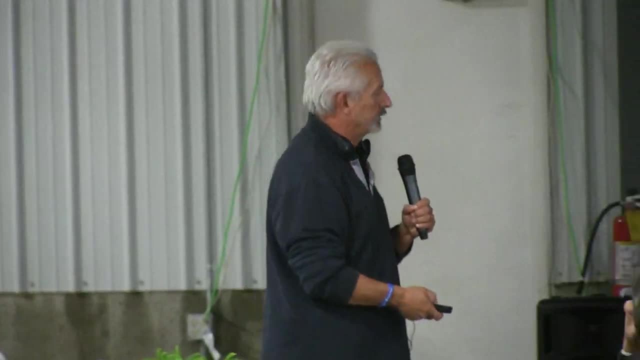 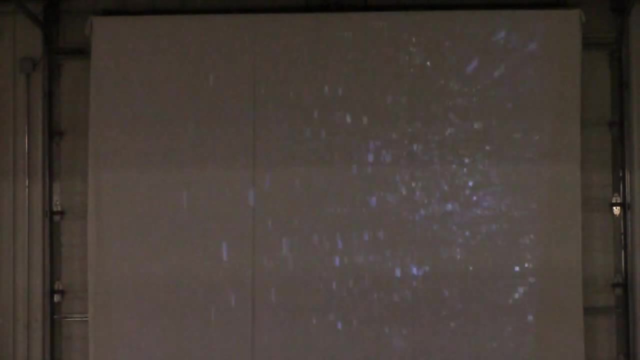 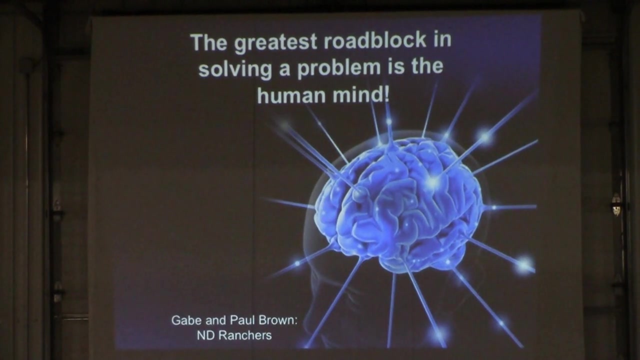 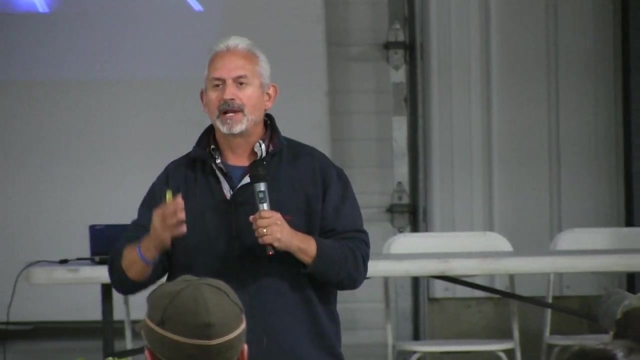 why I'm so focused on context. This is the biggest problem right here. I'll never forget this young Amish farmer, young man in Pennsylvania, Daniel. We were doing the demonstrations and all of a sudden, real strong German accent- He goes. 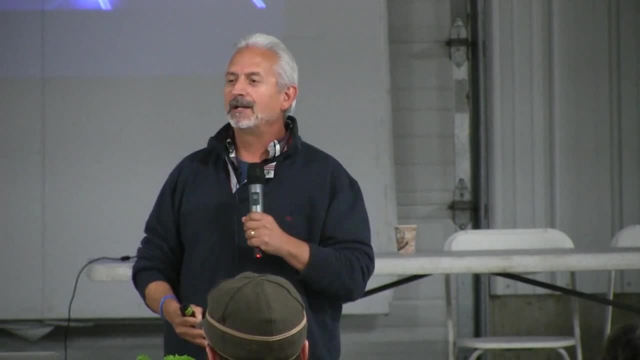 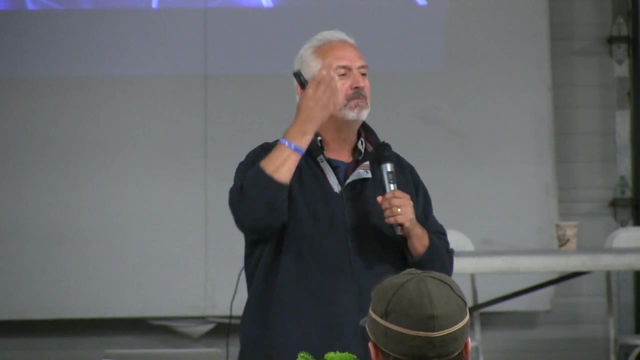 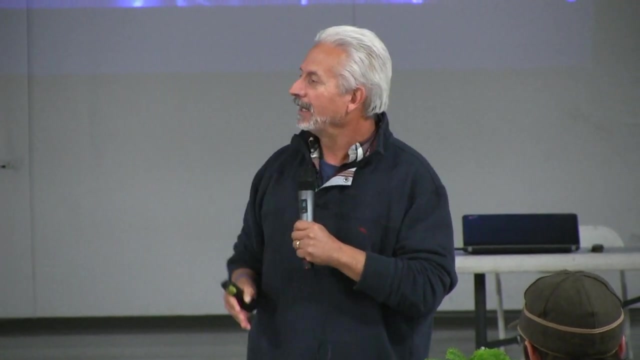 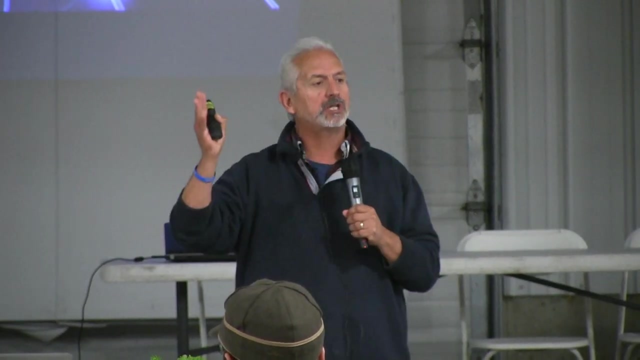 oh, Ray, I get it. I said Daniel, what did you get? He says Ray, the problem is the compaction between my ears. i said, daniel, bless your heart, tillage can't fix that. you got it, daniel. the biggest issue that we have for failure of implementing a new system. 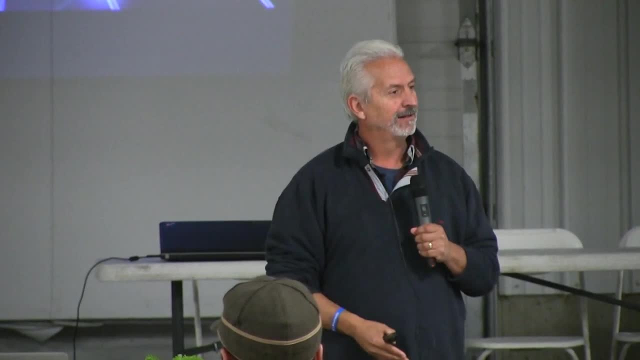 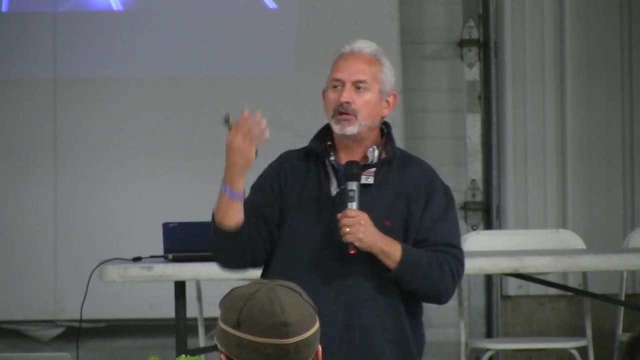 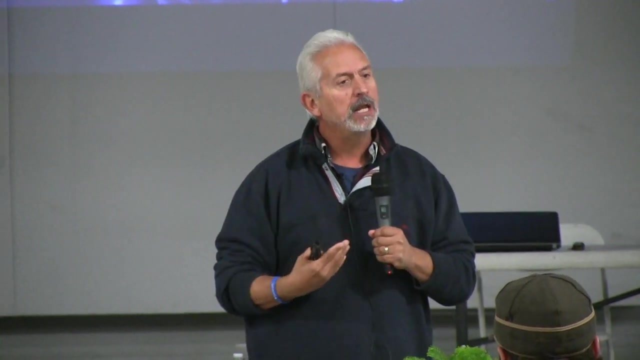 or understanding is your mind. it is your own mind and your own heart and the way you look at the system. you cannot bring your conventional thought process into an ecological, living dynamic system. well, we were taught. it was totally from a different premise, let me continue. so the biggest 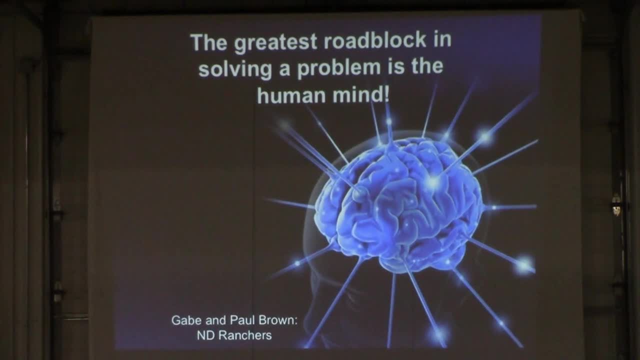 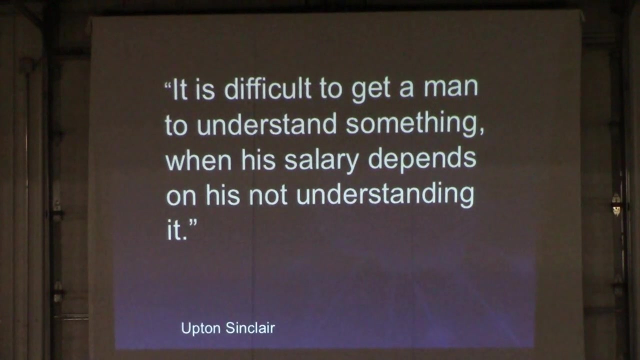 issue is this, and i'm telling you, my wife tells me all the time: husband, you're 99 of your problem. she's right. so the biggest thing we realize you're the problem. it's the way we look at things. let me show you some more. here's another thing why the soil health revolution comes against great. 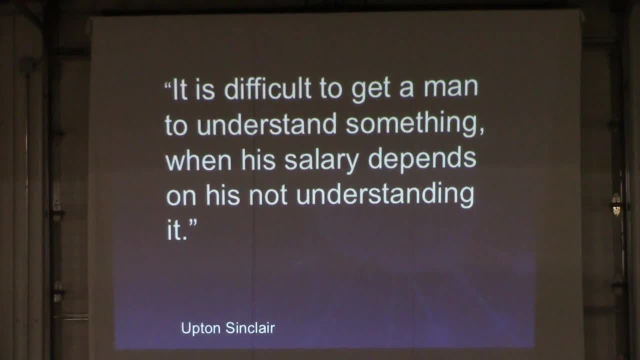 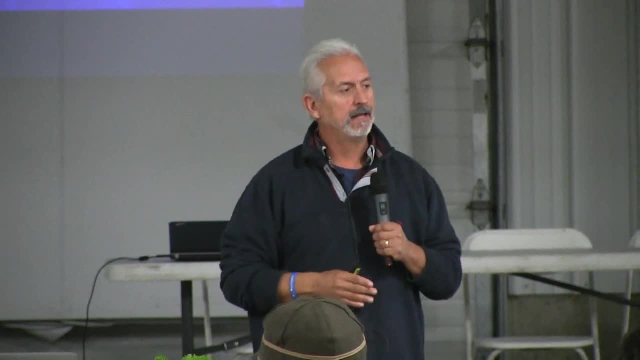 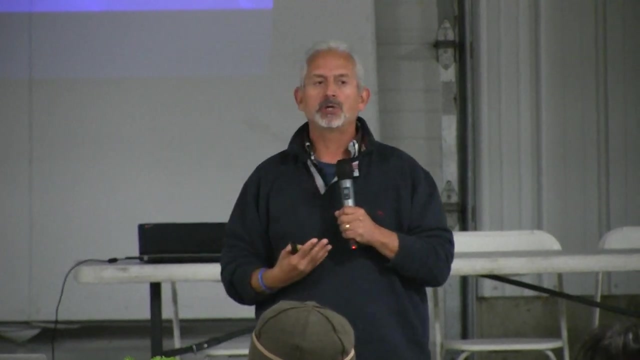 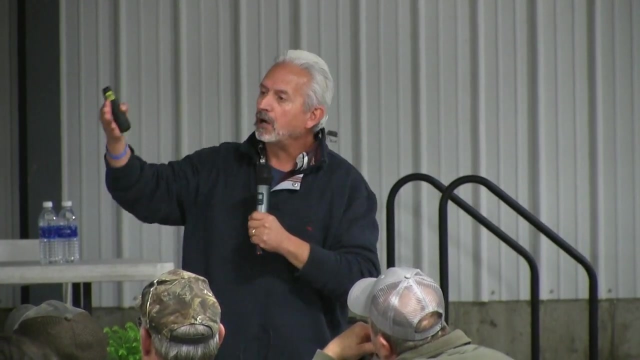 obstacles, whether in government or in anything. it is really tough to educate a man if the check depends upon it him not knowing. there is an incredible incestual relationship in government and big, large agriculture. nobody wants to hear that, but rarely is it for the resource and really the producer, rarely. 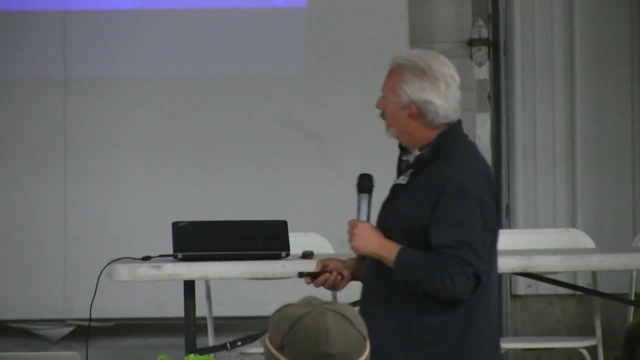 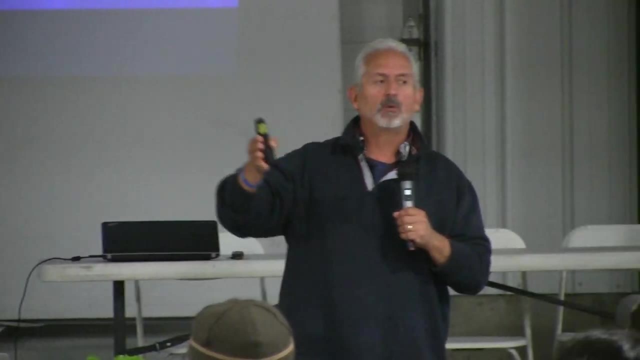 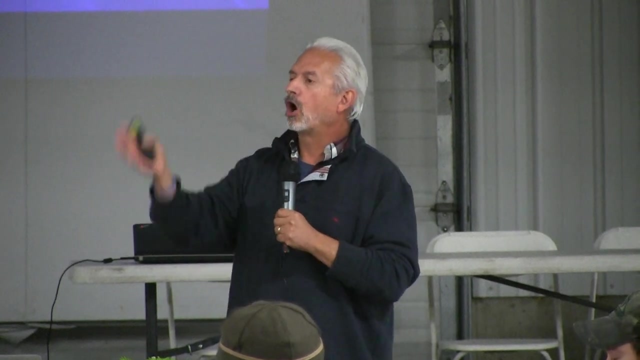 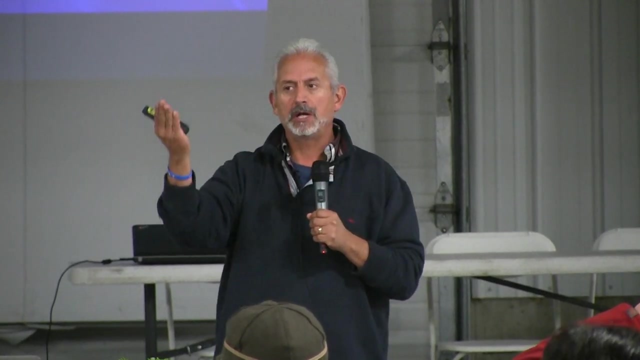 rarely. now let me show you another thing that's very critical: how our science was developed. ladies and gentlemen, i humbly submit to you our science, our agriculture. science was built on the wrong premise. premise means wrong foundation, asking the wrong questions. i had one of my. 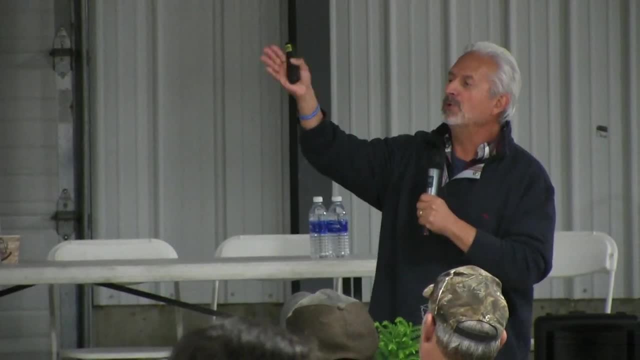 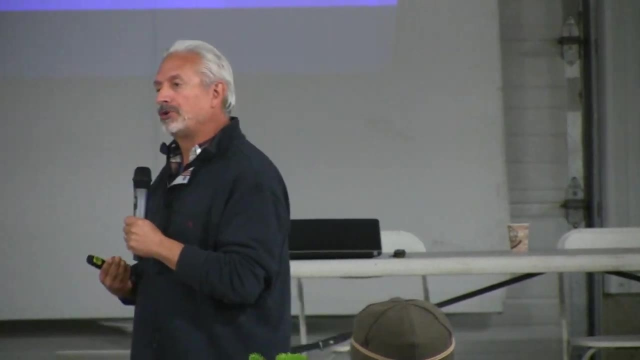 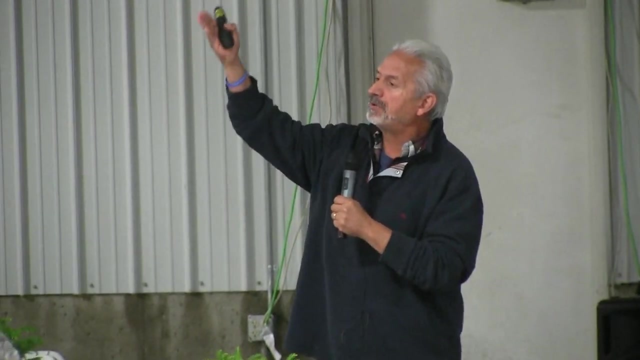 supervisors. tell me. he says: ray, why are you so opposed to science? i said, really, person is reached like a nerd all the time reading soil, ecology books and notebooks all the time, and i'm opposed to science. i said i'm opposed to science that is built on the wrong. 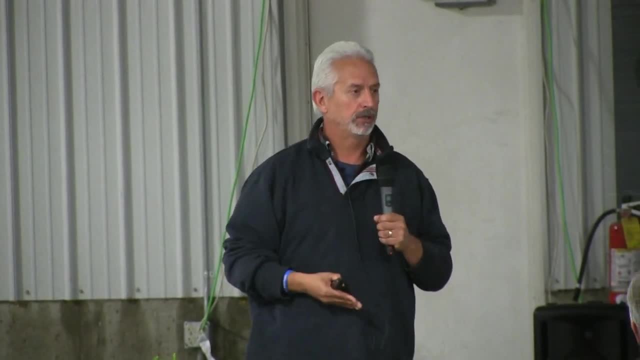 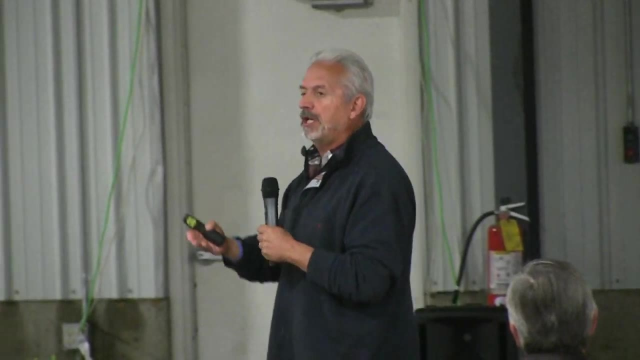 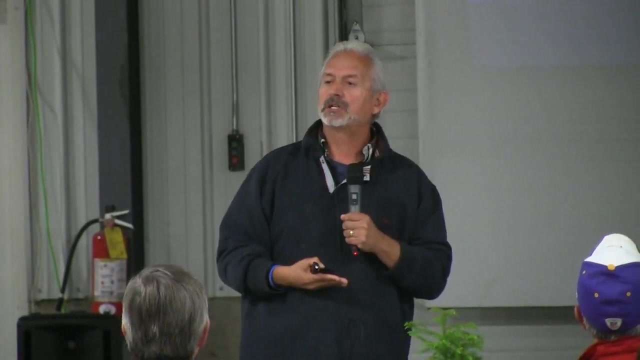 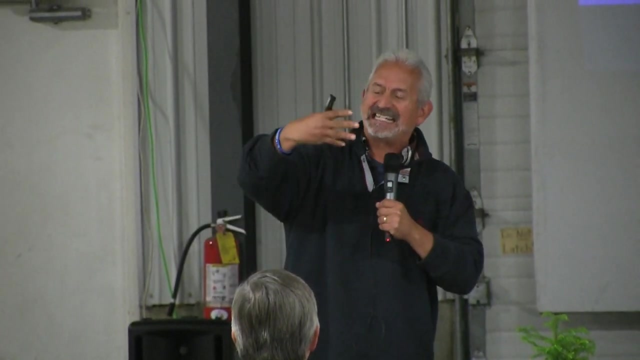 premise: asking wrong questions. this is the current science model. how can we increase the yield? by forcing it genetically, manipulating it, spraying it, controlling it? my first رمضان, The new science is: how do you love it, nurture it, understand it, collaborate with it, understand its synchronies? 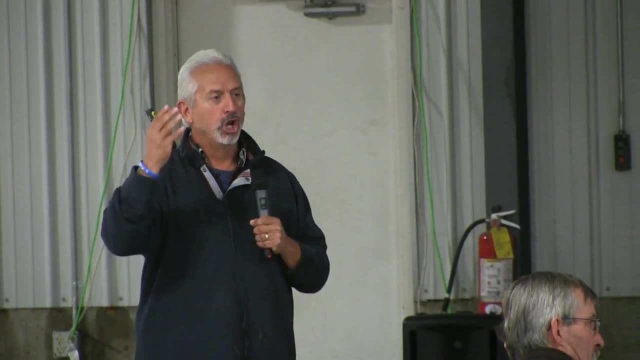 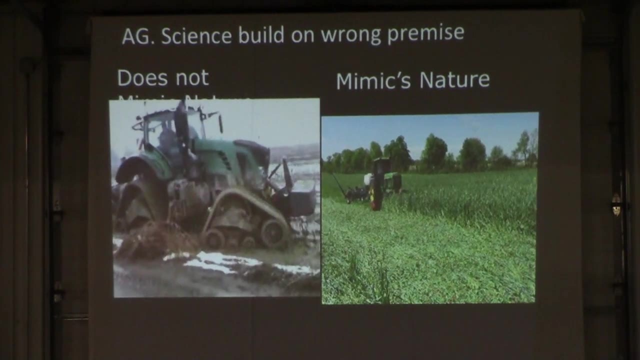 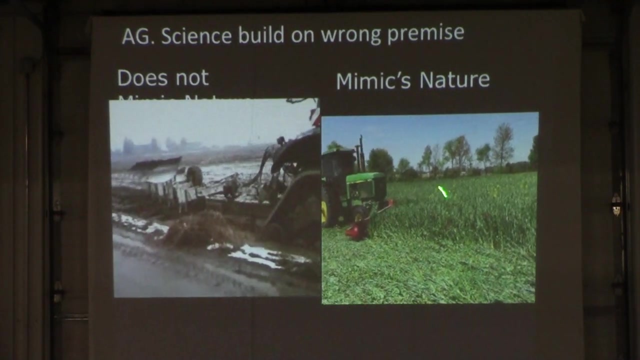 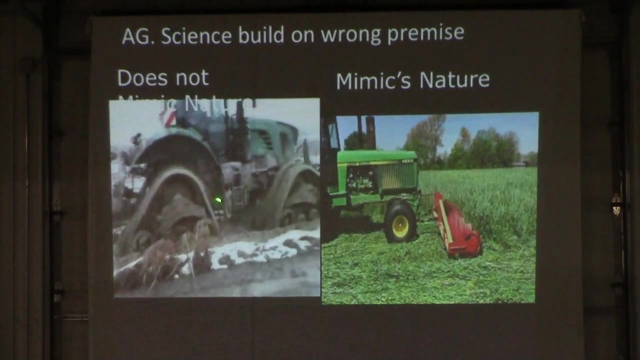 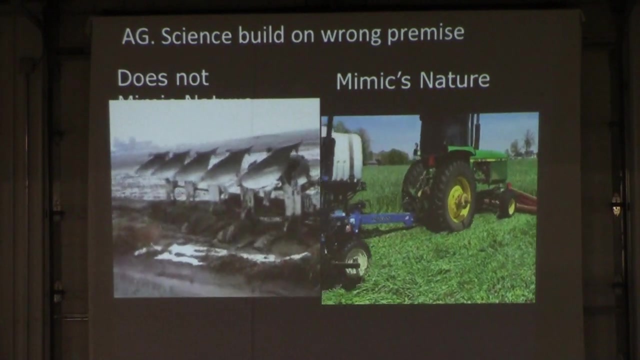 Total different question. Let me show you the two sciences. This is the current science model: Force it, Control it. This is the new science model: Emulate it, Nurture it. We are moving from here to here. Somebody told me: well, Ray, that's pretty extreme. 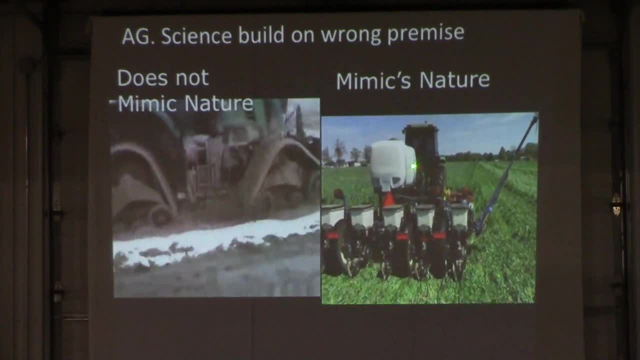 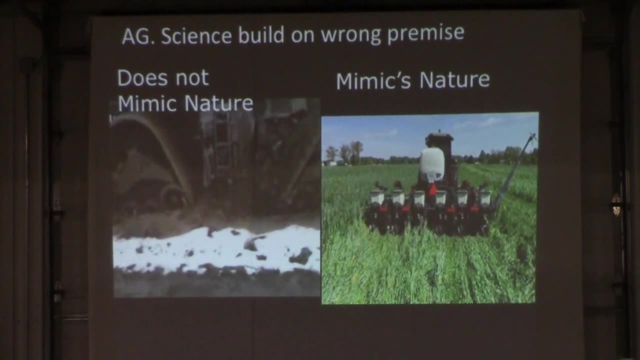 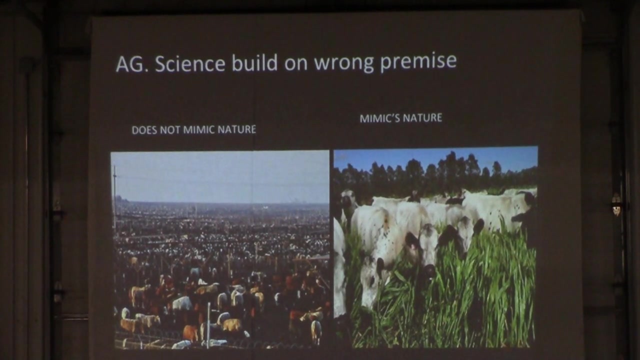 Well, if you lived in the neighborhood where everybody was black- and you did that, you would consider him to be extreme, wouldn't you? Does not mimic natural systems. Mimic natural systems, Gathered like buffalo. We are running cattle like buffalo. 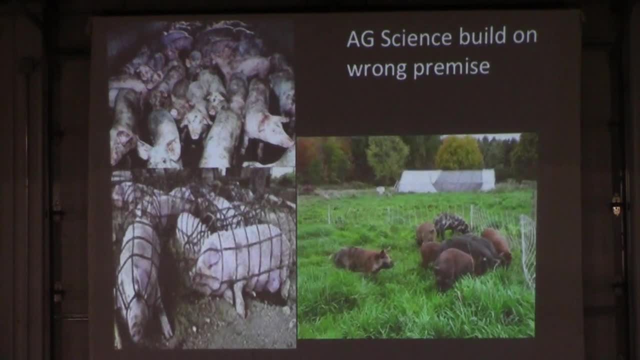 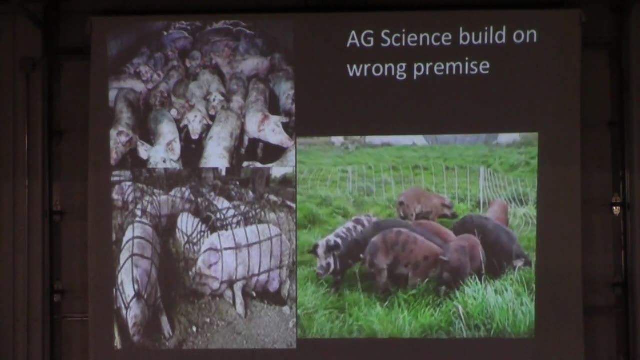 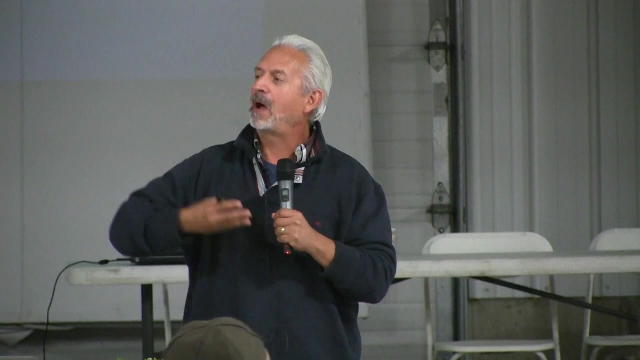 Does not mimic, Mimic, Mimic. We are moving in this direction because now we finally understand if we mimic the natural system, we can make money. We are not forcing it, We are not working against it. It takes a lot of energy to work against it. 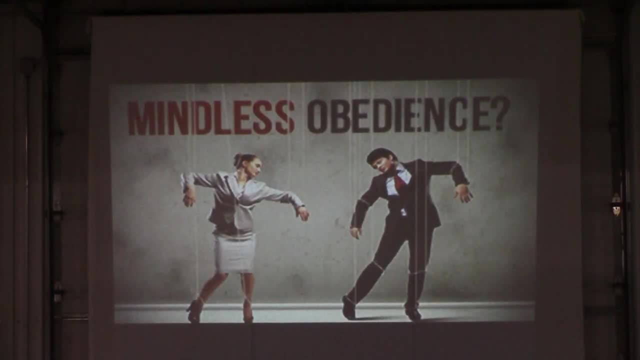 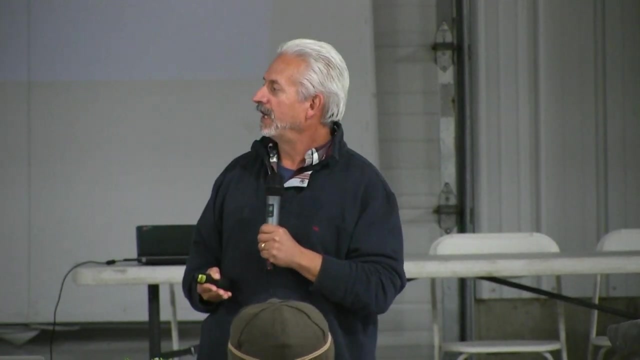 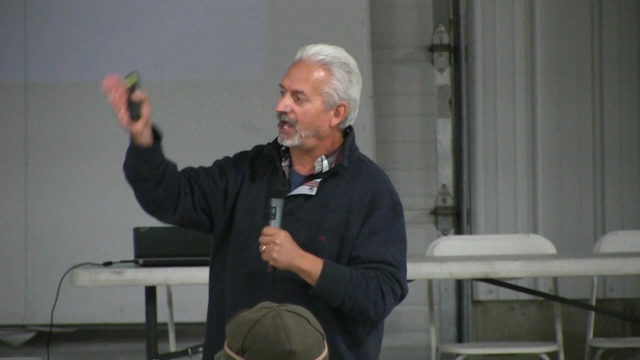 Ladies and gentlemen, I realize I was a product of mindless obedience. I had obedience to the current science model, to the industrial model. It was mindless. I never asked critical questions. am i working with the natural system which is designed and been beautiful and it's and it works? 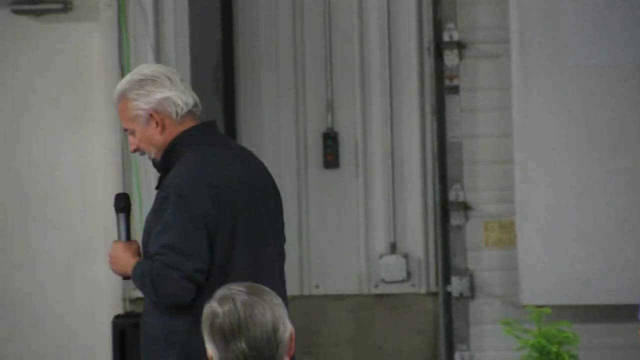 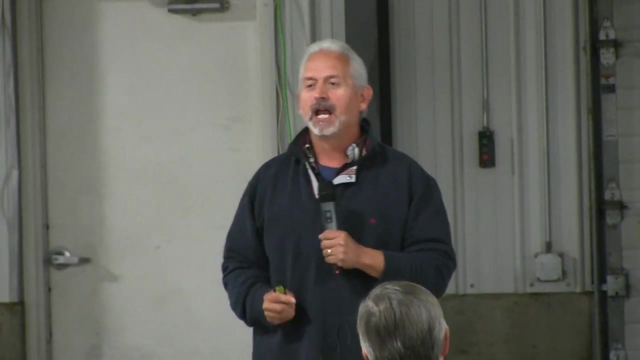 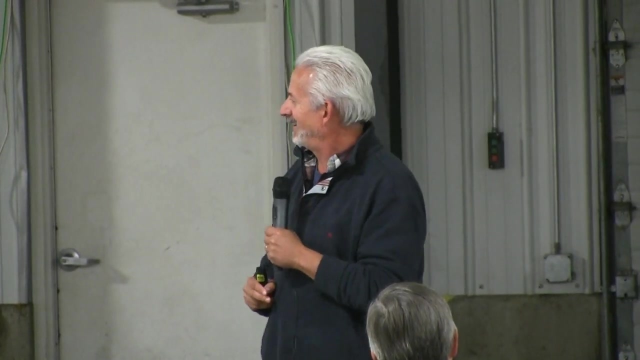 and has been here for many years. see, here's the thing, ladies and gentlemen. i had nobody after eight years of university study. if i'd had one professor that said: ray, now look at me, you're, you're not a very bright boy, your job is to emulate it. it would have just taken one semester. 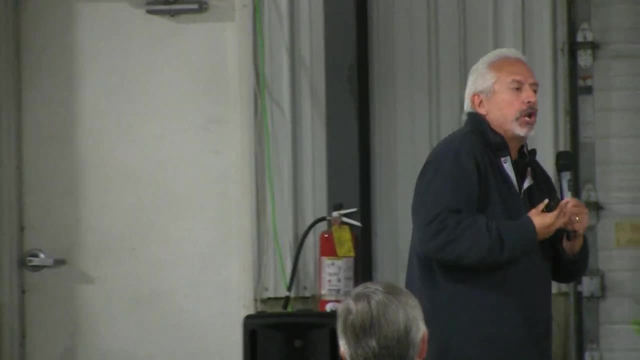 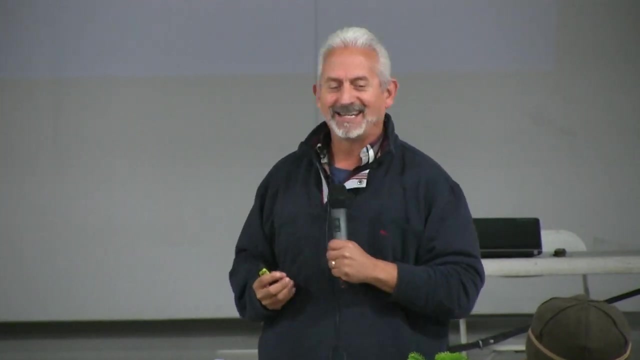 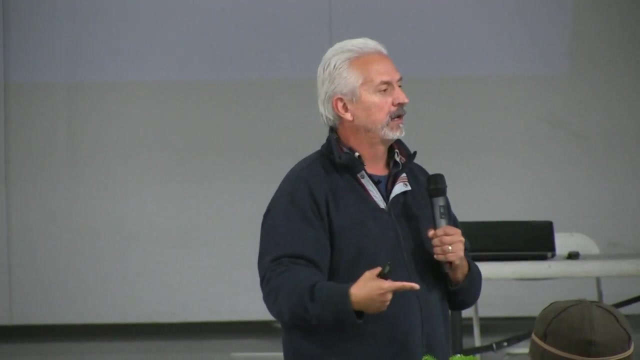 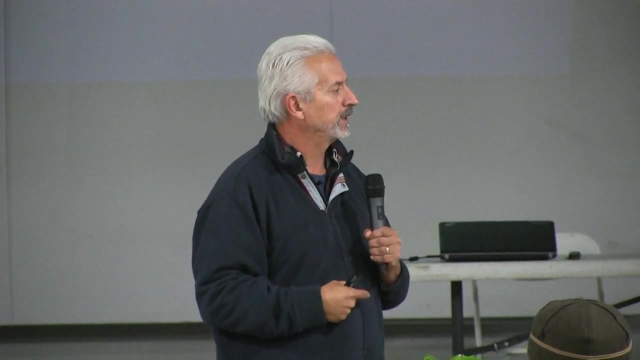 of somebody teaching me agroecology. putting it all together in context. say: your job, ray. emulate it, don't force it. understand it. it would have changed my whole career. i have had to spend 20 years of failure giving bad advice and now i've had to make up for the last 12 years. 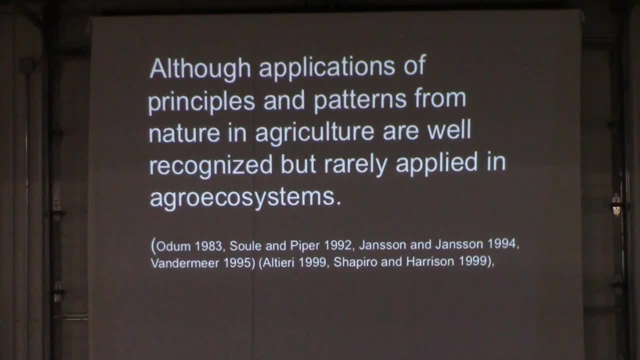 i've had people say: but ray, you're not a very bright boy, you're not a very bright boy, you're not a very bright boy. Where's your documentation of science? I said really, Although applications and principles and patterns of agriculture, of nature and agriculture are well known. 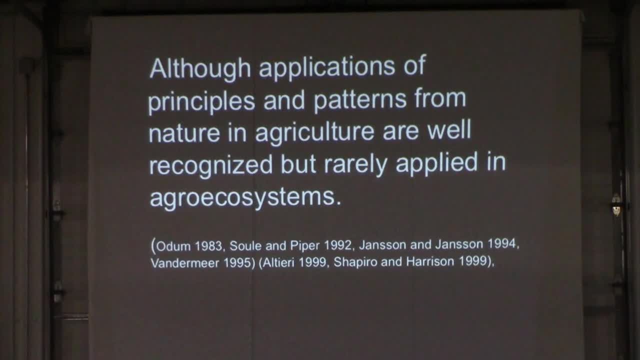 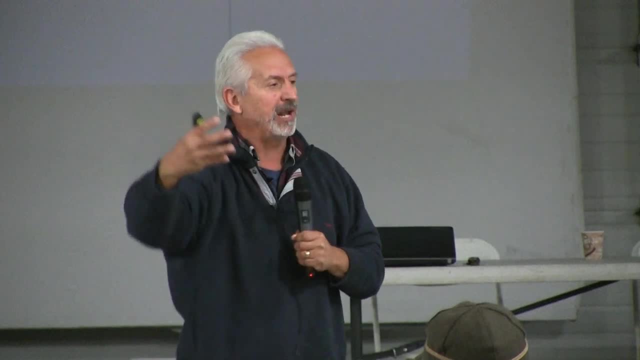 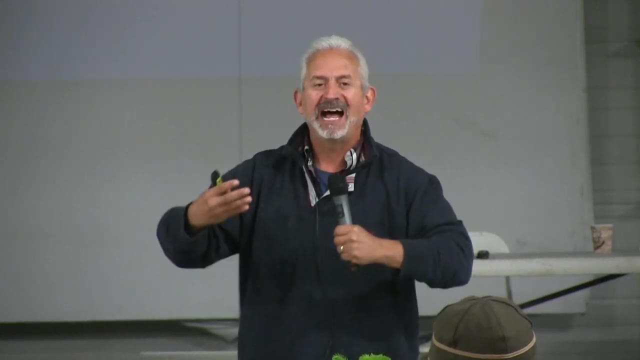 See, I didn't know, See, because I don't know what it is, But it's when I looked at my little farm. I looked at the farm and I looked at nature separately. No, It works the same way, Because it was hewn out of the natural system. 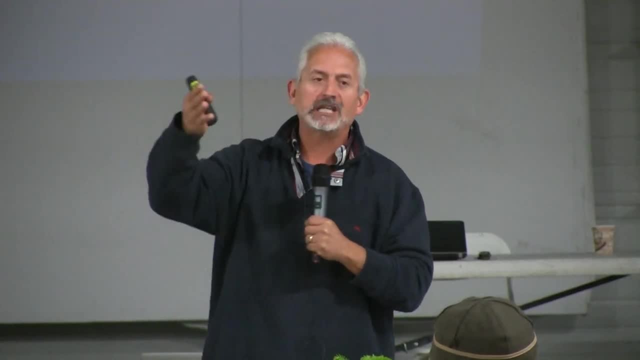 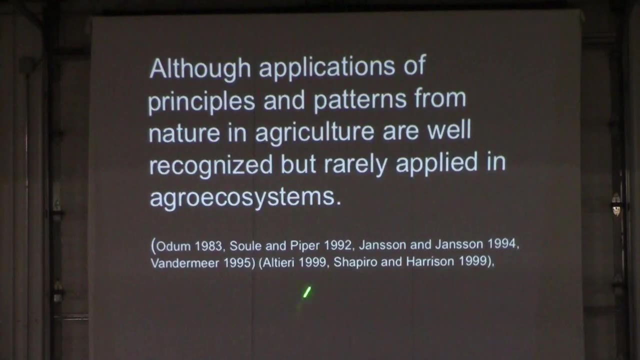 It came out of a forest, It came out of a prairie. It works the same way. I didn't know that, But look at the brilliant scientists. They knew a long, long time ago, But it's rarely applied. It's after years and years of failure. 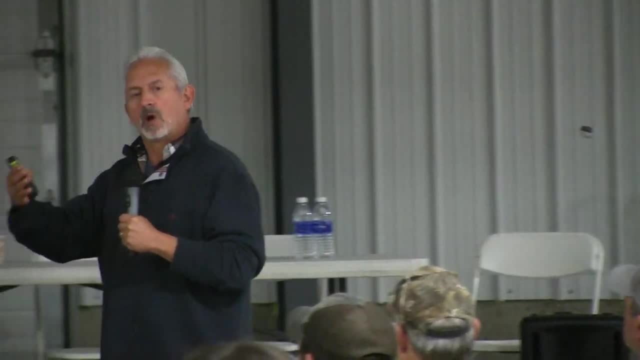 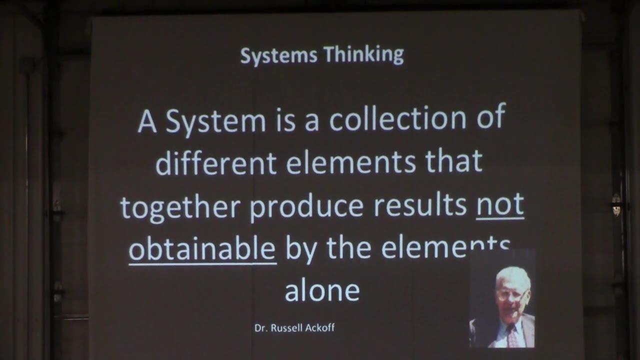 And people are getting sick And they're realizing what's wrong with the current model And they're trying to figure out what's wrong with the current model. Write this down Whoever wants to learn more On YouTube: Dr Russell Akoff. 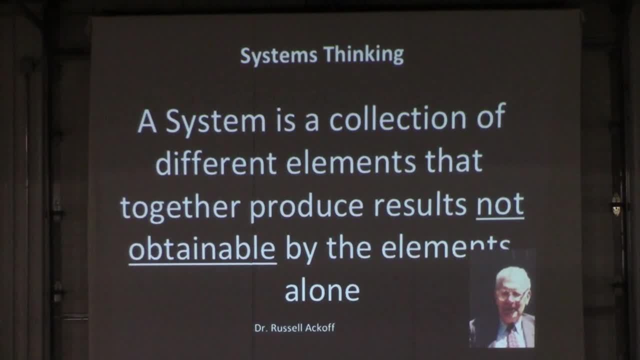 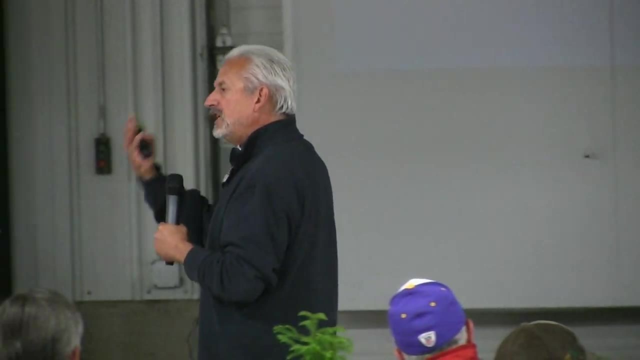 Brilliant, one hour and 30 minute talk on YouTube To teach you how to do systems thinking. See, I wasn't taught to thinking systems. You are an elegant system. This man passed away, but he was brilliant. He's teaching me how to deal with a system. 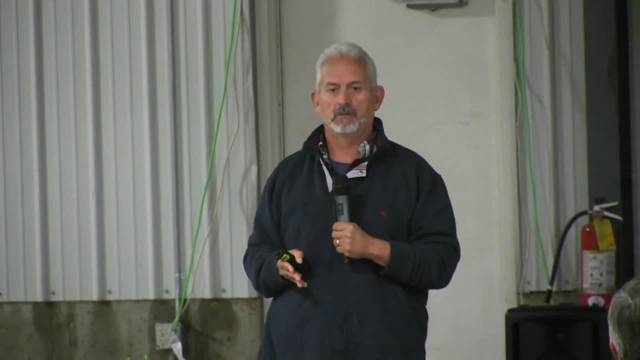 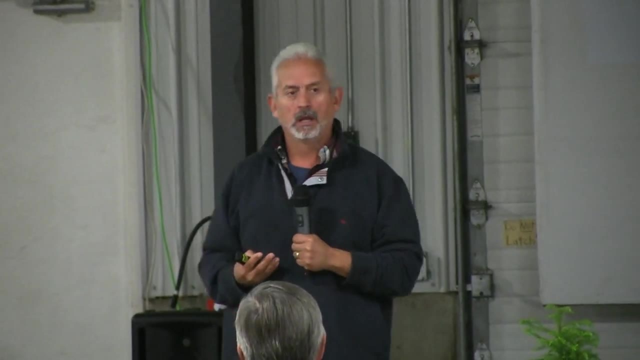 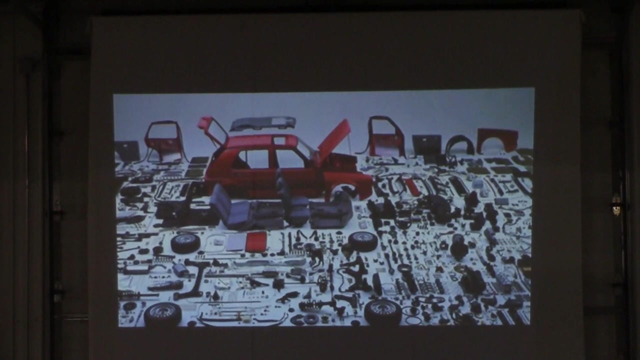 You are dealing with a system. You are dealing with an incredible ecosystem. You are a system. You are seven trillion cells walking together as a collective whole, And a majority of your cells aren't even you. They're bacteria. Let me give an example. 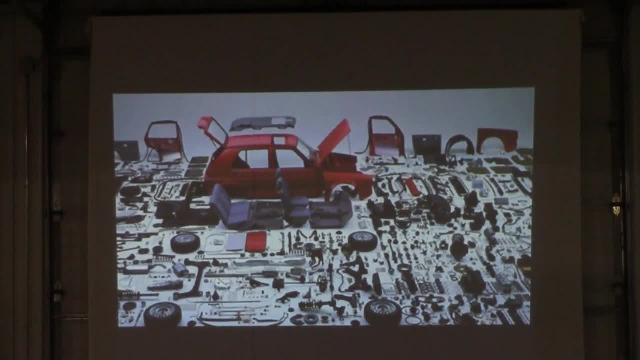 Ladies and gentlemen, what is that a picture of? Is that a picture of a car or parts of a car? How many say it's parts of a car? How many say it's parts of a car? How many say it's a car? 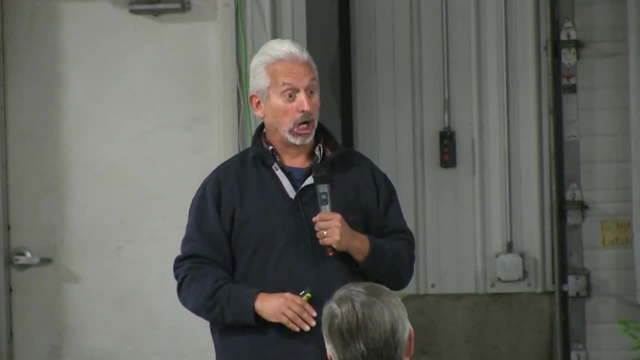 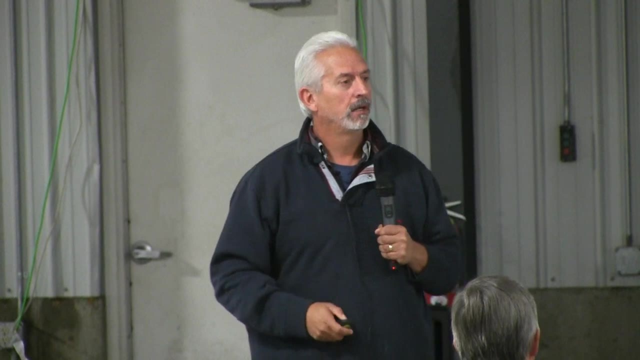 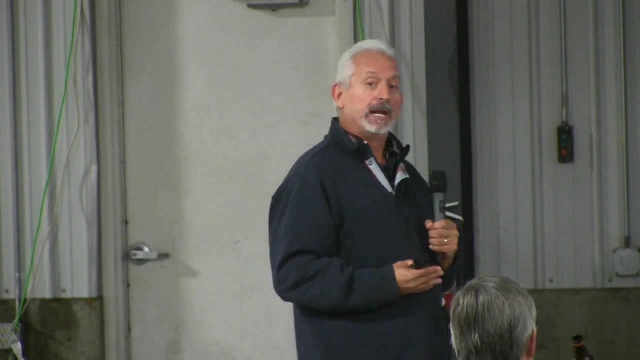 It's a junkyard. It's a junkyard If I jumped on that tire and say get me to Albert Lee Seed, would it get me there? No, it wouldn't. If I jumped on the engine, Tom, would it get me there? 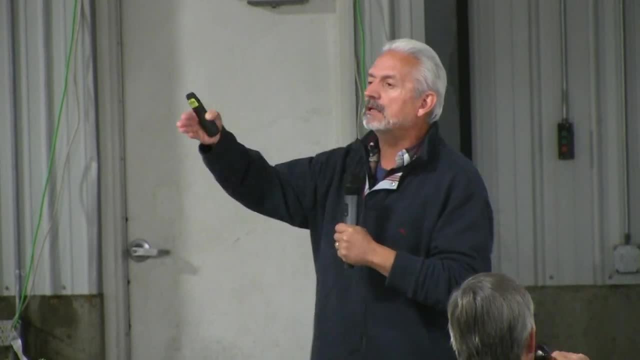 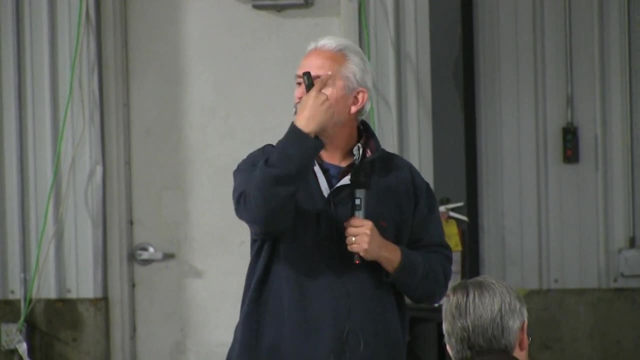 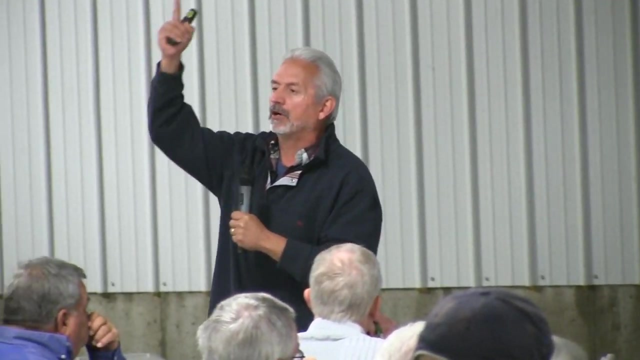 No, It's the pieces collectively working together as a whole make up a car. This is what you want. This is what you call reductionist science. Reductionist science is: you study the little pieces, but you forget they're connected to the whole. 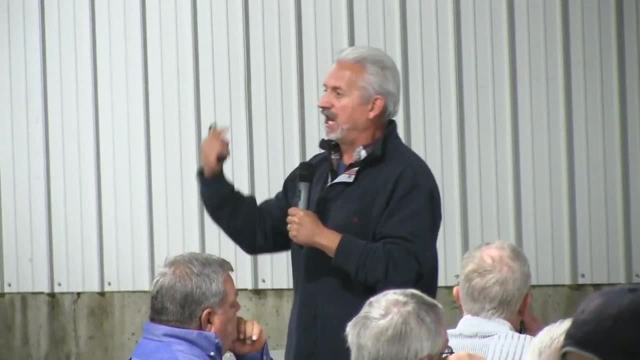 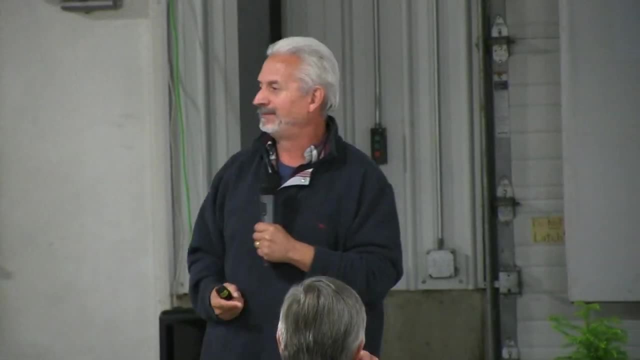 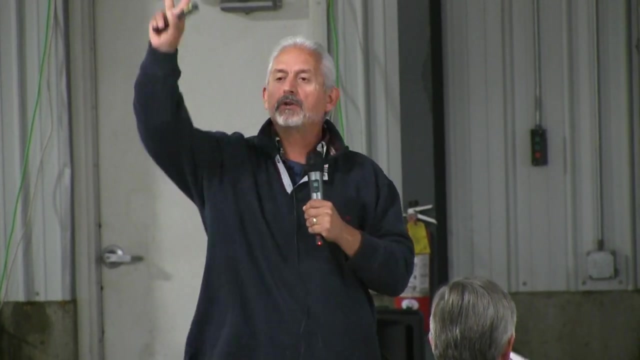 See, reductionist science is mesmerizing. It is powerful. We couldn't have an iPhone, We couldn't get to the moon, We couldn't build a car without it. But here's the problem: It does not work well in dynamic living ecosystems. 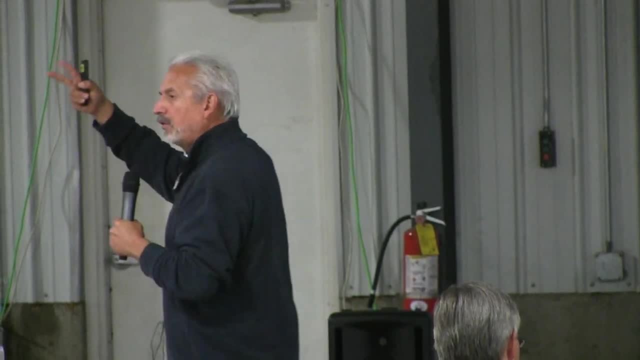 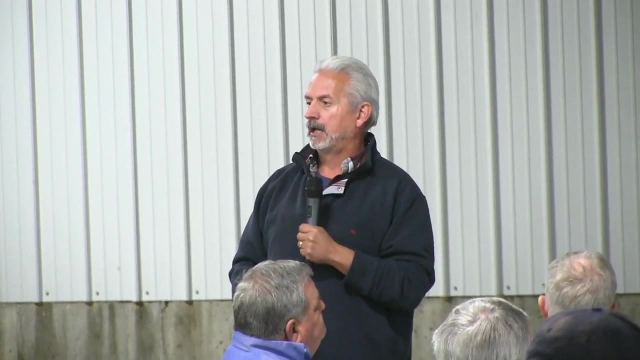 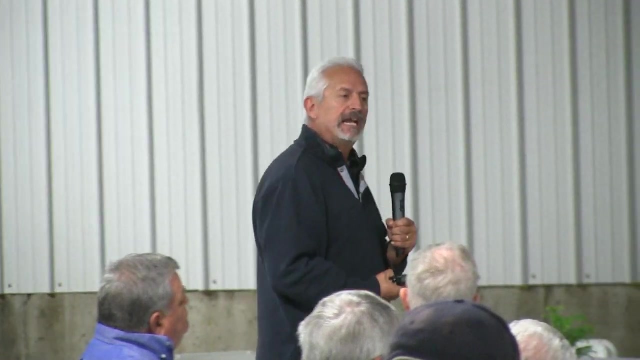 What are the two most sickest things happening in our country? Our medical field and our agriculture. Two parallel worlds trying to make the human body like a machine. Same thing with natural systems. It does not work well, That is Newtonian physics. 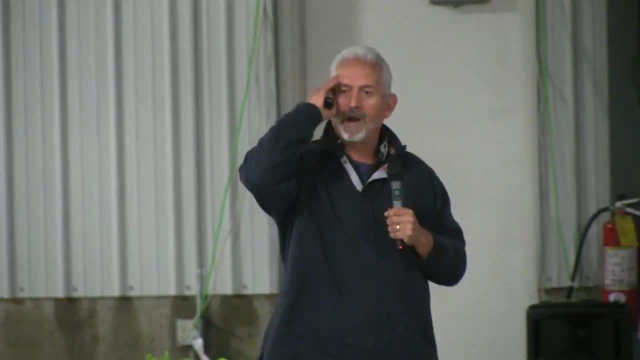 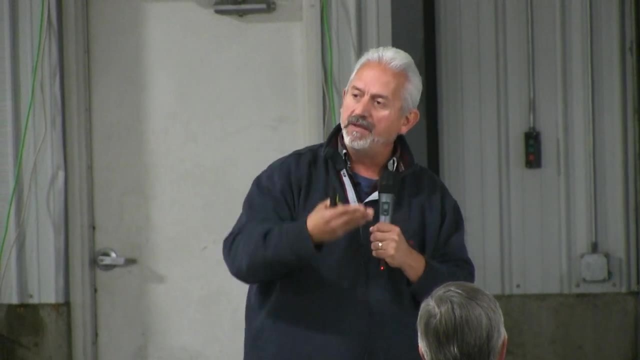 It's not a machine. Aristotle came up with this Western thought process. It's a machine. It is not a machine, It is dynamic living, just like you are. Then, if it is, then we have to deal with the fact of. 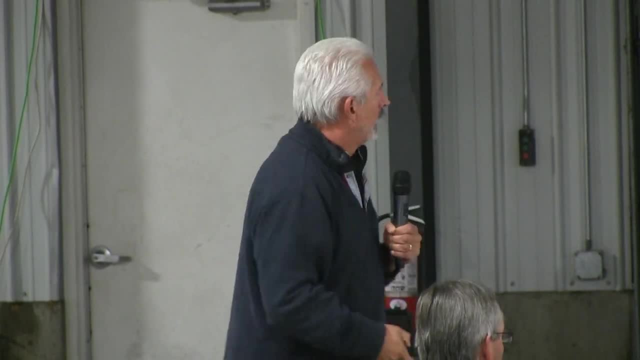 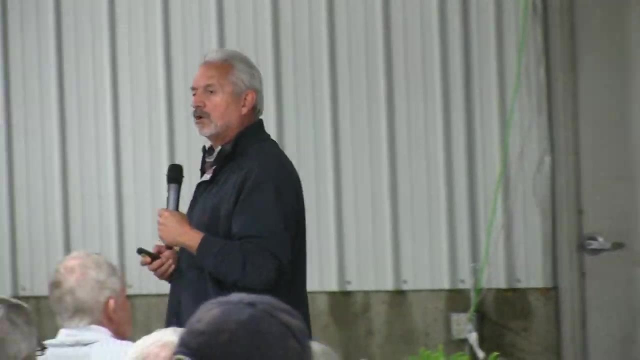 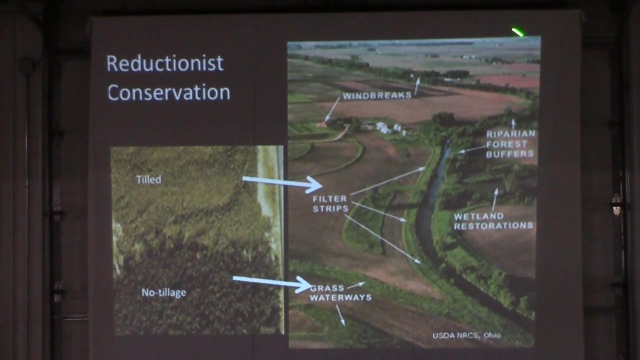 Relationship. Let me give you an example. after 32 years of my career going all over the country trying to promote conservation, This is a product of reductionist science. Please notice this whole landscape. When you walked into NRCS office, it was like a cafeteria. 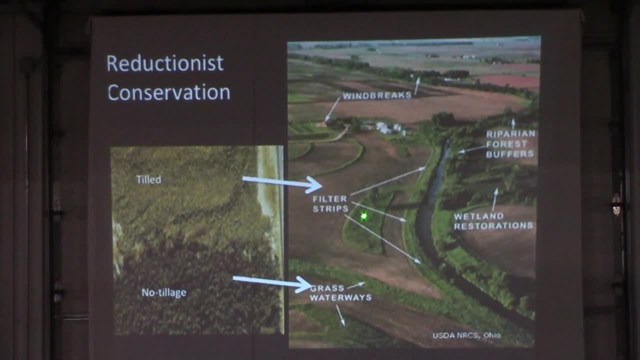 I would say: what do you want, Mr Producer? Do you want a little nice buffer strip, a little filter? What do you want? Do you want a nice windbreak, just like a cafeteria, putting out pieces like a blind person? 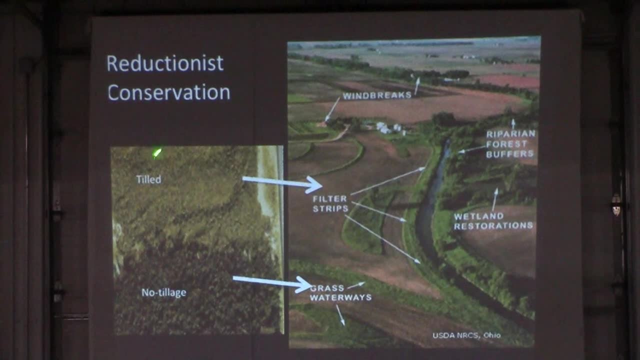 The sad thing about it, the only functioning soil in that whole picture is the filter strips, the riparian corridor where you have living covers and plants 24-7.. In the other part of the landscape, where it's tilled, there is no aggregate stability. 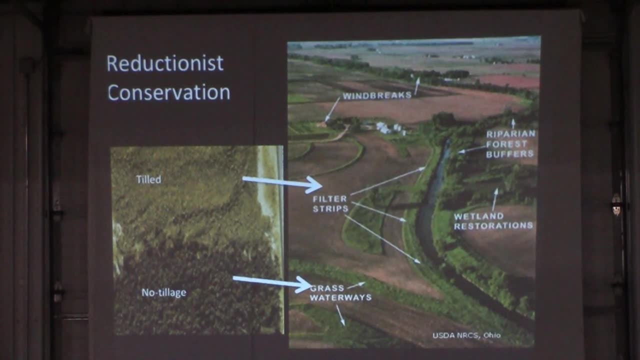 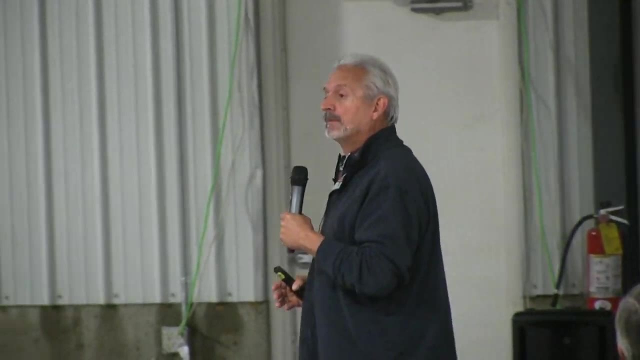 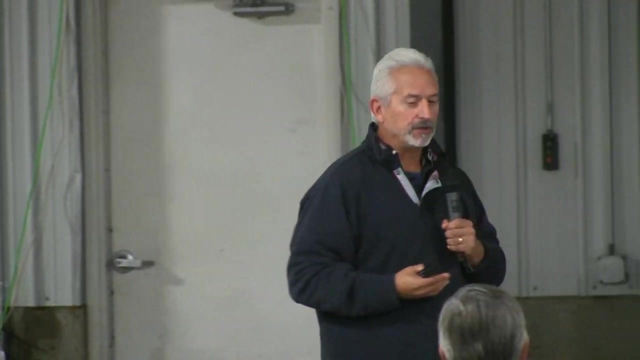 The water is running off, The only functioning soil in that whole landscape. Now, am I opposed to windbreaks and all those? No, We need them. In fact, they give us, gives nature space. Now, I love to do this. 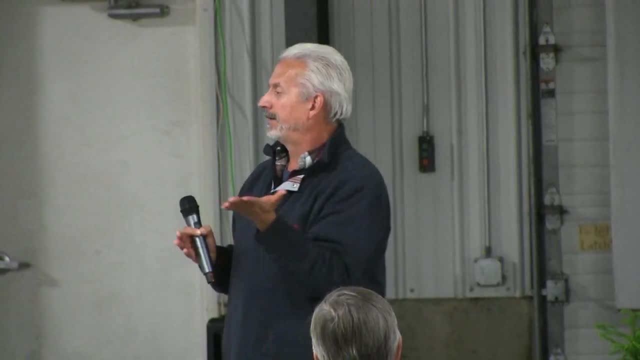 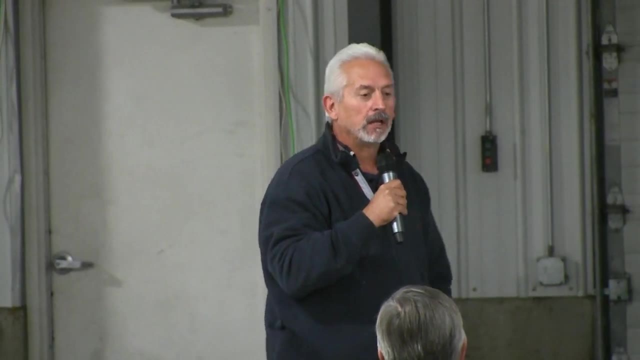 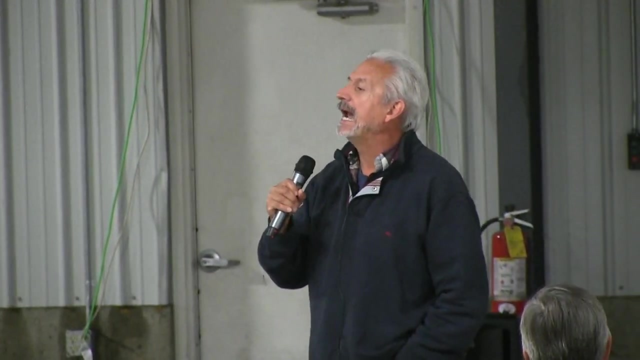 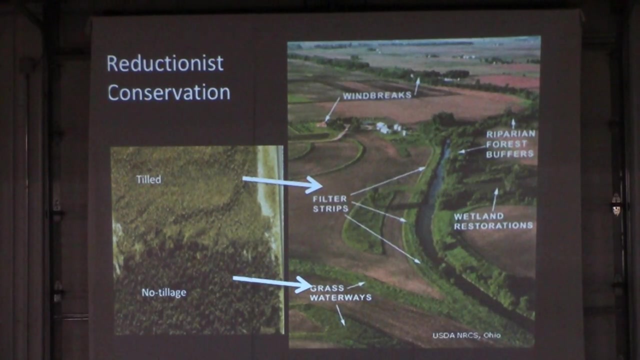 If I get an insect, put it on my hand right here and I smash it audience. what does it die of? Lack of space? Nature's the same thing. it needs space. We need these, But we want to change that. every part of that soil is covered 24-7. 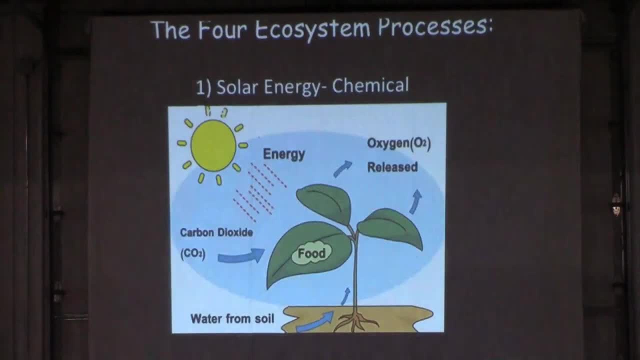 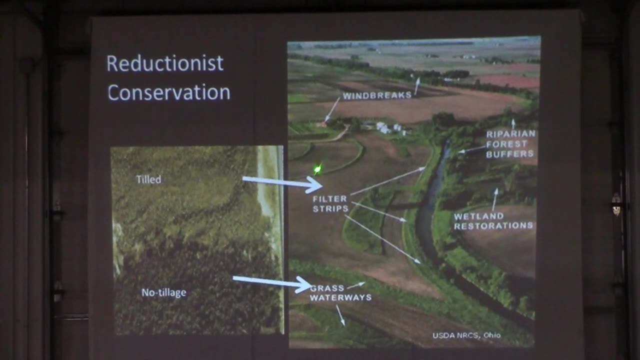 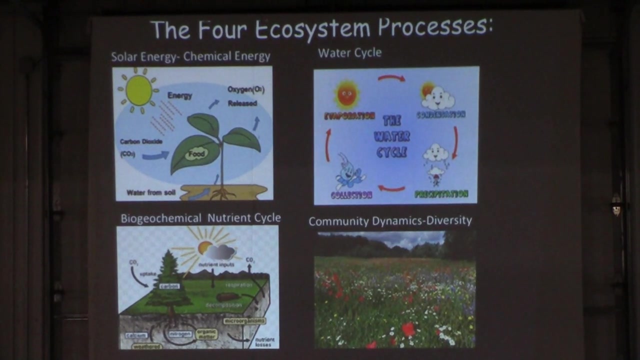 That field right here is not capturing energy. Let's go back here. That field is not capturing sun. It's spilling sun and leaking nutrients. Let's continue. Four things you have to really understand when you walk on your farm, Whether it's a pasture system, rangeland system, all of it. 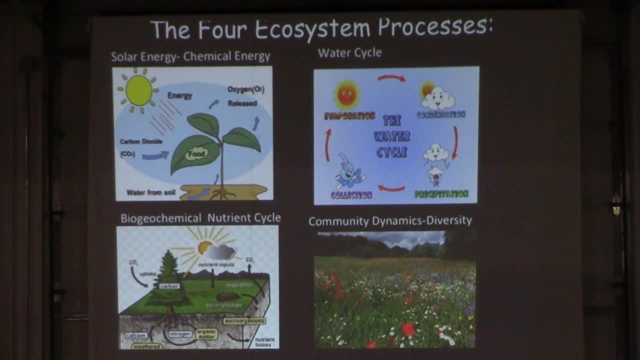 This has kind of bypassed me and I don't know why I wasn't taught this. Maybe I was just slow. I have called the four ecosystem processes of the soil Four ecosystems, In a simple way. this is how the house works. 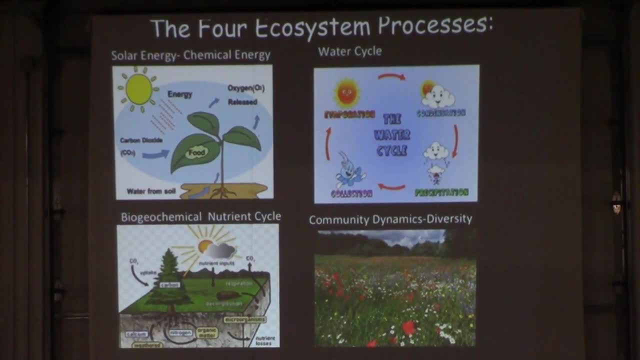 This is how the planet works. These are four critical things. When I walk in the field, I better see these. First one: I got to capture sun. My job is to convert sun into liquid sun. Second job is I got to make sure the water cycle is working. 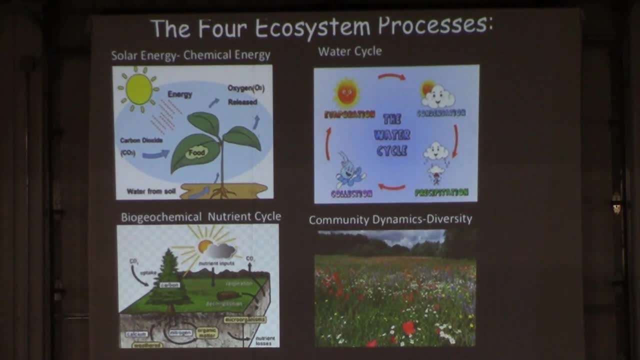 Water cycle is not complete until it goes into the soil, not runoff. I tell people we don't have a runoff problem in this country, We have an infiltration problem. We'll talk about that in a second. Then nutrient cycling. There's a reason why scientists call it the biogeochemical nutrient. 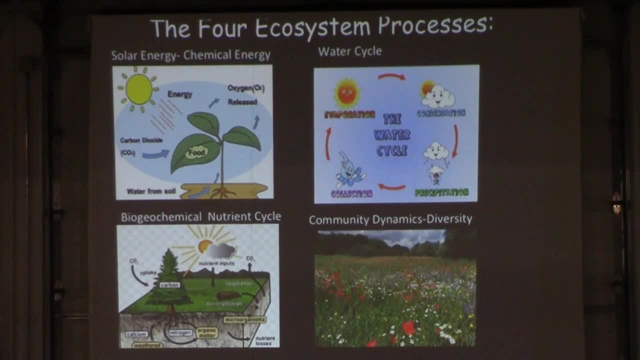 Biological first, Then it's geological and it's chemical, but it's biological first And then the last one: diversity. Diversity is the ability of the natural ecosystem to pass nutrients and mass to one organism to another organism. It is the conduit of life. 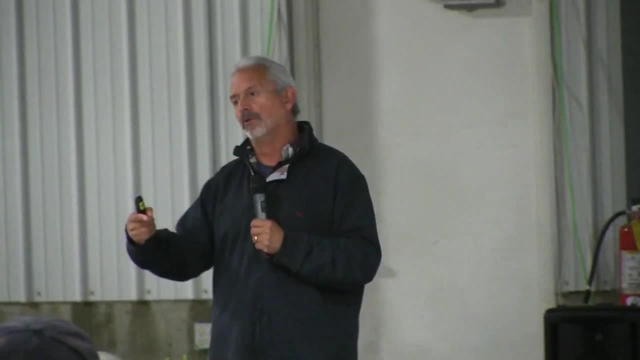 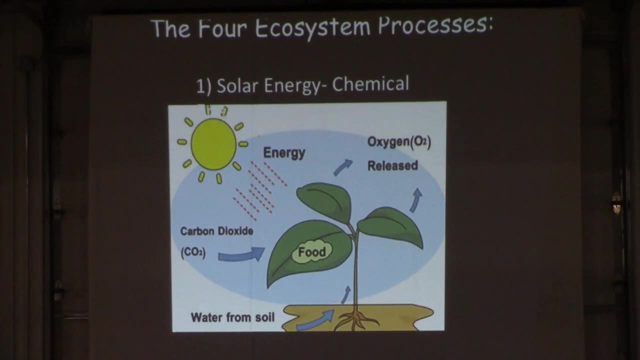 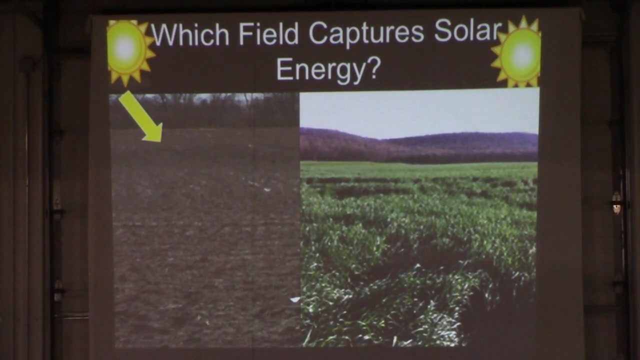 Diversity is. The more diverse you have rotations and animals, the more you flow energy into the system. First one, capture sun. So blasted critical. Which field is capturing sun, ladies and gentlemen? That's Illinois. Is this one feeding microbes? 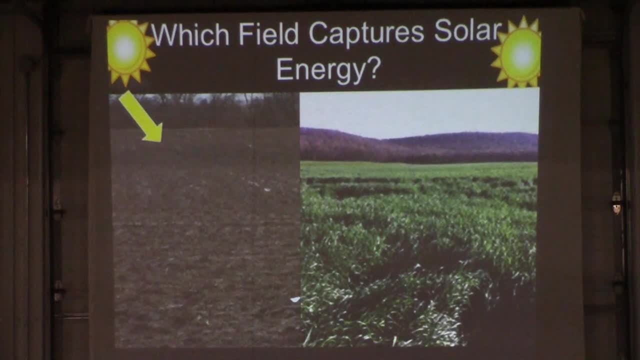 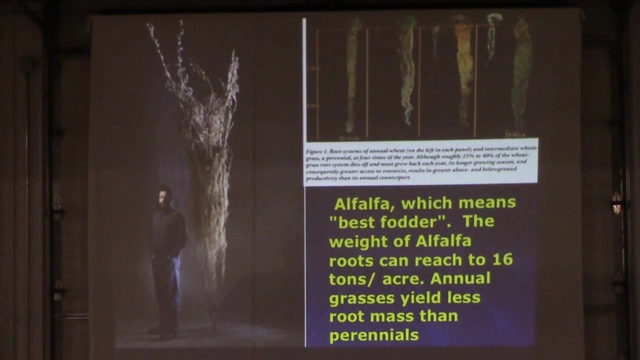 Is it feeding microbiology? Is it storing nutrients? Is it sequestering? Is it nurturing? This is costing money and costing us billions in health. It's not feeding microbes. This one is My job. living roots, that is the conduit of energy going into the system. 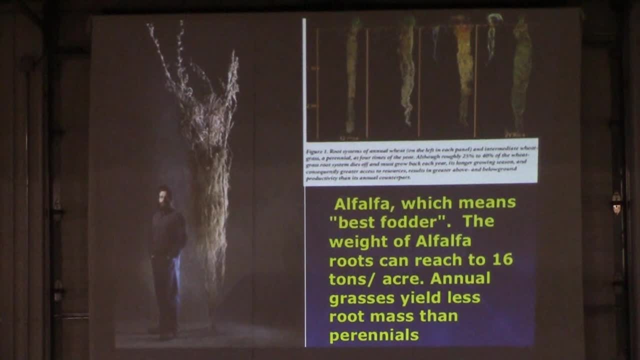 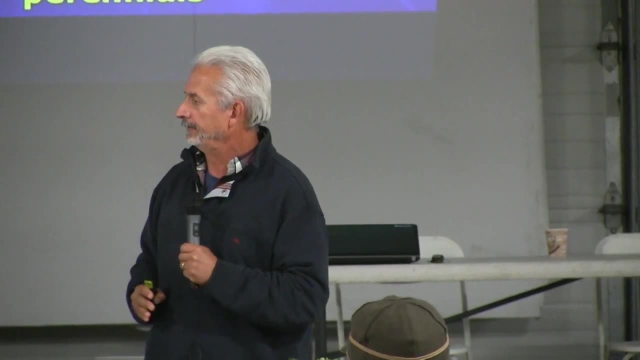 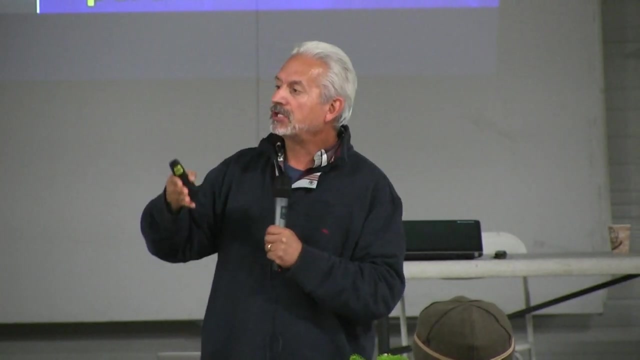 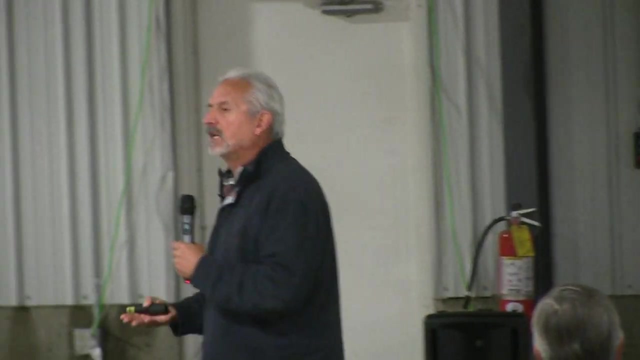 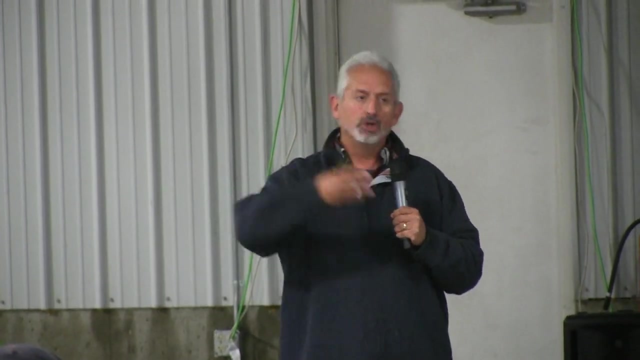 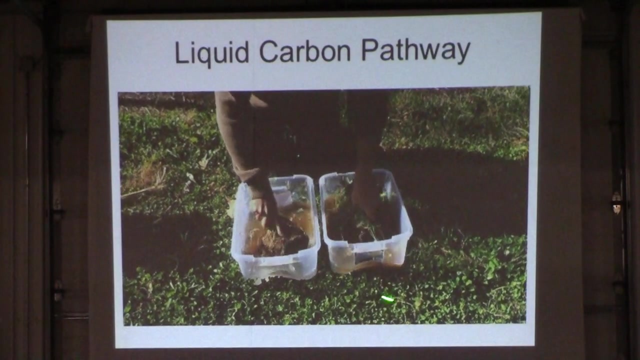 See, We can't. We need to be successful. We need to be successful in this. How, How, How, How, How. Without plants and microbes, you have geology. This is the liquid carbon pathway. There's a little simple test I do when I work on the field day with producers. 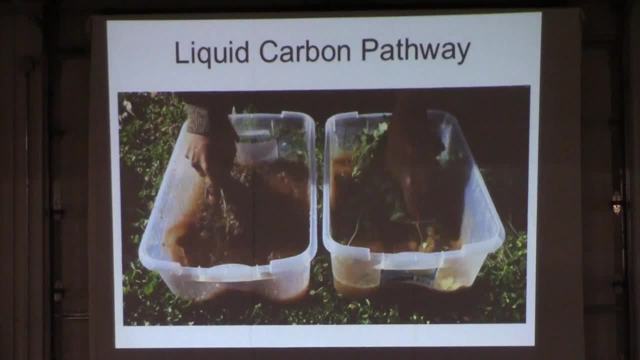 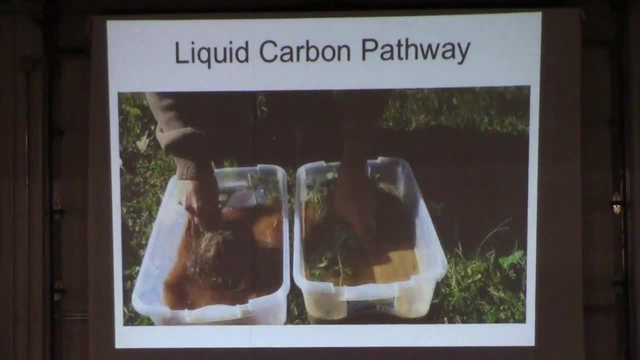 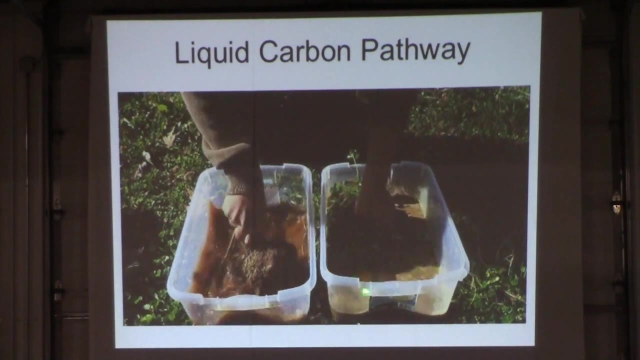 This is corn. This is a multi-specie mix. in my backyard It's called the scum test. I used a modification from Dr Christine Nichols, who is a soil microbiologist. Look at this white frothy material, Yo. there's about 200 carbonaceous molecules produced from the plant. 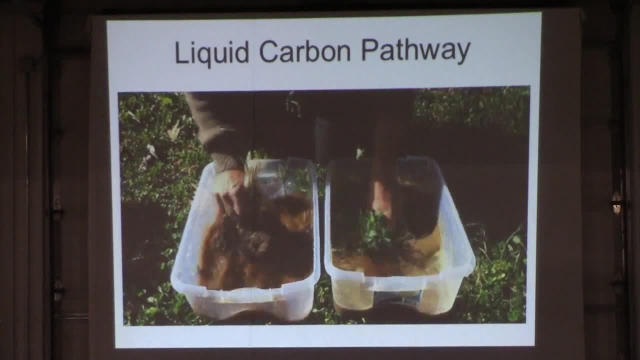 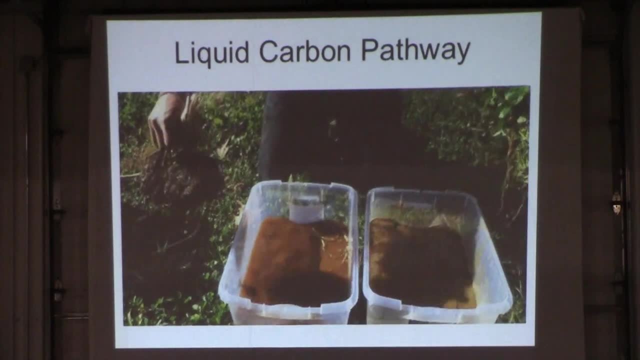 converting it and changing the mononucleosides, sugars, carbohydrates, all these allelopathic chemicals. It's the way plants communicate and it's the way it feeds biology. Look at the difference between these two. Look at that mix. 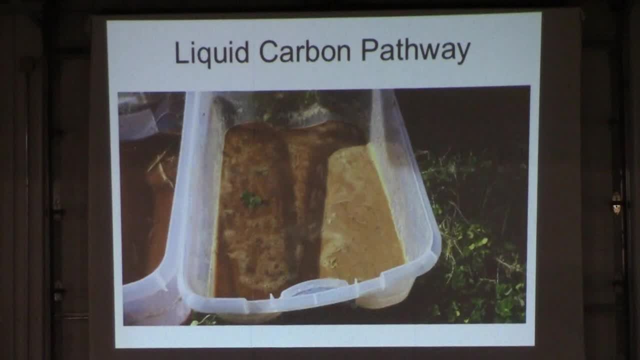 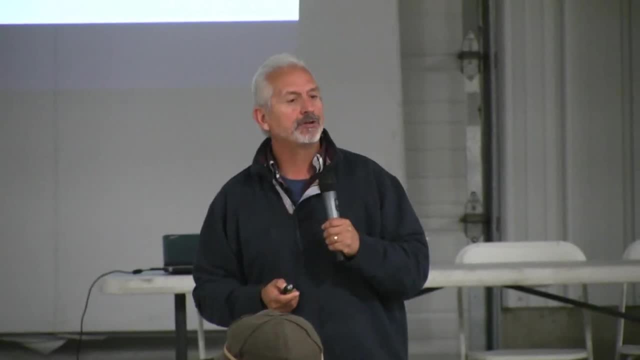 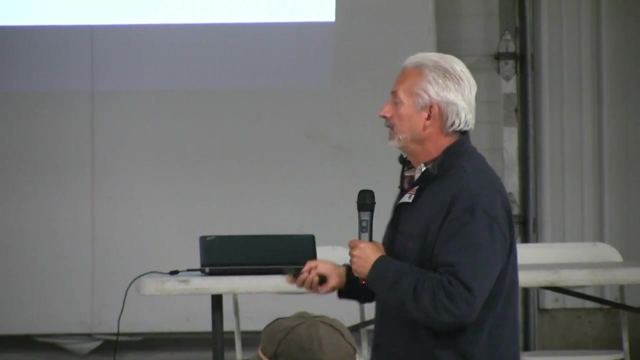 Then I went and took that white frothy material, sent it to the lab. It had 170.. It had 17 parts of carbon and 18 parts per million nitrogen leaking. That was done in the winter, leaking those carbonaceous compounds. 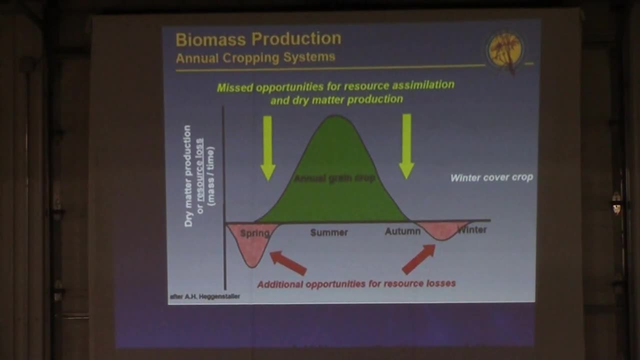 My job and see this graph. somebody told me you know, if you really look at the graph, it's really. it should be a lot more truncated because we are not capturing energy. So right now, nationally, globally, we're not capturing sun energy here. 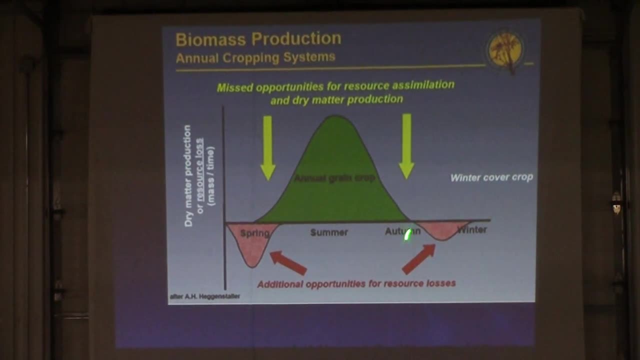 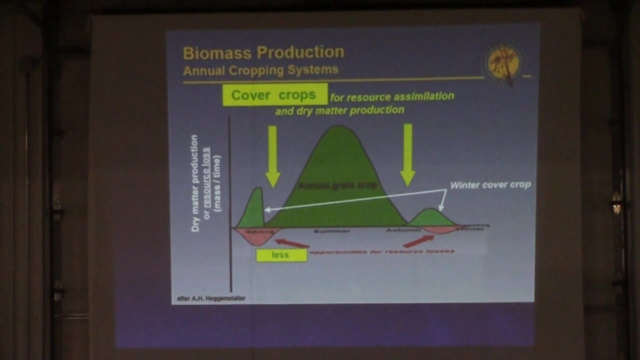 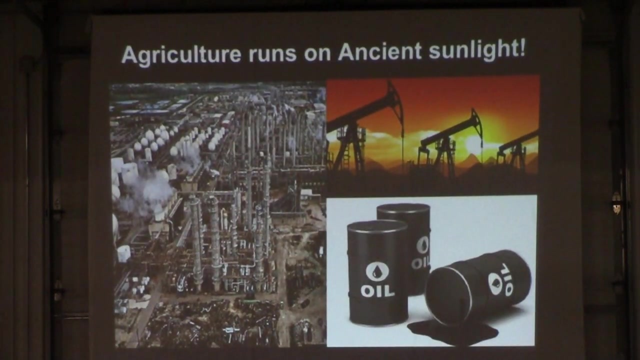 We're not capturing sun energy here. We're not capturing sun here. We're leaking nutrients here, We're leaking nutrients here. Our job is to cover those gaps. Feed biology 24-7 as much as possible. One of the things I look at when I walk into an operation. 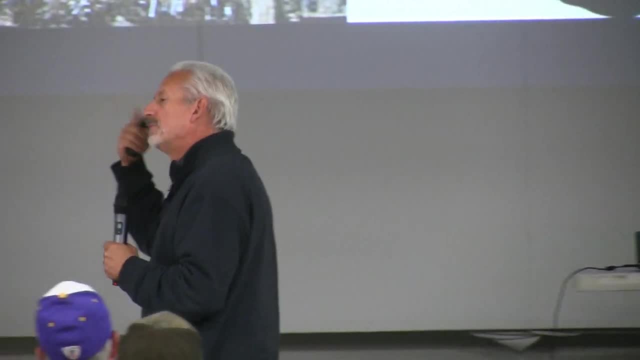 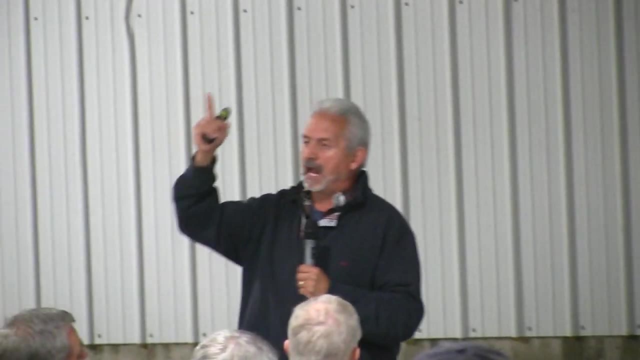 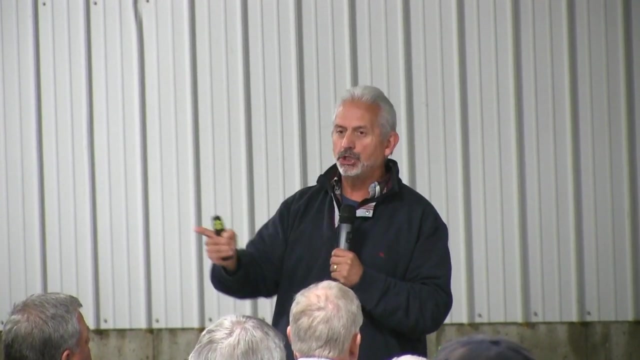 and I sit there and I come up with my shovel and I listen to the producer after I watch his soil dig into the soil. then my whole thing is here And I ask it's registering in my mind. is this farm and ranch running on ancient sunlight or new sunlight? 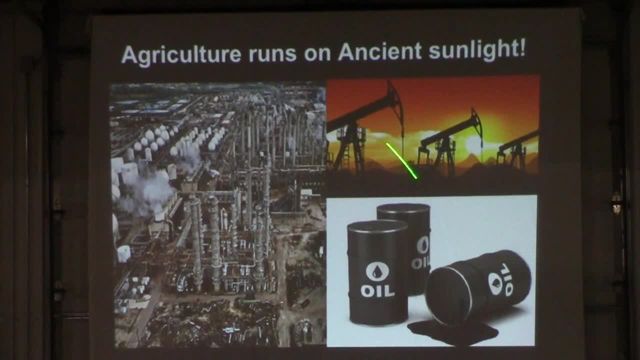 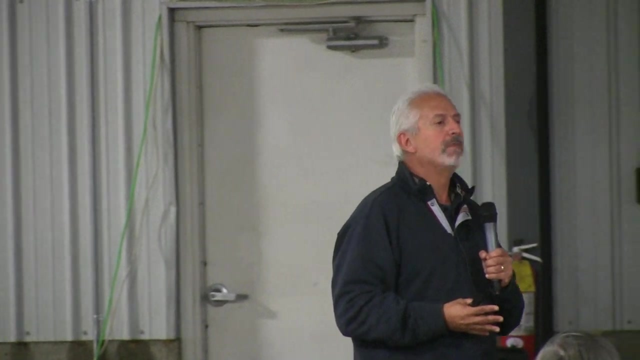 A majority of our farms are running on this. ladies and gentlemen, See, because we have convinced a lot of people, it's all about yield. The biggest impediment of change on your operation is yield. You don't make money on yield. You make money on how you can reduce your inputs. 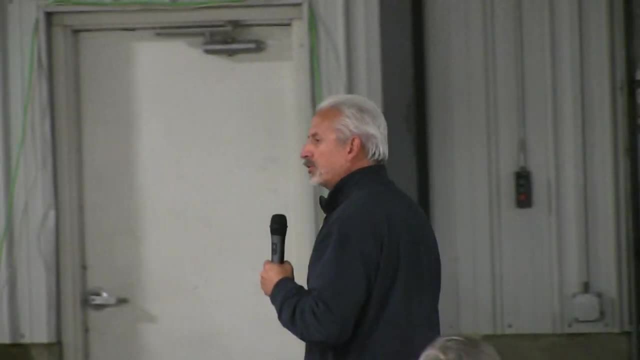 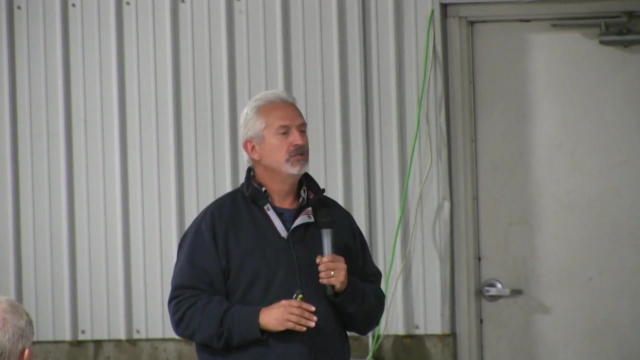 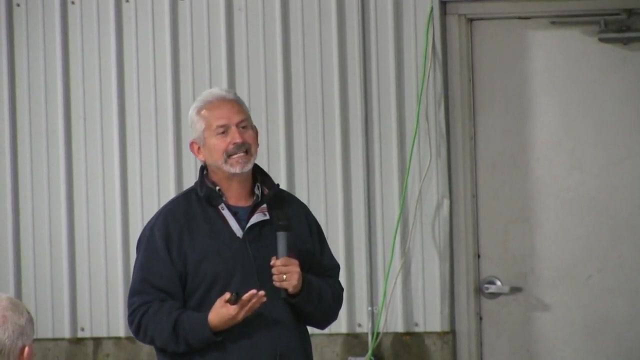 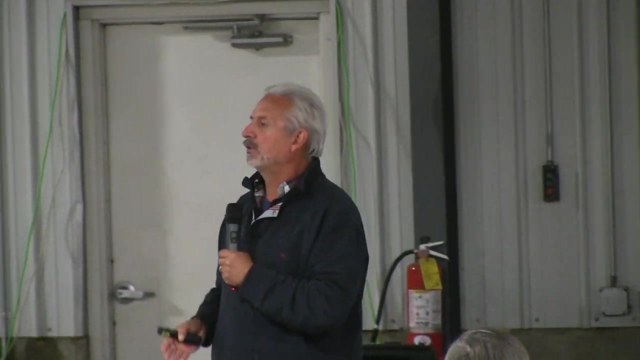 I had a farmer that produced 270 bushel corn in Arkansas and lost money. It's never been about yield, It's about synchrony, collaboration, understanding the system, reducing your inputs- Because you heard the couple of speakers. they said there's going to be a point where they keep growing too much corn. 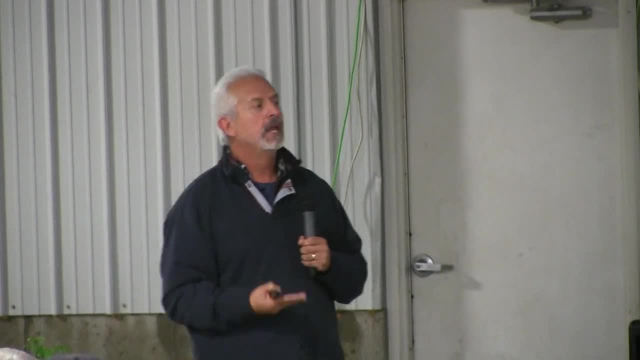 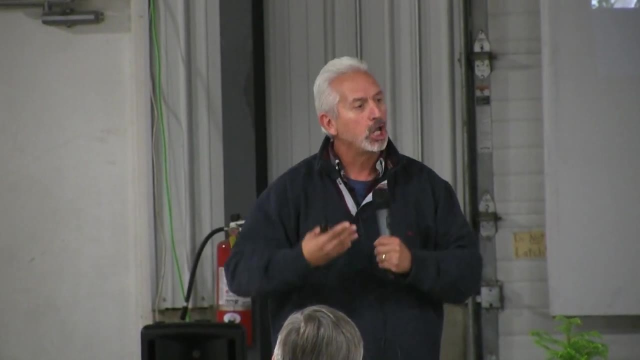 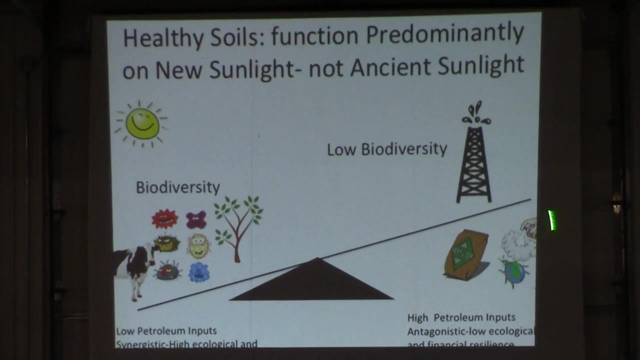 And if you keep growing more corn and more soybean, the prices get more deflated. But the ones that are going to do well is the one that's diversified and synchronized with the natural system, because their inputs are low. So is it run on this or is it run on this? 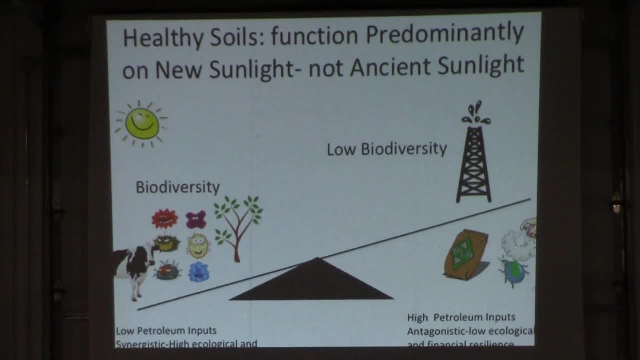 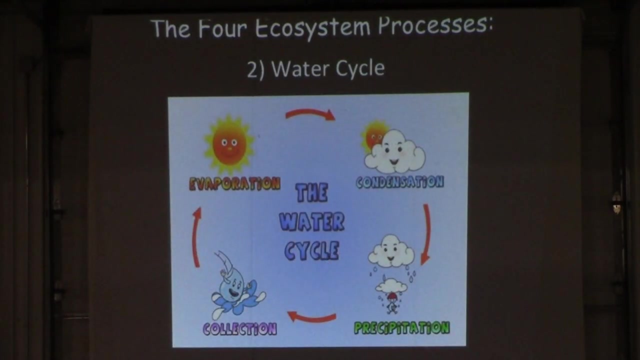 Pretty simple And the soil will tell you if you're doing that. And the checkbook And money, Mama, she knows where the money is flowing. Water cycle: Okay, If I cannot get the water in the ground, in the soil, I can't get nutrient cycling. 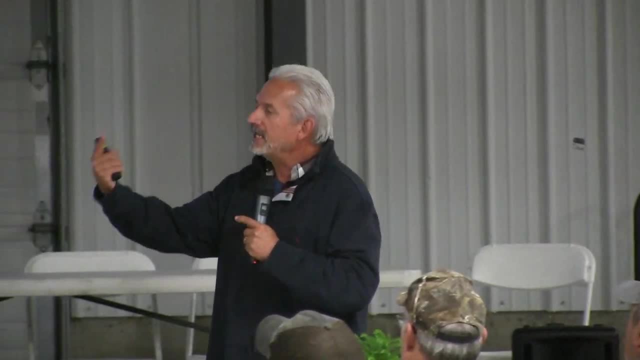 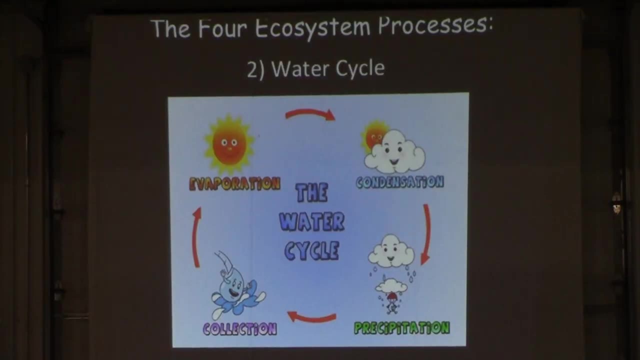 I'm not going to be capturing solar energy efficiently. These are intimately connected. Do not separate these things. Let me show you a dysfunctional water cycle. Water cycle The fully appreciated The potential runoff and erosion from a conventionally tilled field like this would really need to be. 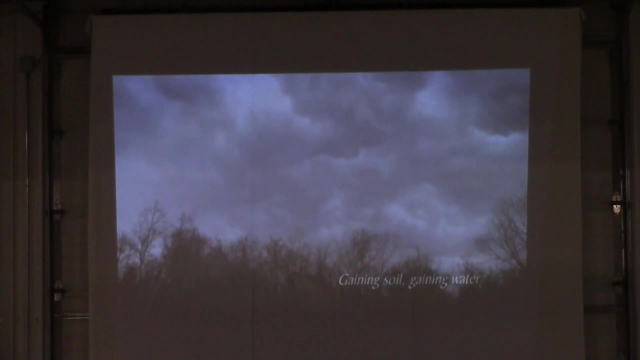 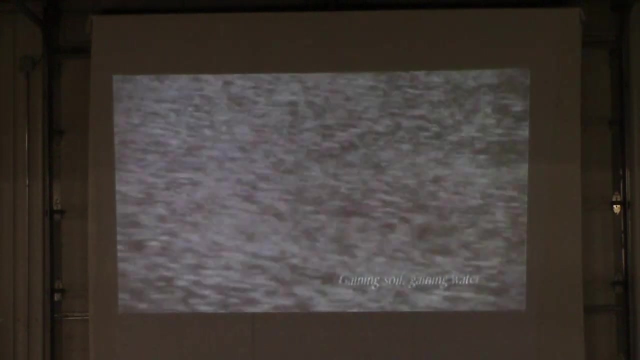 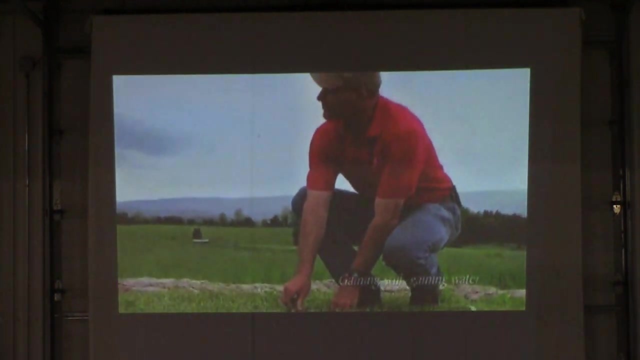 out here during the most intense thunderstorm of the year, Since most people don't want to do that here in Virginia. if you use a rainfall simulator, it will tell a story of what happens when it rains really hard. On the left, we start with a tray of dry, wet soil taken. 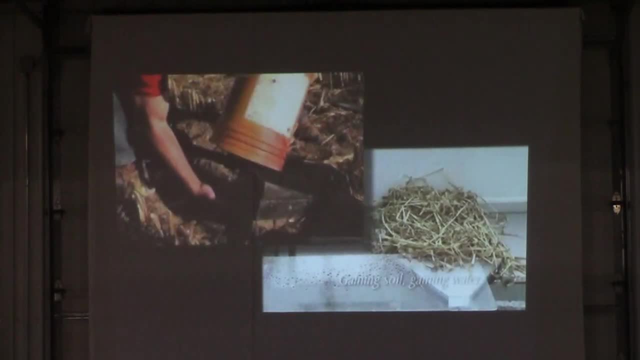 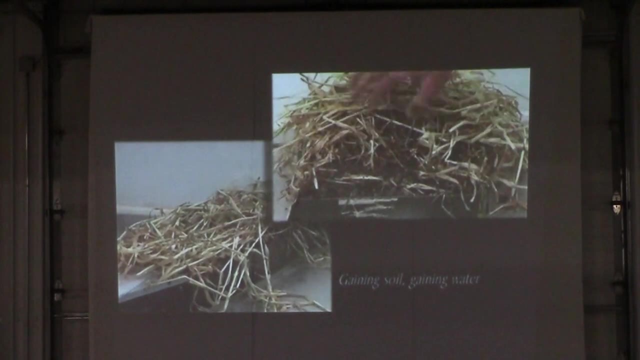 from a clean till field. On the right, we start with a slice of intact surface soil from a long-term no-till field. This soil is not only protected with a mulch of cover crop residue, it also has a stable, porous sponge structure. 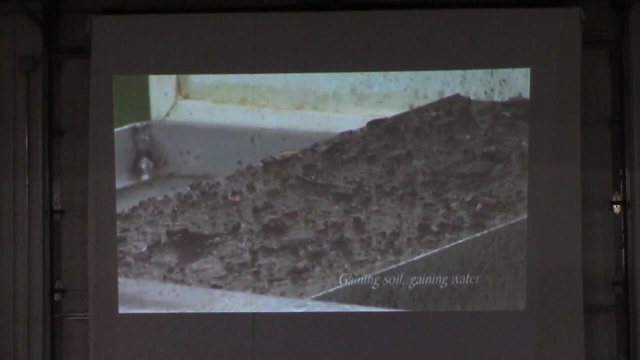 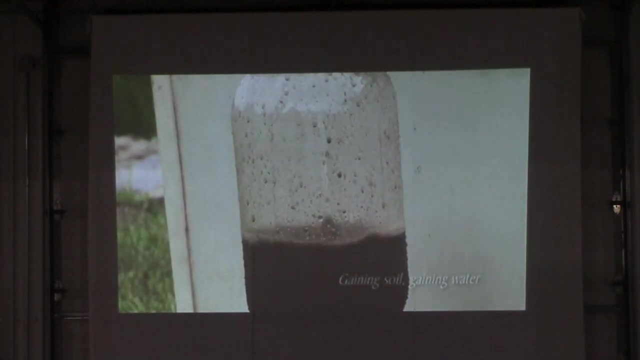 You know, years ago- as a kid I remember- you know you'd get these big heavy thunderstorms in the summer and it would just wash the field And you'd end up with mud down the road- And I'm talking about mud that you'd go over there every day. 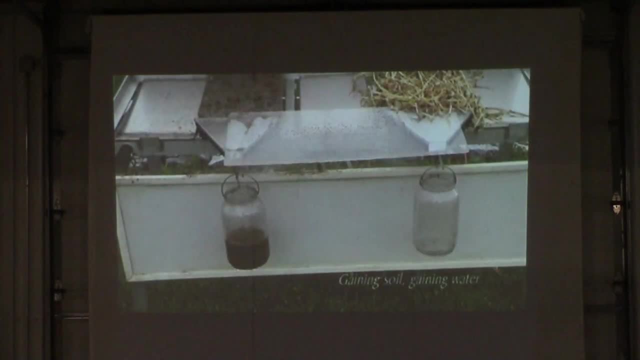 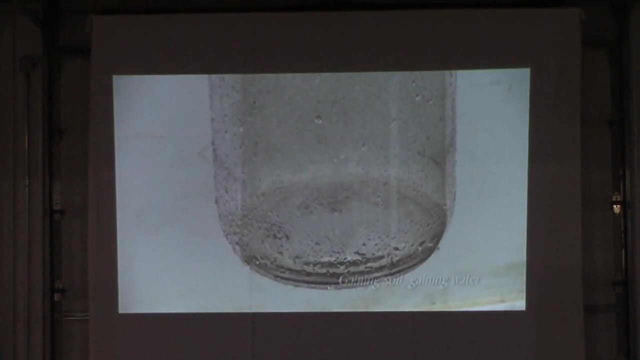 You'd go over there and skid loader and scoop out of the way so the cars could go down the road. What I'm seeing now is I'm seeing these heavy rainfalls and I'm barely seeing a trickle coming out of the field. 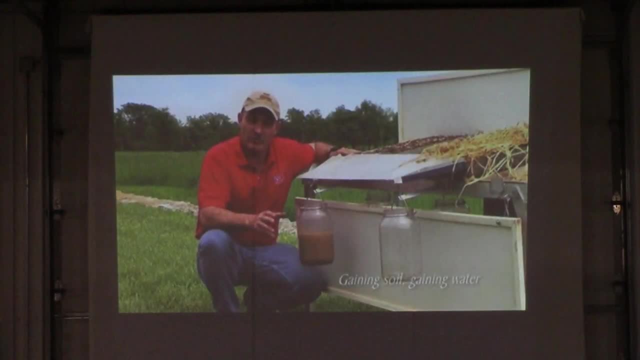 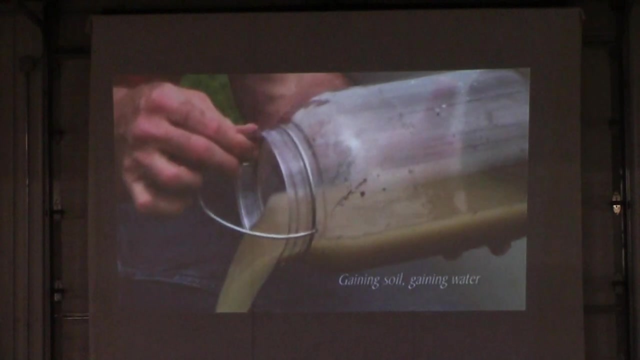 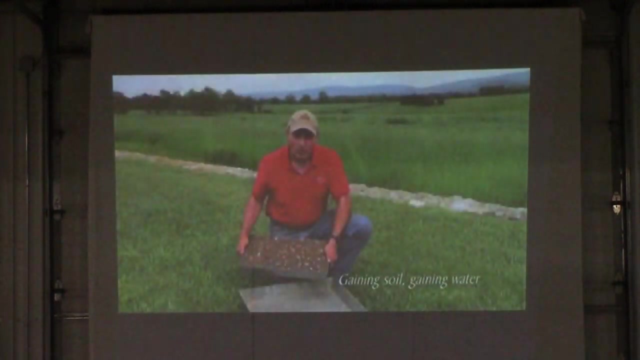 After we simulate an extremely intense thunderstorm for five minutes, the differences are obvious. Most of the water we apply to this soil has run off into this jar, carrying away with it a thin but very significant layer of topsoil. We just applied an inch and a half of very intense rainfall to this bare tilled soil. 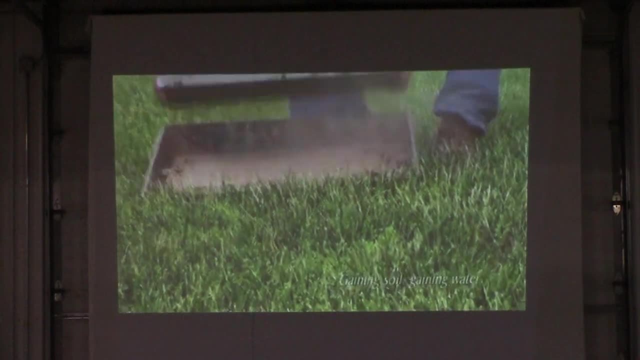 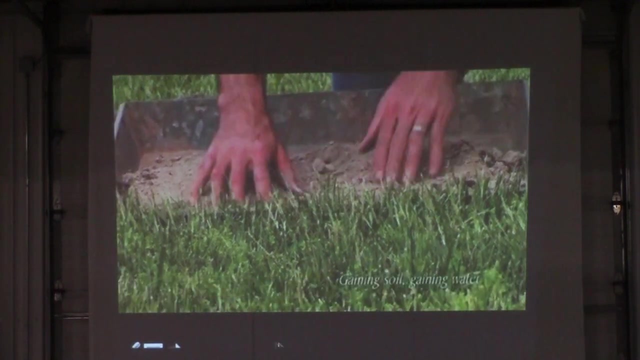 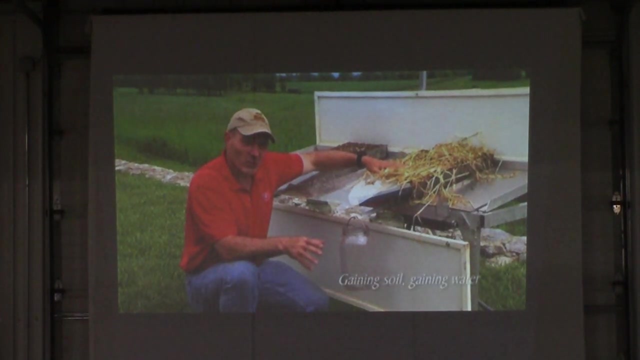 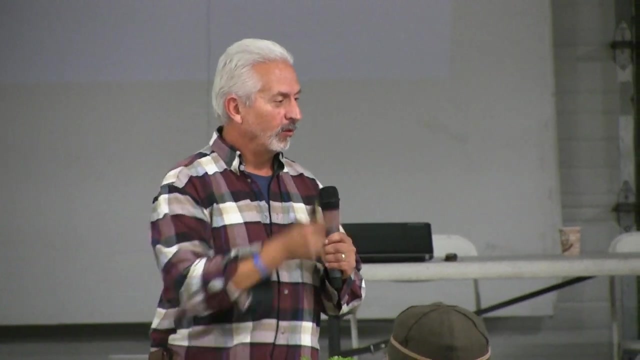 Obviously, we harvested very little for future plant use. Meanwhile, Okay class. How does tillage? Why is tillage so important? It's so destructive, So intrusive. What does it do? Kills the microbes, Kills the microbes, It severs fungus. The minute you till you wake up, bacteria called Ostriches. They're opportunists. They eat the biotic glues. They eat the biotic glues, They start consuming the organic matter. They start consuming the organic matter And then it goes up into the atmosphere. 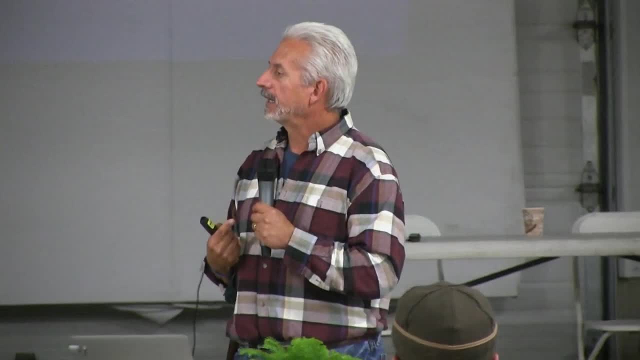 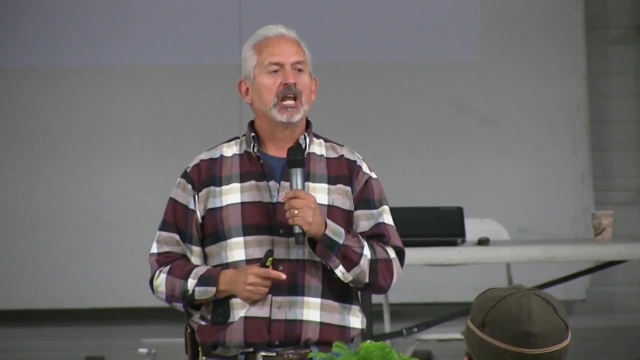 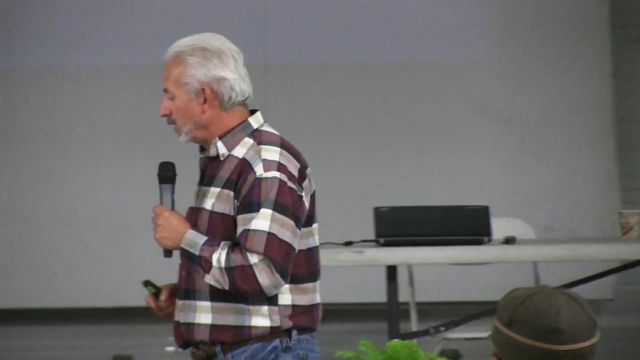 Then you skim it once they die, They stimulate. They stimulate weeds Because they release nitrogen. Please understand: 40% organic matter. It's dead microbe carcasses. If I said the word organic matter, what are some of the things that comes to your mind? 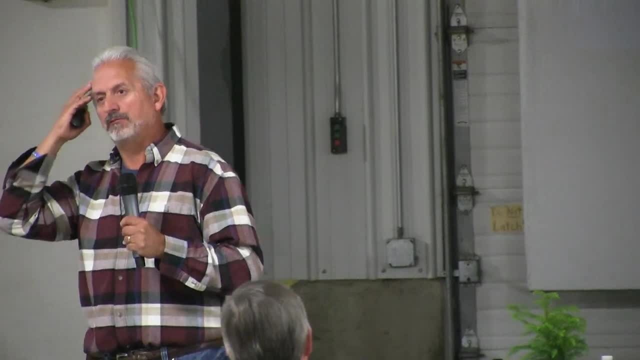 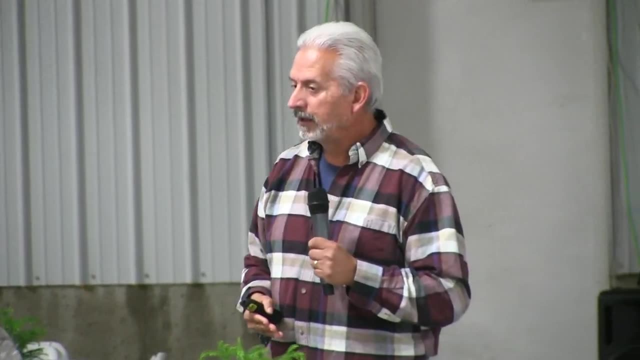 What do you think when you say organic matter? What comes to your mind Quickly Roots? What else do you think? Dead plants Good. What else? Light stuff, That real fluffy dark stuff, right, But how many would say? 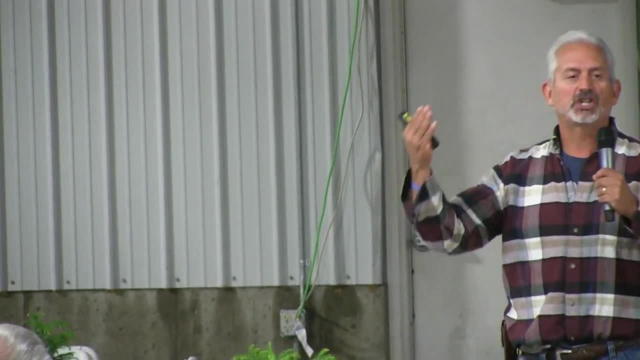 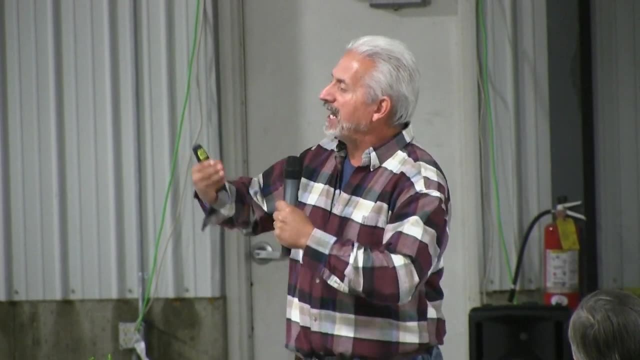 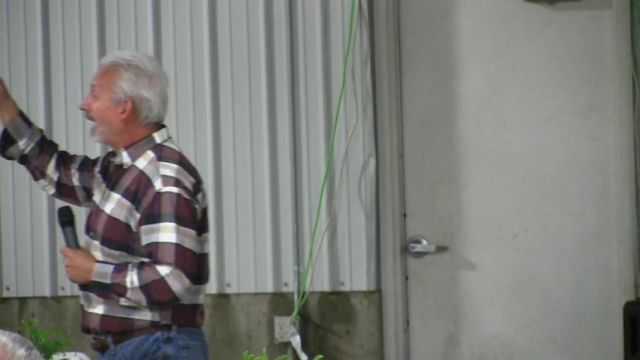 Oh, no, man, we're getting there. It's the excretions and secretions of life and death, of microbes feeding on each other And then, when they die, they create these incredible super molecules that quote the particles That came across my mind right away. right, 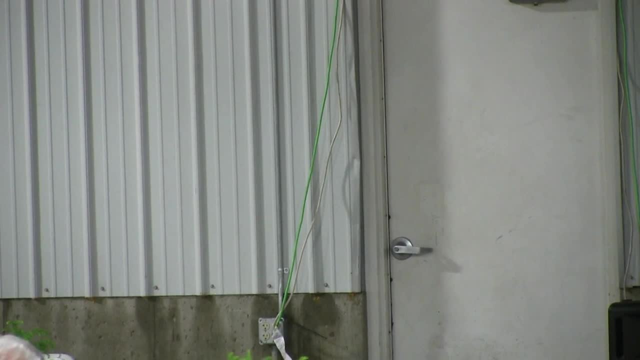 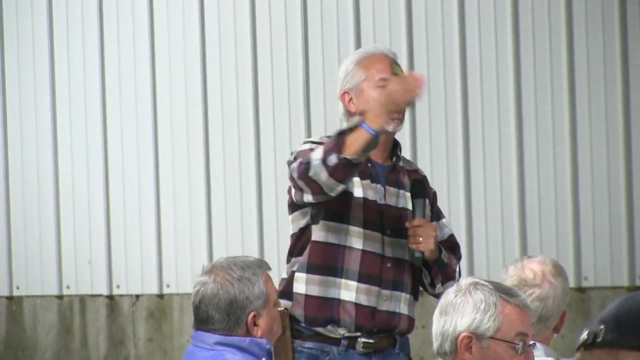 It turns the geology, the sand, silt and clay. I don't care if you're in Minnesota, I don't care if you're in Michigan, I don't care if you're in New Mexico, You all have sand, silt and clay. 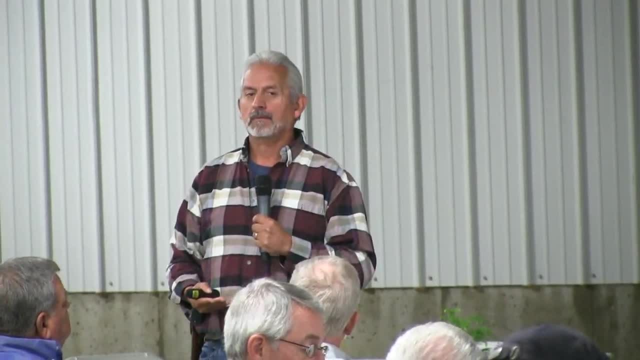 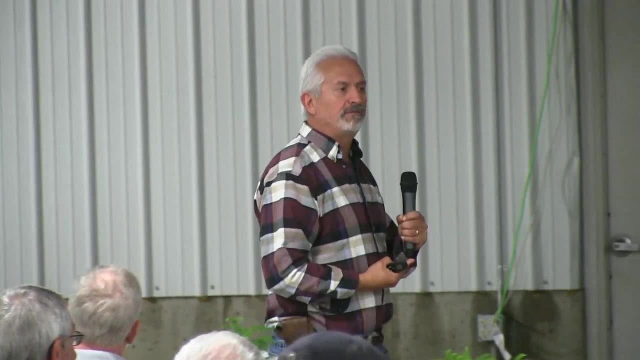 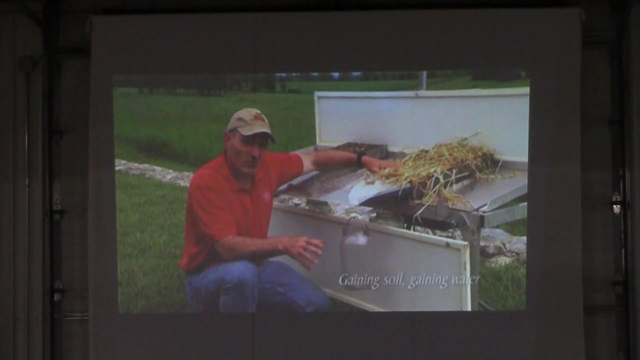 But what is different is the climate and the biological process which happens all over the globe. It's the secretions of life, The fusion. I'll show you in a while. Those glues are gone in that conventional field. Does it happen in our pastoral systems? 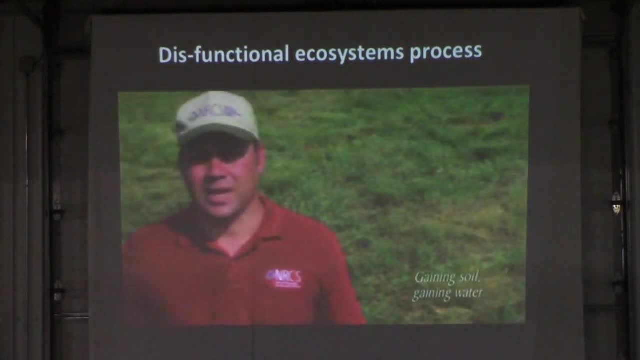 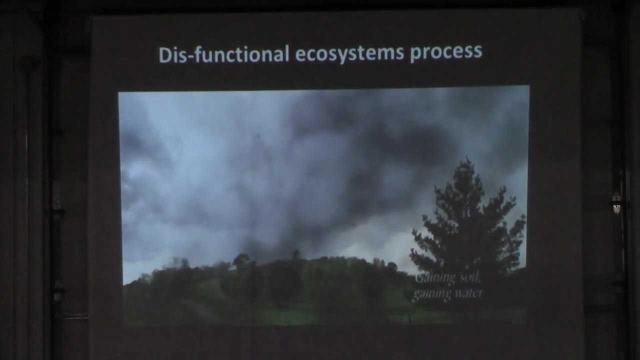 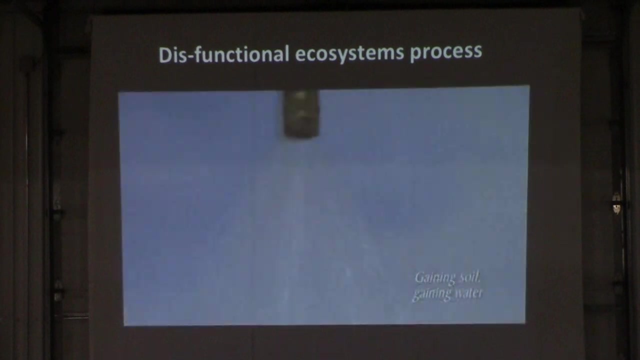 Between a continuous migration, So in our pastoral systems, versus a rotational grazed pasture. to really see the difference, you actually have to be out there during the heaviest thunderstorm of the year. NRCS uses a rainfall simulator to demonstrate the effects of infiltration. 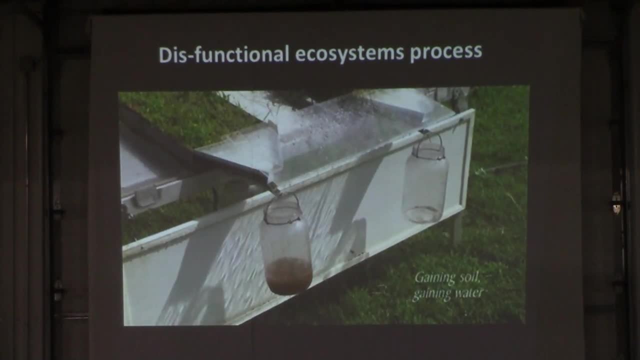 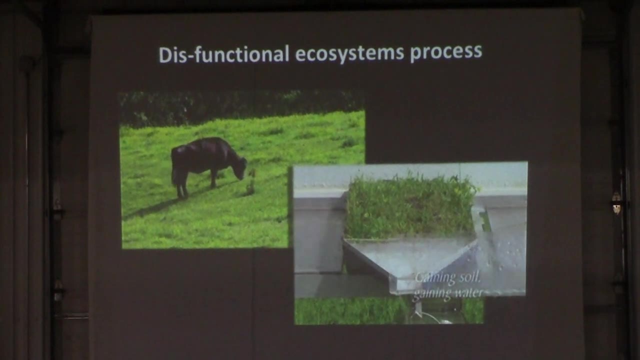 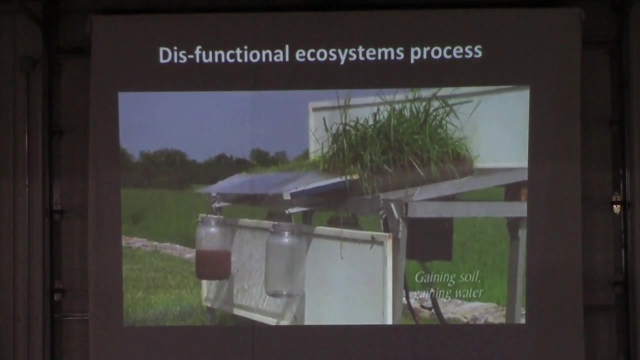 versus runoff on pasture surfaces. These pasture samples were collected from actual pastures just down the road from each other. One represents continuous overstock and overgrazed pasture. The other represents a rotational grade produced in rest of the pasture. All rainfall runoff is funneled. 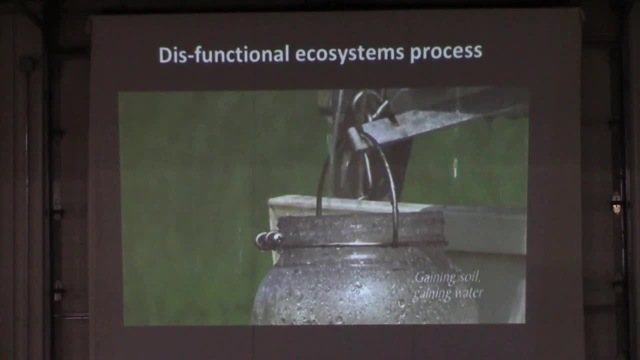 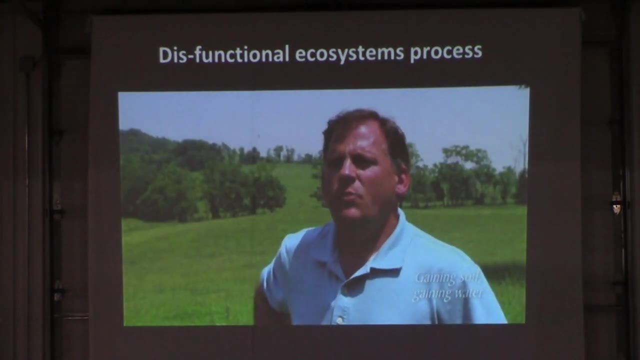 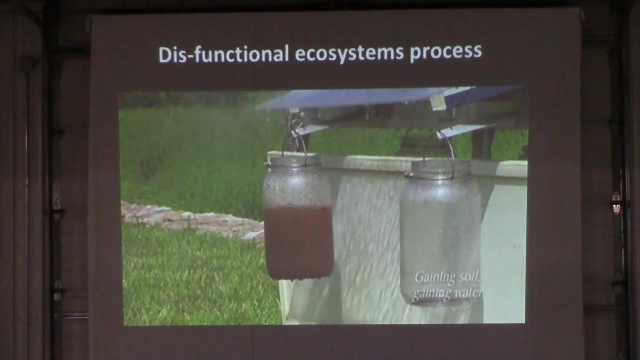 into a collection jug on the front of the demonstration table. This allows us to visually compare both the volume and clarity of the runoff. The most important nutrient we have to manage is water. With rotational grazing, particularly during the summer, we have more water infiltration. 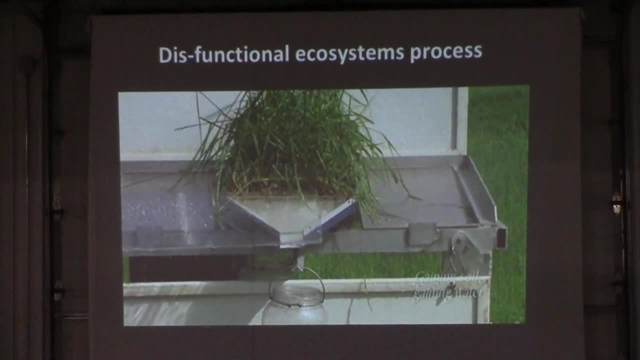 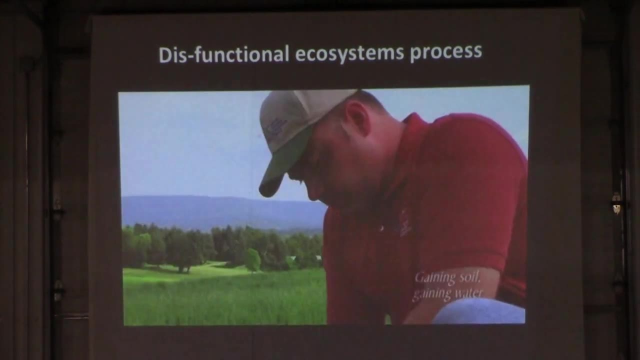 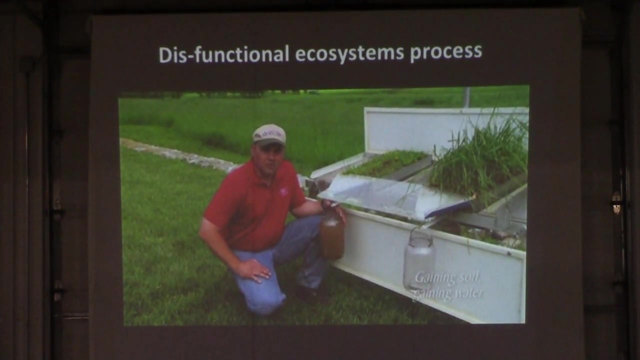 because we have a better cover on the ground. The sanctuary cover intercepts the water particle and allows it to run off. By the end of the demonstration it's amazing to see how much more runoff occurs on the continuous overgrazed pasture versus the well rested. 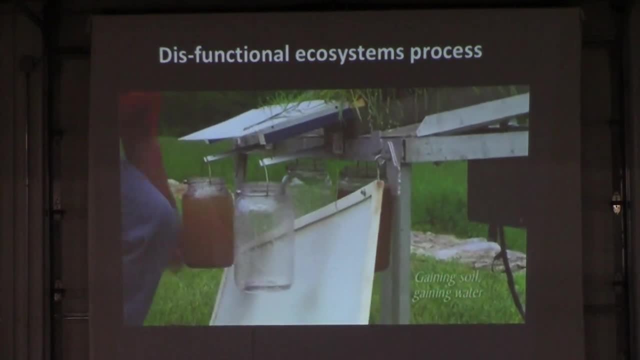 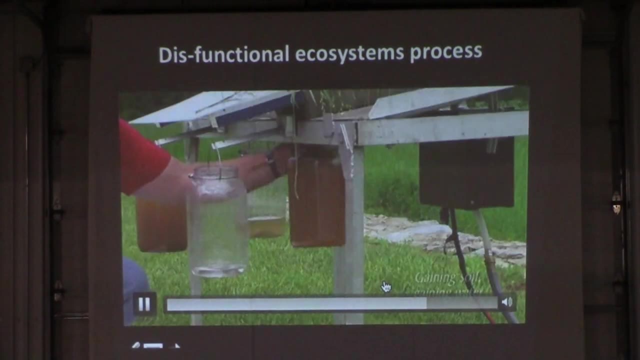 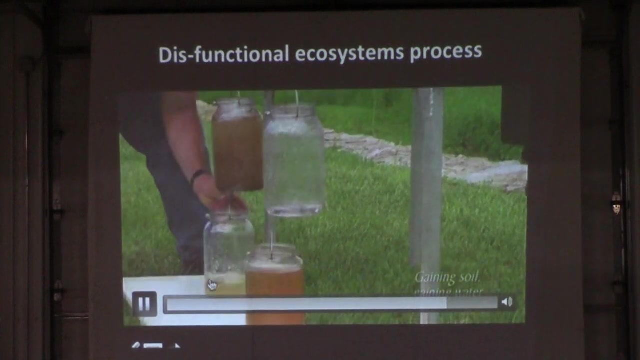 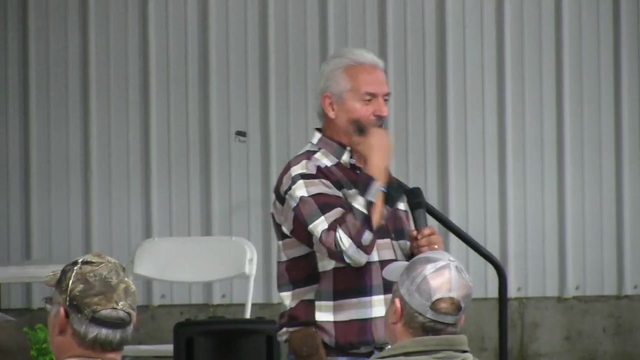 rotational grazed pasture. Here you can see how much more water looks in and absorbs over the rotational grazed, well rested pasture and how much more water actually runs off. Hey class, Make sure you're not away, Make sure you're awake. How come so much water came out of that? 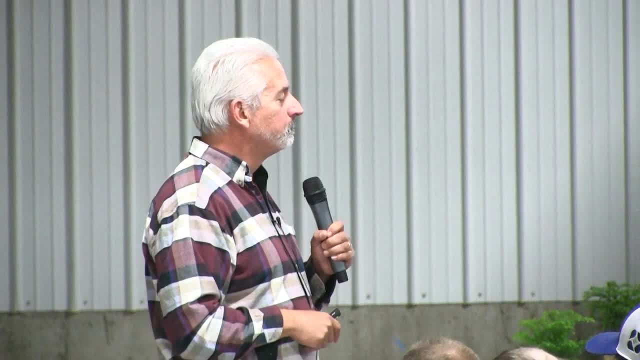 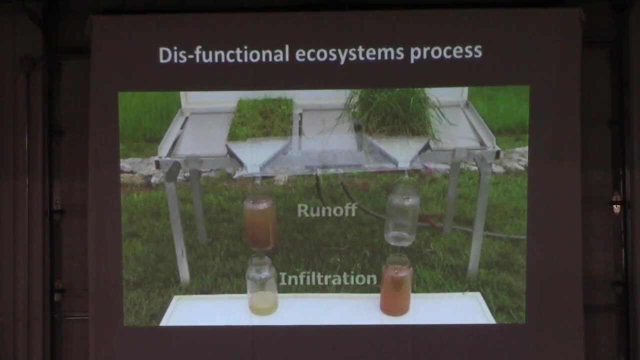 overgrazed pasture class. Come on Confidence. What happened? You didn't till it, It's not tilled. Look how much sediment came off Sediment. Look how much infiltrated. So what's going on? What do you think? 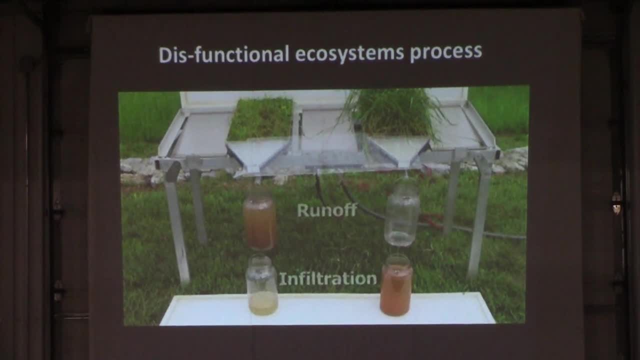 No aggregation. Good, Good comment. Has the aggregation different from here to here? If I did the slake test, if I did a slake test, would it break up? Do you think it would hold together or would it break up? 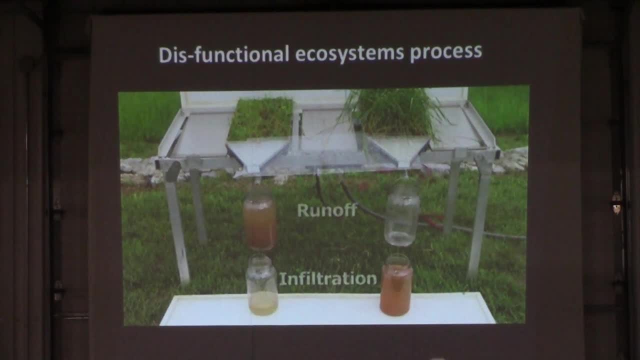 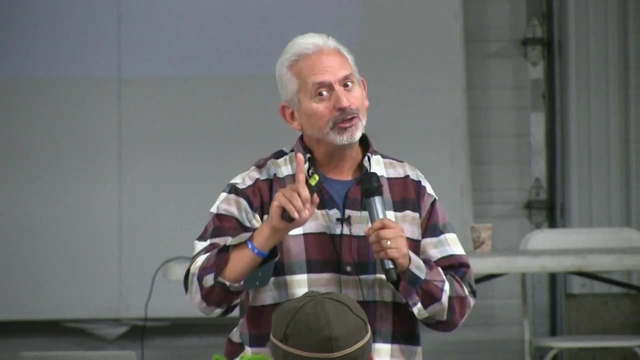 You think so It would hold, But you're right. You'd have to take it to a lab to see the diminished aggregate stability. You're right, But you can't do it with a slake test From visual. look at the difference. 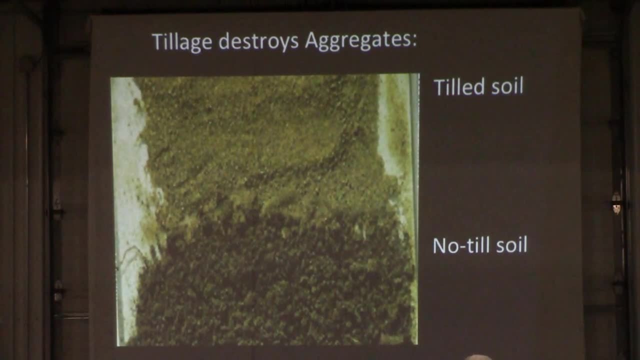 The cottage cheese is gone. It's been tilled. It's gone. It's overgrazed. When you overgraze, you affect the biology. When you till, you affect the biology. It takes a lot of energy. See those aggregates. 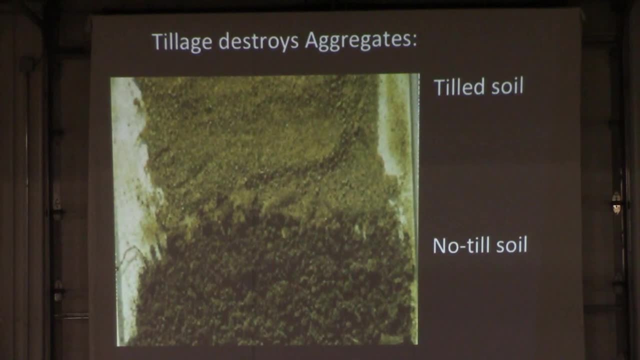 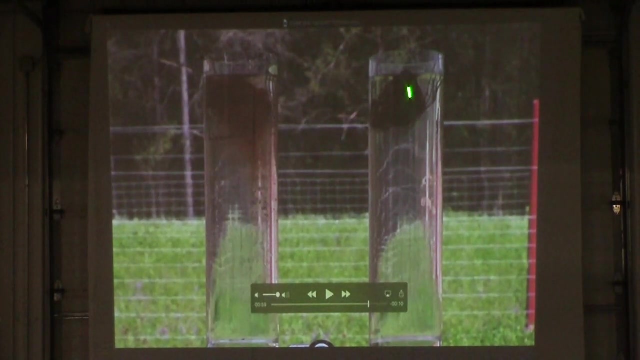 only last 37 days. You have to be feeding them all the time. It takes a lot of carbon to feed those. It takes microbes, It takes fungus earthworms. Let me show you this slake test. This is a 6.5% organic matter. 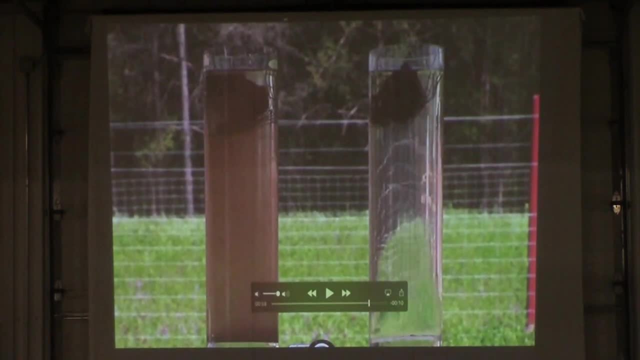 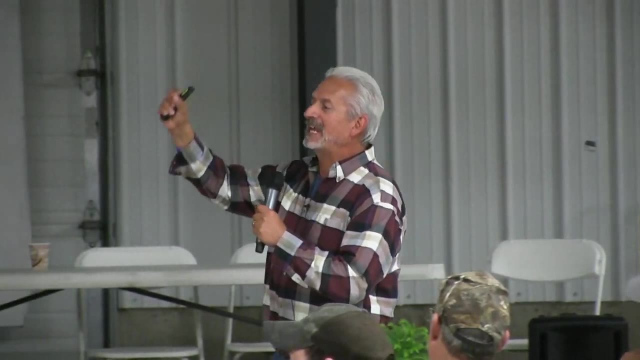 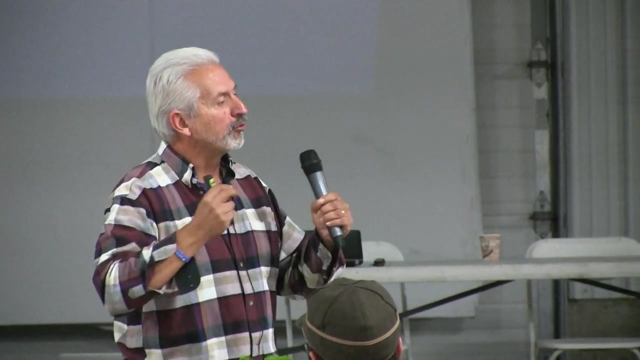 This is half a percent same soil. See, what happens is there's no more biotic glues. and the sands and silts and the clay they disassociate. Now they fill the pores. Now you have runoff. It does not have the glues, It does not have. 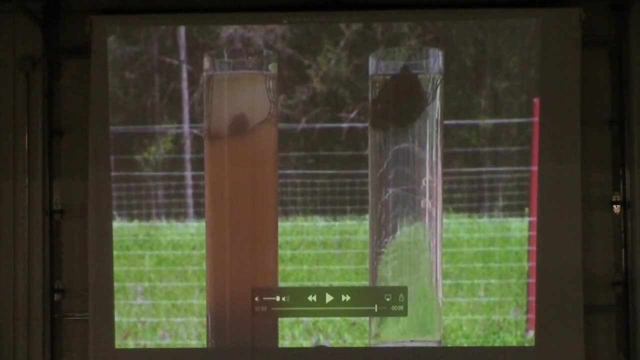 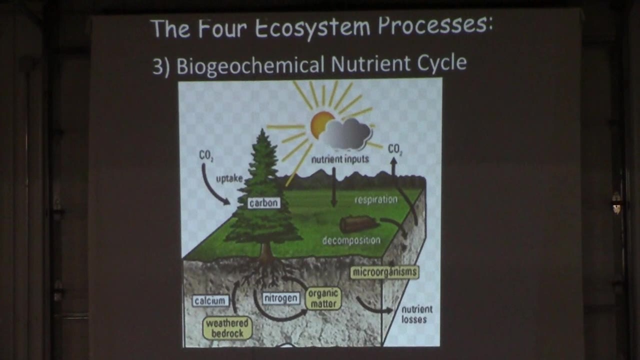 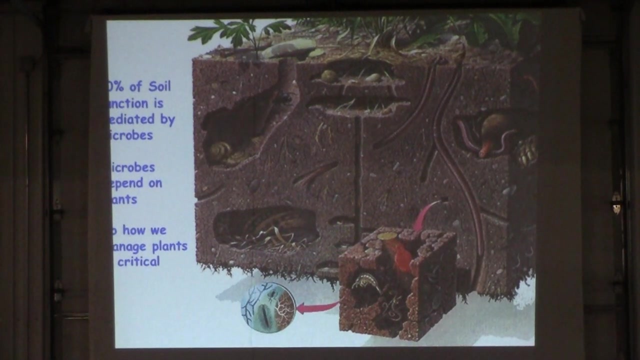 the integrity Now biogeochemical nutrient cycle. This is one of the reasons why we have so many leaky systems. Most people don't realize 90% of our nutrients, nitrogen especially, is biological. It comes from the microbes. 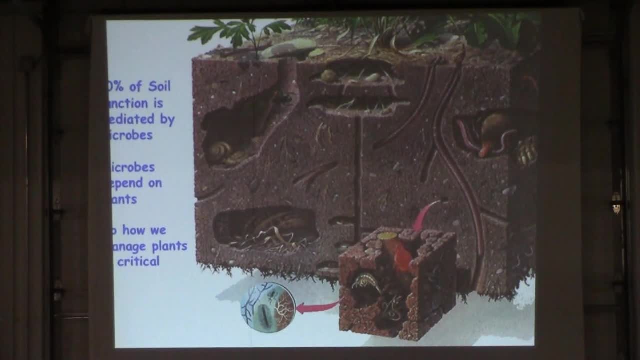 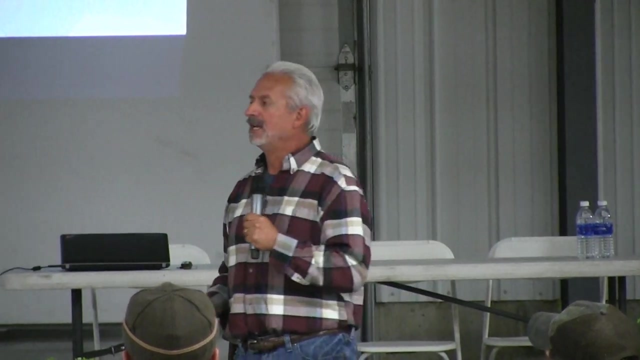 They produce 90%. See, most people think that fertilizer feeds the plant. Fertilizer does not feed the plant. You heard the speaker, two speakers before from the guy from Europe. 30-40% of that nitrogen only reaches the plant. 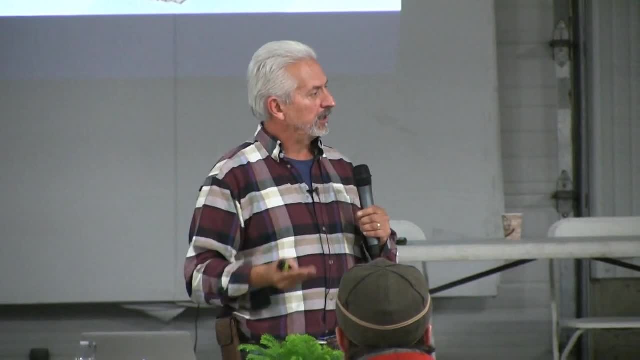 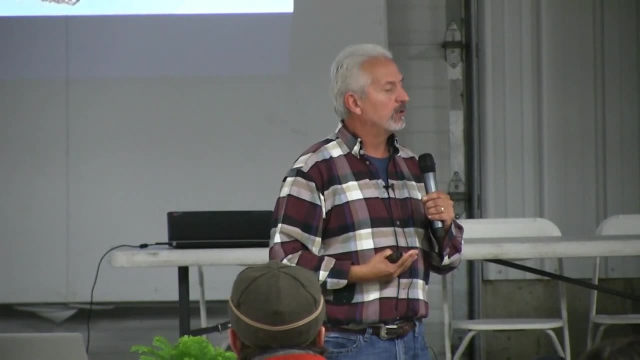 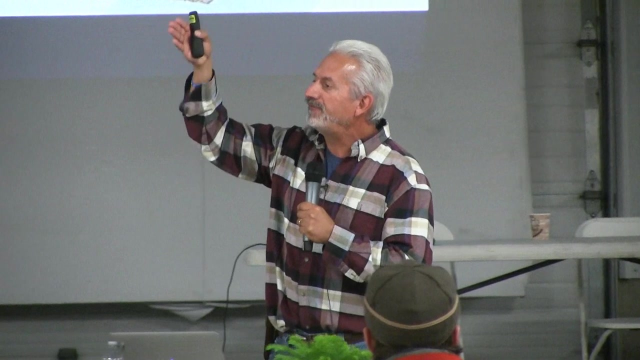 60% is gone. It's either leaked, leached off, but a majority- the mafia, take it. Who's the mafia? The microbes. They're the first feeders. guys, Please understand, they feed first, They're the first. 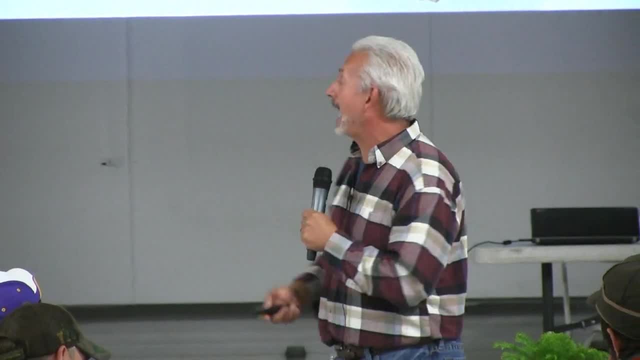 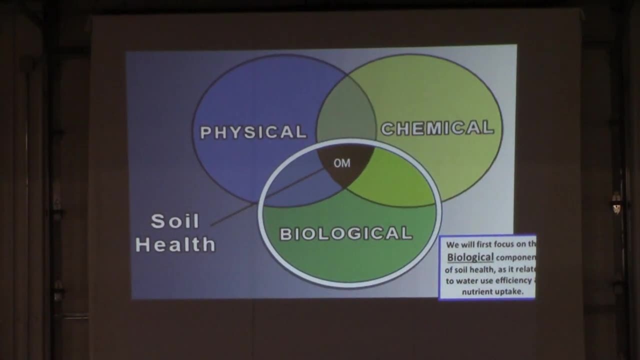 feeders, not plants. They'll take the nitrogen and they'll release it back. This is the paradigm I got out of soil science. See, this is where it starts changing. I was taught that biology, the physical and the chemical all are of equal value and importance. 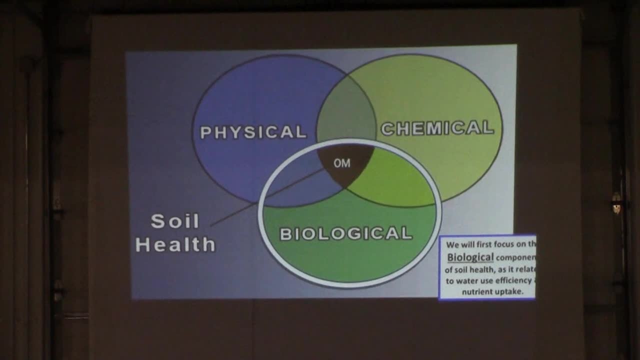 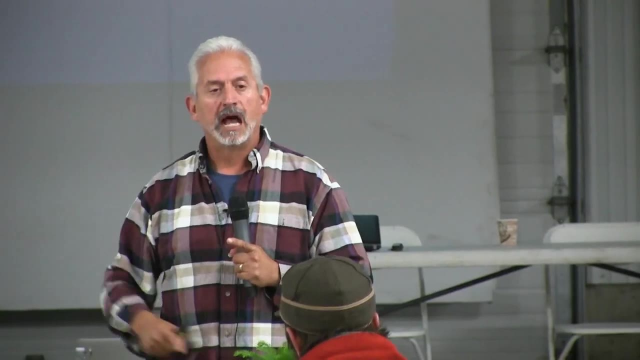 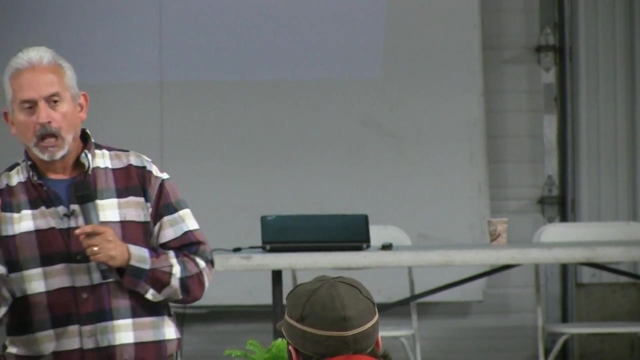 That's why the circles are all equal size. Do you agree with that chart? How many are like with him? How many agree with that? Raise your hand. Oh, you're afraid to raise your hand, aren't you? He's right. 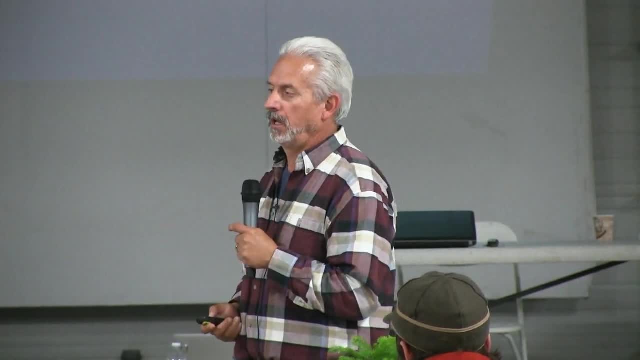 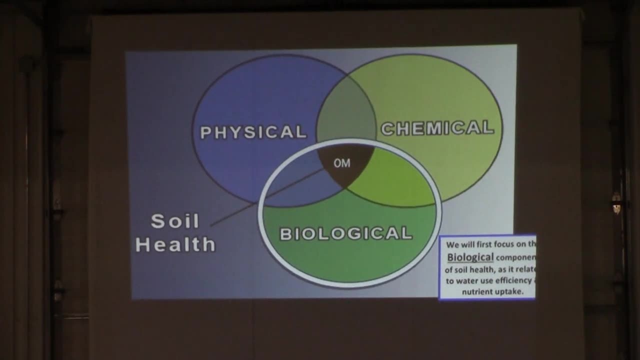 They're not equal value. They're not equal value. Biology builds the structure, builds the glues. In fact, without biology, you can't have organic matter, You can't have those biotic substances, And it's that that regulates the chemistry. 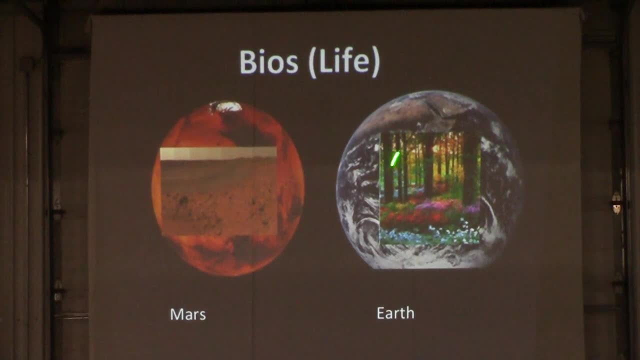 Example: Mars, chemical physical, Earth, chemical physical. They're both chemical physical. What's the difference between them? Biology, Life, Life. They are totally different. They're not of equal value. They will never be of equal value. 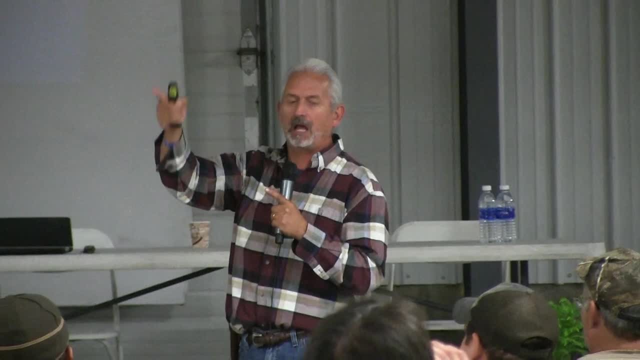 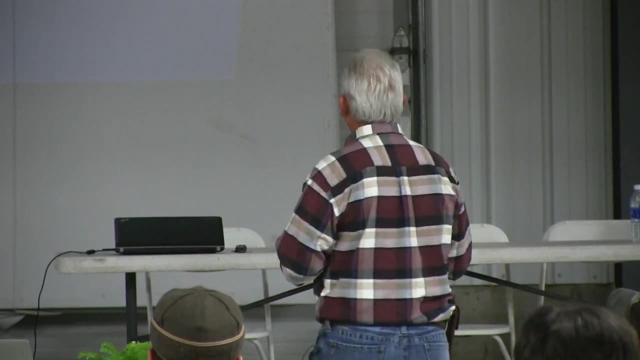 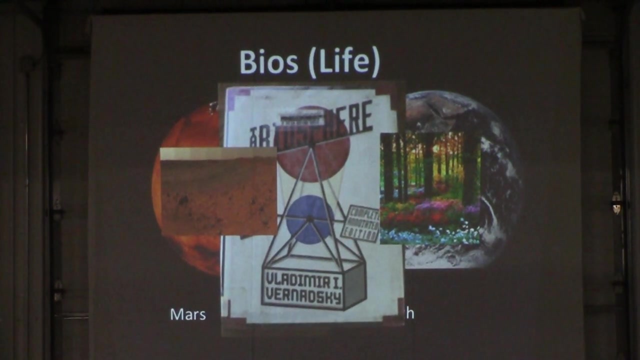 Until that is absorbed in your mind- that you, your soil, is a biological system, you will not change the way you do business. There's a great book. Whoever wants to muster the strength to read it. it's called by Vladimir Vrndisky. 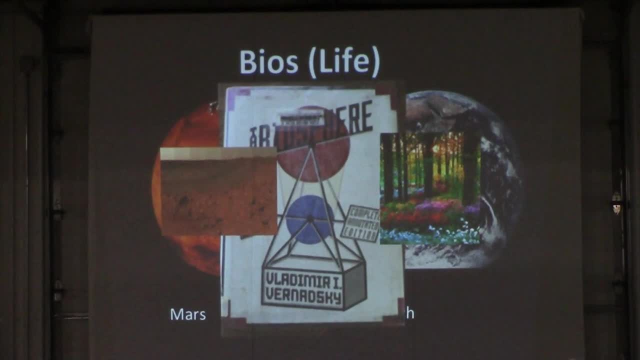 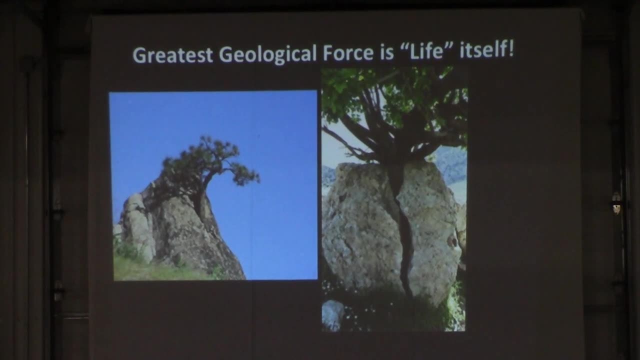 The Russians were so far ahead of us. He said: the most powerful force that you can do in the globe is biology. Let me show you. That is amazing. I love that. How many have seen that? Raise your hand. You've seen it? huh. 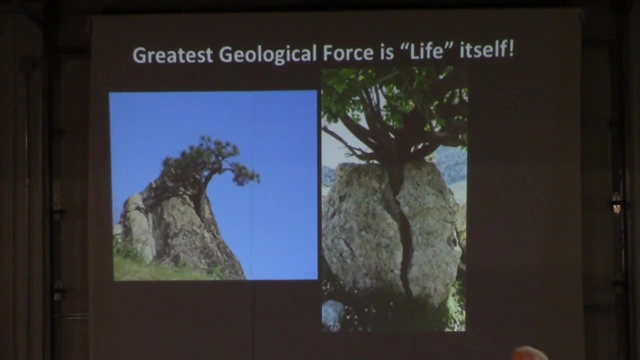 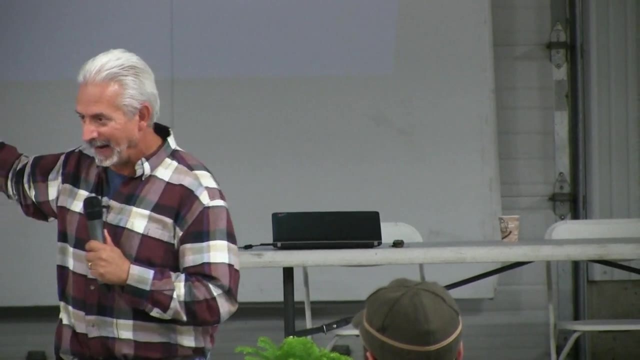 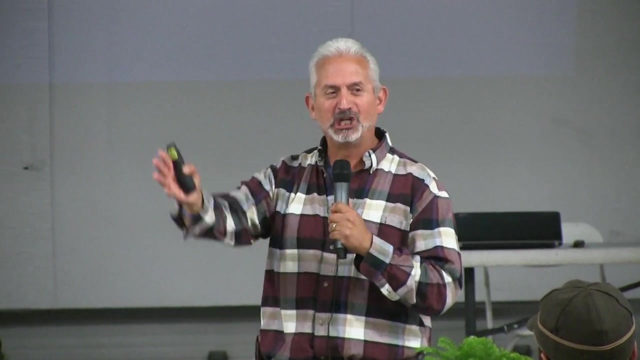 Isn't that cool. I tell farmers that's a compaction issue, That's compaction. So what do farmers do to break up compaction? They get a plot. Let's break it up. man, Diesel, Horsepower. Ladies and gentlemen, 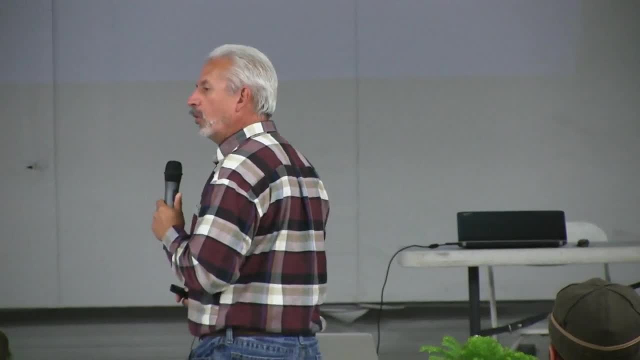 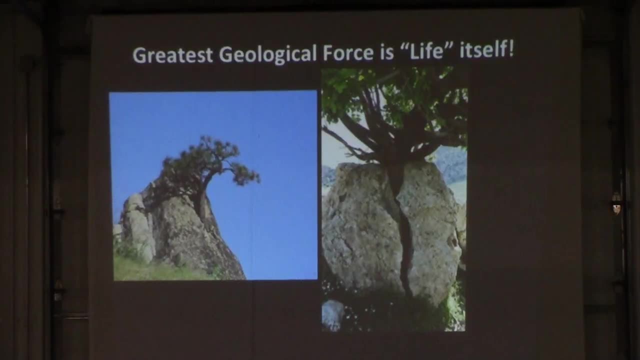 I could never explain years ago why that happened. I would sit there and go. how does it do that, Ladies and gentlemen? those trees are incredibly mycorrhizal fungi. These fungus release these powerful enzymes, dissolve the rock down Bacteria. 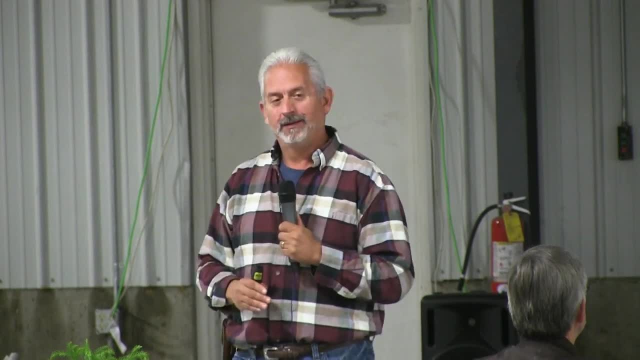 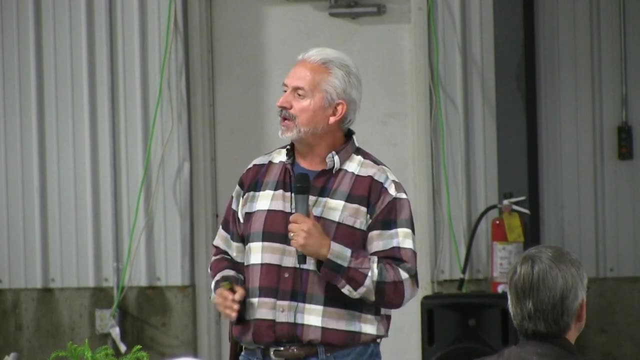 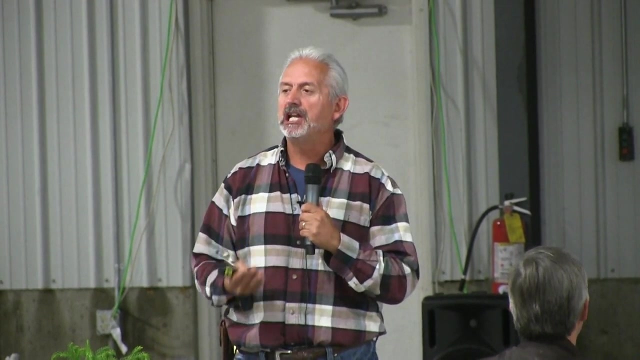 can break rock down. If it does that, what is the most powerful thing I can stick in my farm right after corn and soybean Living cover. See, your plowing disc can't leak these powerful enzymes and they cannot leak these acids. 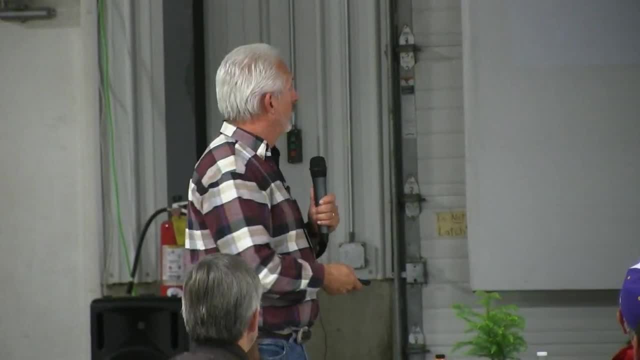 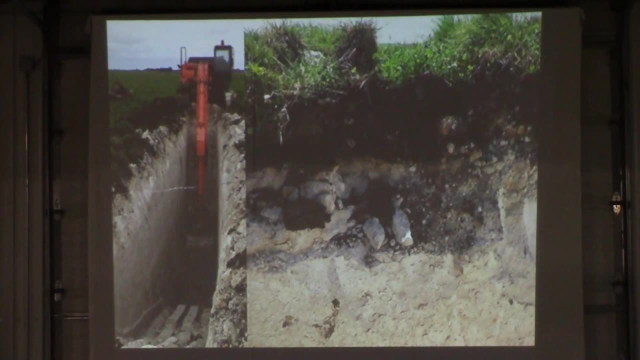 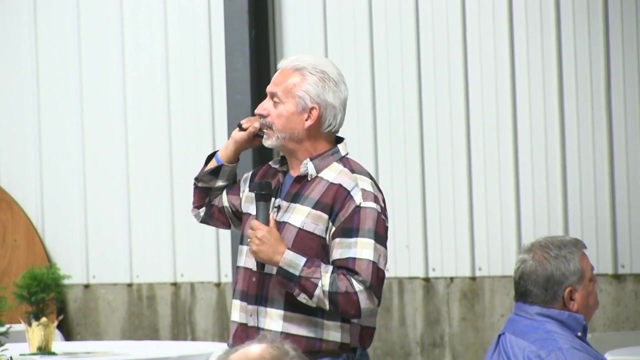 Tillage fixes nothing. Life does Look how powerful it is. Ladies and gentlemen, that is it. You think you have it rough. How would you like to farm that? That sucks. Southern Missouri is pretty close to that where I live. 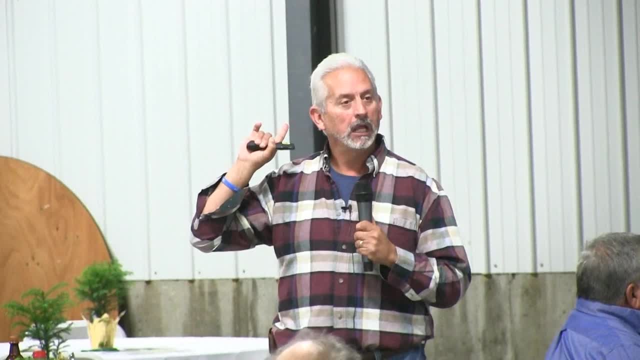 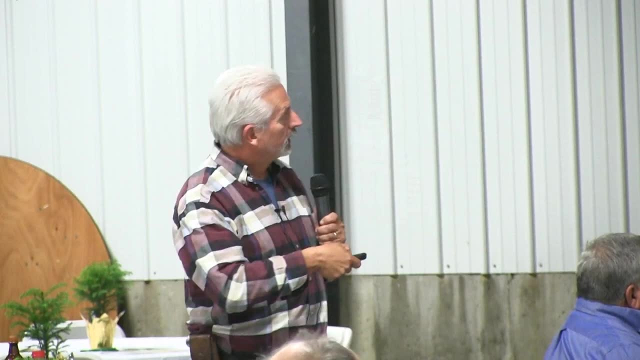 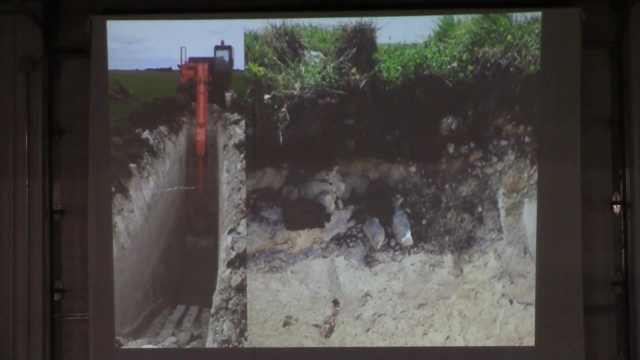 That's why I only spend $1,800 an acre, Because most of my land is rock And I'm good with it Once I understand biology, That's old calcium carbonate sea beds. I have a question for you, sir. How come it's dark up here? 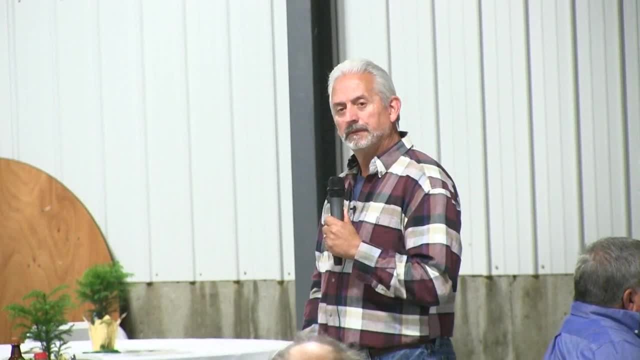 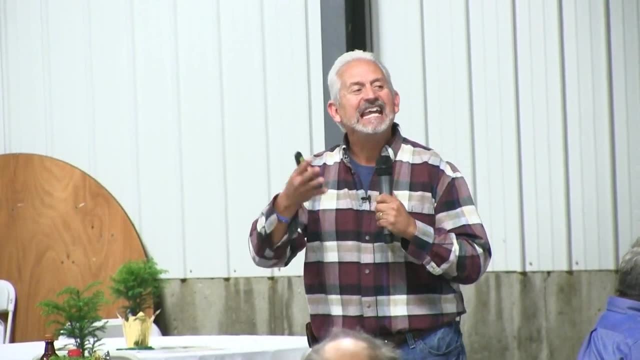 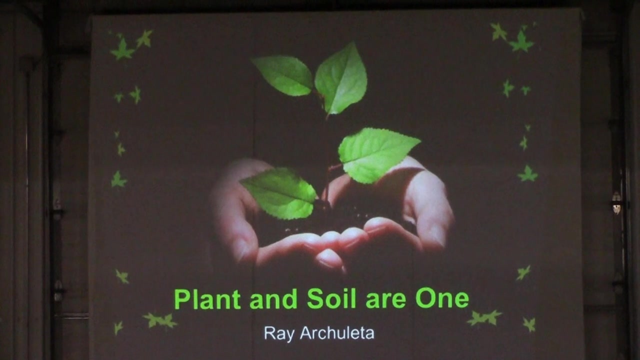 The power of biology. We underestimate the power of it. We've been so busy doing the sides. One night, after reading a research paper from a brilliant scientist, I come running out of my bedroom like I had fire on my hair. I said, wife, I get it. 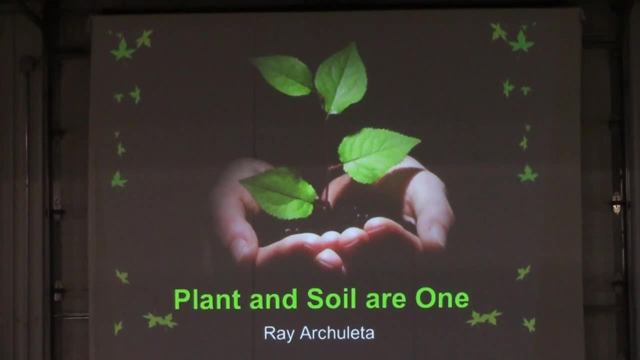 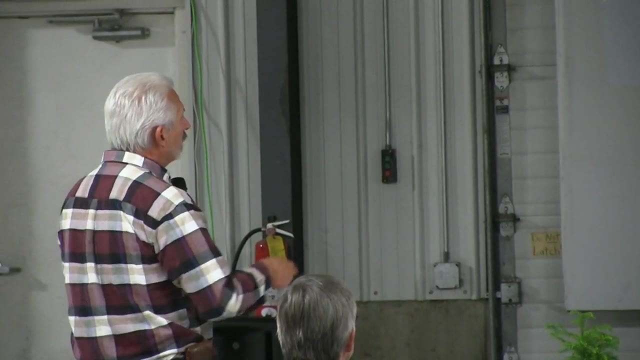 She goes: what husband? The plant and soil are one. She rolled her eyes. She goes: oh my God, that guy's disturbed. I can't even take him back. Understand it's one. The moment you get your corn and soybean, you make it one again. 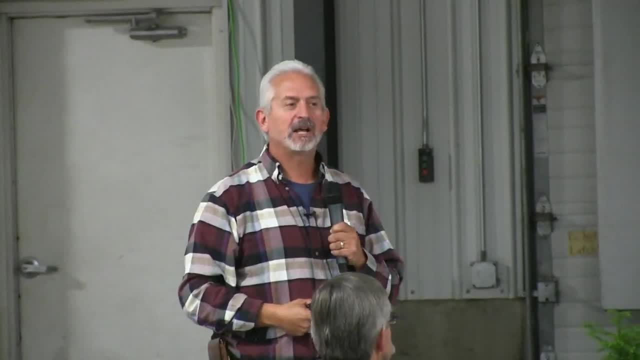 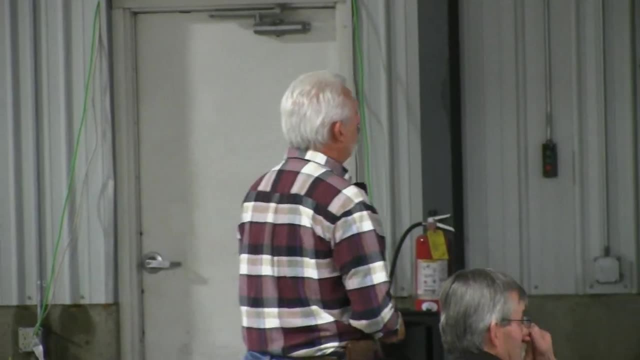 Cover crops are not optional. When somebody tells me I don't want to do cover crops, I smile. You don't know how the soil works, do you? Let me show you some more. Build my point. This is what I want, ladies and gentlemen. This is why. 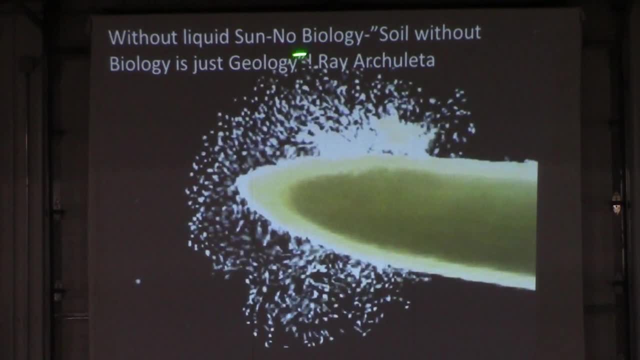 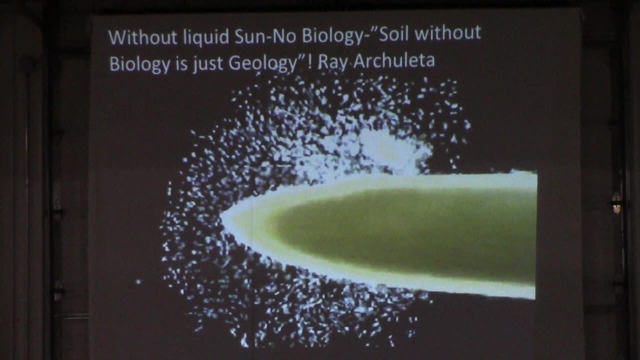 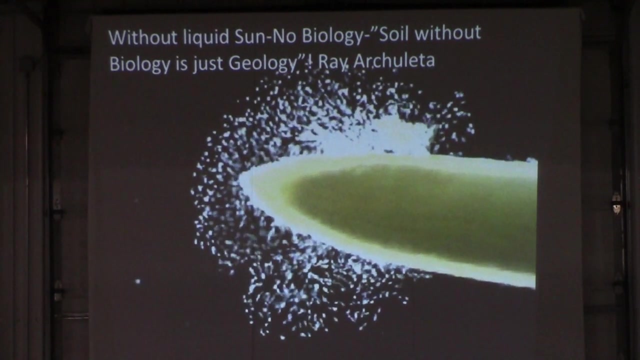 corn, does that? soybean? every living plant that is a root exuding liquid sun into the soil. They will leak 40 to 70% of their energy to feed microbes, to make an association and say: look you, give me liquid sun, I will bring zinc. 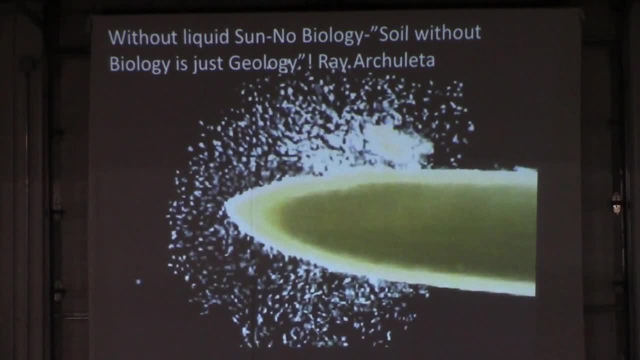 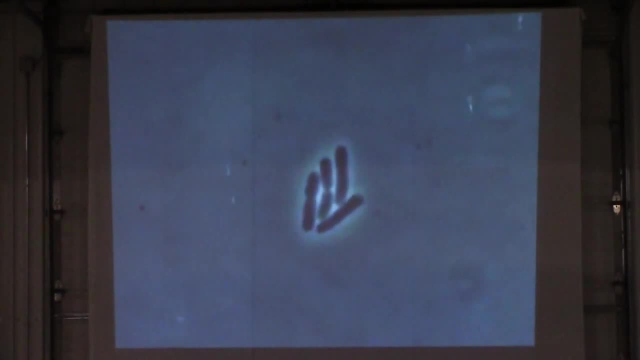 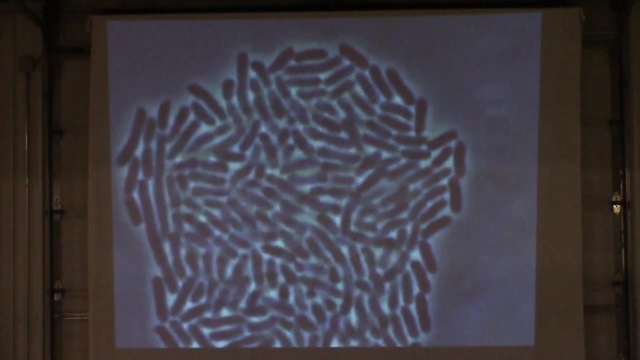 I will bring phosphorus, I will take it out of the rock, I will make it available to you. They're not doing it for free, And the moment I do that, then the bacteria populate like crazy. They replicate every 20 minutes. 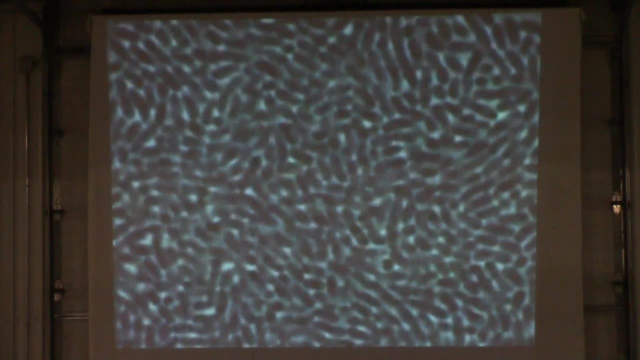 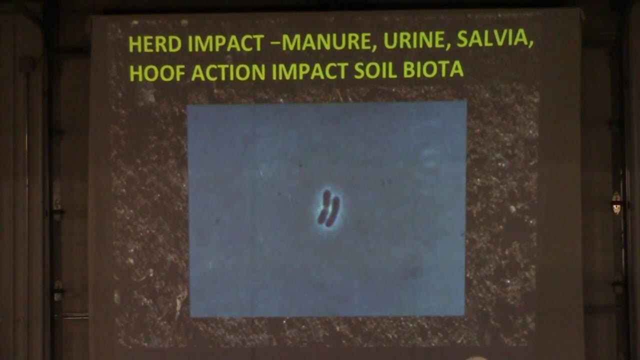 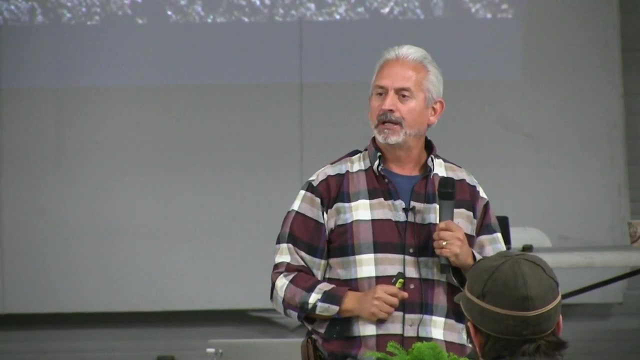 from billions of them And they are so fast. We are seeing, when we put our CO2 respiration, that they're like spontaneous, That the CO2 respiration just goes crazy after one rain, After 24 hours, So the moment. and then the other critters. 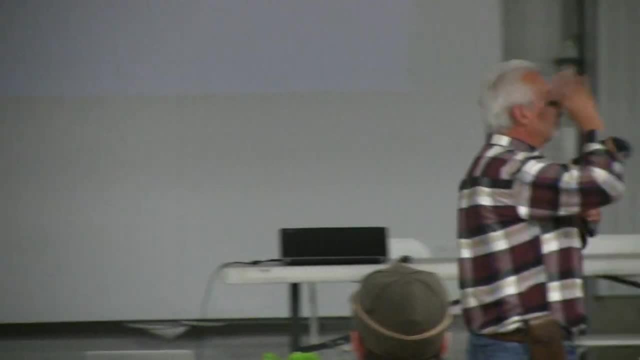 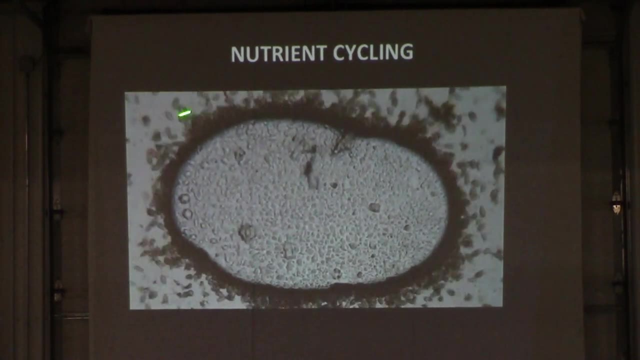 come and eat them. This is what happens, Because you're wondering where all the nitrogen is coming from. These are protozoa grazing around an air bubble and they're consuming bacteria. See when the protozoa eats a bacteria and they have a higher carbon. 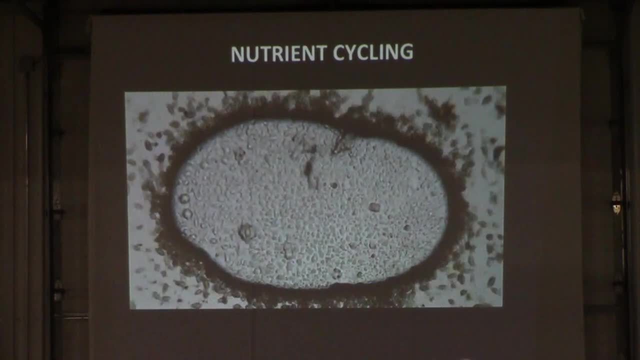 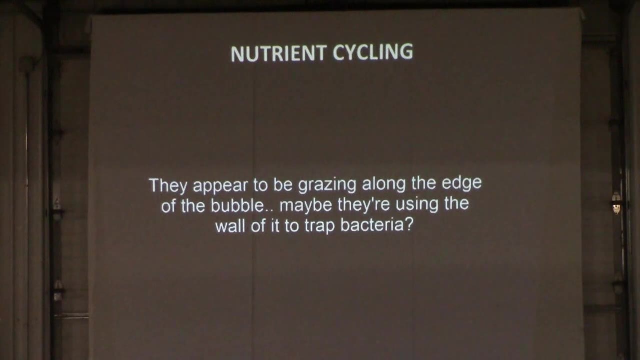 nitrogen ratio, the bacteria. so it's excess nitrogen. they excrete it. So there's 17 to 117 pounds of N. I didn't make that up. Dr Patrick Lavelle, buy his book on soil ecology Powerful. That's what we can do. 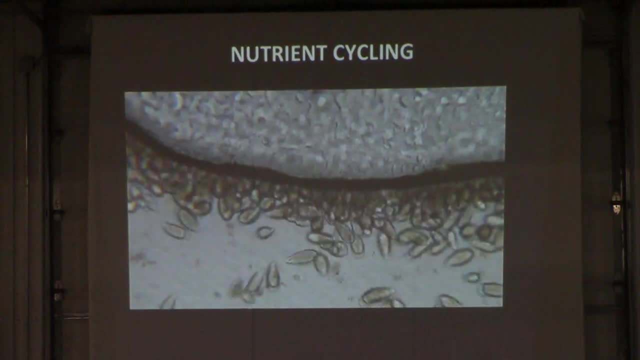 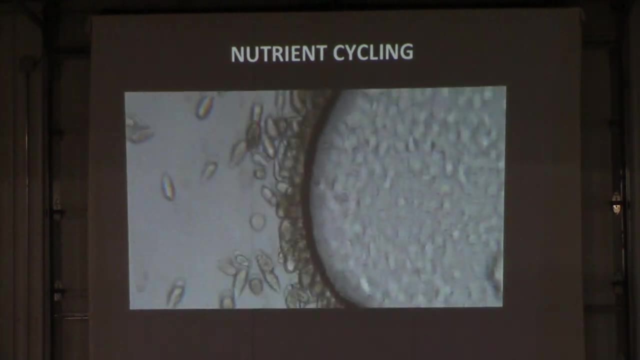 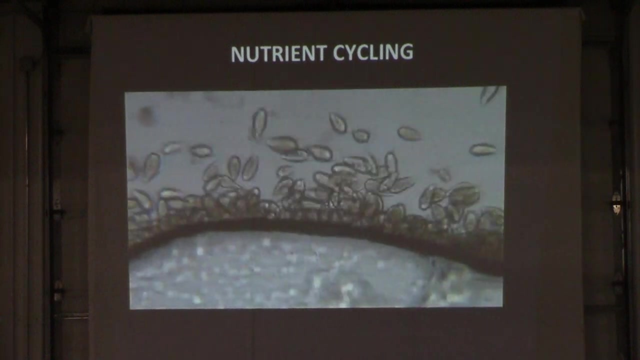 with biology. This is where our nitrogen And what I love about it, these bacteria and all these organisms do it at room temperature. I don't have to copious amounts of natural gas to make chemical fertilizer. They do it. They're my little fertilizer. 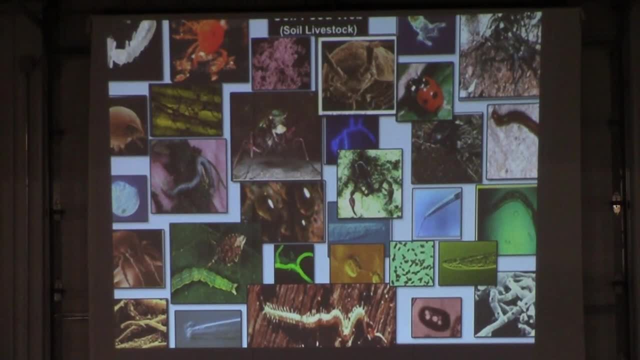 bags. This is the part I missed. I missed this, Did not realize they run the nutrient cycle. They run the nutrient cycle. They're part of the water cycle. See, if you have no aggregates, if the water does not go into the ground, your water cycle. 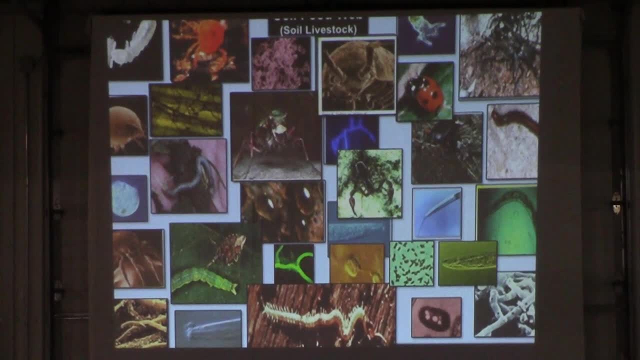 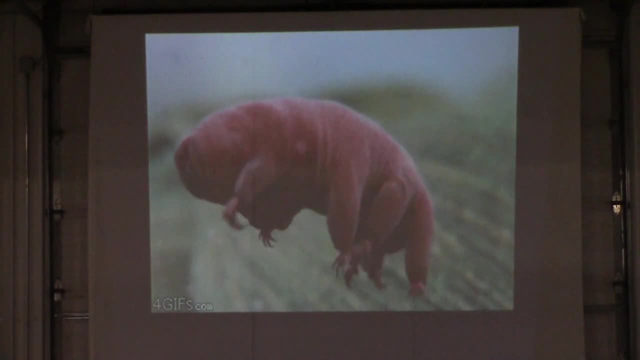 is diminished. I would have never thought the microbes are connected to the water cycle. Wow, Now that is. when I see that beauty, I get goosebumps. That's what you're dealing with, folks. That's a water bear, It's an aquatic. 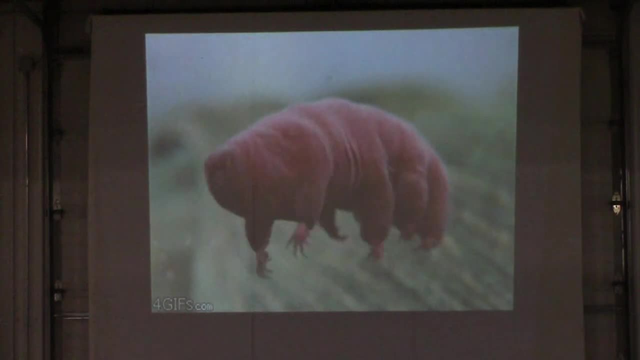 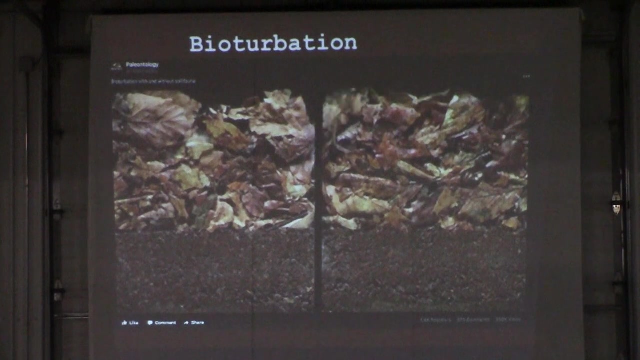 and it's in our soil, in our water systems. It's a subaquatic organism. Soils are subaquatic, They're subaquatic, They fork on water. Now people say: well, Ray, if you have a residue problem, you have. 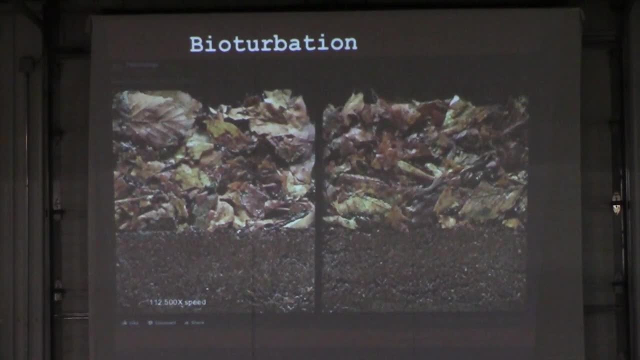 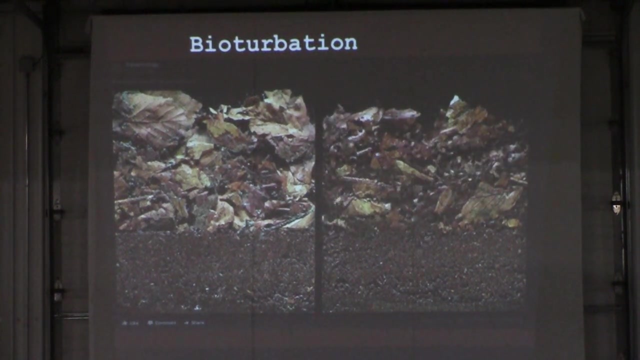 a biology problem. chemical fertilizer will not fix it. This is a picture of just fungus and bacteria. This would be common in a system that is not healthy. A good, healthy system would have this bioturbation. See, people think I have to put my lime and I have to do. 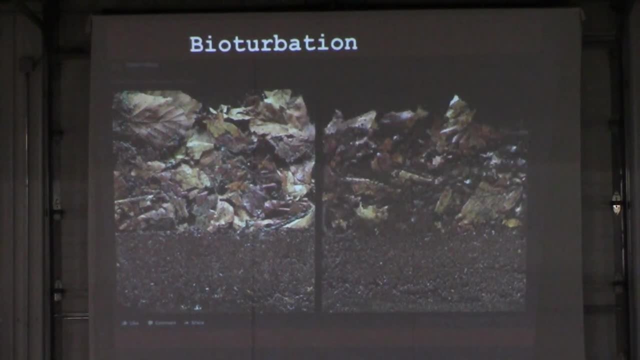 and they would blame no-till saying: well, I'm never going to get my nutrients to the bottom, How am I going to get my calcium to go? I don't worry about that. These guys will take it down with roots living. 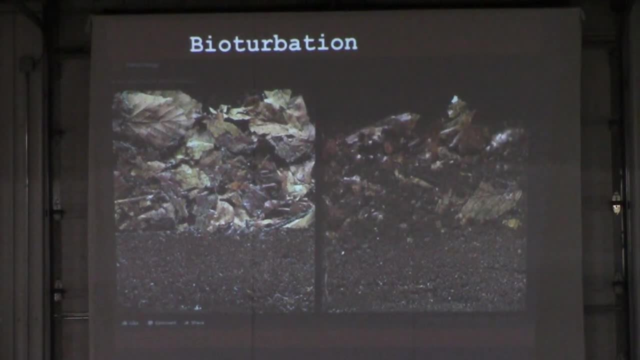 covers, The biology will move the nutrients down. The recent no-till, the old no-till studies said there's stratification. Well, there's stratification because some of our no-till systems were not healthy and functional. We promoted no-till out of 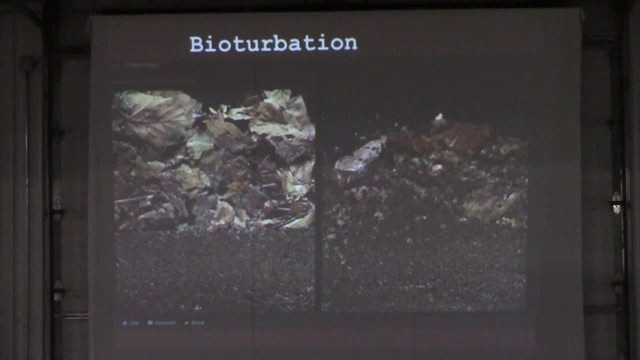 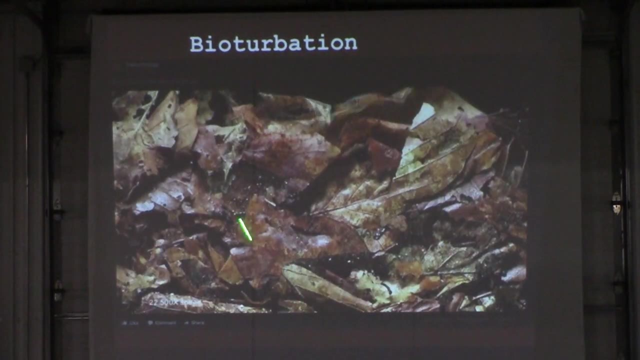 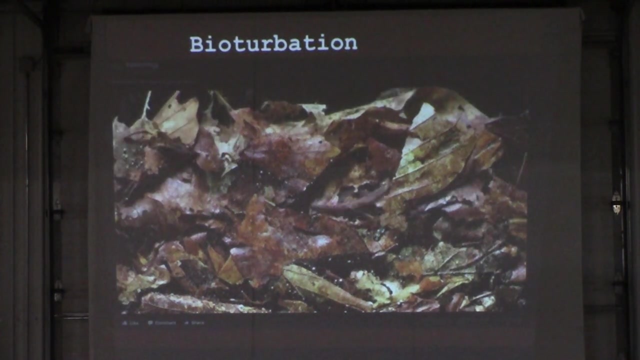 context. No-till does not work well without covers. We forgot 50% of the story. See, in an organic system where you're tilling all this, you're messing up on all that elegance, You're breaking the house down. 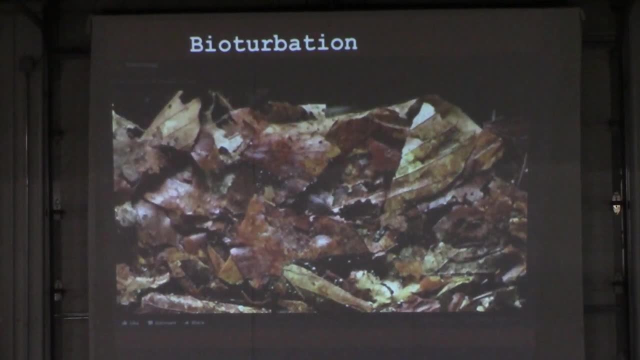 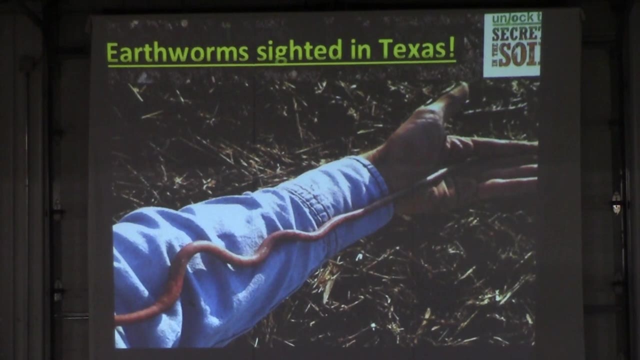 And when you spray too much, you're messing with the house, You're messing with the factory workers. We'll talk about that Now. that's an earthworm. Everything's big in Texas That is off a producer. He's a. 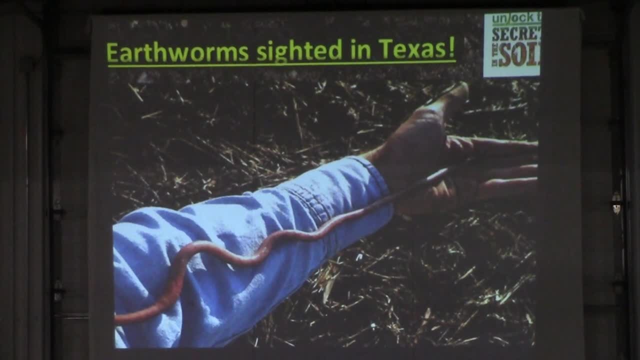 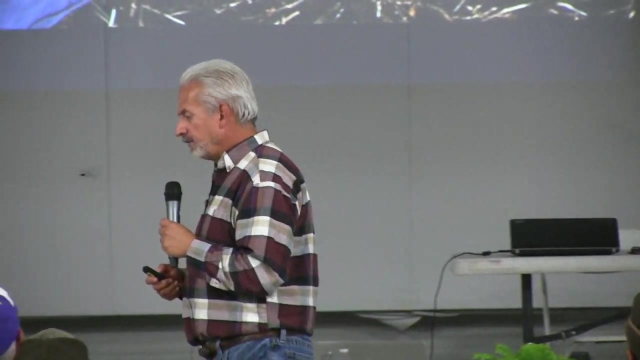 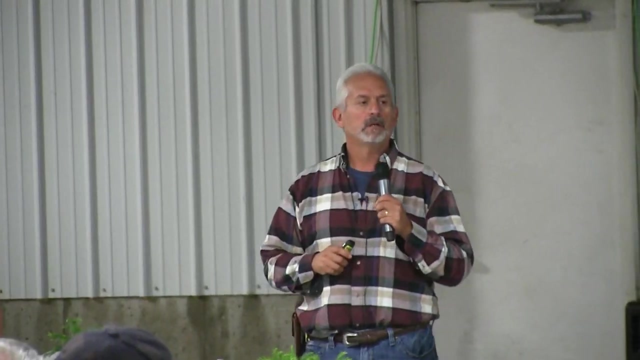 lawyer, John Regan. You heard me talk years ago. He said: Ray, I thought you were insane. I am, And I'm incredibly biased Folks. I've met one non-bias human being. He was dead. We're all. 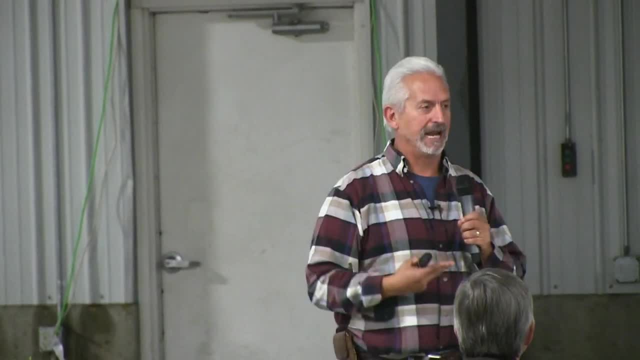 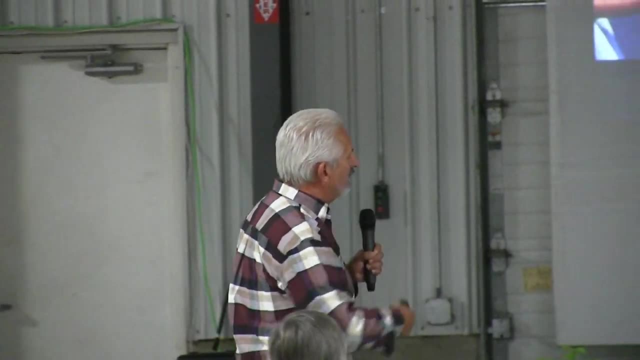 biased. I am biased towards life. now I'm biased towards biology. This man said: Ray, I did this. cover crops in this no-till and look at after five years I have earthworms. like that Man, I'd be scared to go on this place without a shotgun. 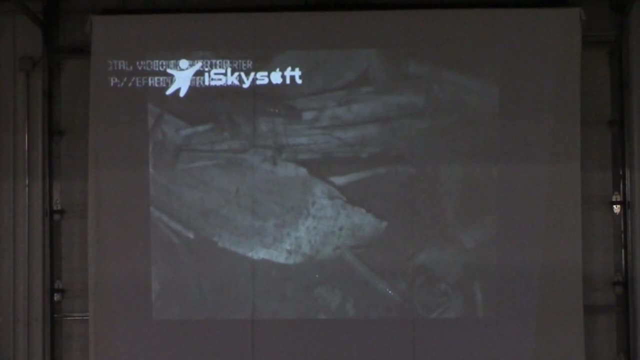 Ladies and gentlemen, this is Odette Menard's video. I was blown away. I didn't know that these earthworms are farming. I didn't know that they were getting the residue, bringing that down to the wormhole twisted it. 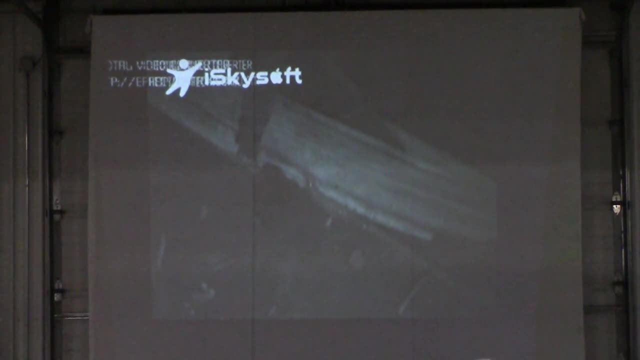 right there so that the fungus and bacteria will break down and the aggregation of biology would there and then they would consume them. This is amazing. This is a special camera at night. This is the reason I never go to my garden by myself. 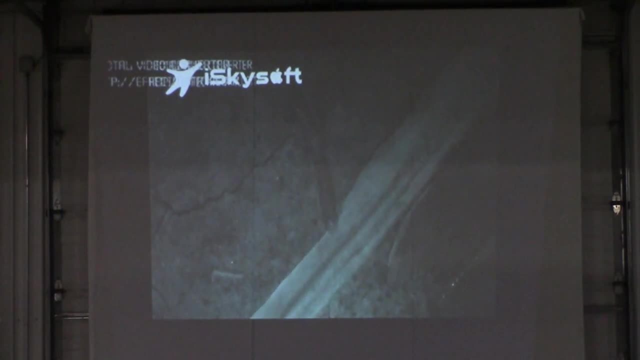 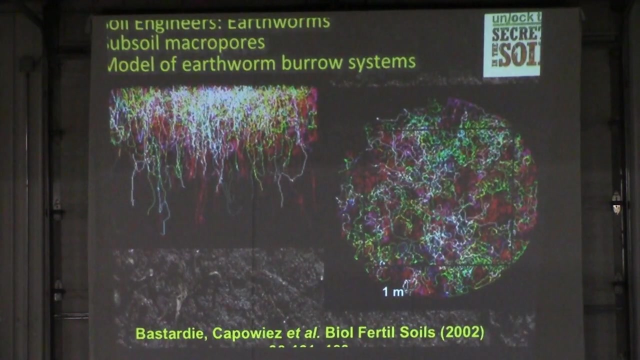 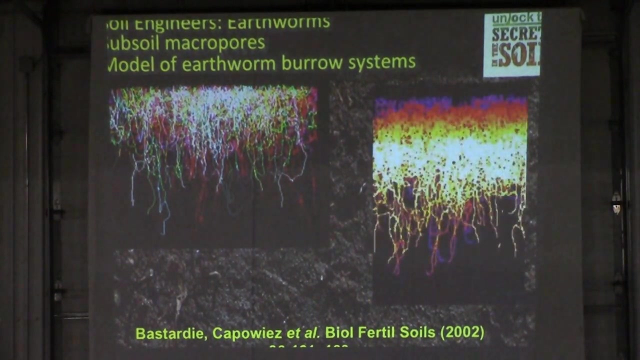 I always take somebody with me. Look at that. If you have a residue breakdown issue, you have a biology issue. They will take a forest floor down in the summer. That is a molding that they pull the special plastics or whatever they pull for the molding material. 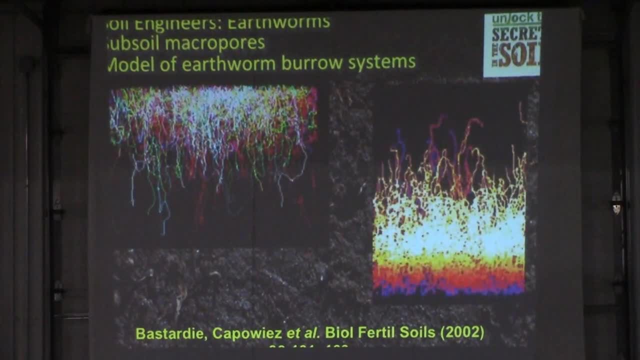 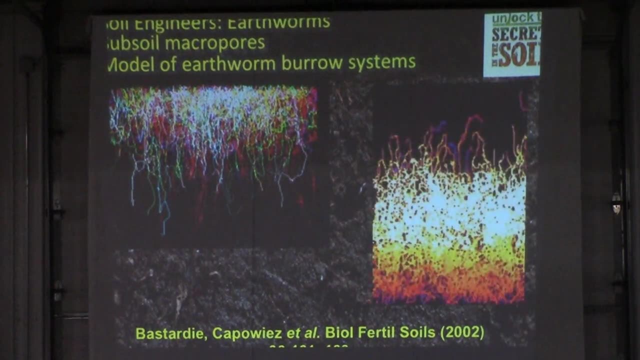 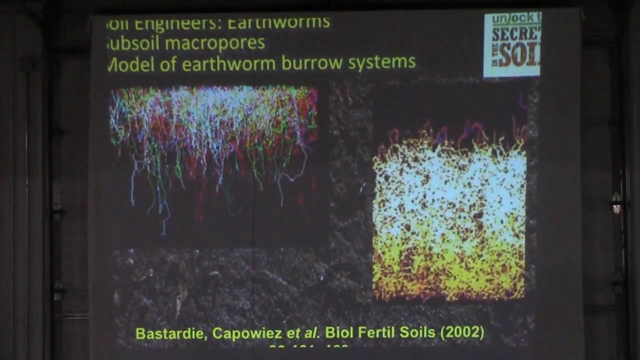 and they pour them in the wormholes. Does that impact infiltration? What if you're running a pivot and you have biology like that? It makes a huge difference Whether the water stays on the surface and evaporates or it goes in and changes the infiltration rates. 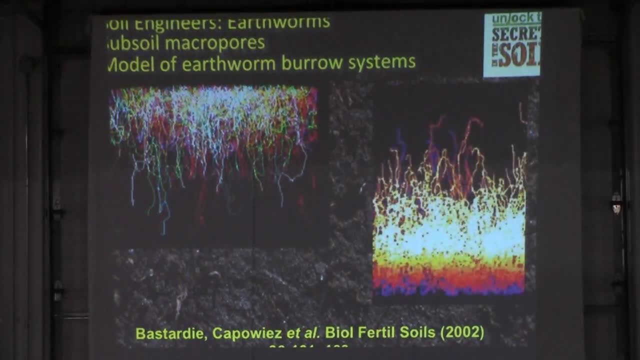 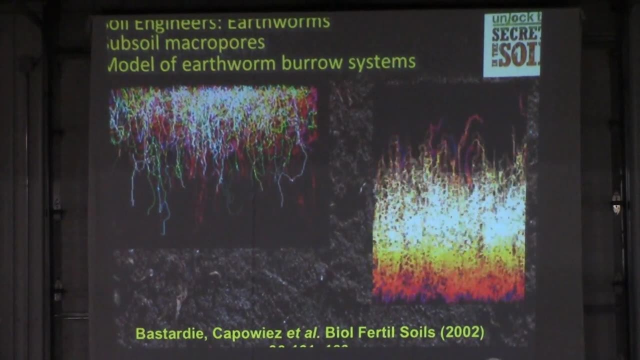 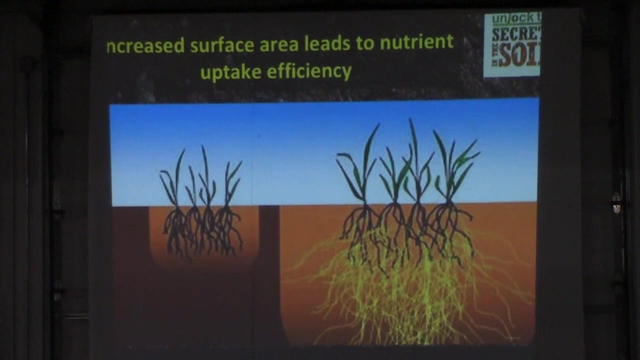 Huge difference. And then those wormholes are laced rich in bacteria and phosphorous, And then your soybean and corn go. thank you, Reduction of inputs. Let me show you what happens with the Arabisco and mycorrhizae fungus. 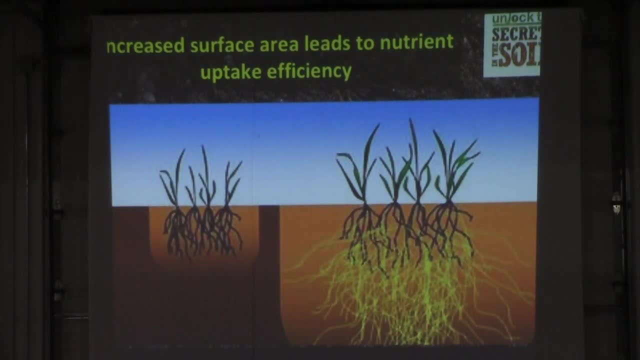 90% of terrestrial plants are Arabisco and mycorrhizae fungi. This is without the fungus. Look how much access of water and nutrients they have With this association. look what they have. This is what gets me through the drought. 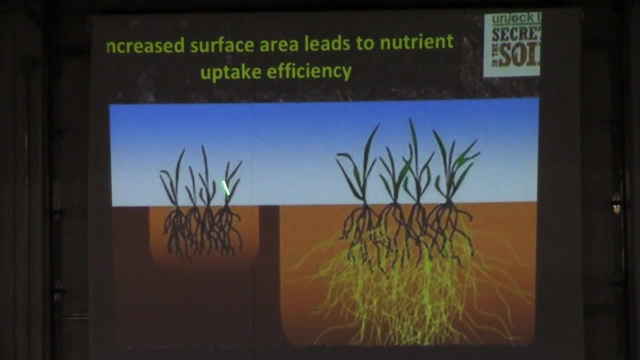 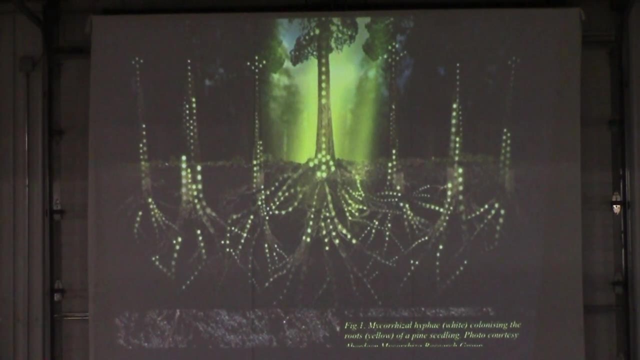 This is what brings my phosphorus, my nutrients and my organic in. It's the underground network Scientists now know in the forest that's how they communicate. They have done some radioisotope carbon and injected it on the plants and they wrap it in a plastic bag. 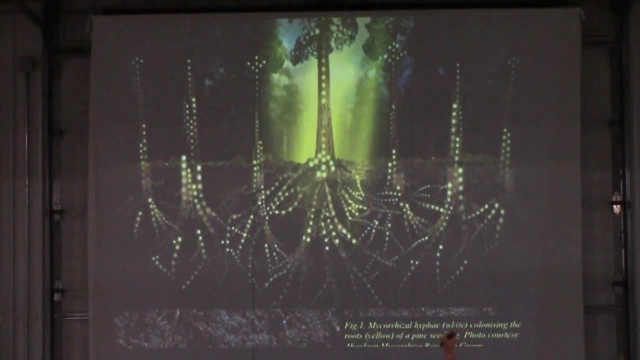 and wrap the branch and they follow the next day with the Geiger counter and they're finding it all the way down, this radioisotope carbon. and they're finding out that the big trees are feeding the baby trees. So when I put a legume out there, 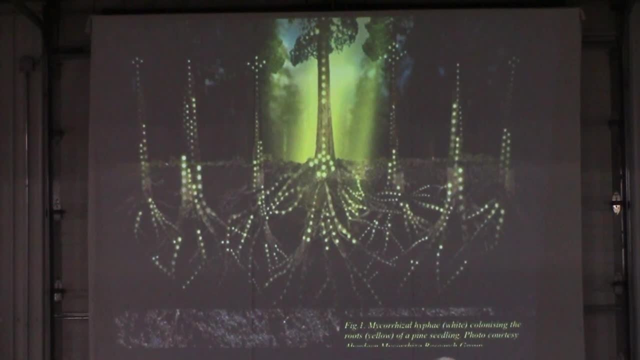 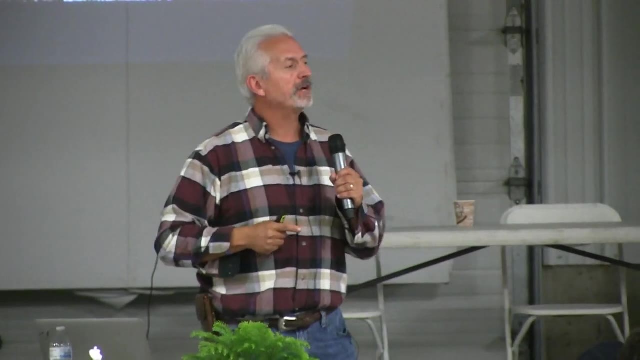 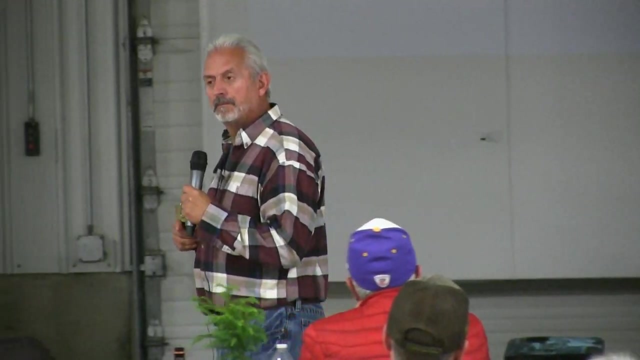 and I'm intercropping my legume right next to my corn. what do you think they're doing? They're communicating to each other, Gentlemen. this is why we have guys growing corn with less than 100 units. It's through that complex network. 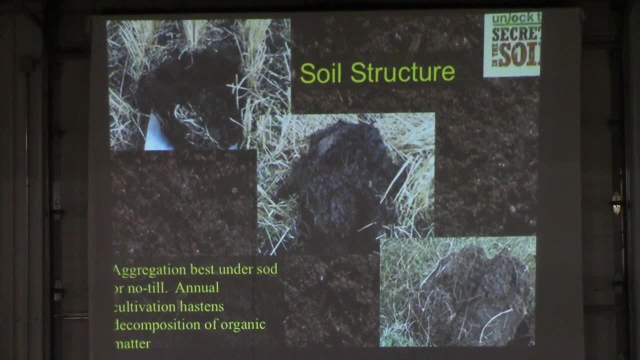 So what hurts those networks? Tillage, Fallow, Fungicides, Over application of manures. if you have over 200 pounds of pea, you shut down those spores, Insecticides, In fact, everything is connected. Everything is one. 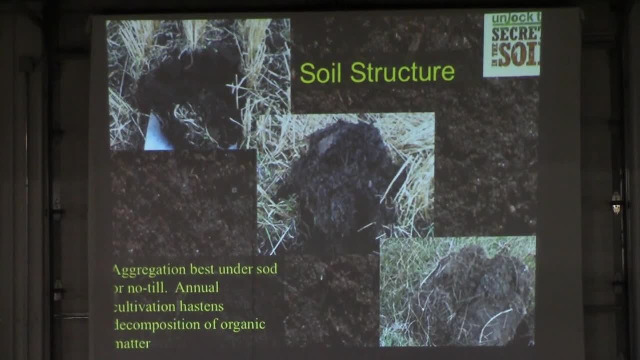 Then you affect aggregation. Fungus are critical for aggregation. So if you keep spraying copious amounts of fungicide, you hurt the system. Then you have issues with phosphorus take up. Now. did you hear me say not to use these tools? 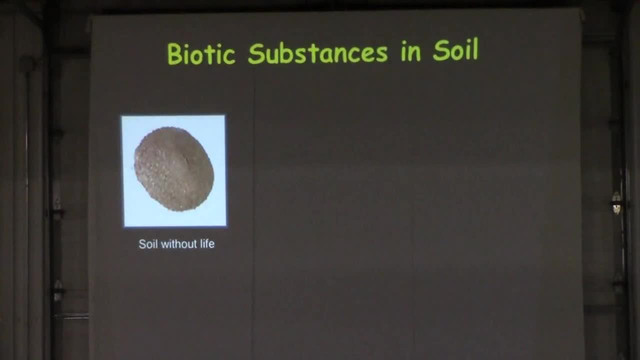 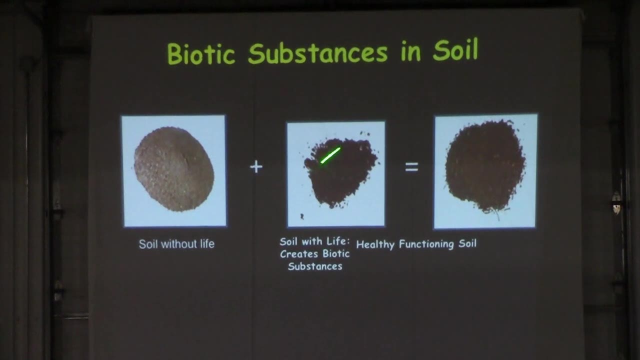 Didn't say that at all. Let me show you how we're going to manage our disturbances: Geology, Life, The secretions of life, Coding. Now you have soil, The fungus, The bacteria, All of them working in synchrony. 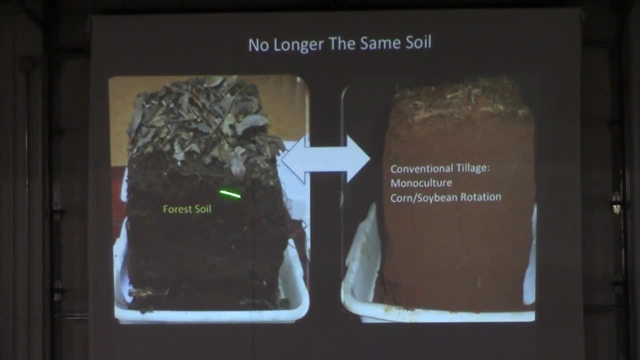 in collaboration Create those biotic substances. That's not one time Monoculture Tillage, Corn, soybean rotation, We took it from here to here And in our country we have a spectrum from there to here. Does it infect? 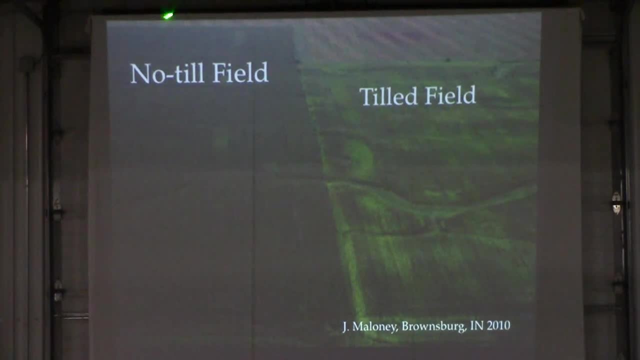 our nutrients, how we hold them. It sure does Once you start putting covers. This is a tilled field. Notice, you cannot see it, but from the sky, The integrity of these soils, The aggregates, These aggregates, These super molecules help hold calcium and hold. 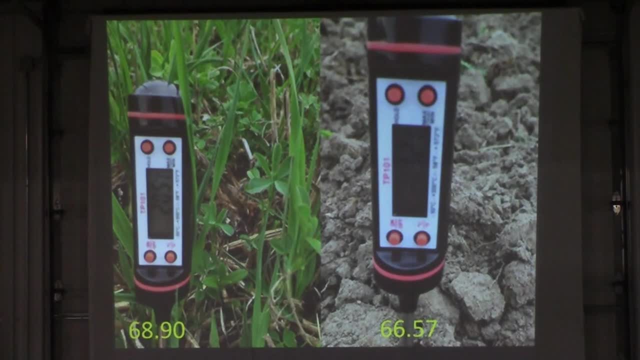 the nutrients in place. Also, when you use covers, the soil temperature is warmer, Not colder. I read a book by Dr Geicher. He went all over the world, Brilliant scientist. He called it temperature of the soil. He said he went everywhere. 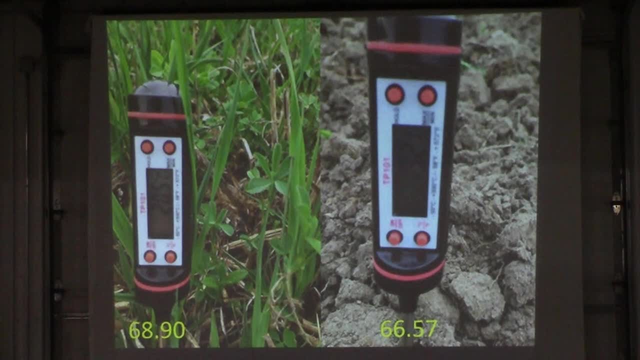 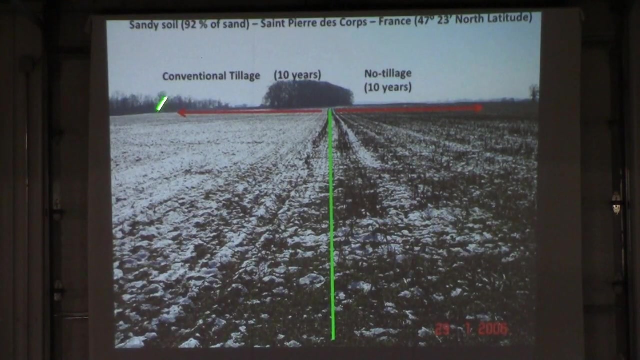 And he said: the best way to regulate temperature and moisture is what Living plant? I just saved you 400 pages. Look at here. This is a conventional tilled soil. This is a no tilled soil- Sandy soil in France. Why does this one have less snow? 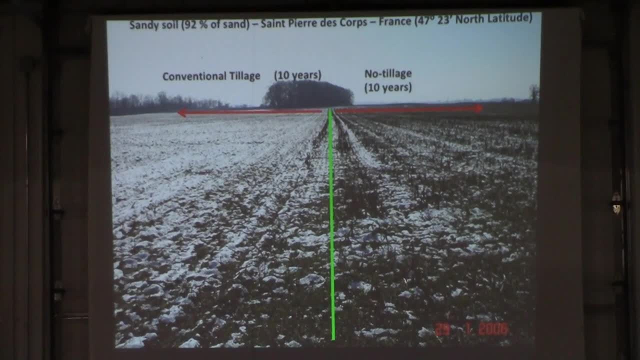 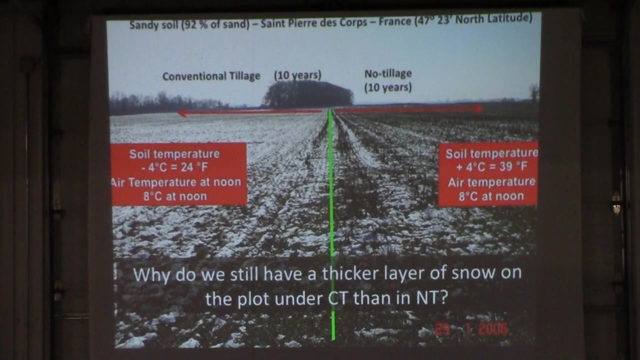 Class Why It just snowed on one side of the line Right. I've had farmers say that all the time. Microbes, The temperatures here, The respiring microbial biomass is huge. Five minutes, Oh, I'm in trouble. 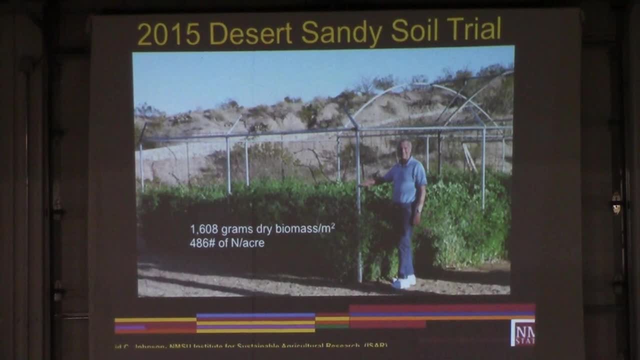 Okay, Let's go here. This is very powerful. This just came off the press. This is Dr David Johnson. Oh, Okay, Okay, Thank you. I've been watching Kenny and I'm making sure I'm in time. I get too excited about this because it's just. 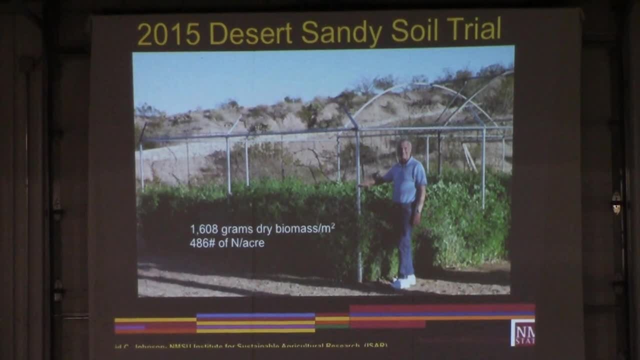 like a starving dog in a meat house. Just go crazy. Dr David Johnson came out with some recent research. I think it's awesome when a guy at 50 years old goes back and gets his PhD and graduates at 60 years old. 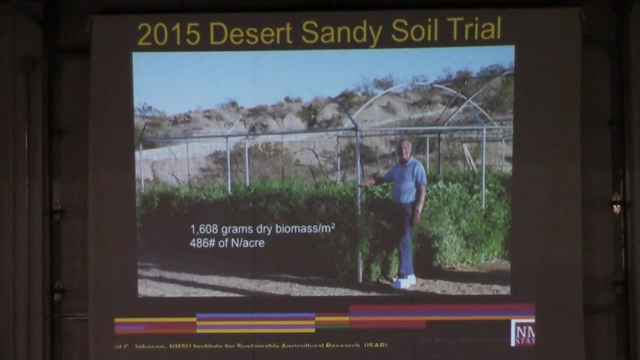 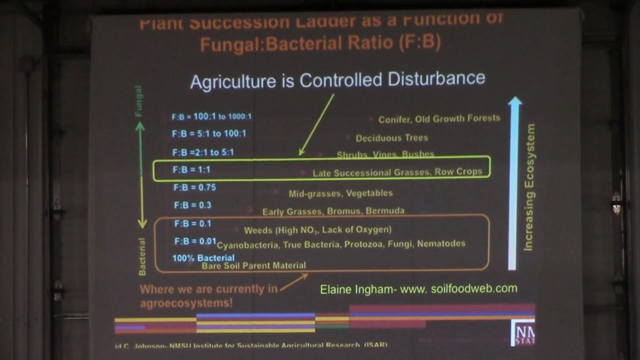 Awesome. Some of the best scientists or the older scientists, It's just amazing. Let me show you what he came up with. We're going to show you. I'll pass this slide here out of place. Okay, His research has shown in the: 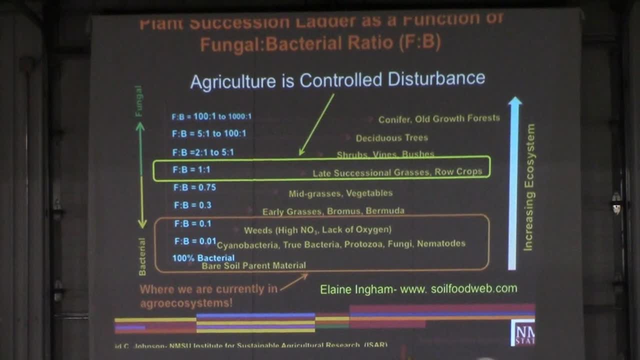 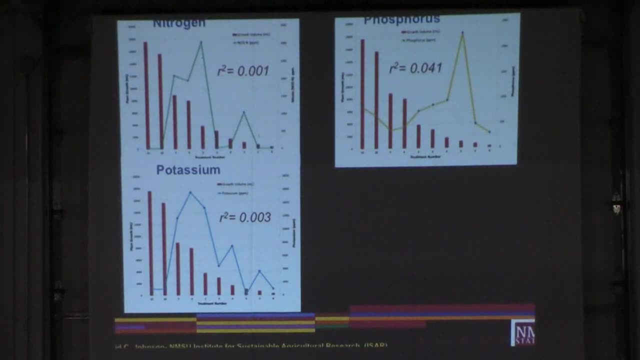 early stages of plant growth. it is not nitrogen, it is not phosphorus, it's not potassium, that actually even organic matter that makes a difference in plant health in the early stages. I'll say it again: It's not nitrogen, It's not phosphorus. 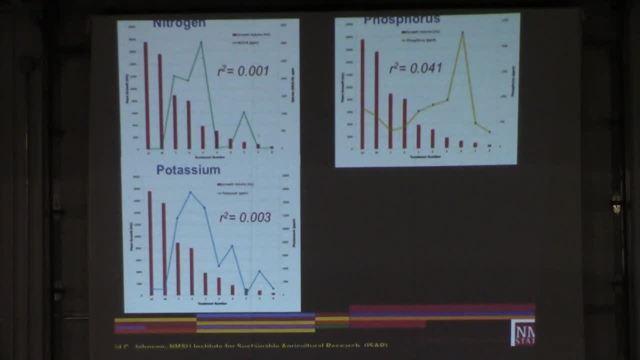 It's not potassium, It's not organic matter. I'll give you an example here: The organic matter slide is missing. This is a anybody that has a little bit of science background: an R square of 0.01.. How many know? 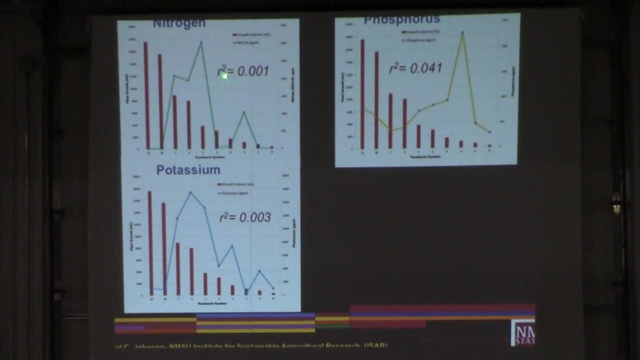 a little bit of stat. Raise your hand. I like to see a 0.6 or 0.7 to show not causality, but there's something there. Nitrogen had nothing to do with plant growth in the early stages, Neither did potassium. 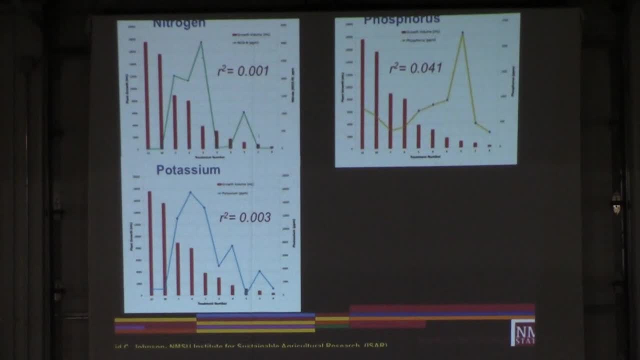 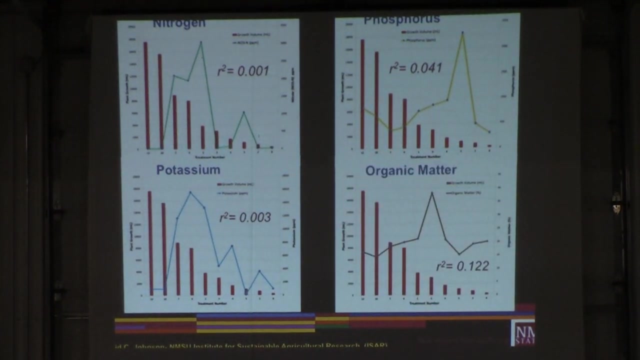 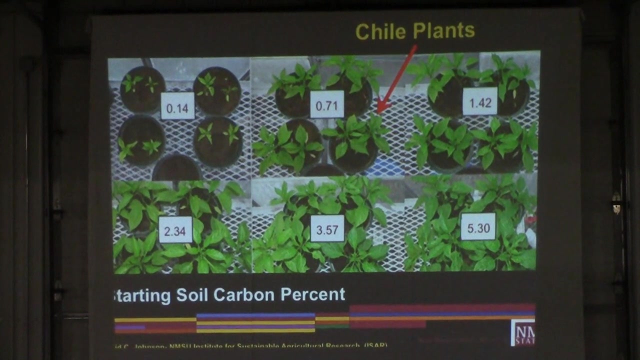 Neither did phosphorus, Neither did organic matter. What really made the difference? Anybody have a guess. Moisture, Not in the early stages. There's the organic matter. Temperature: It was fungus to bacteria ratios. It is more critical in the early. 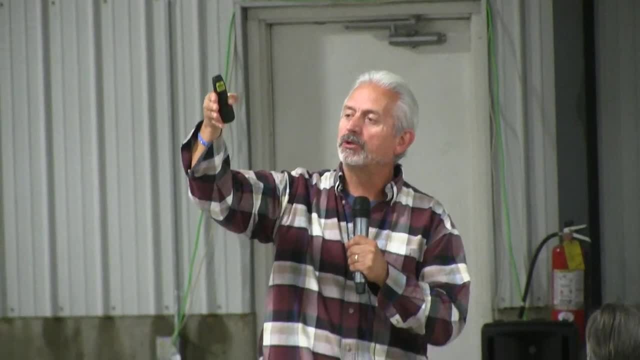 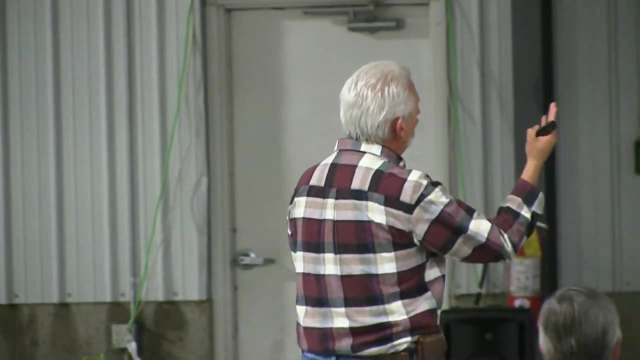 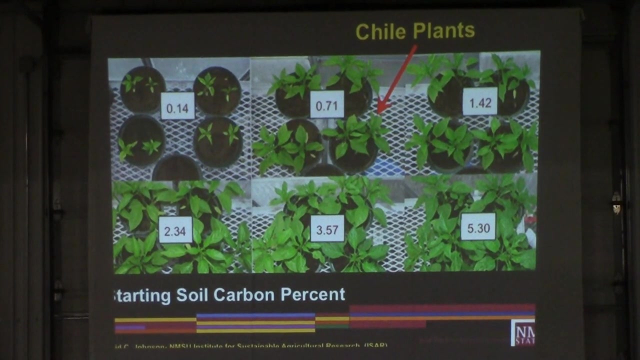 stages that fungus and bacteria ratios are right for plants to do well health-wise. Why do you think that is, Matt? Why is the fungus to bacteria ratios? Look at the heavy bacteria: More fungus. the chili plants did better Replicated research. 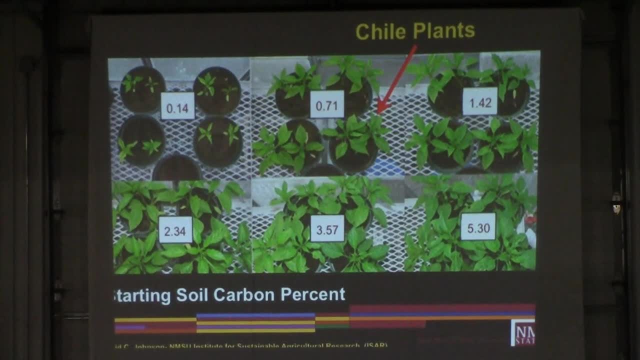 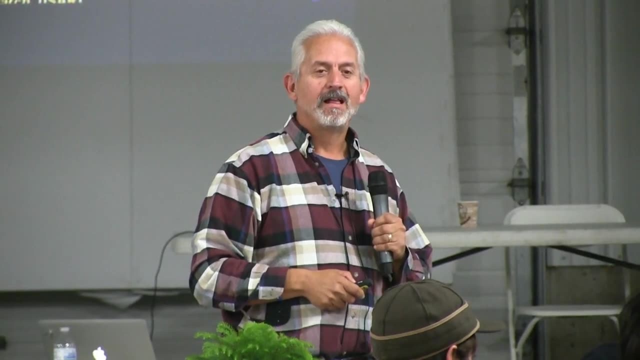 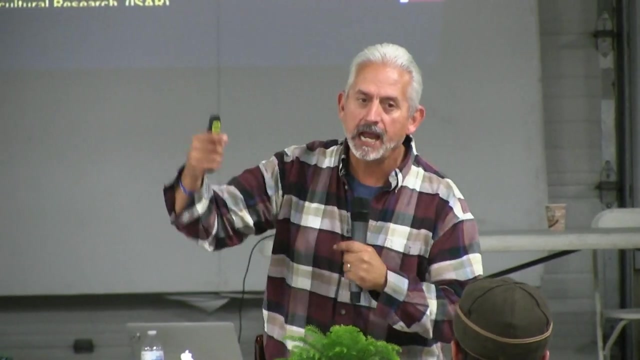 Once you think about it, it makes sense. What do you think? What do you think? See, if you don't have the association with the fungus and bacteria, you cannot get the access to the nitrogen, You can't get access to the phosphorus and the potassium and the organic. 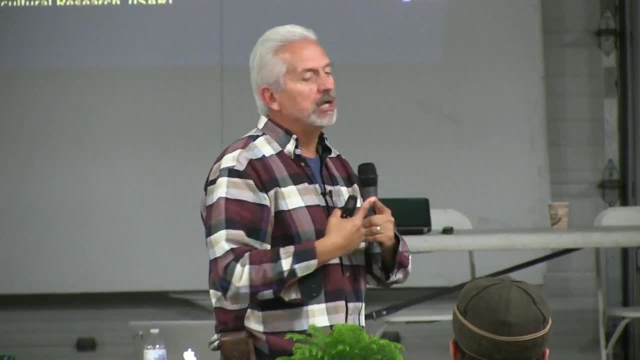 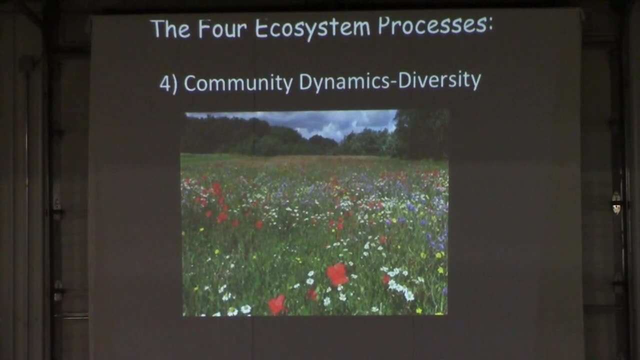 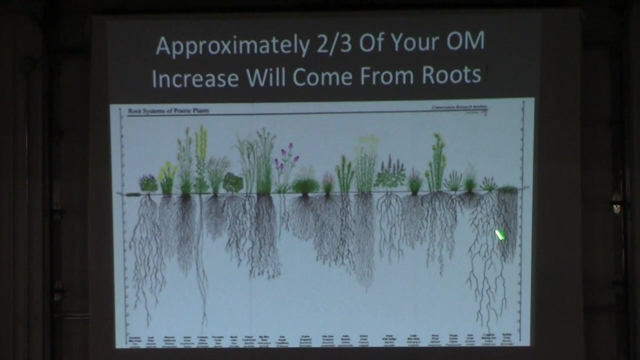 matter That association of biology is critical. Okay, Diversity, This is what we're doing. Diversity runs that engine. We need more diversity in our operation, Rotational diversity and cover crop diversity. We are designing our mixes to look this way. 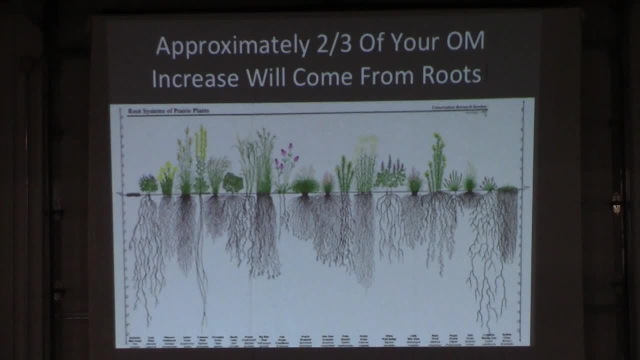 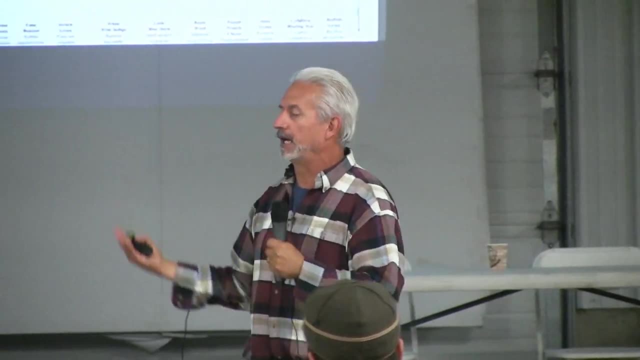 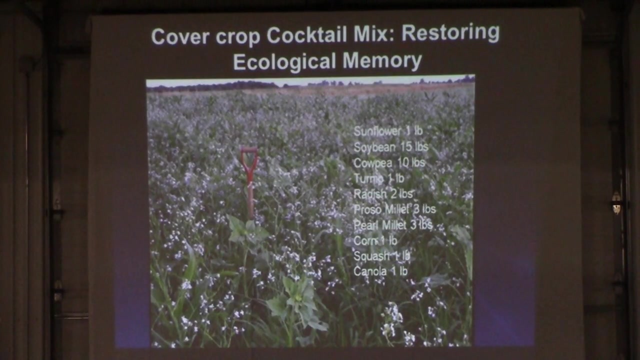 I want the architecture on top, I want the architecture on the bottom. That's why prairies have hundreds of species. That's why we are designing our cover crop mixes to look like the prairie or the forest. We are designing mixes all over the country that. 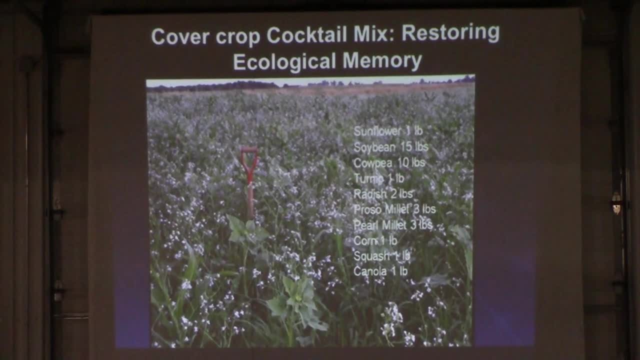 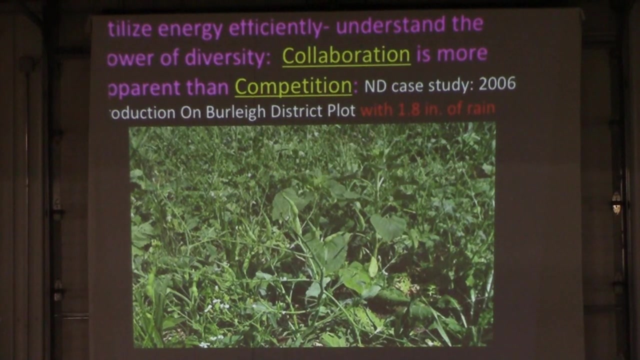 look like that. So after corn, after soybean, after wheat, we have a multi-species mixes, feeding biology. Let me show you how powerful those mixes are. It was in 2006 in North Dakota where we learned the power of diversity. 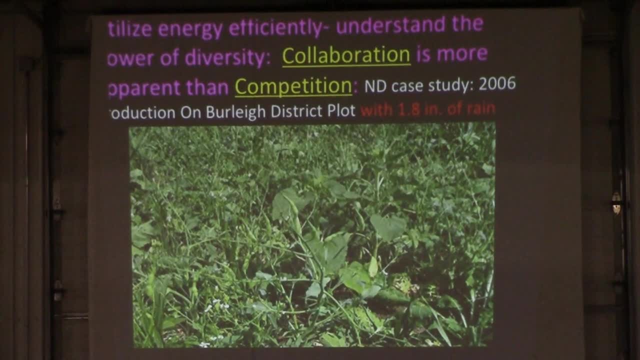 That's why I started throwing some of my books when I went to graduate school and threw it out. about competition: See, I'm saying nature is more collaborative than she is competitive. Does competition happen? Yes, But is it the overarching principle of the natural system? 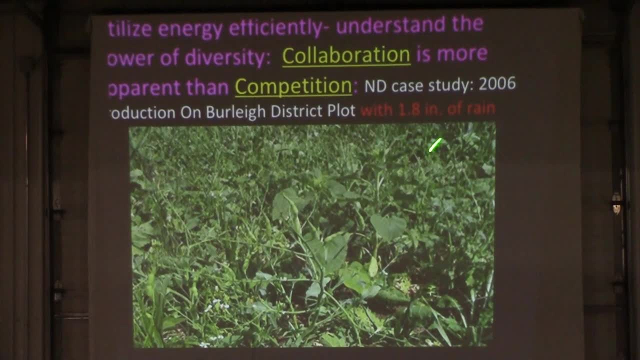 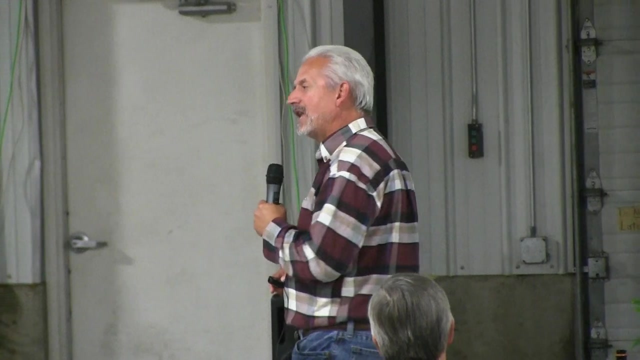 No, Let me give an example: 1.8 inches of rain. These are test plots that were 1.8 inches Give you perspective of North Dakota. They got about 100 and some days They have 230, some days frost days. Very short growing season. They get up to 100 inches of snow. It blows. How many of you have been to North Dakota? It's pretty brutal there. I am a warm season cover crop. I would win or kill there 16 inches of. 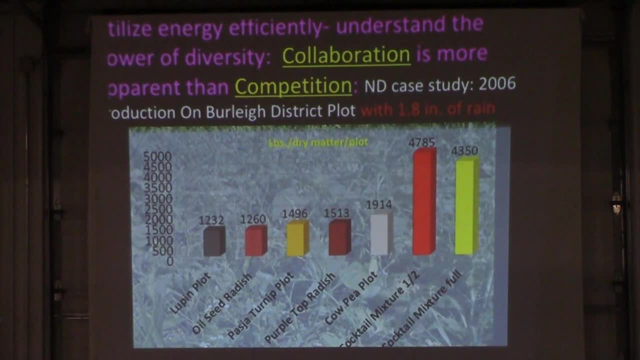 rain typical. Let me show you what these farmers and ranchers did in the district in NRCS DC. They planted some plots. They planted in this plot lupine, oilseed, pasha, purple, cowpea, cocktail boom. And in this: 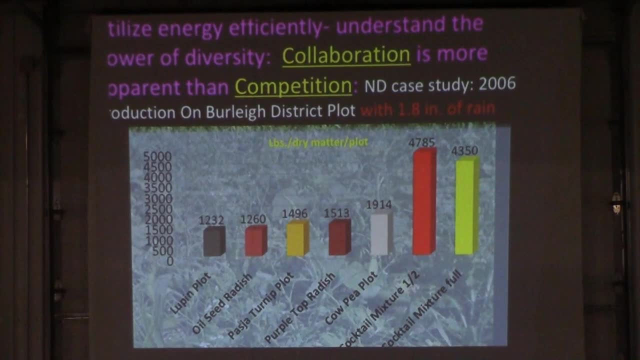 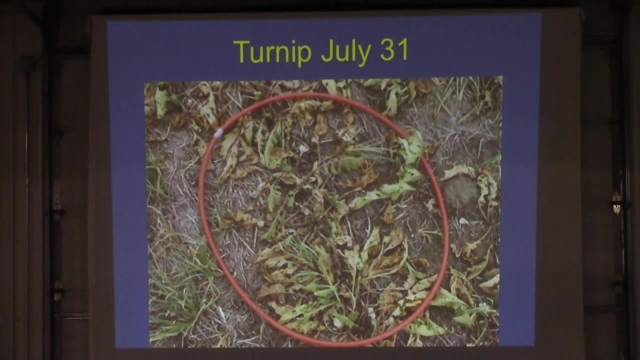 last plot. they took all these seeds and threw them into this plot. Remember, this whole plot only got 1.8 inches of rain. Let me show you how it looked. I would expect that with 1.8 inches of rain. 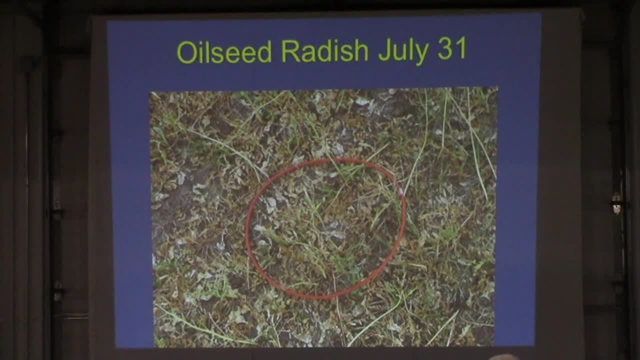 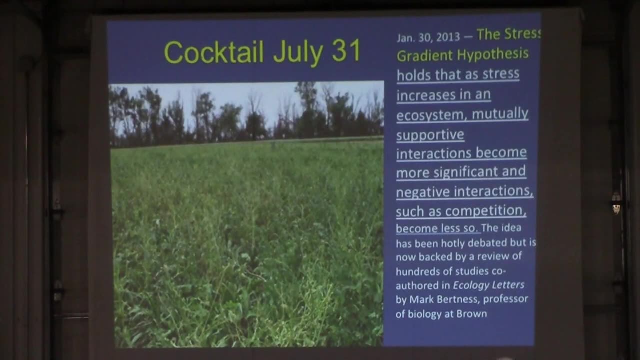 Death. Look at the other monoculture oilseed. But look what happened the moment they threw all the seeds together. You can see the brown plots right there. How did that happen? Oh, it's only North Dakota. God loves North Dakota. 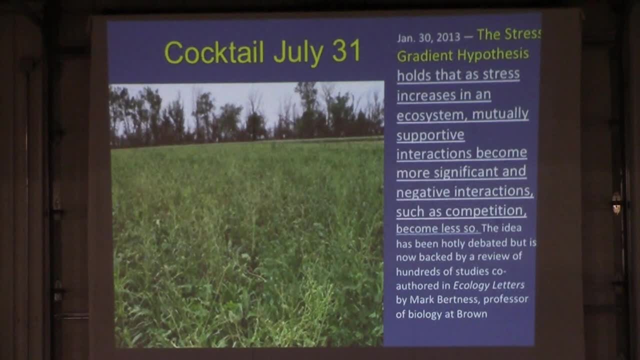 You know how many times I go all over the country and the first thing they say is: Ray, you don't understand our climate, You don't understand our soils. Oh, so biology stops in Minnesota State line. Is this Mars? Write this down. The stress gradient. 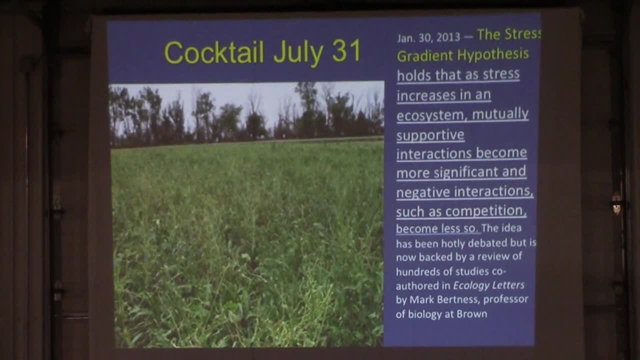 hypothesis by Dr Brown. He says in natural ecosystems, as the natural system becomes more stressed, it does not compete, It collaborates. It's a meta-analysis of all the research. Mark Burton says you can get that in ecological letters. We saw that in life. 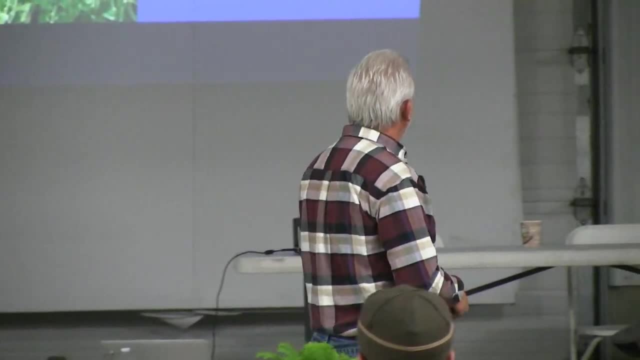 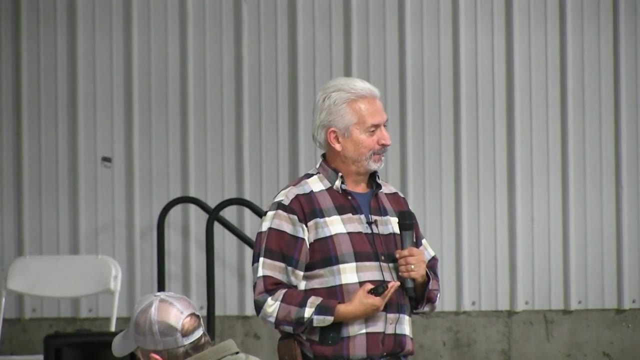 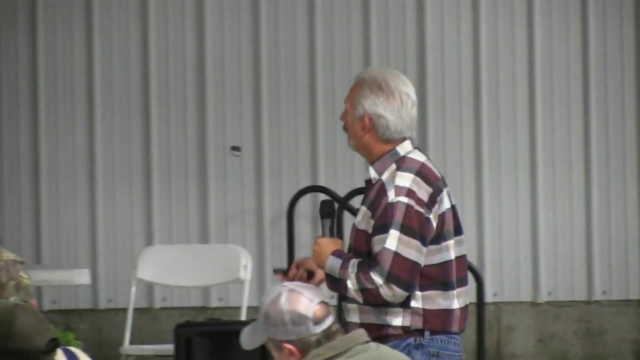 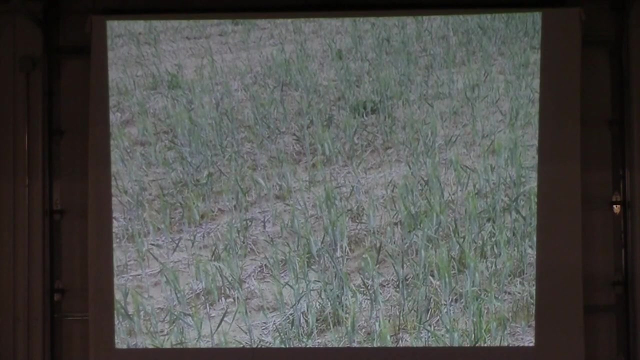 Everybody got that down. It's called the stress gradient hypothesis. When nature gets stressed, it collaborates. Pretty darn cool Wheat science book, But it only happens in North Dakota. Let me show you: Canada Grass Multi-species mix. 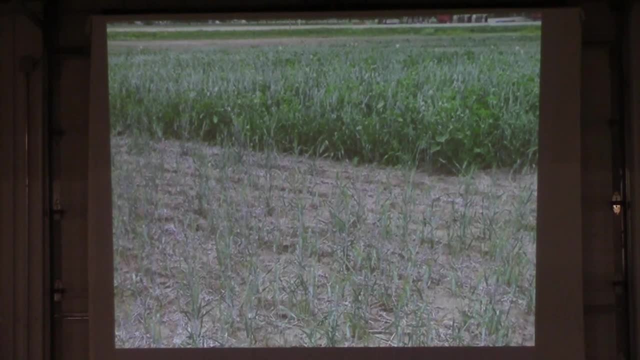 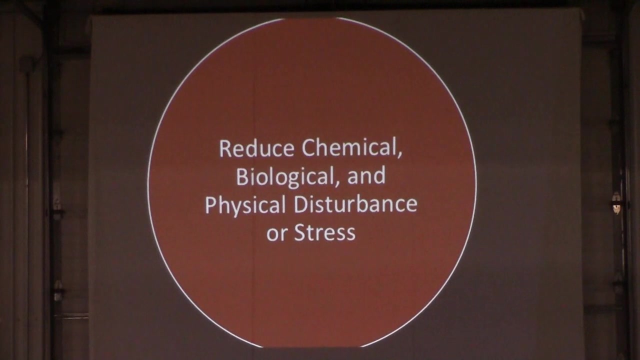 Side by side, Oh, but Canada. It is happening everywhere. ladies and gentlemen, The power and synergy of biology, That is so darn cool. Now, how do we reduce this One of the principles? How do we reduce the stress? How do we? 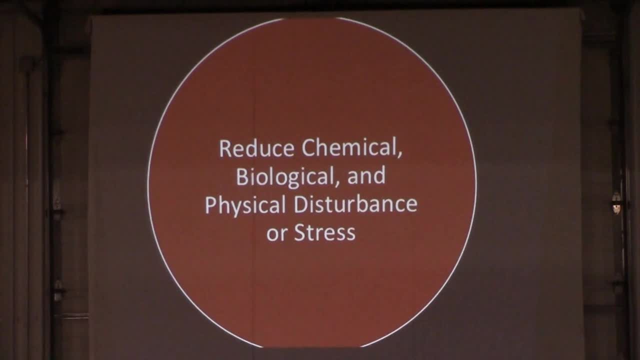 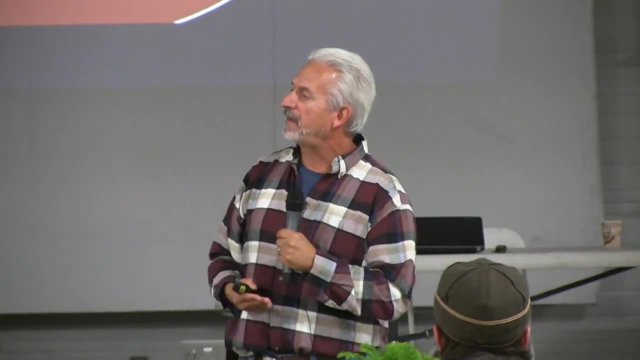 reduce the stresses in our system, Because I'm telling you, if you do not get a grip on this, I don't care how much cover crops you do, I don't care how much diversity you do, you are never going to get past first base. 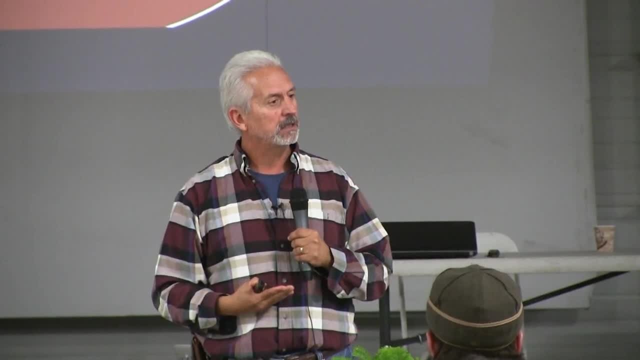 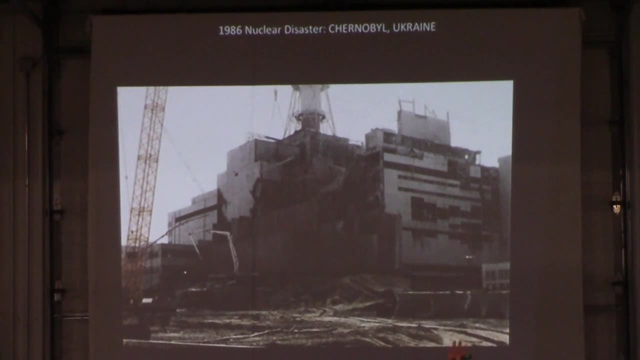 You got to manage your chemical and physical and biological stresses. Let me give you perspective. How many were born before 86? Raise your hand. Do you remember Chernobyl? Do you guys remember All of us? I remember that, Remember. 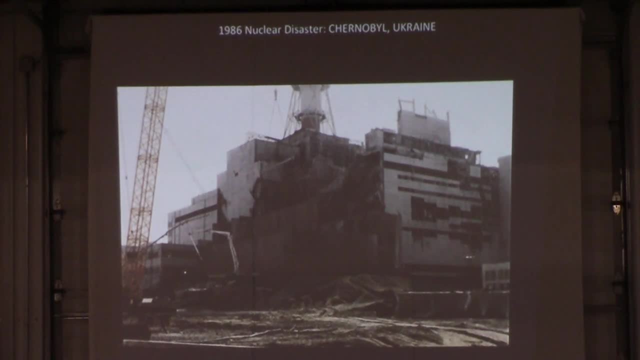 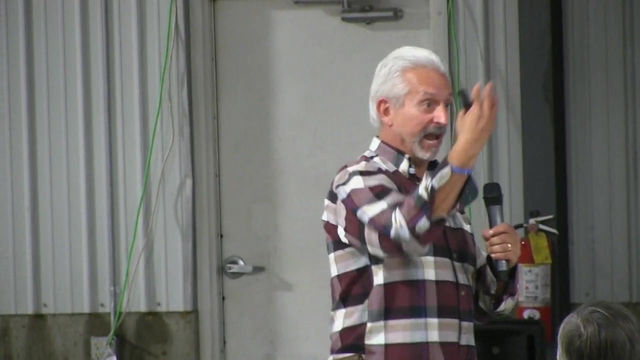 I was not very old And when that happened, they said that we were going to have a disaster. There was going to be death. Nobody was ever going to live in that place, ever. The scientists said this was the biggest disaster. Is that what you? 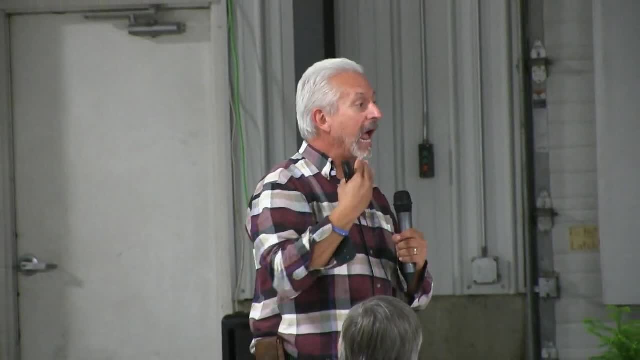 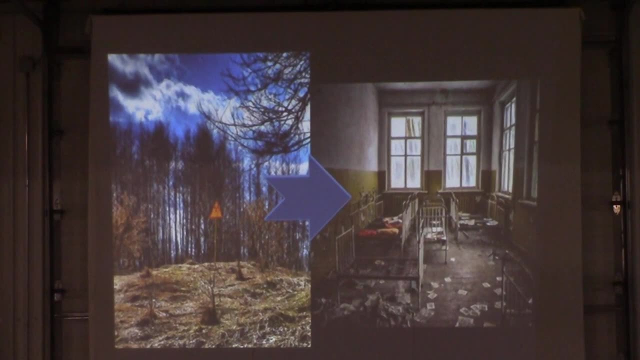 learned guys? You remember that? Oh yeah, We remember in the news. it was like whoa In fact: eight kilometers death. This radioactive material got everywhere Toxic. They had to clear cities. It was a disaster. Thousands of people. 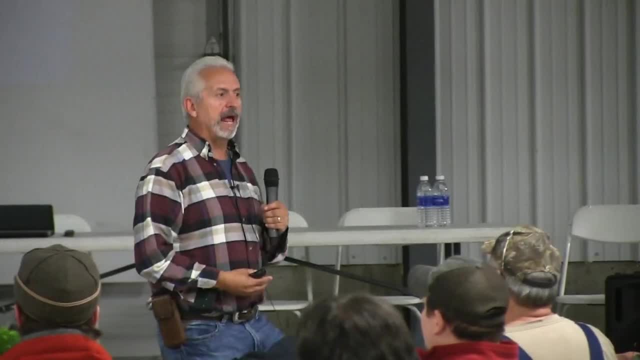 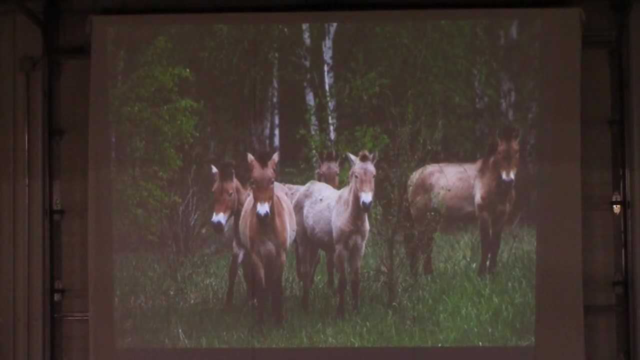 lost their lives, Got cancer and died. Do you remember that? Look at it now. How did that happen? How could this should be a movement landscape? There should be nothing but death out there. Do you know why it's recovering? Exactly, You beat me. 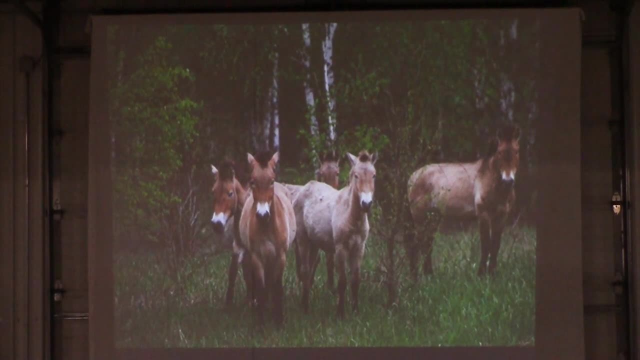 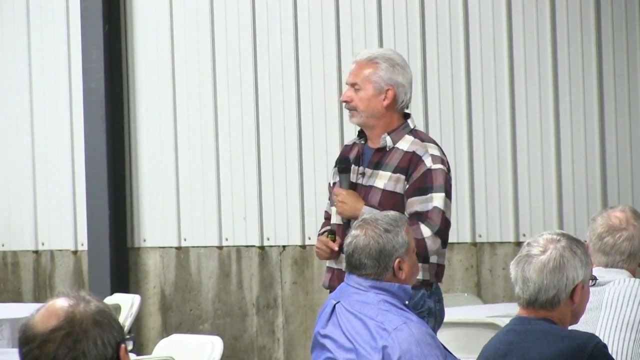 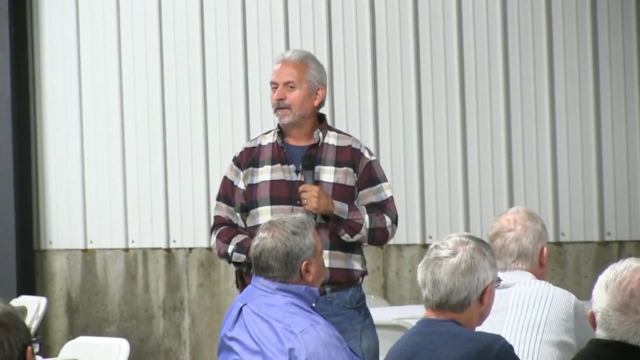 to the punchline. There is no man there. We have more possibility of healing Chernobyl than our typical agriculture field, See, because it gets recovery time. It gets rest. See, we're continually spraying fungicides and insecticides and chemicals. 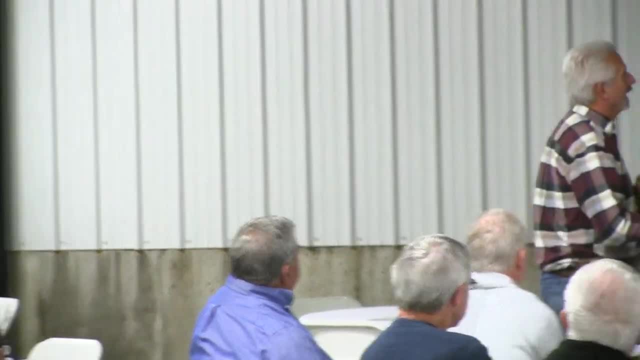 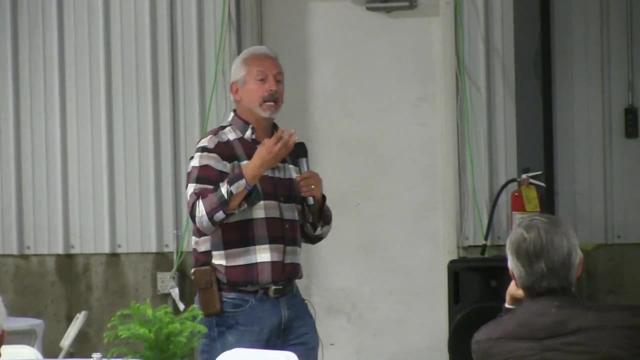 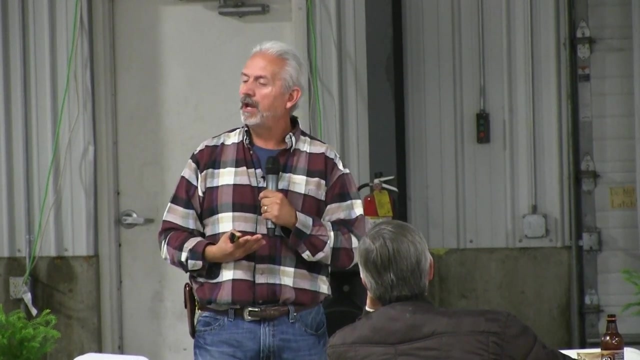 and we're saying that's okay. Yeah, And see, the neat thing is these other predators are kicking in. They were shocked. Scientists were shocked that there wasn't as much mutation as they thought. They thought death was going to prevail. The reason I show you guys is: 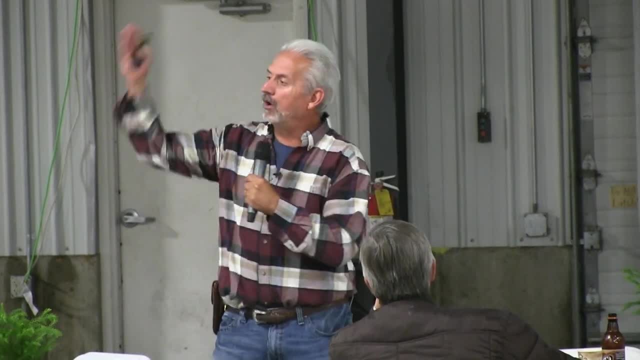 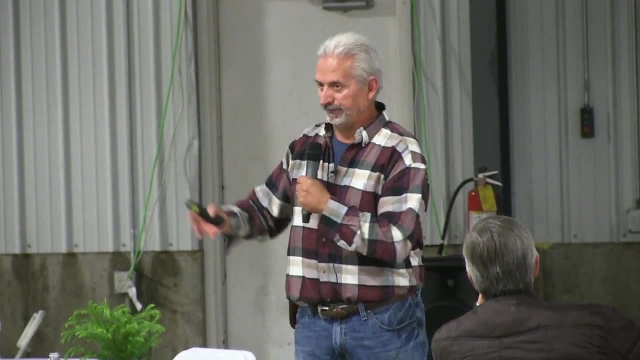 learn how to manage your stresses, because there's camps of saying, oh, we can't use glyphosate, And there's camps of tillage. I'm in the camp of facilitate life and careful with your disturbances. Let me show you This is. 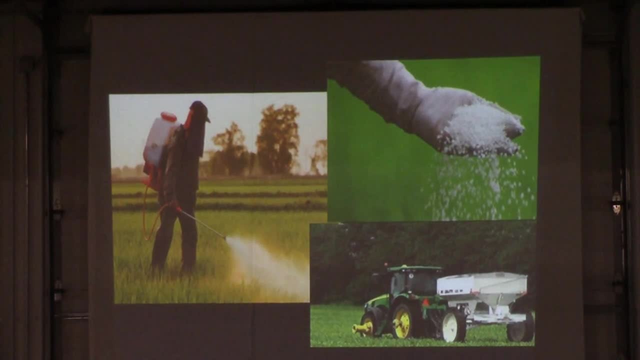 a salt. Now, let me give one of you guys a bath in salt. What would happen to you? Ha, You would die, Unless you eat a huge amount of salt. Let me spray you. This is what I'm saying is, and not one time. 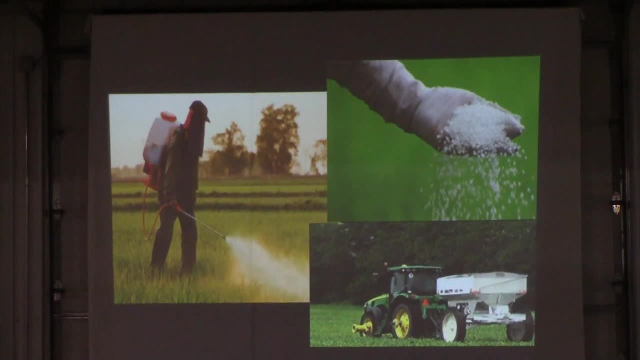 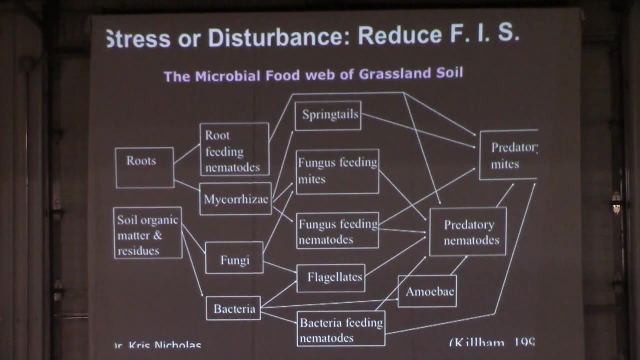 did you hear me in my presentation not say to use these tools? Use them with incredible wisdom? Let me show you what I'm talking about. This is a food web of a prairie system. If you impact the mycorrhizae, you impact this organism. 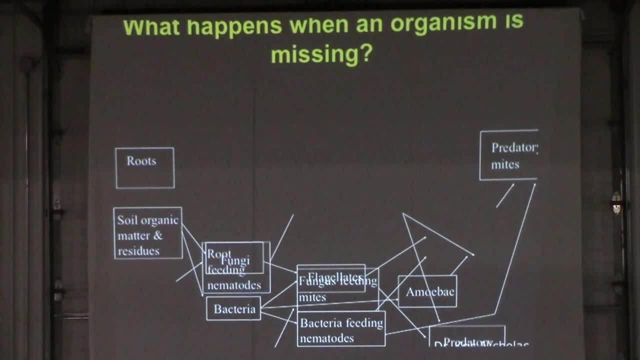 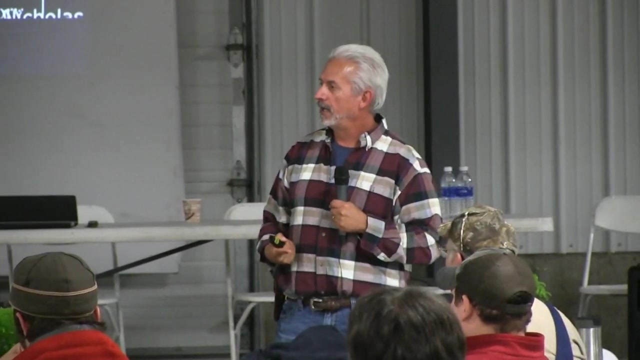 this organism, all organisms, others, you impact the whole system. the system collapses. What I'm saying to you, everything's connected, Quantum physics, all is one Theology, all is one Ecology, all is one. Do not think you don't have. 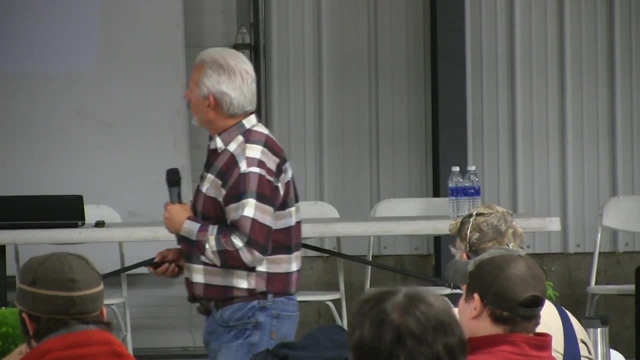 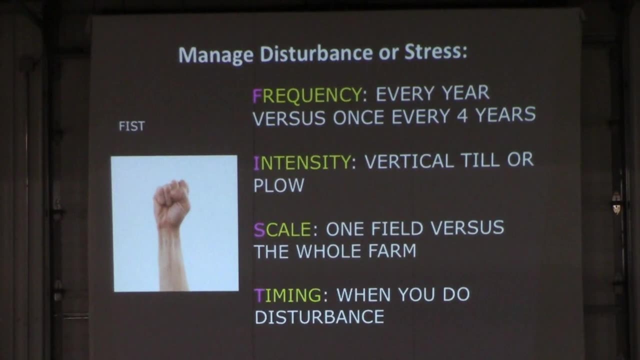 unintended consequences when you go out there and do something. This is my acronym I use for managing disturbance: FIST. The reason I put a fist is because this is what we've been doing to nature. We're going to force you. Here's what I tell you about. 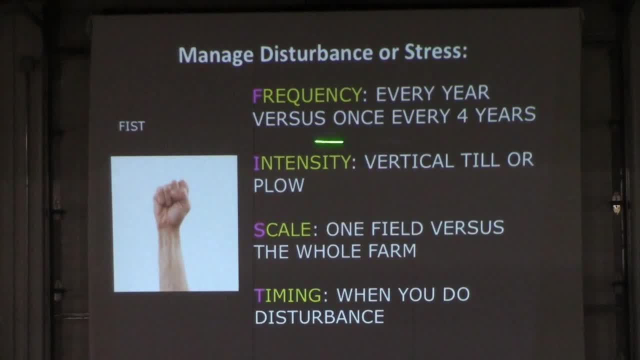 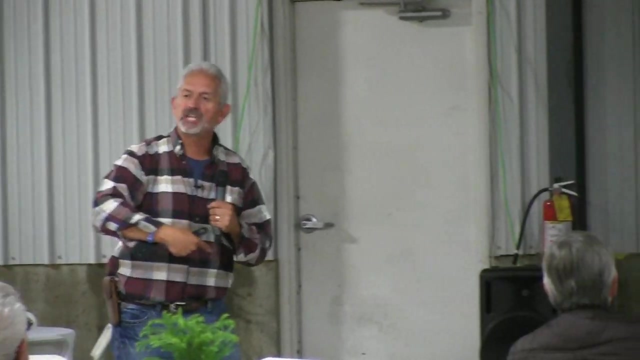 disturbances of physical, chemical and biological. Watch the frequency of your disturbance. The more frequent you distill, the more frequent you spray chemicals, the more you hurt the system. Please understand the difference between chronic stress and acute stress Every one of us were designed to handle. stress. You cannot handle chronic stress, but you can handle an acute stress If you lift weights and you build muscle. that's a stressor. You need it. Our bodies are designed that way, But it was not designed to handle chronic stress. Chronic stress is when you keep eating bad food, never sleep, eat and continue eating poorly. you will get sick. Same thing with natural systems. Understand the differences between the stressors. Can the system handle an occasional tillage? Yes, it can. 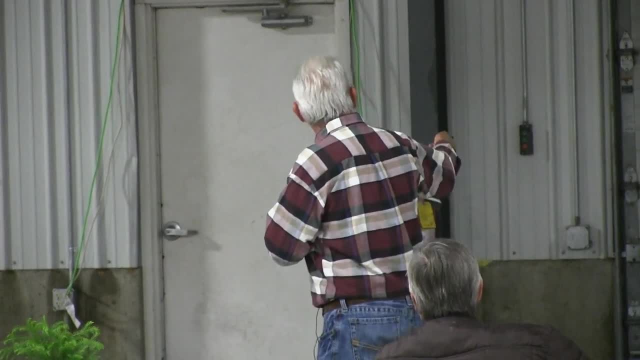 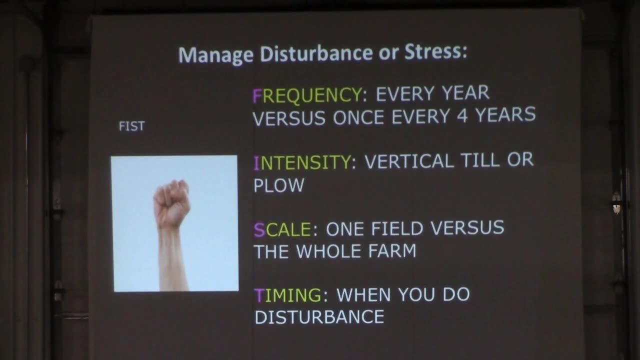 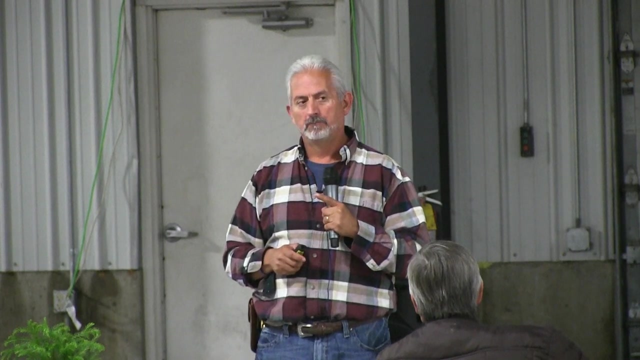 But it also deals with the intensity of it, the scale of it and the timing of it. How about an occasional roundup? It can handle it, But not all the time. The problem is that we spray it like water and they've lost it. It's just a. 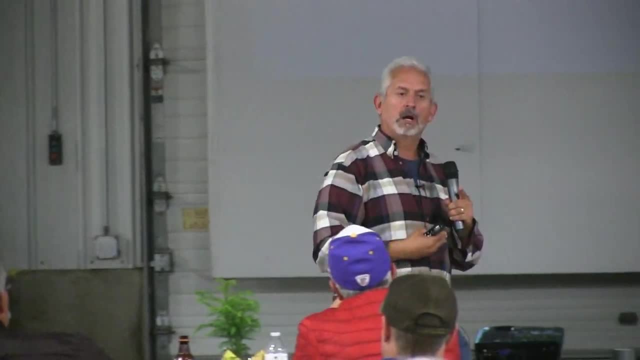 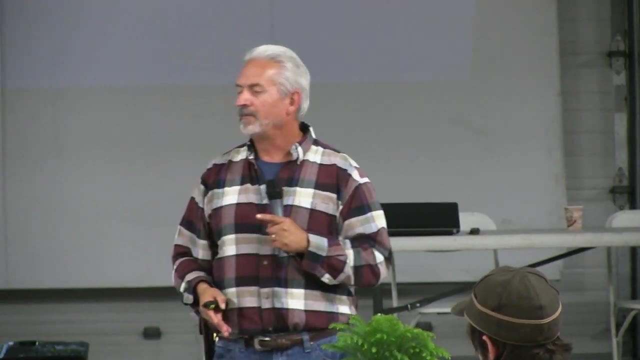 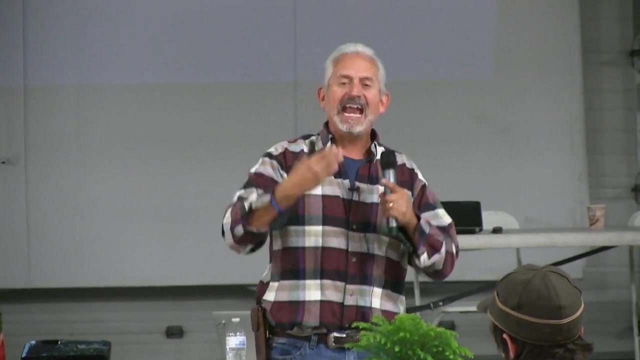 matter of time. You heard the two speakers before. It will mutate, It will change. That's why I love the concept of agroecology. Agroecology is the bridge between conventional to organic. My goal is: I don't want the producer to do any of. 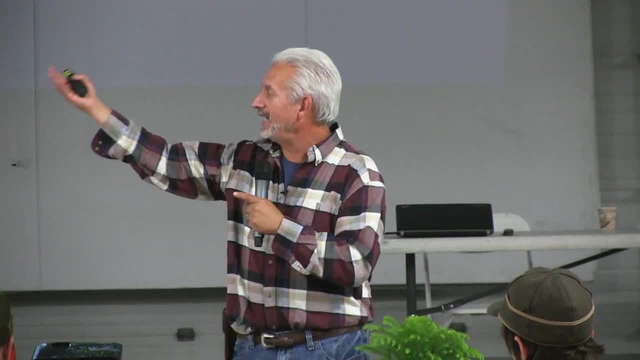 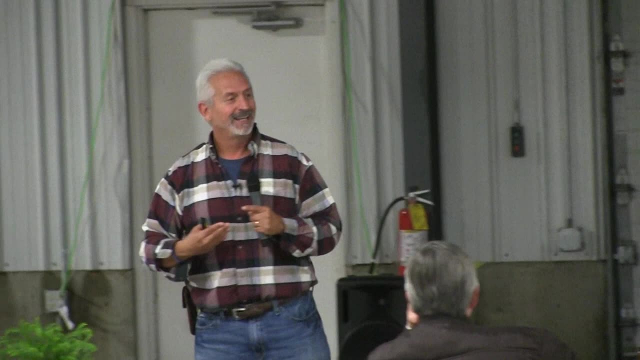 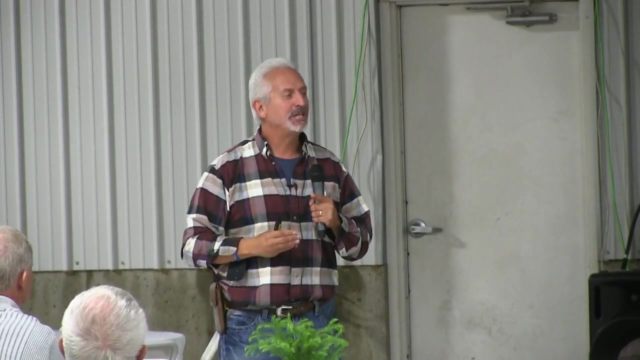 it, So he makes more money. You heard the lady, young lady, talk about. the more you have less of these chemicals, the more you will be rewarded, And rightly so, Because people are paying for your understanding and your integrity, That's. 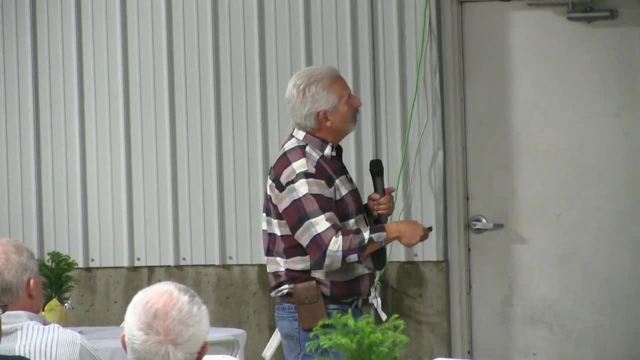 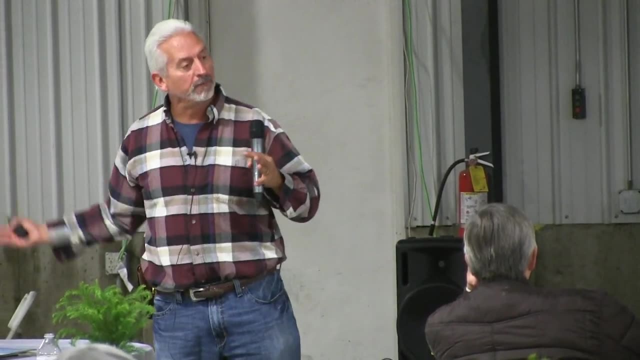 what they're paying for. The more you're intense your tillage, the more you're going to mess things up. If you till one small part of the farm versus the whole farm, it makes a huge difference. And then when you do your tillage and when 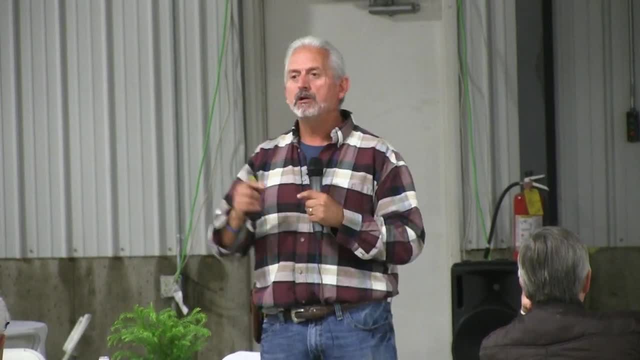 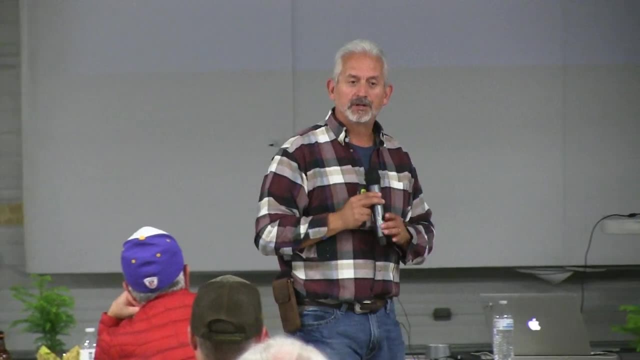 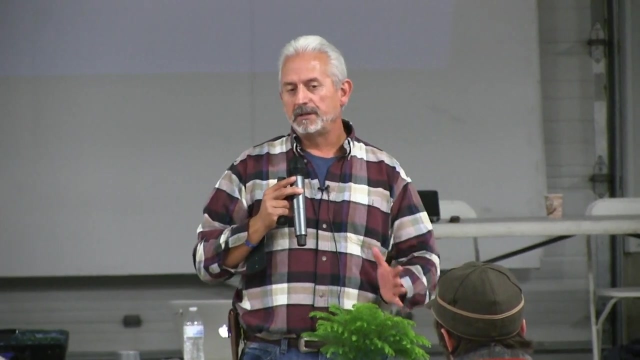 you apply your chemicals. This is the way we do chemicals right now, Insecticides: This is how we manage it. Matt, There's Matt right there. What if I told Matt? I said: Matt, now I want you to take a little bit of. 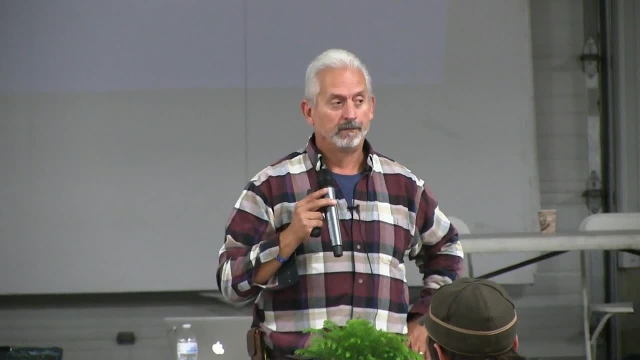 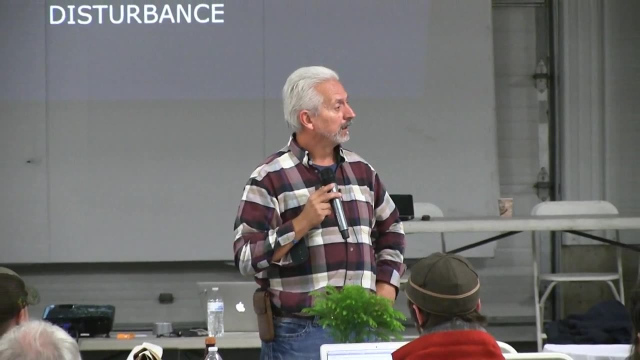 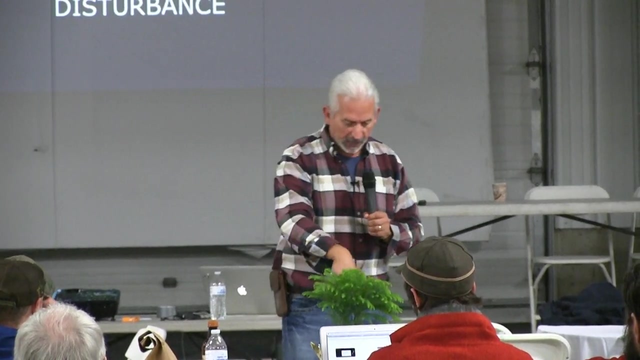 chemo just in case you get cancer. You think Matt would be would enjoy that. That's the way we do. insecticide right now, And fungicide- Oh producer calls him in. I got an outbreak here- Instead of doing the scouting. 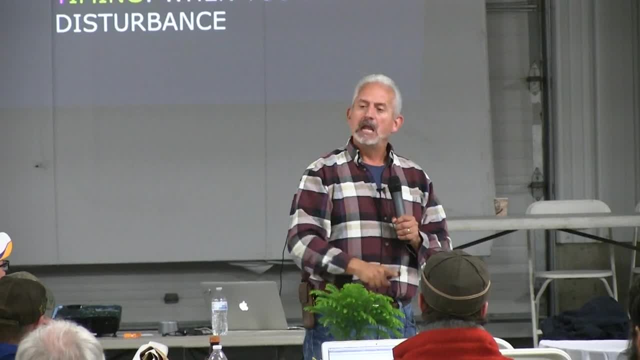 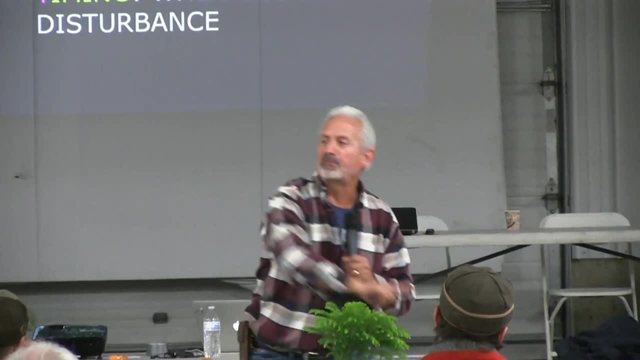 and looking at that field and just spraying that one field. But no, It may spread to the next field. I want you to get that field, that field and that field, And then the neighbors watch, then you spray the whole thing. 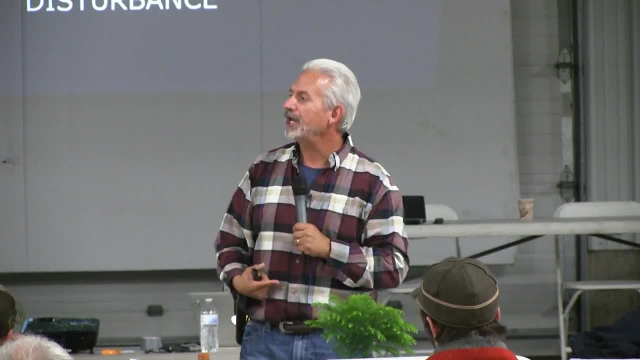 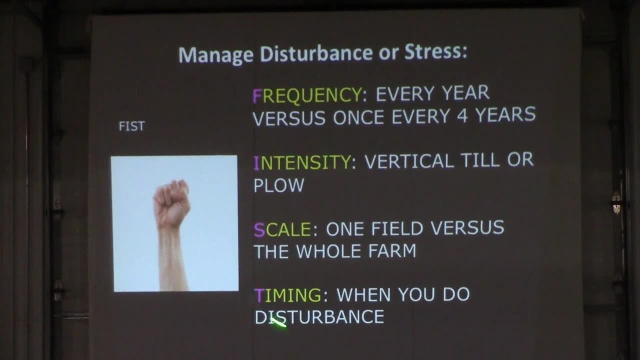 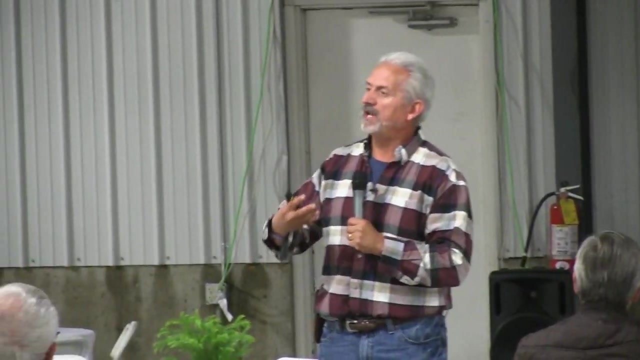 Then you hurt biology and life, And now it costs you money. Timing is everything. Some people say: well, Ray, when do I till? I'm an organic farmer, I would till when it's colder. The microbes are not going to eat your lunch so badly. 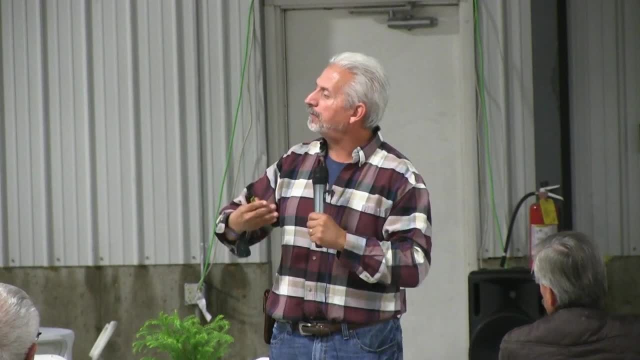 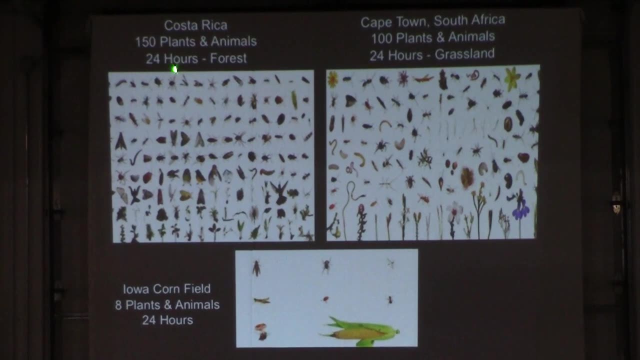 I say roll cover crops, Stop the tillage as much as possible. Look at the chemist, Look what happens. This is the diversity in Costa Rica. This is South Africa. This is the Iowa cornfield, Michigan's right next to it, Minnesota's right next to it. 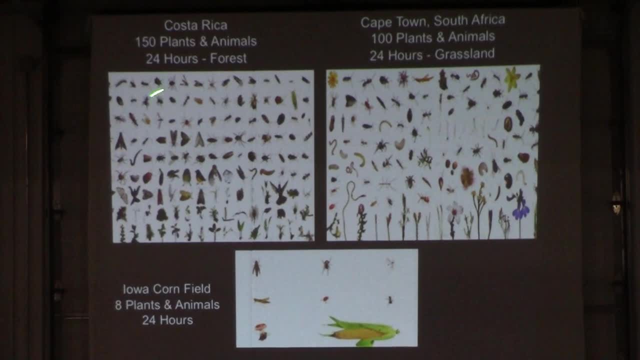 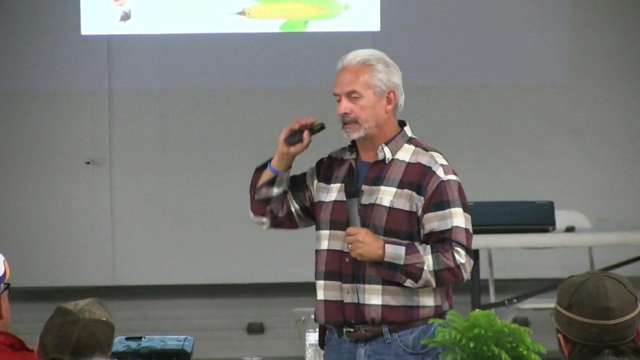 This is the diversity, This diversity we need. Nature is self-healing, self-regulating. Insects multiply every two hours. ladies and gentlemen, I have a question for you. Why are we overrun by insects? Do you think we could actually control? all the insect population? Really No, stinking way. Nature is self-healing, self-regulating. How come all of us don't have cancer? Cancer is just a cell gone crazy. no self-healing mechanism. Why don't we all have cancer? 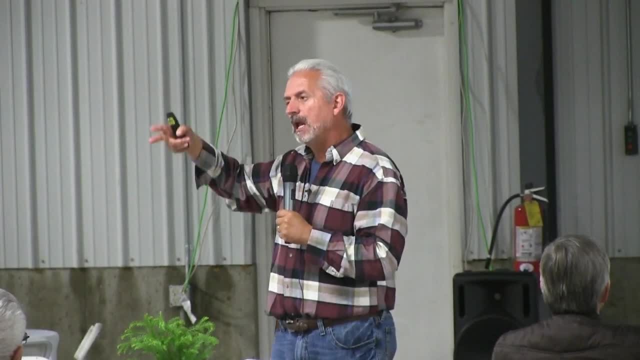 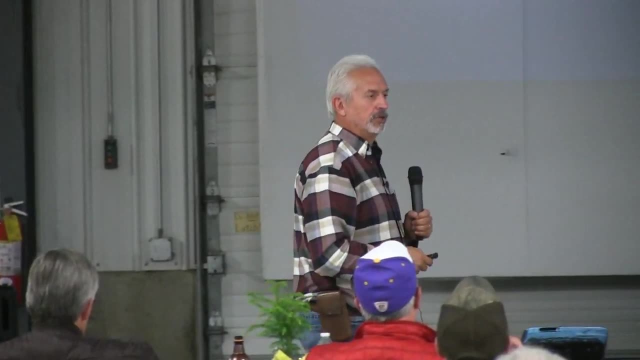 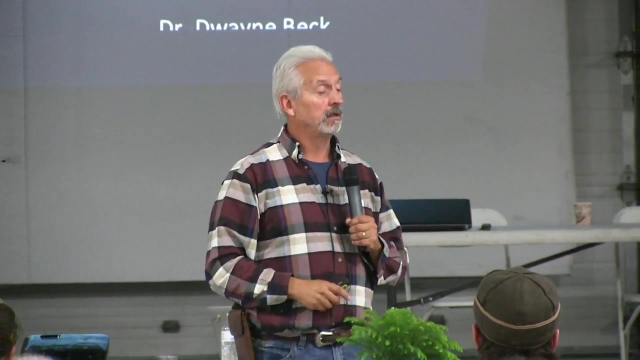 See, the natural system is designed to be healthy guys. Let's make it very clear about tillage. They knew in the 30s that tillage destroyed aggregates. We knew that, Dr Dwayne Beck, all tillage destroys soil structure. 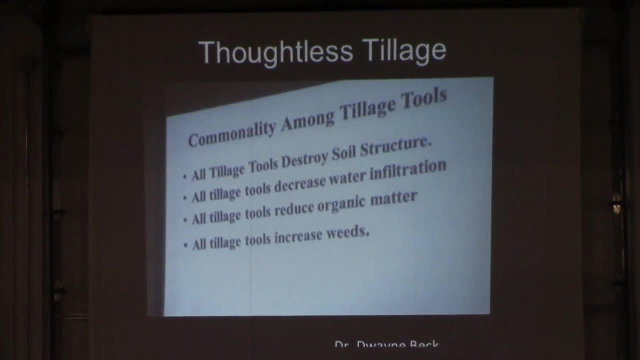 I don't care. All of it does All. tillage destroys, impedes water infiltration, It reduces organic matter and it stimulates weeds. That is the beginning of secondary succession. Tillage is not your buddy. You have to be careful how you use it. 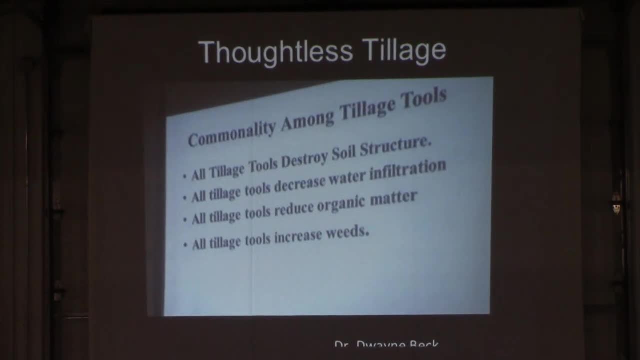 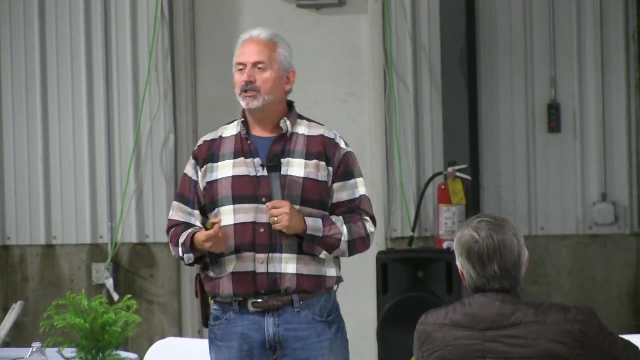 Reduce it as much as you can. I went to go speak in the organic group and the guys said to me: Ray, thank you for not beating me up with tillage. I said no, He said you taught me something very important. This is how I want you to. 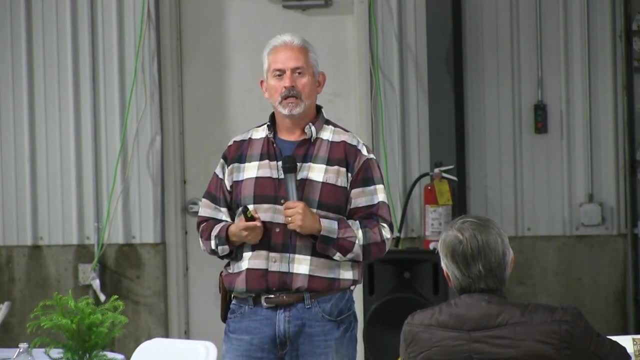 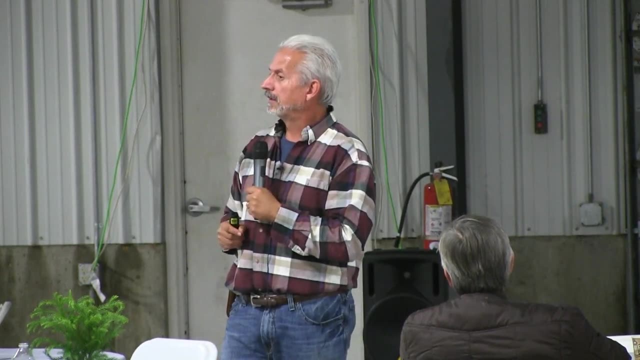 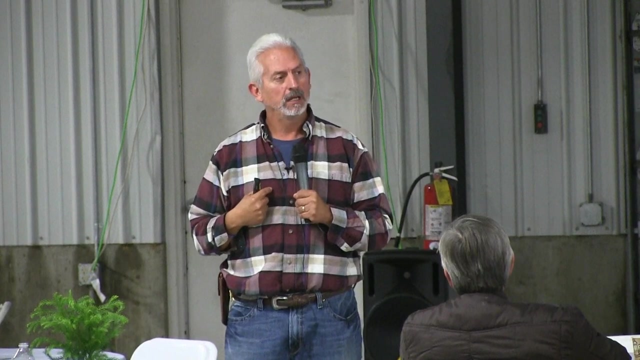 think of tillage guys. When you're out there tilling it better hurt Like you're running over your favorite pet- Then I know you understand And you'll figure every way how to reduce it. That's understanding. That's where I want you to be. 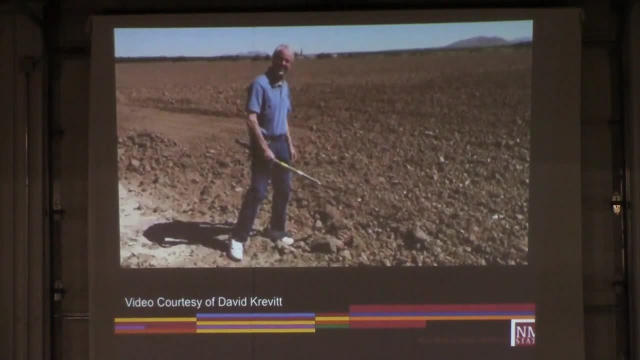 This is Dr Johnson. This is Las Cruces. This is a soil that has been tilled to death and hardly no organic matter. That's a clod. That's a clod. That's a clod. That's not a rock. 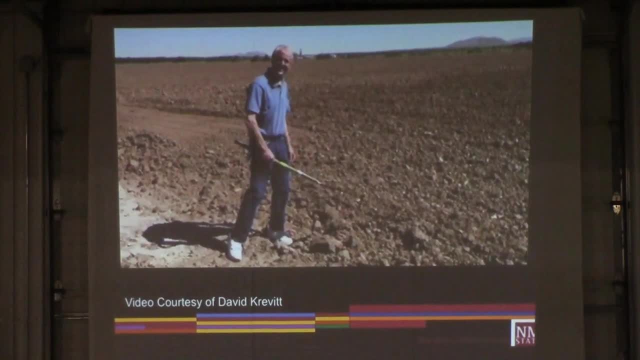 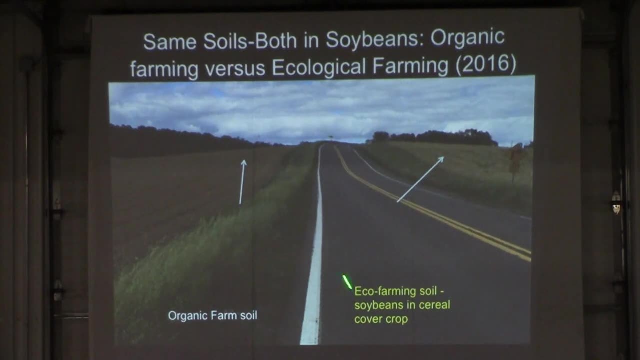 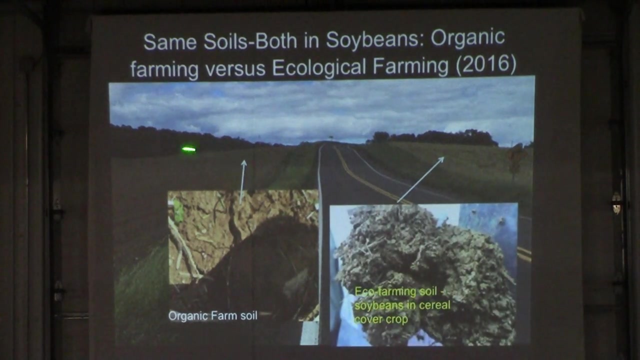 A majority of our soils in this country are carbon depleted. Everywhere Organic farm, no-till, multi-species mix and an occasional roundup and herbicide- The only thing that separates same soil types. Look at the difference- Same soils. 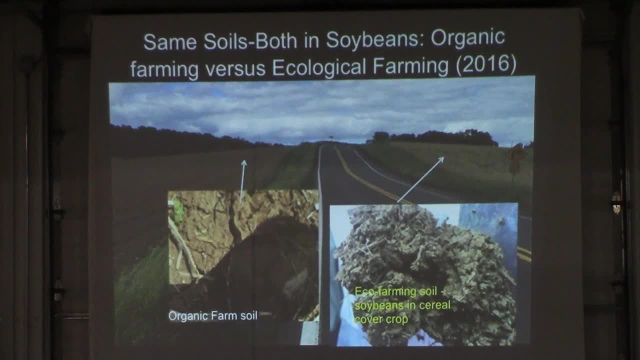 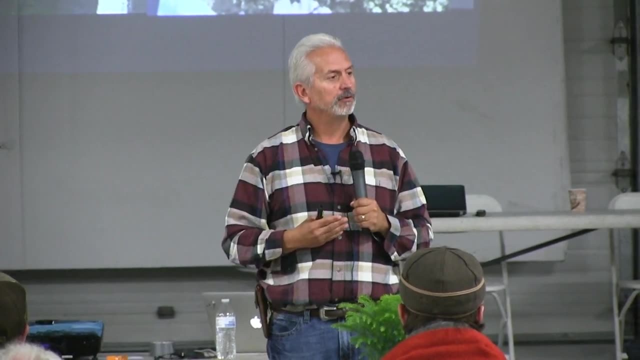 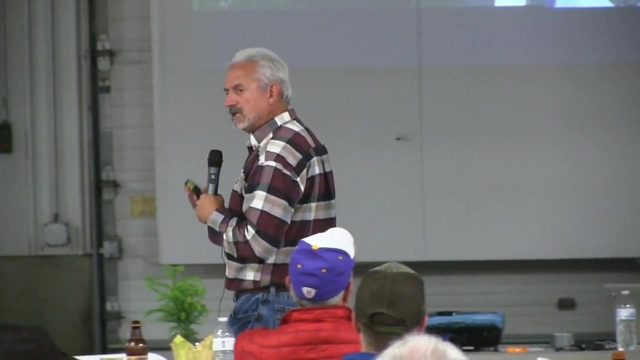 See, ladies and gentlemen, it's never been about organic, It's about regenerative ag. I have been in some of the most organic fields, absolutely destroyed and eroded. Same thing with no-till Sprayed to death: Does it impact everything? 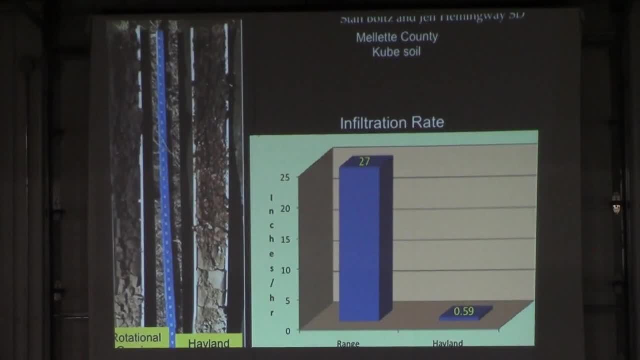 Yes, it does. Look at the even our grazing system. Look at the rotational grazing. Look at the colors. This is South Dakota. Look at the infiltration rates. Look at hay land, Another thing that's very, very destructive to the soil. 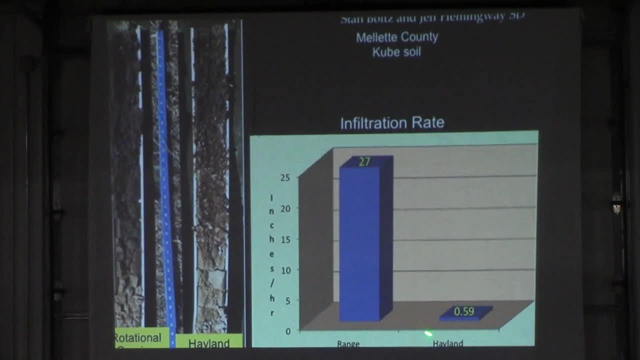 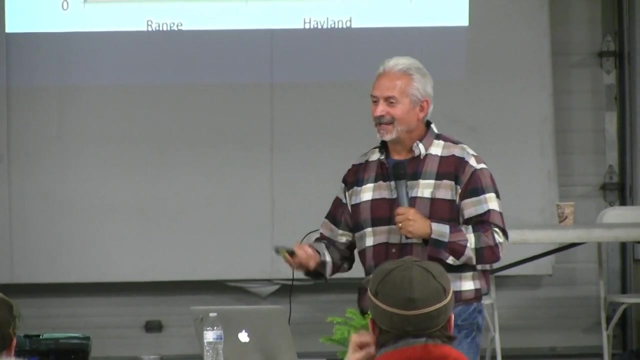 is haying. Look at the infiltration rates in a hay field. Why is that? Look at the colors you're taking from the factory workers. You're always removing, Always taking. So how do you fix it? Buy new land, Take it from the neighbor right. 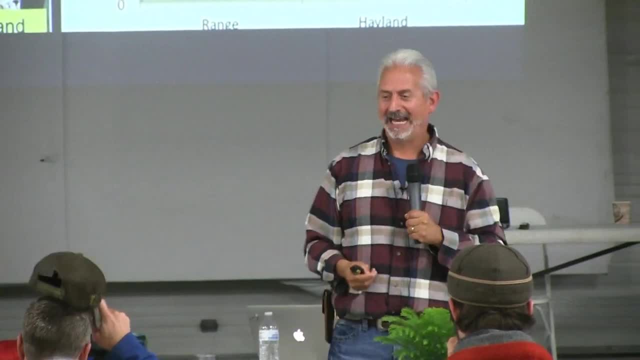 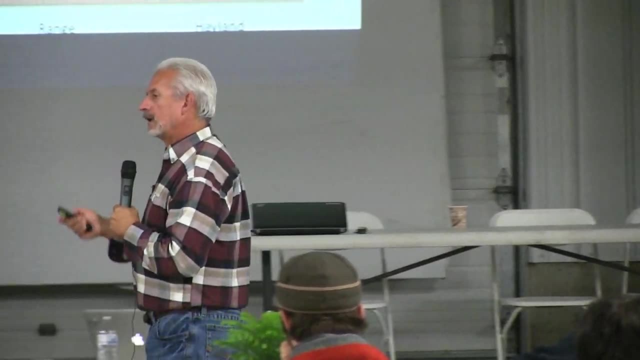 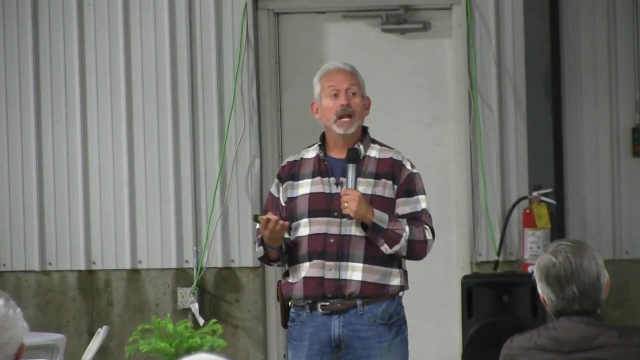 Buy your hay. I buy my hay. I never take my. I used to raise hay. Never again. I will buy it. Now somebody will say, Ray, aren't you taking from them? They need the money. I'd rather them not do it. 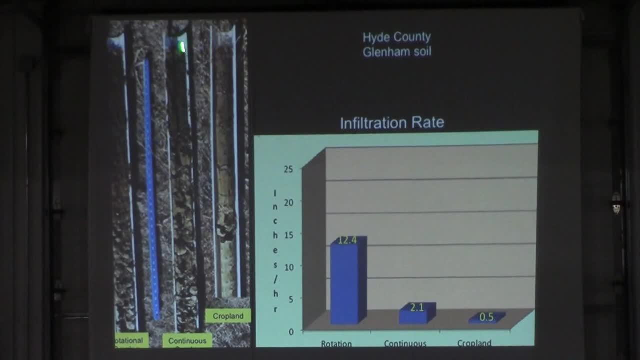 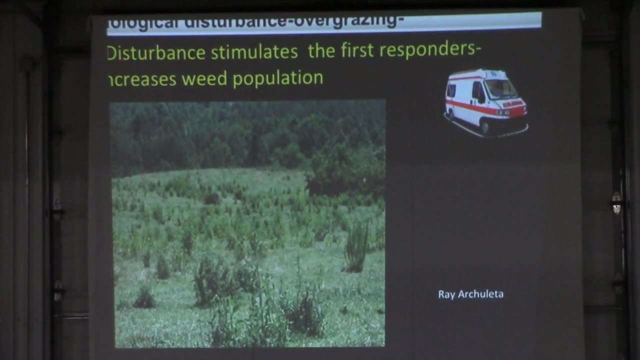 Crop land: Continuous. Look at that. Rotational grazing, Continuous grazing. Let the cows do whatever they want. Look at crop land. Look at the infiltration rates. Same soil types. Okay, so If you have problems with weeds, Does anybody in here not have problems with weeds? 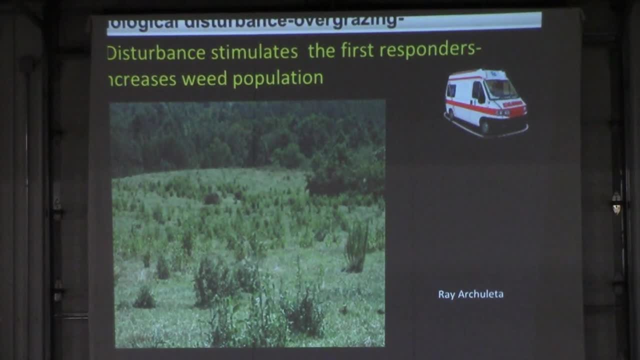 and you hardly have any weeds on your farm, Raise your hand. I didn't think so. When I know that producers have problems with weeds in their pasture, they're overgrazing. If farmers have problems with weeds in their farm, they're over. 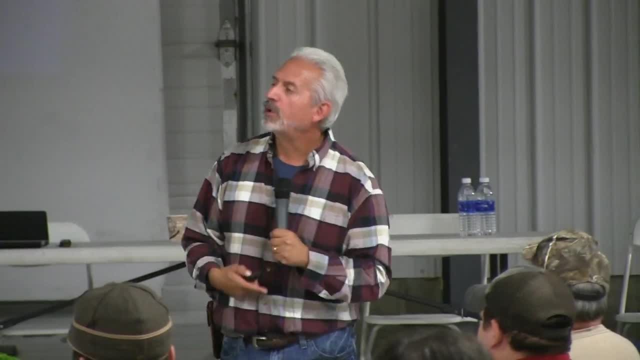 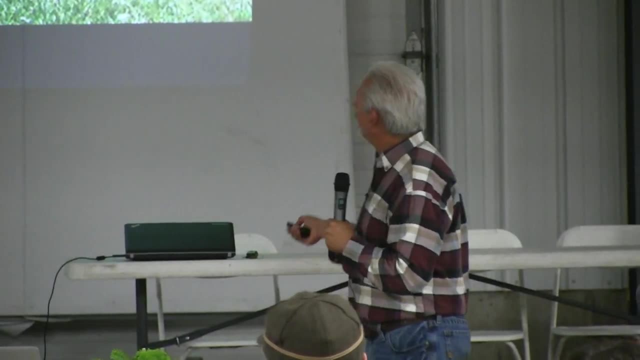 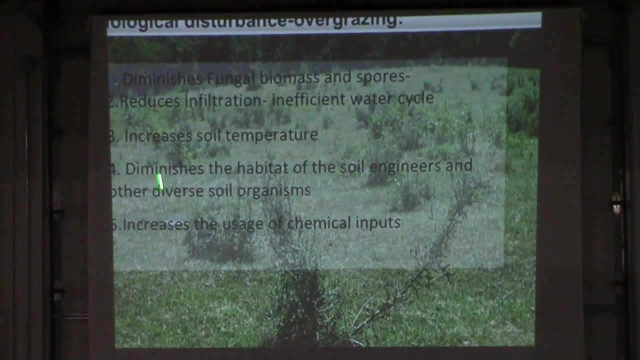 they're doing too much tillage, Poor rotations. Nature's healers and scabs are the weeds. I call them the first responders. When you impact that system, you diminish the biology. Anytime you see these scabs out there, they're telling you something. 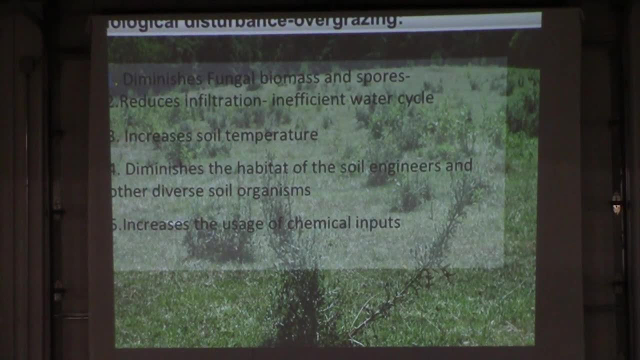 They're the healers. There's a book I recommend for everybody. It's called Guardians of the Soil by Dr Something. Just write the word free: Guardians of the Soil. I have changed completely the way I look at weeds: Guardians of the Soil. 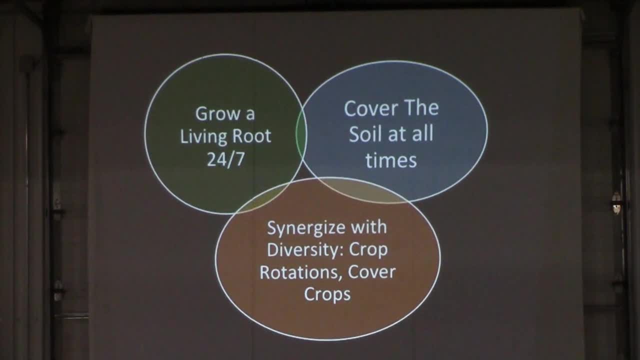 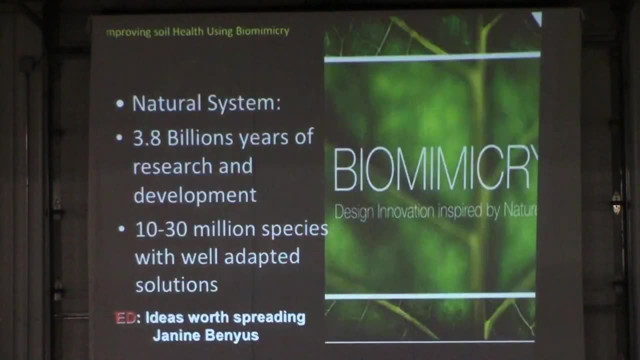 Okay, now we're getting close. How much time do I have? Kenny, Ten minutes, Let's go quickly. Okay, now the other three. Synergize covers living roots. Okay, Everybody. I would write her name down. 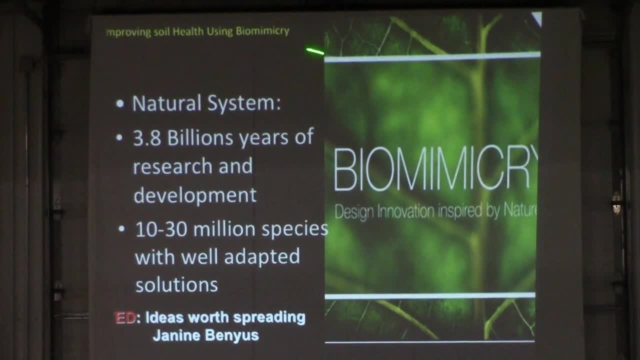 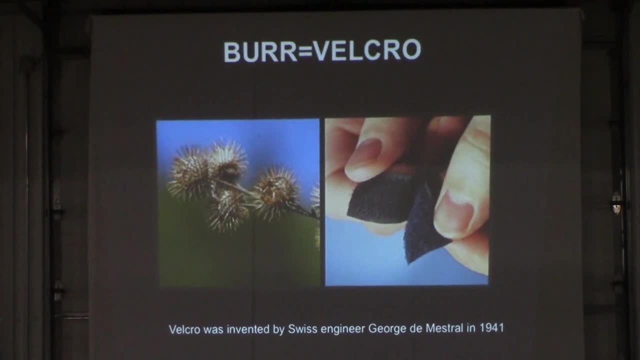 Her name is Janine Benyus. TED Talk. She gives the most awesome TED Talks on biomimicry, mimic life. Their TED Talks are awesome. She says man nature's got 3.8 billion years of research and development. 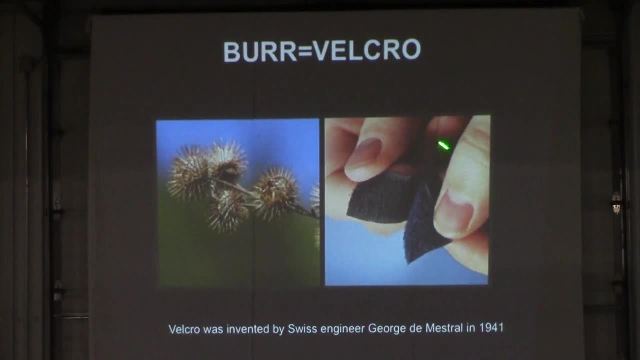 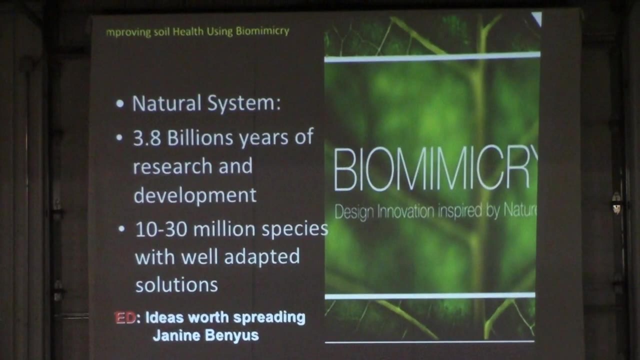 In fact, some of our most awesome research has come from. some of our most incredible inventions have come from nature itself. Velcro Janine Benyus: Just type the word biomimicry, She'll come up. She's an amazing speaker too. 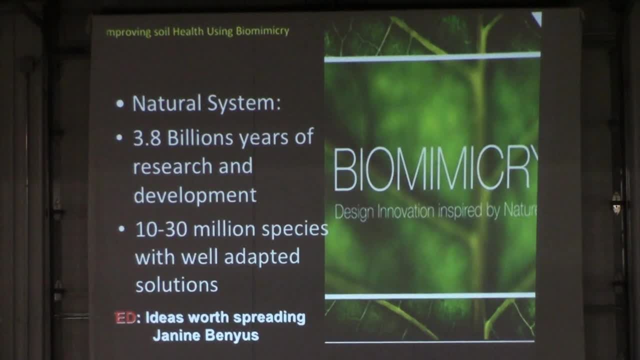 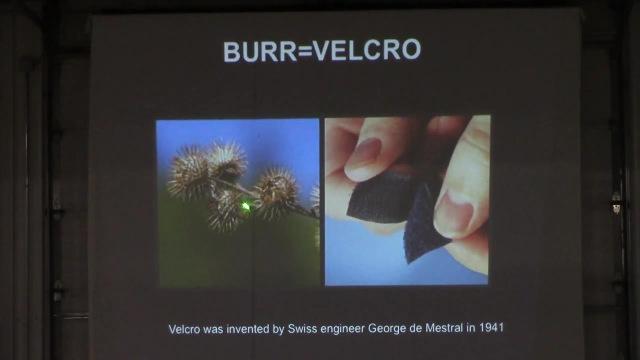 Love her. I bought her book. They have an institution of biomimicry. Can you imagine going to school? What do you do? Well, I'm a biomimicry. Very cool, Velcro was designed. an engineer found out its design. 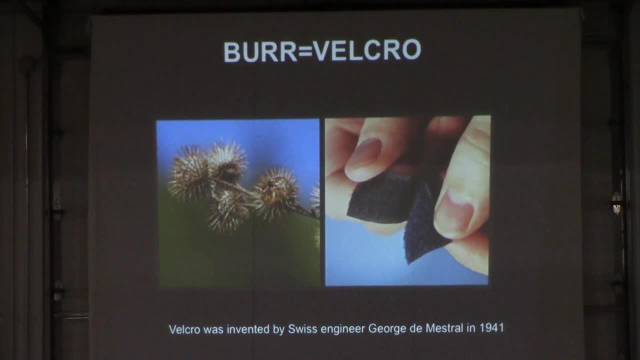 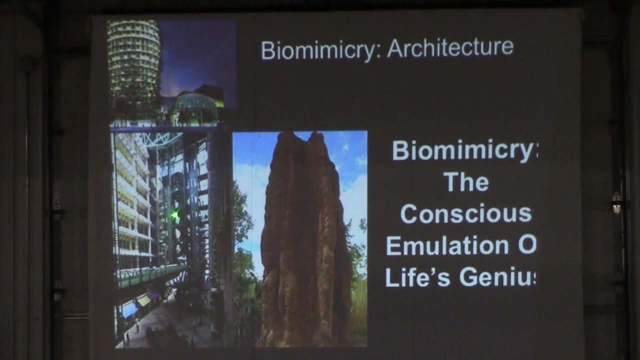 and he knew from the it was stuck to its dog's fur And the name of that engineer is Millionaire, Billionaire, Billionaire. We are mimicking termite mounds. ladies and gentlemen, right now We are mimicking those termite mounds. 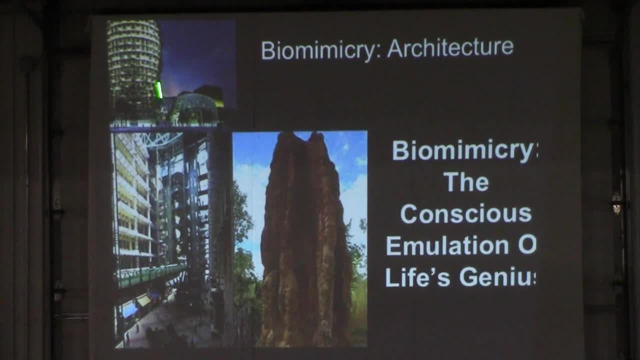 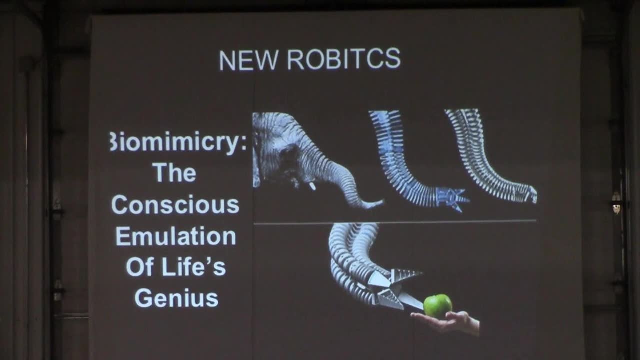 because they are incredible for regulating temperature. We are now putting it in our buildings and reducing it by 90%. We're mimicking elephant trunks. The answer is in the natural system, She argues. well, if the answer is in the natural system, how come? 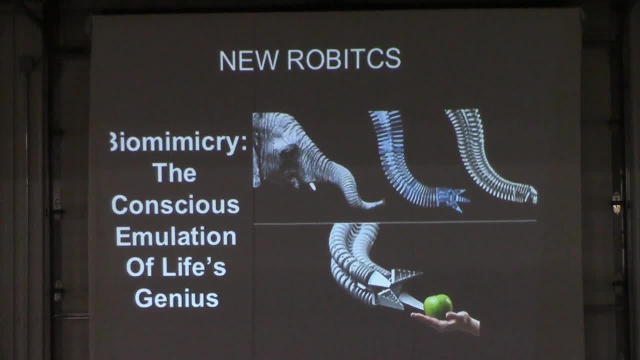 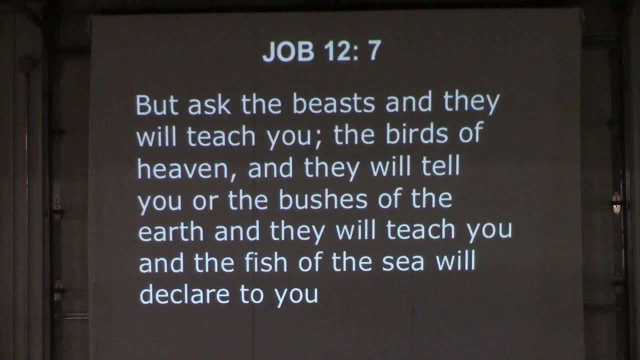 we don't farm like a prairie in the forest. That's what we're starting to do. That's called agroecology. Biomimicry has been around for a long time, ladies and gentlemen. It's biblical: Ask the beast. 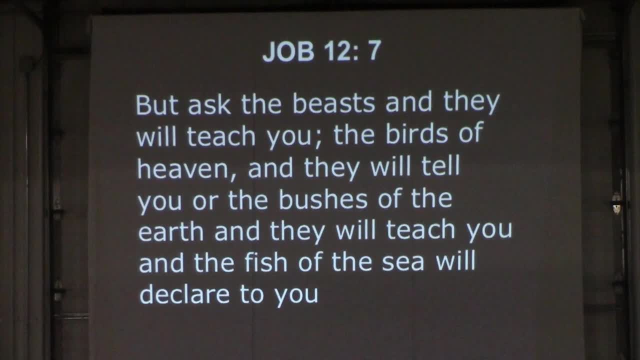 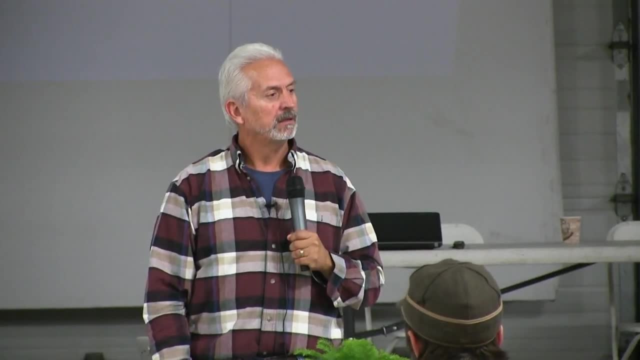 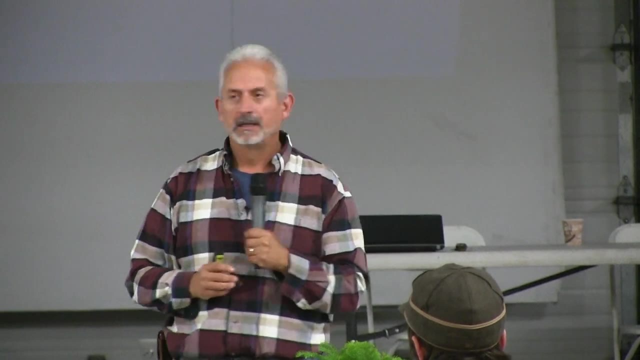 They will tell you How many of you, just recently, in the last six months, have just actually walked up on your forest and just sat there and contemplated and observed. It's hard when we're so distracted from it. Do you know why I missed it? 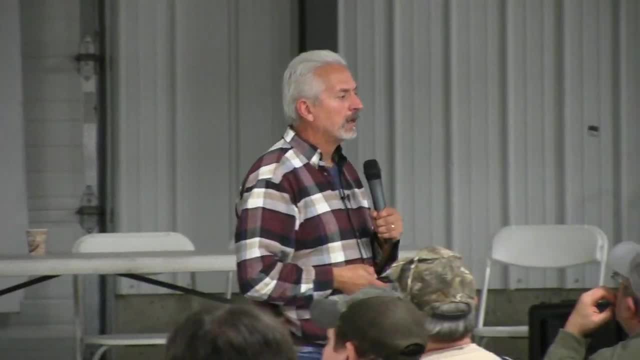 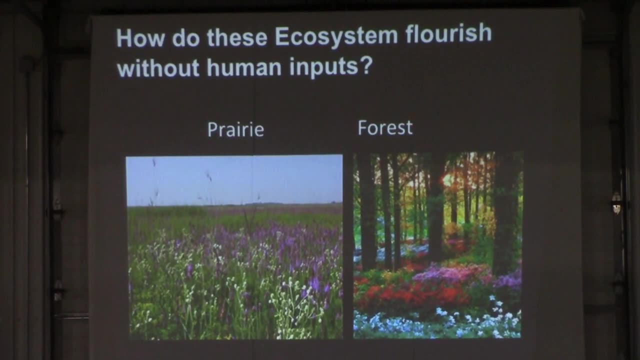 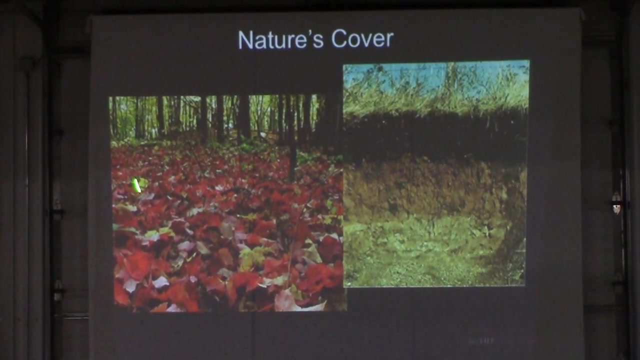 Eight years of university study, I forgot. Nobody taught me to be an observer. This is the goal, And let me show you how farmers are doing it now. This is what we're mimicking: The forest floors. we're mimicking the. 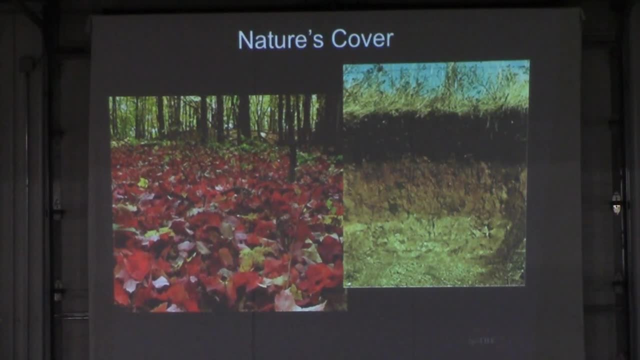 architecture on the top, and we're also mimicking the armor. If you walk in the forest, what do you see all the time? Armor. I want my soil armored and I want green growing out of it. Let me show you what we're doing. 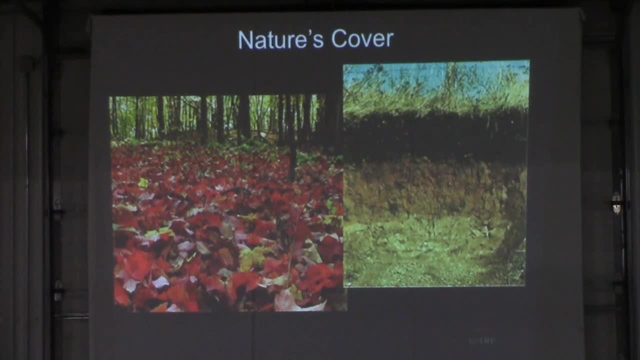 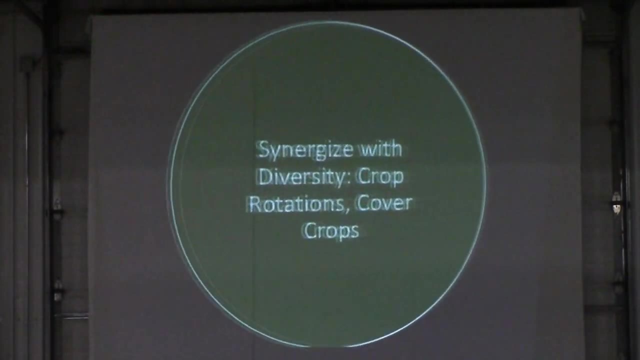 The same in the prairie. If you walk in your lawn, you pull your lawn aside and guess what you're going to see? Brown, That's called the detritus sphere. It's always present. Look what our farmers are doing. 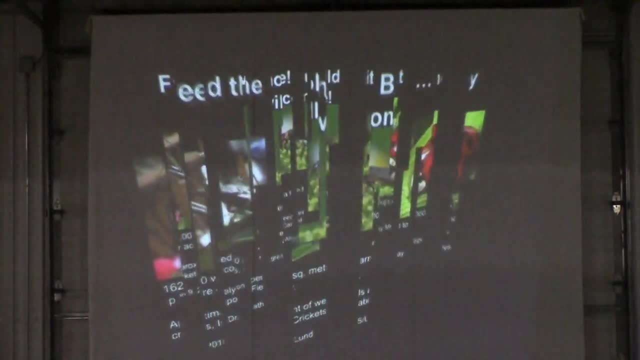 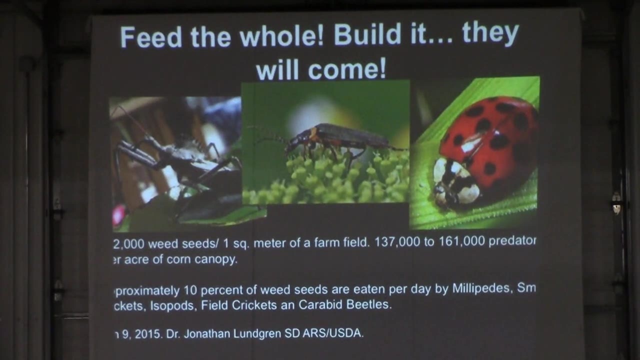 We're designing mixes to do this and we're putting them out there so we can bring diversity, because if we bring diversity, we're going to have all the insects, the natural predators. Oh, by the way, just recently, research came out: 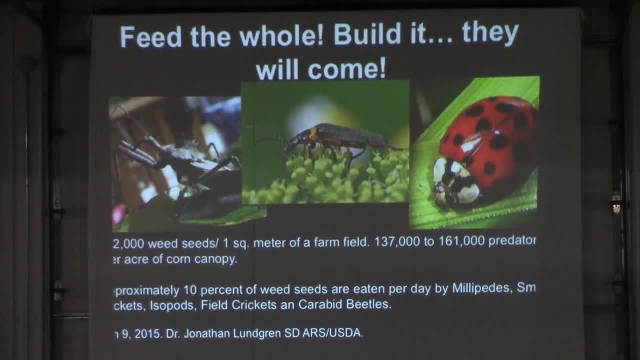 just yesterday that I saw fungicides are hurting bee populations. That's pretty devastating. Now we not only know the neonics, but the fungicides are hurting our bee population And the number one money producer per acre is honey. So if I bring, 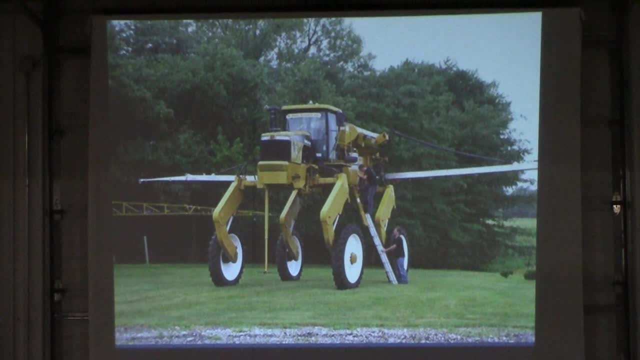 this is what farmers are doing. How many have actually seen one of those? When I went to the organic conference, one of the people in the organic conference in Pennsylvania said that's a cancer machine. I said that cancer machine is a cover crop machine. 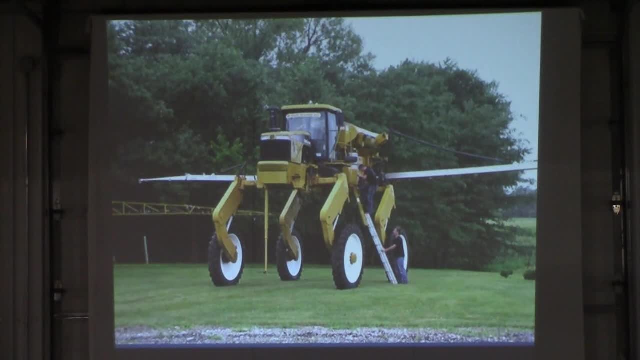 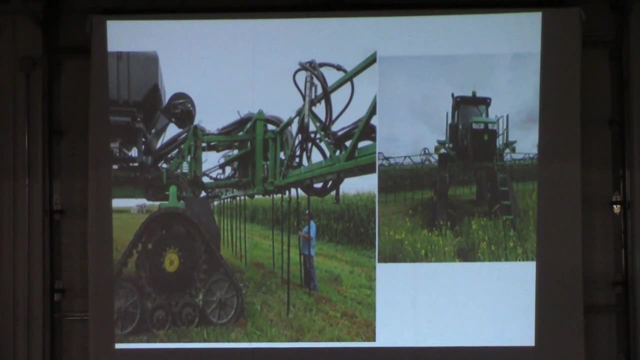 also blowing cover crop seed on standing corn. Farmers are building this. People have asked me: are the big operators catching on? I had one guy that came to one of our schools: convert 30,000 acres into cover as a no-till. 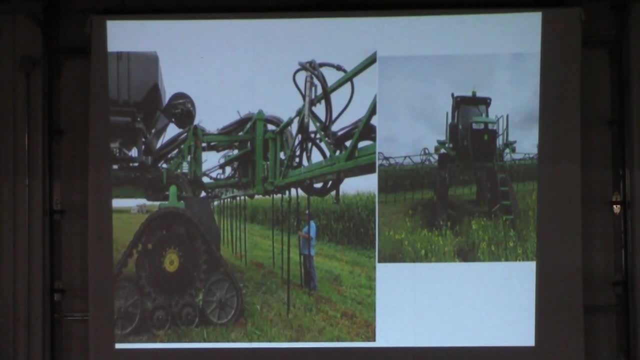 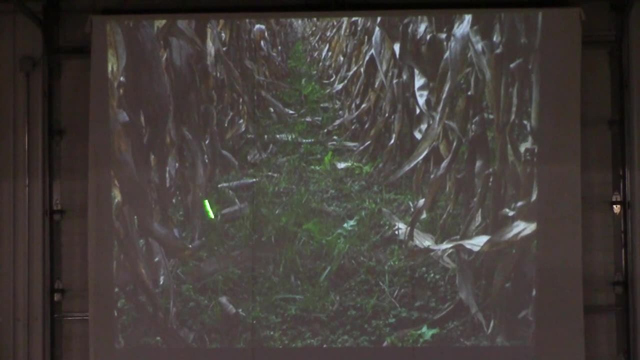 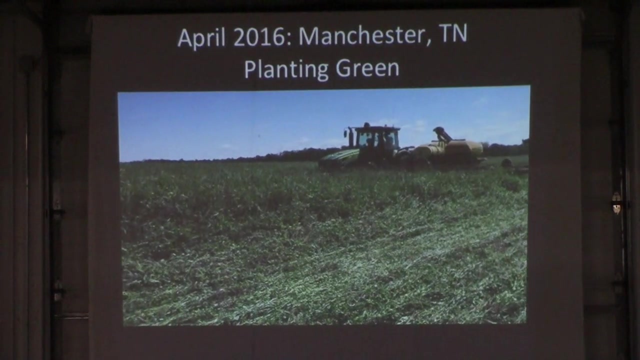 One soil demonstration. Look at that dropping it. Why do they do that? Why are they willing to invest in that? Because of this, ladies and gentlemen: they want living cover, capturing sun. They understand soil function. now This is spreading through the country. 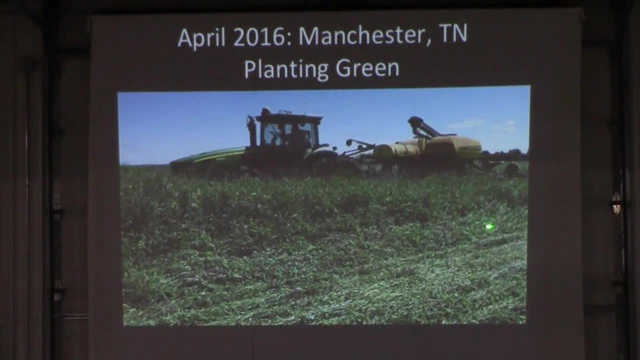 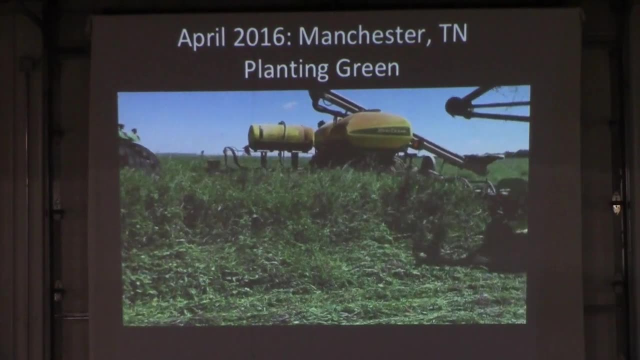 This is going to be farming of the future. I'm so excited about it. This farmer is capturing water cycles working. He's capturing sun to the last minute. The nutrient cycling that's a multi-species mix with legumes He is. 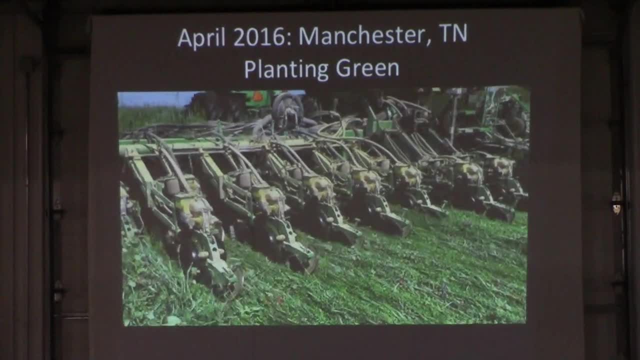 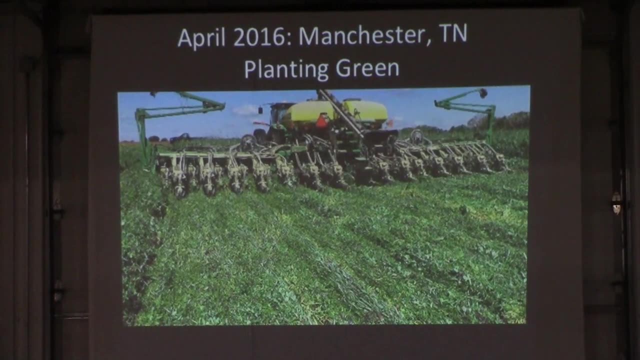 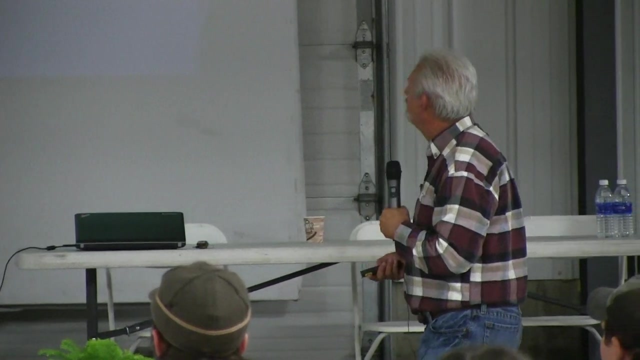 diversity. He is planting corn and we also plant soybean. We have hundreds of thousands of acres through the country doing this. This is in Tennessee. He is capturing. he is following all the ecosystem processes to the last minute. No roller needed. 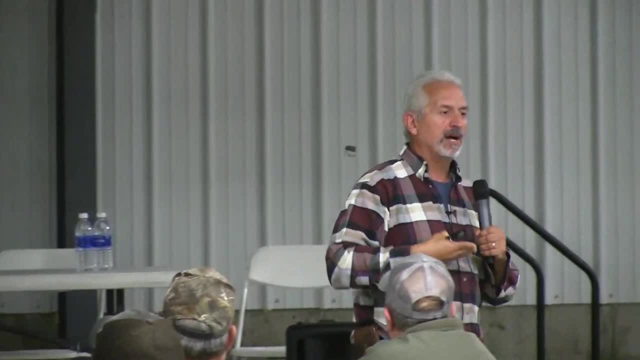 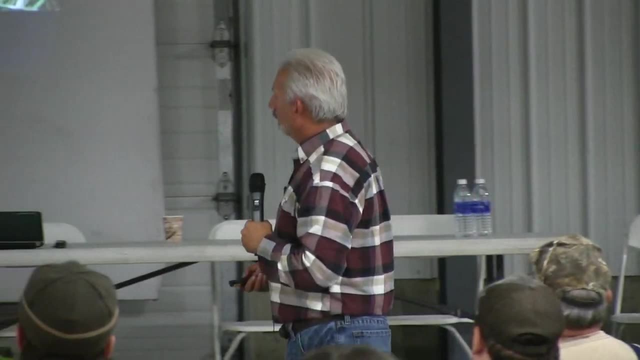 We designed the right amount of vetch, about two to three pounds. It helped to lay it down and we love sugar rye. We plant our corn right into it And those planters are amazing. Cut right through it. This is Adam Daugherty, one of our. 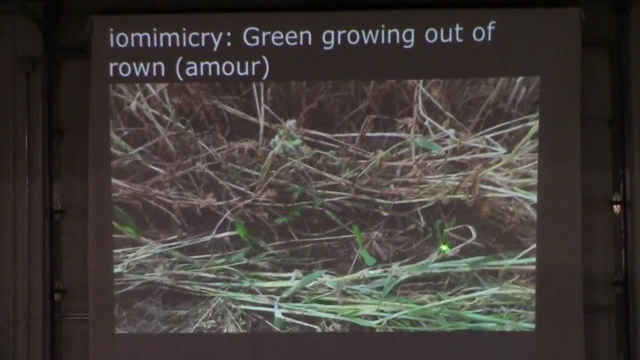 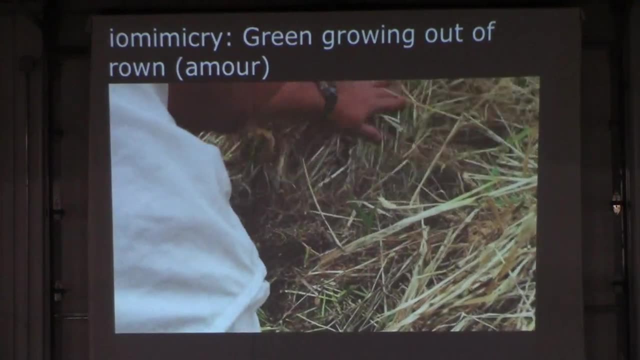 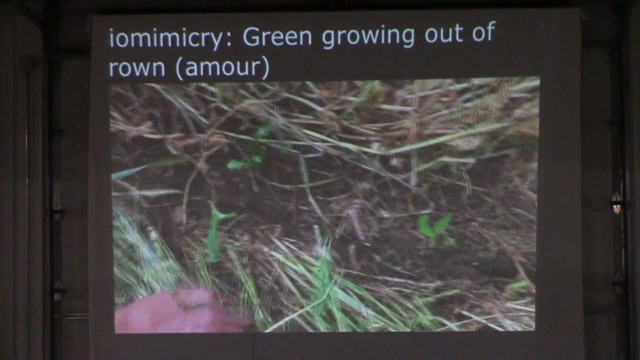 best DCs in the country. There he's pulling the corn away That young man. in less than three years, 40% of his county is covered. When I drive, you know what I see? Bare, bare, bare bare. 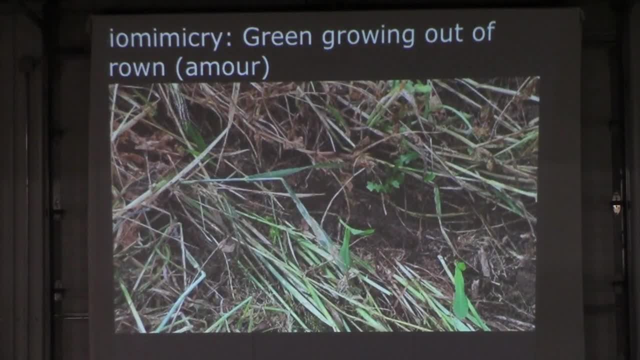 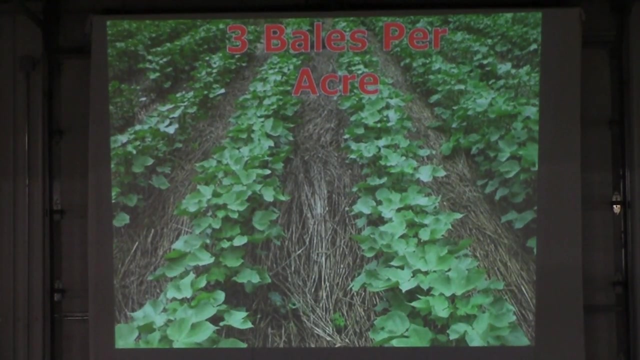 bare, bare fields, Naked fields, And his county is covered, covered, covered. It's amazing to be in a place that there's cover. It's exciting We're doing it in cotton. Look at the weed suppression. We were losing the battle in the south of. 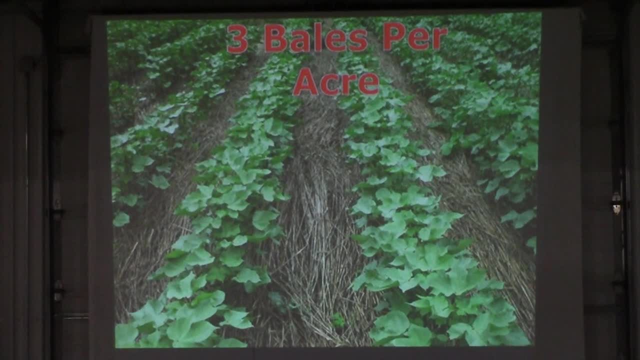 Arkansas Farmers were giving up farms because uh pigweed was overcoming them. They were roundup resistant. There was nothing that controlled the pigweed. Cereal rye, in combination with chemistry, we have brought farms back. They have been resurrected. 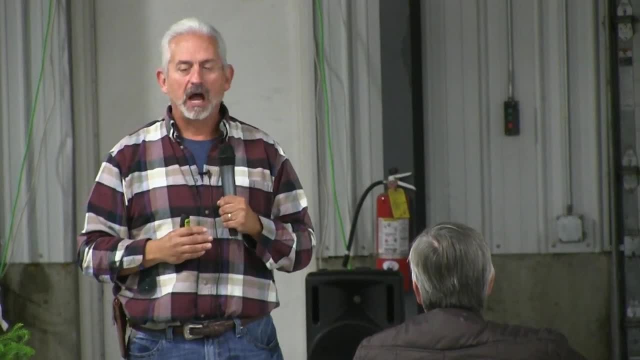 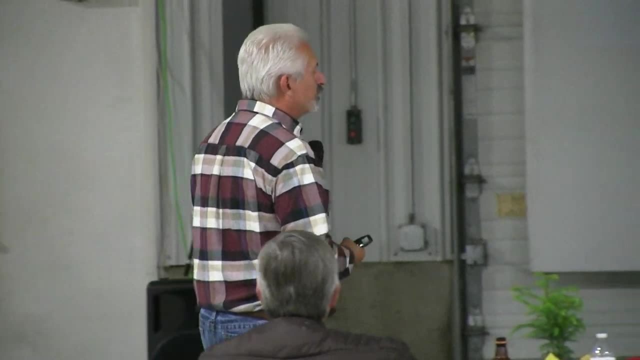 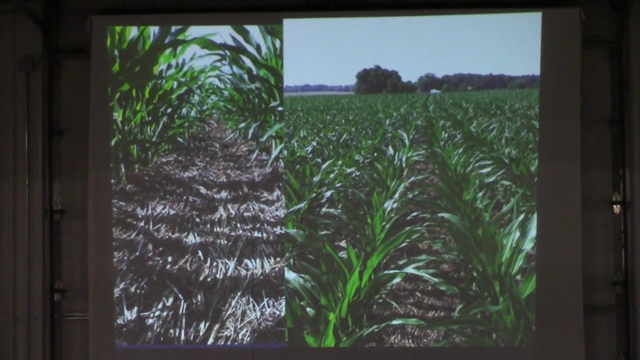 from the death. They have come back to life through covers. We were able to control it. Pigweed hates cereal rye. It's allopathy. It does not affect corn. People say, well, it's affected corn. It's not true. We've. 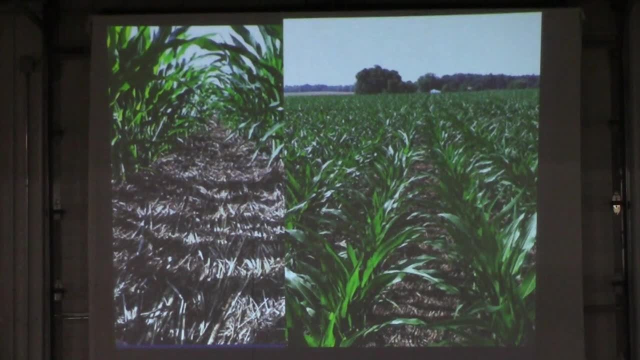 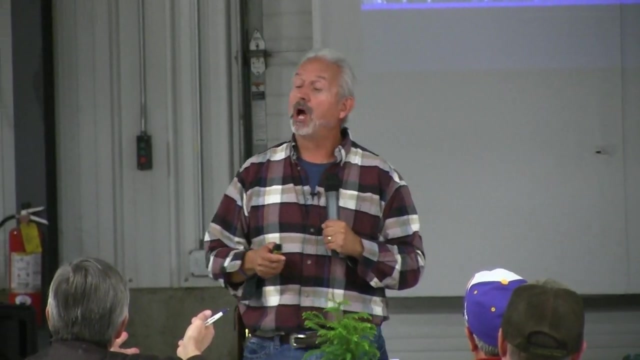 done thousands of acres. When you have a round, you have a problem with cereal rye. it's a nitrogen issue. Please understand. they will steal all the nitrogen out of the soil. It's designed to do that. Yes, sir, Yes, Well, no. 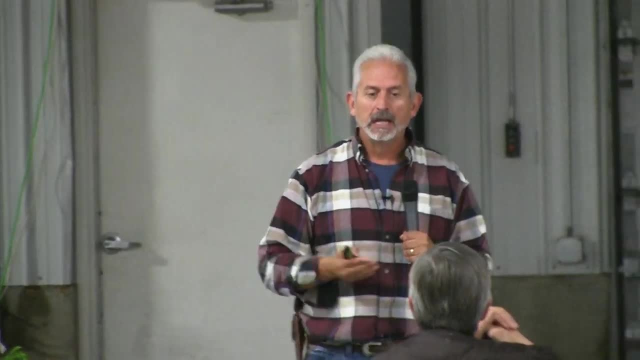 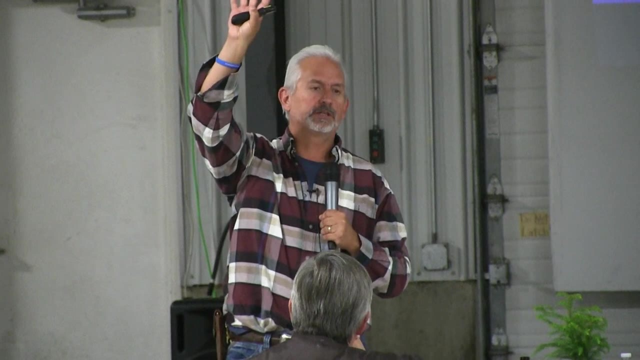 We've seen. we've had great success with it. Here's the kick. Here's something you have to watch. You have to. I, if you have a chance between standing it or rolling it, I prefer rolling it, But because you're so far north, you're just. 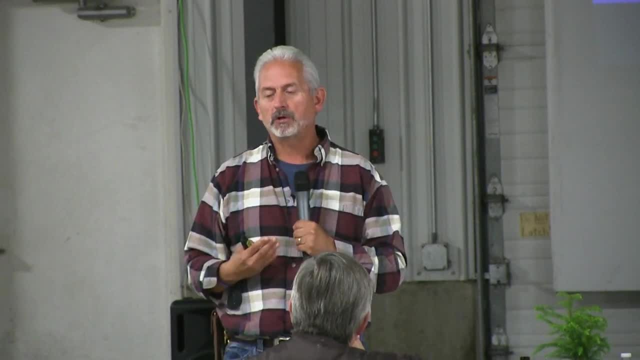 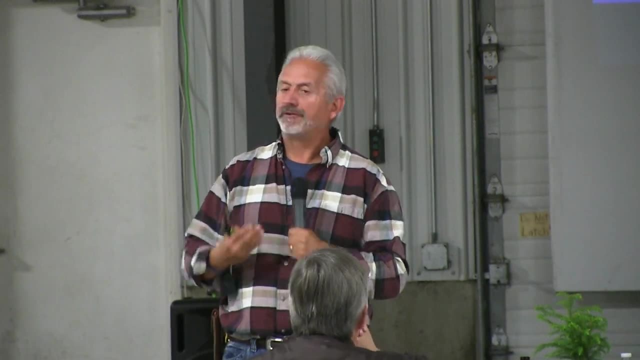 going to do it standing. We don't have those issues. But please understand where the struggle is. You're having soils now that filtrate, that hold water. They're functioning. I had a young farmer call me one time. He says from: 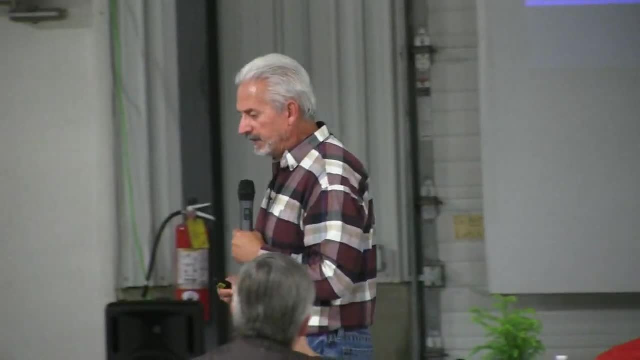 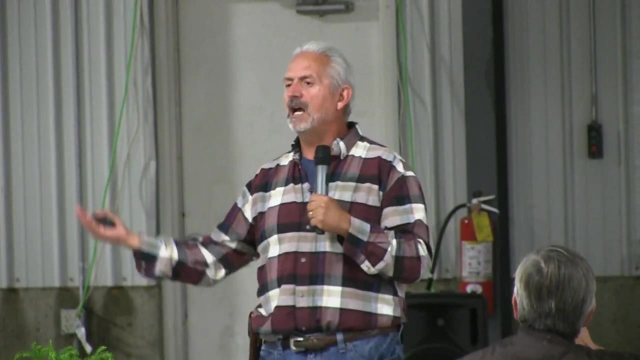 South Dakota. He was so frustrated He emailed me and gave and said: Ray, I do the no-till, I do the covers And I integrate animals and my corn looks like crap. We've got 25 inches of rain all in. 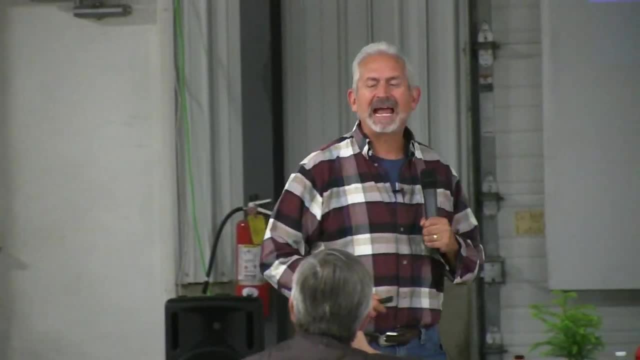 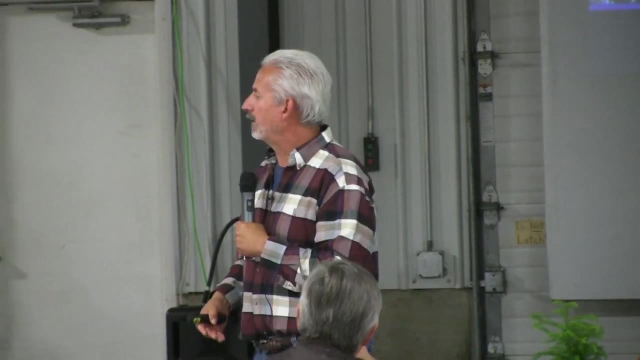 one month. I emailed him back. He says: my neighbor's corn look great, Mine looks terrible, It's yellowing. I'm going to plow the whole stinking farm. I emailed him back. I said: don't, The water ran off. 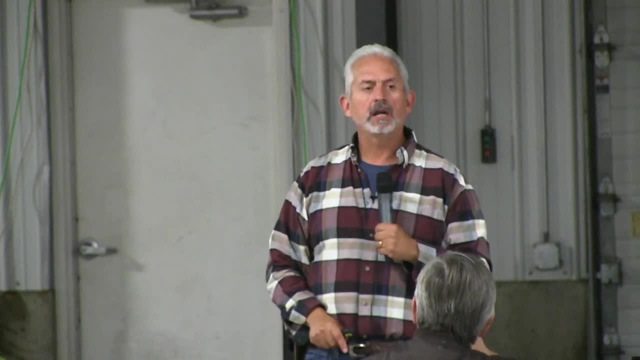 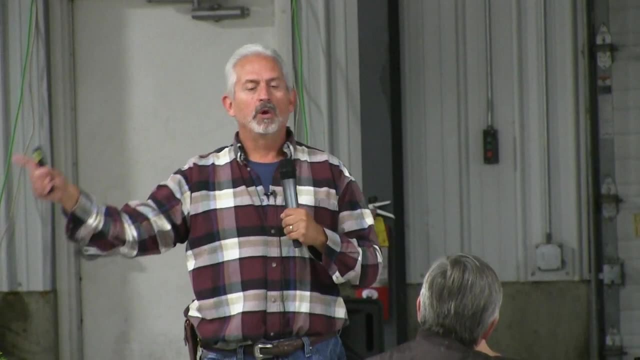 all your neighbor's fields. Two months later he emails me. He says: all excited. He says: Ray, I walked the fields. Every one of my neighbor's fields were overcome with weeds. We went into a drought. My corn looks great. 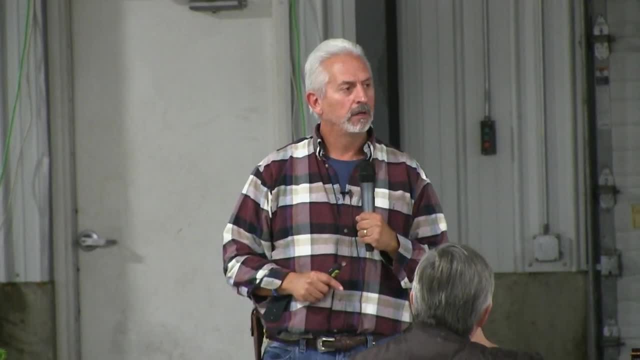 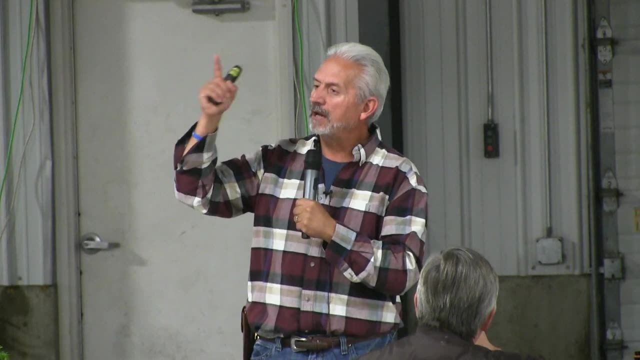 I said: do not mimic your neighbor, You'll go broke. You go observe. Luckily, he says I didn't plow my field. I said I'm glad, Thank your brother. He stood in front of the plow. 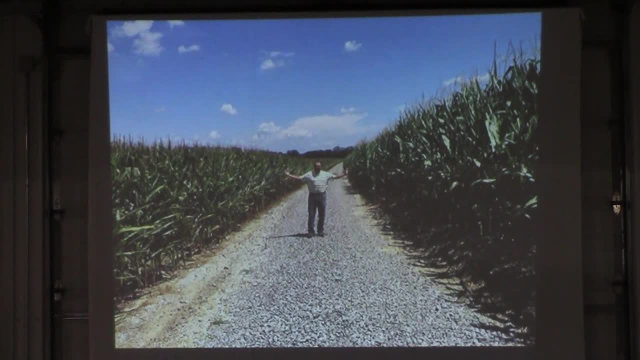 Here's the covers. Notice the difference. This is worth 30 years of no-till. This county has been no-till for 40 years. 80% of that county is no-till. This young man took it from. this is regular. 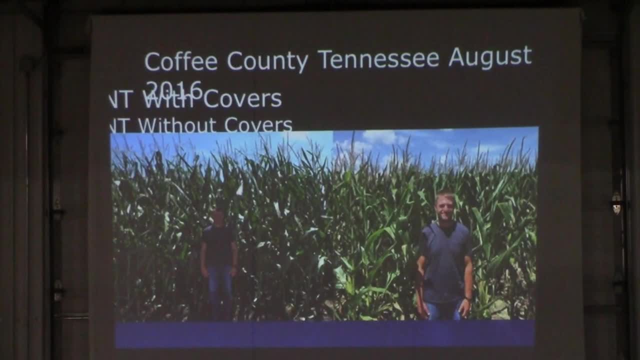 no-till. This is no-till. with rolled covers, Area gets 50 inches of rain. These guys are averaging 250, 260 bushel easy. Are they as good of soils as Iowa? No, but they're doing. look what we've done with those soils. 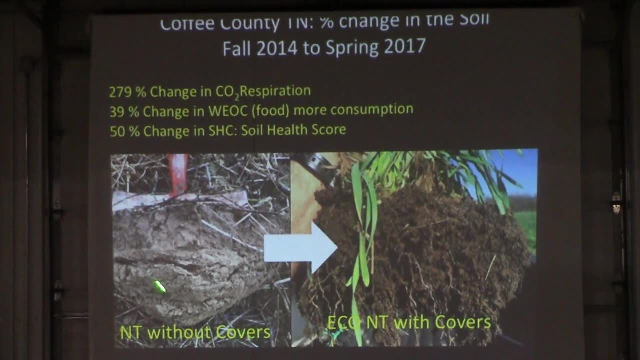 in less than three years, No-till without covers. That's the way the soils look like: Stratified, oxidized. They had layers of compaction. Look at what happens with three years of covers: 279% change in respiration. The microbes are going. 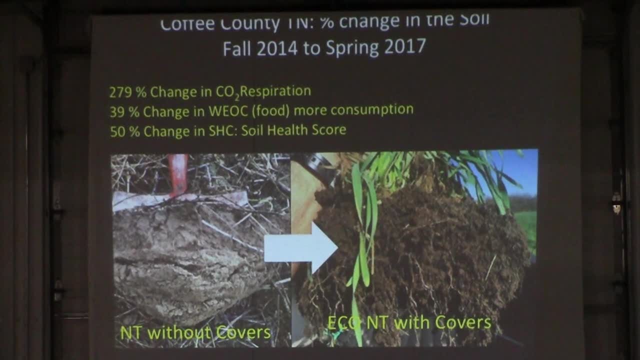 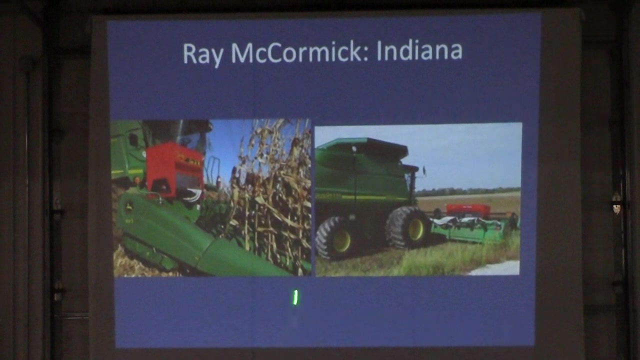 They consume huge amounts of food. They will. if you trip in those fields over there, you'll be dissolved. They are cycling The soil. health scores jumped up 50% in less than three years. We are using the Gandy seed box. 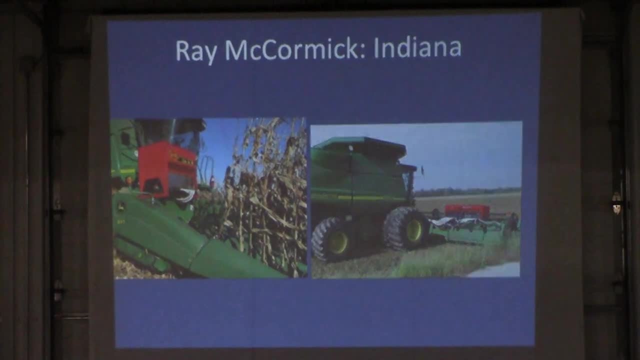 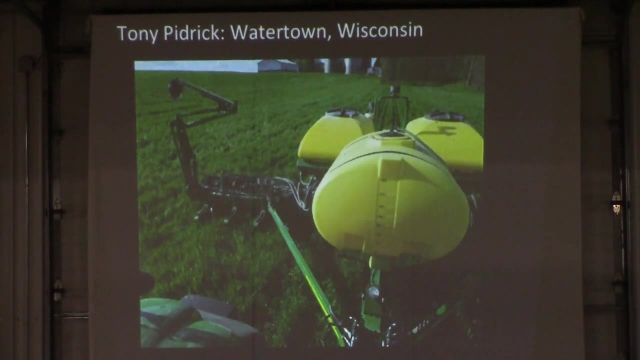 This is Indiana As they're harvesting corn. that thing is dropping cover crop seed- Amazing. Here is my buddy, Tom Pedrick, Wisconsin, Watertown. He's been doing planting green for the last two, three years. I've been all over. 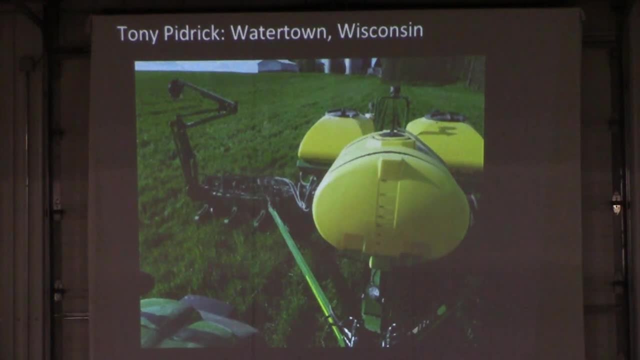 Wisconsin talking and I said, Tony, why didn't you let me show that slide? I didn't want people to get all I don't know. I don't want people to think I'm crazy. Now he's got a large group of farmers following him, He's got a huge 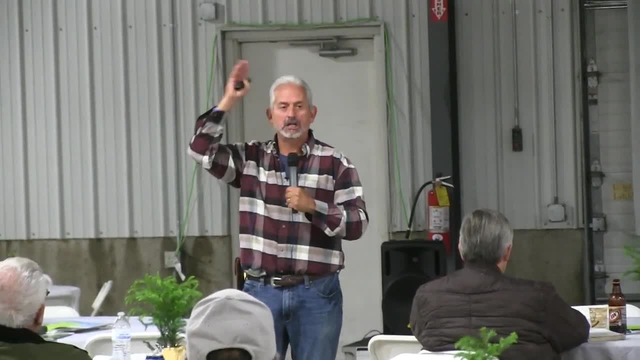 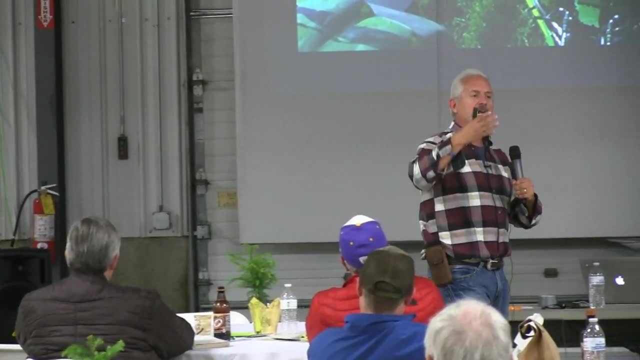 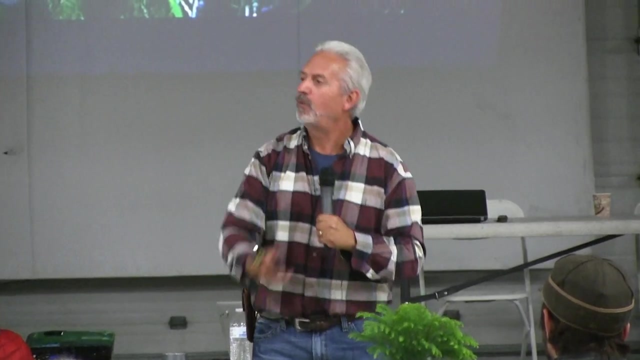 group. They have soil health communities where they're doing planting green This year. he said the rains came. my neighbors were drowned out because we have heavy soils. I did not drown out because those covers saved my bacon. It rained and it rained and he sucked the water. 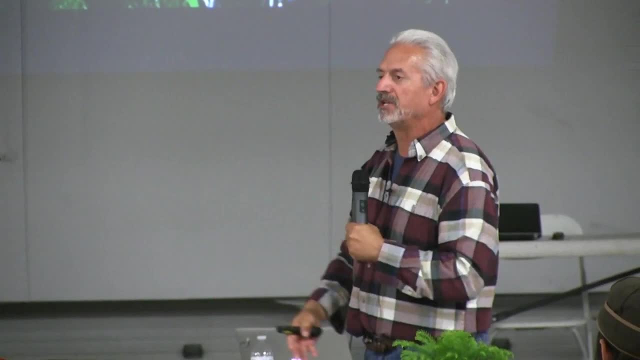 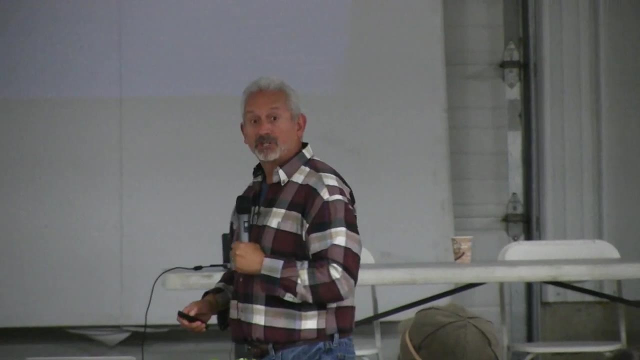 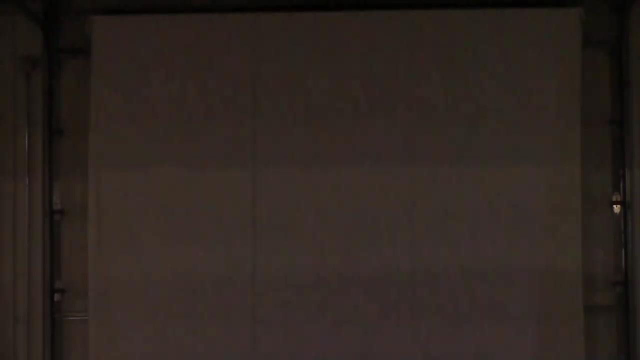 out and I was able to get out there and plant, and my corn produced 260 bushel Ka-ching, Mimic nature. How much time do I have, Kenny? Three minutes. Well, since I got so much, let me get down to the. 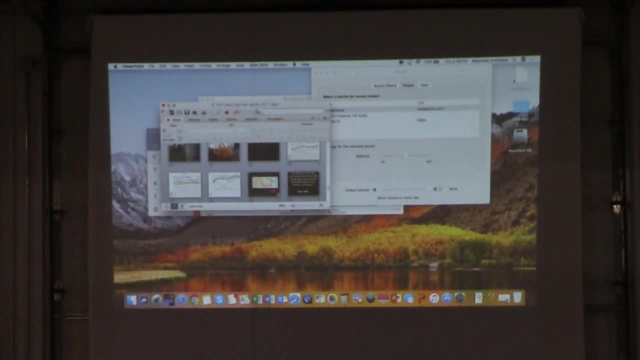 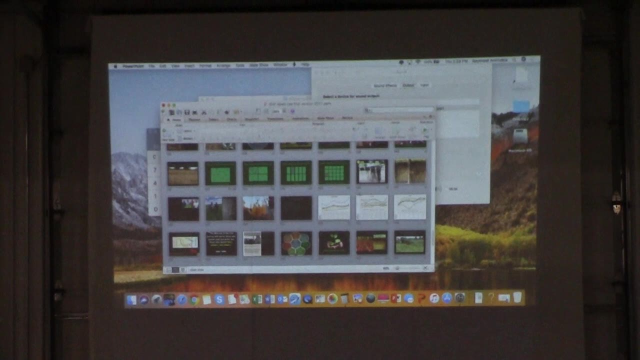 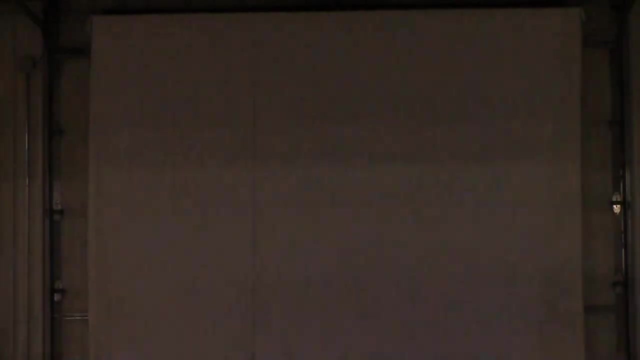 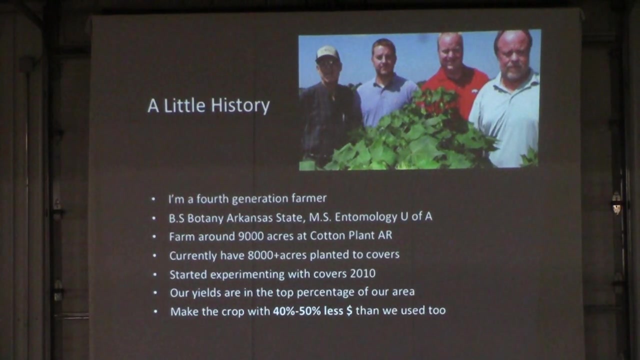 punchline because I got three minutes. Okay, here we go. It's a good way to end. This young man is pretty impressive. How many have been to Arkansas? by the way, That place looks like the moon. Love the people in Arkansas. But they were taught like the rest of us. Before I left I was responsible for Arkansas to do soil health in Louisiana. This young man is pretty impressive. He got his master's from Mississippi, from Arkansas. He farms about 9,000 acres. 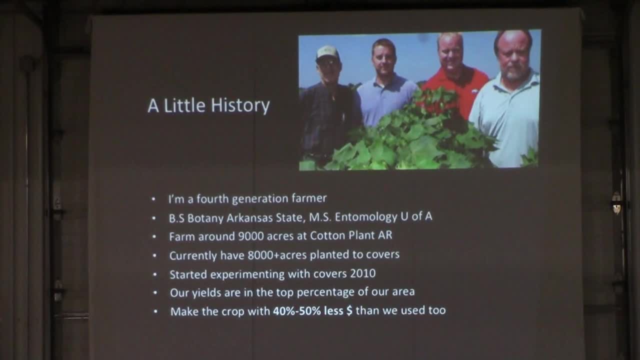 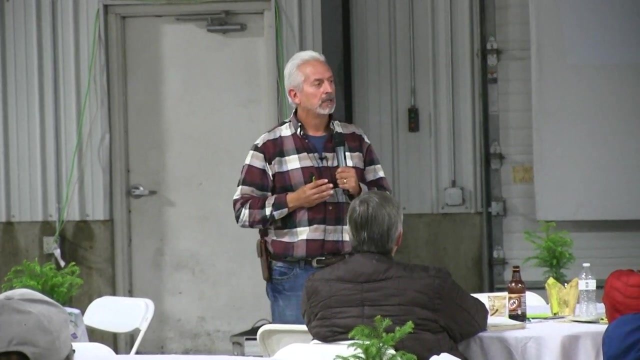 of cotton. He now has over 8,000 acres in covers. Adam, I said: my gosh, why did you do this? He says: Ray, we were desperate. I knew We kept going this way. We were bleeding. 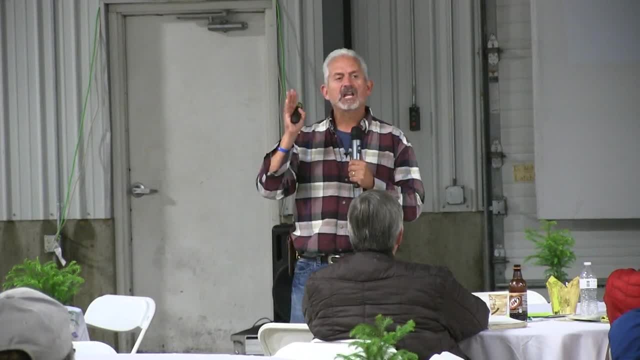 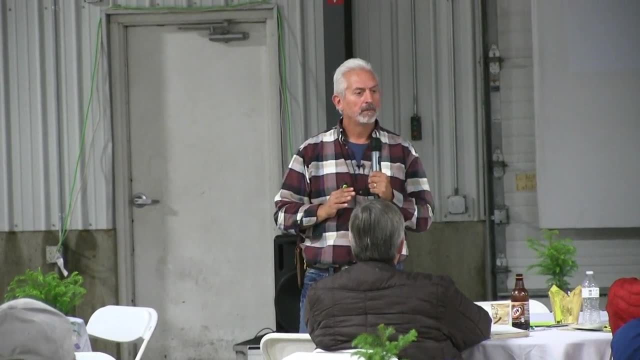 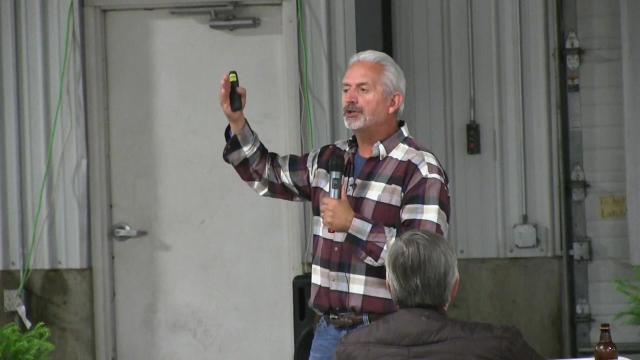 The pigweed was killing us. It was destroying us. These guys get 50 to 60 inches of rain guys and they still irrigate 60 inches of rain and they irrigate. The soils are so destroyed that all the water. 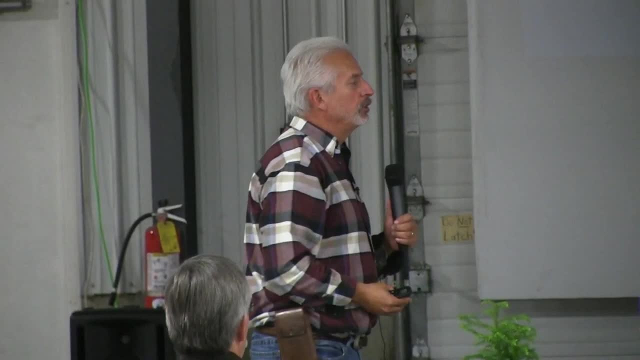 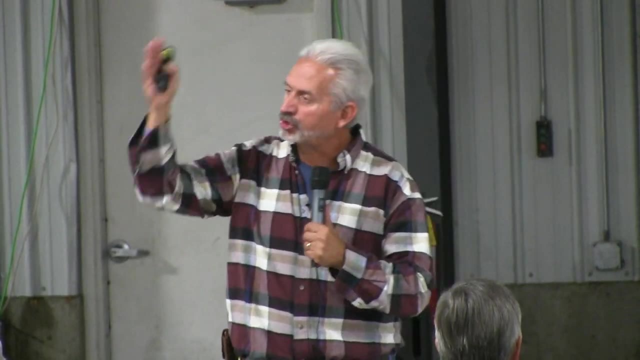 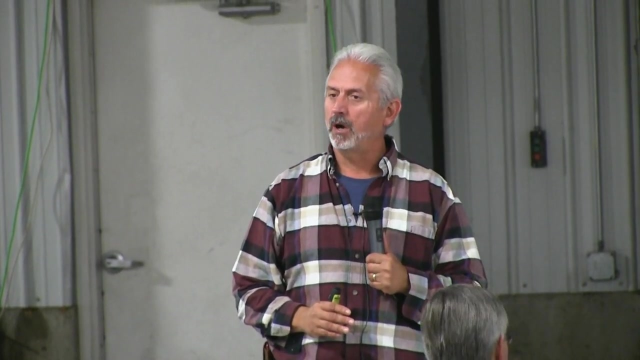 runs off Majority. I said, Adam, what changed you? He says desperation, Ray. I watched you and David Brandt on YouTube. I was one night surfing and I had to find answers because we were bleeding financially. We couldn't take this anymore. 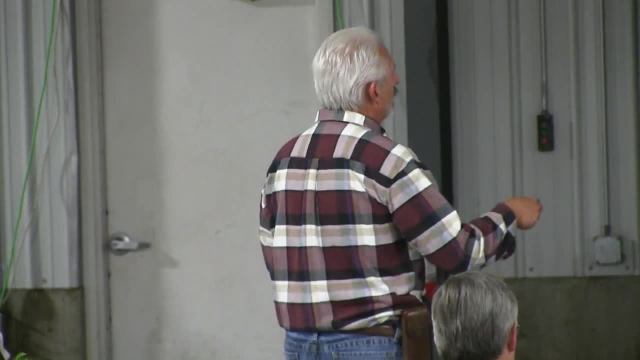 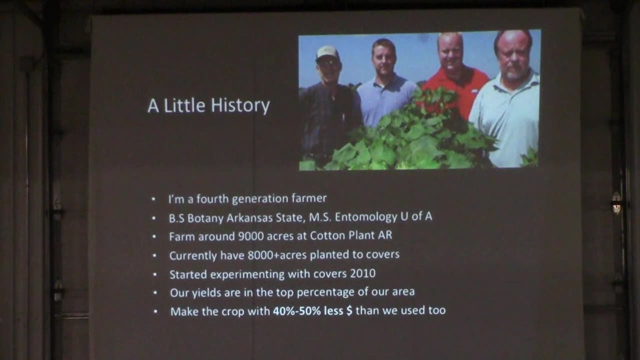 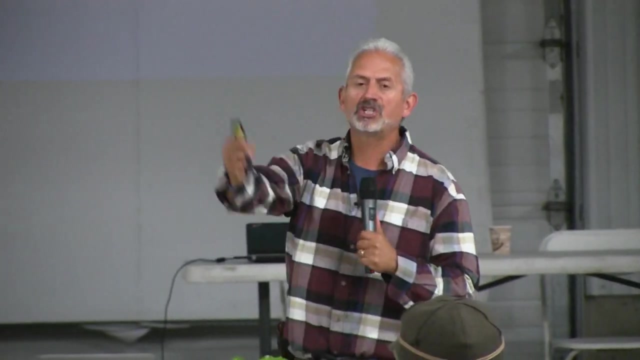 I said: my gosh, what did your professor tell you when you started using covers? He said: Ray, he told me that we were going to go broke. I said: how did you respond? What did he tell you? He said: you're going to be invaded by insects. 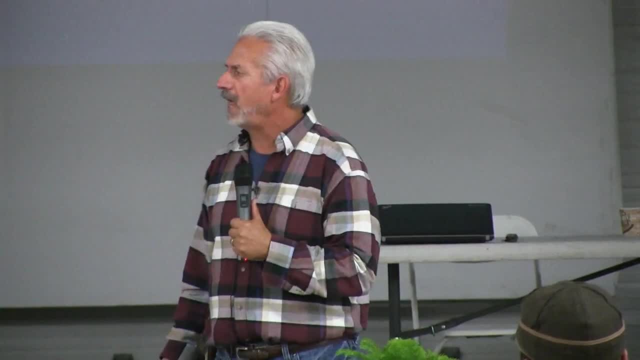 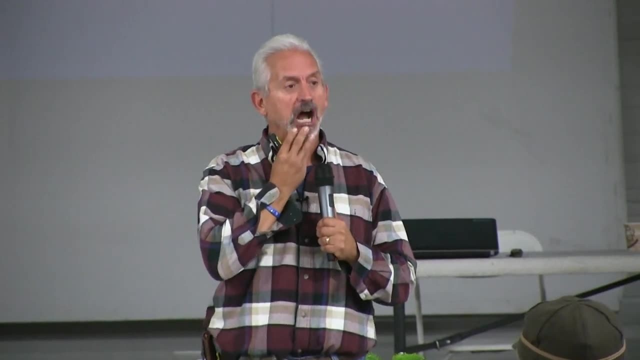 You're going to take all these pests. You're going to bring all this disease because your covers are going to do that. I go whoa. Does he believe in beneficials? There's 1,700 beneficials for every pest. 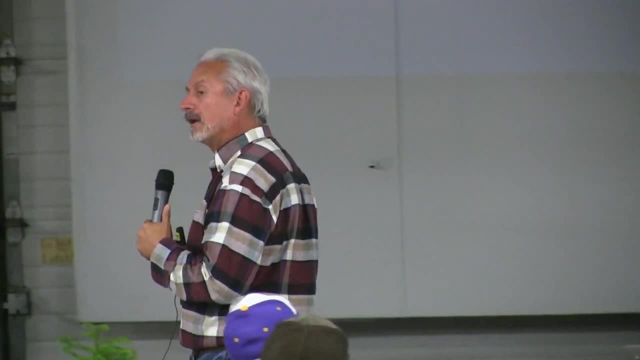 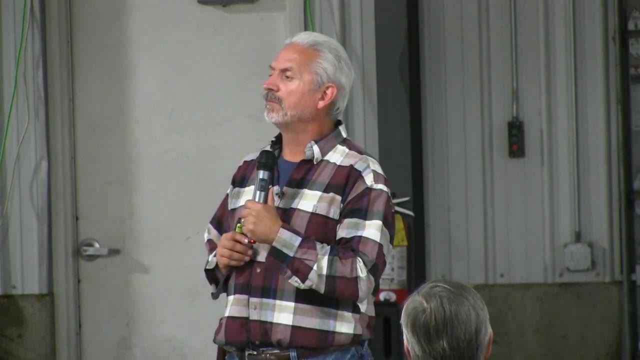 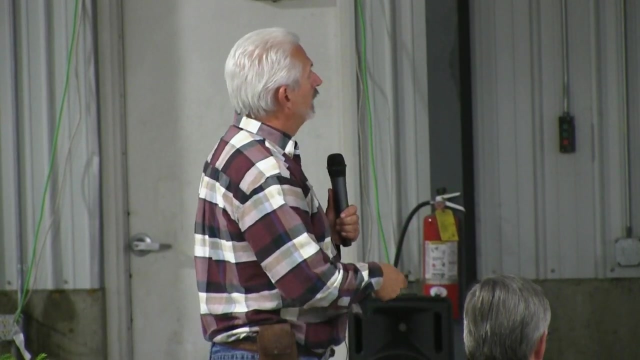 How did you respond to him? He said, Ray, I told him my brother and I don't get our research money from Monsanto, We get it from ourselves. He's now lowered his debt from $5.4 million down to $2.7. 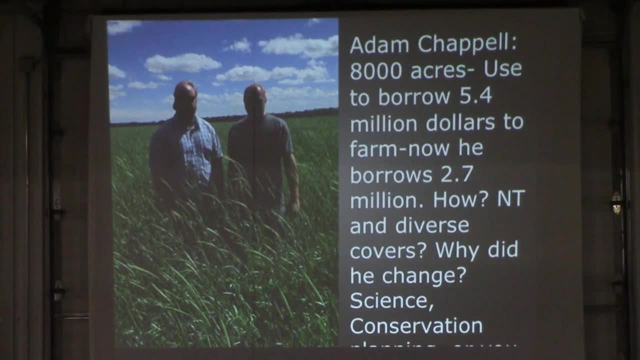 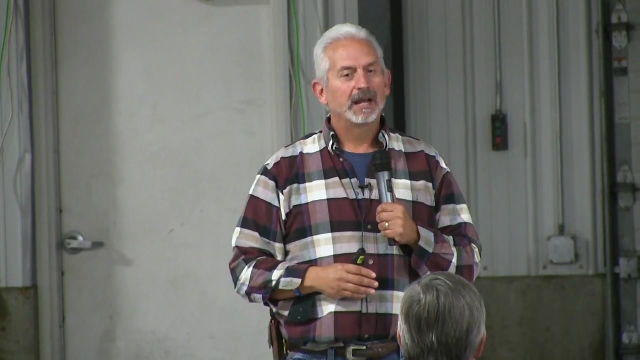 in five years, No-till covers is going to bring animals and sheep. He's so excited. He says, Ray, now we're going to do all kinds of other things. I'm going to have my dad paid for. Adam, would you go back? 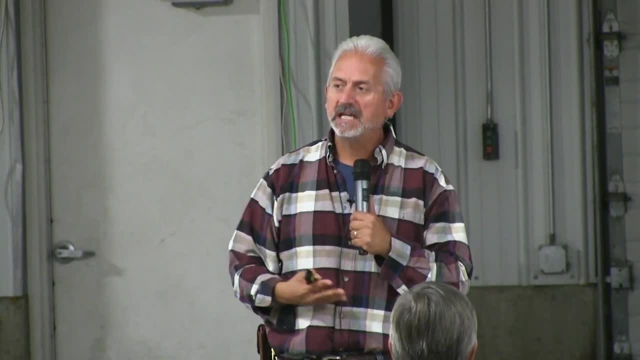 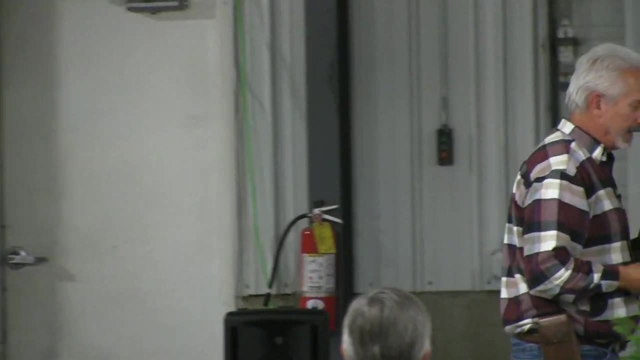 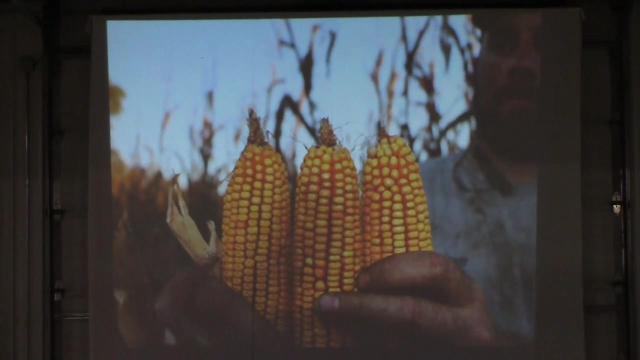 He said: never I'm making money. now I am flowing with the system, I'm working and collaborating with nature. It's changed everything for him. It's changed his whole life. Ladies and gentlemen, the last one, This young man, 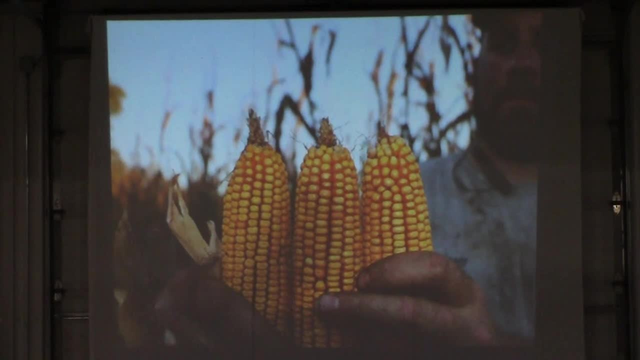 Russell Hedrick. If you ever get to Russell Hedrick, watch him on YouTube. This young man knows how to manage nutrients. He lives in North Carolina. Why is he such a good farmer? He never grew up on the farm. He was a fireman Wanted to. 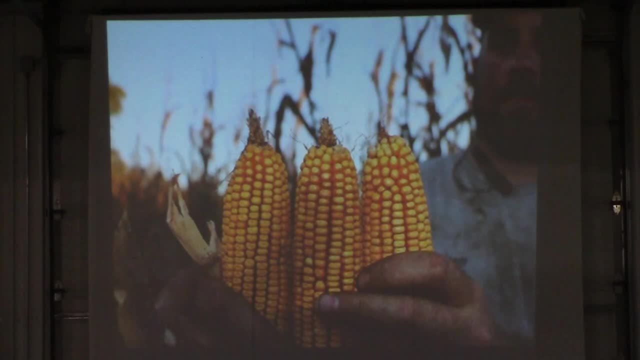 farm Started with four acres, 40 acres. Now he's farming 1,000 to 1,200 acres. People are saying: Russell, would you farm my place? I said: Russell, what did you do? He watched our YouTube videos. Now he's. 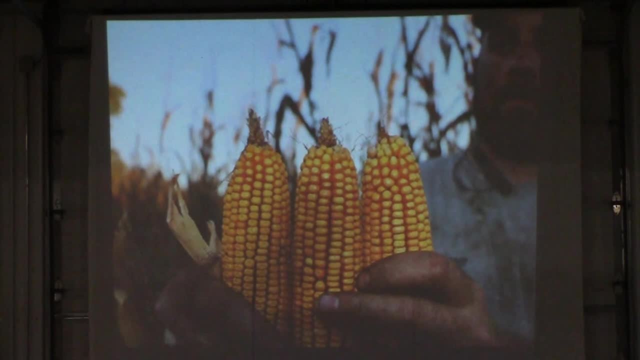 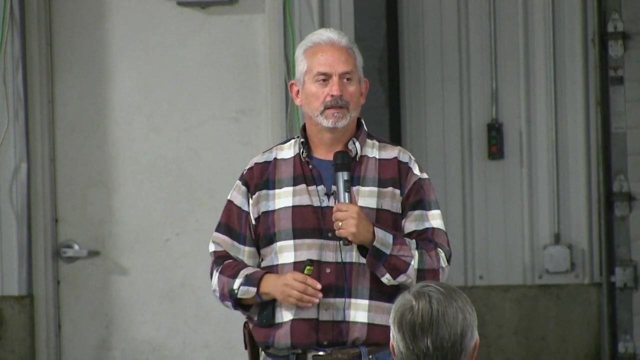 no-till cover crop. Last year, 2016,, he won the yield contest dry land for North Carolina: 318 bushel dry land yield With 140 units of end No-till multi-species- the Rick Haney test. 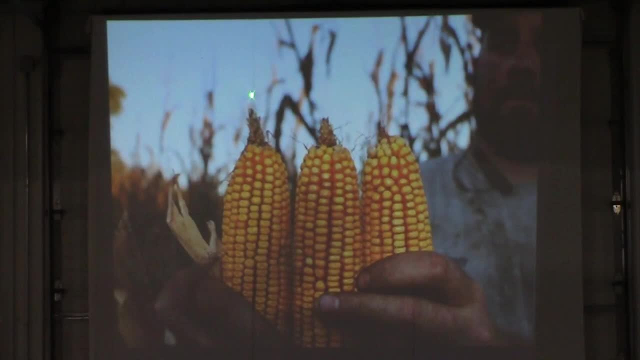 And he puts test plots all the time. Can you please tell me which corn is the zero rate, half rate, full rate of fertilizer? Anybody Which is the half rate, Which is the full rate? These are plots right next to each. 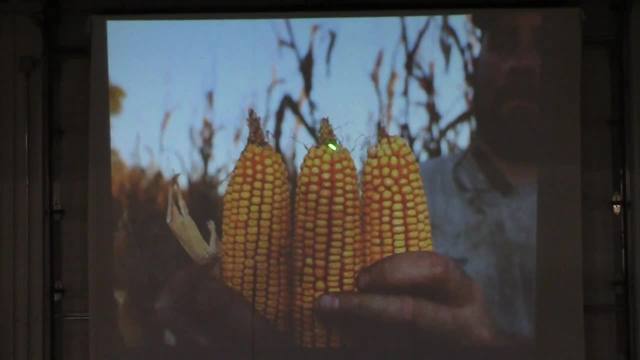 other Half rate's in the middle, Zero rate's on the right The right. It's actually the opposite. You're right about this way. Zero nitrogen half rate, nitrogen full rate. Only a seven bushel difference between these two.